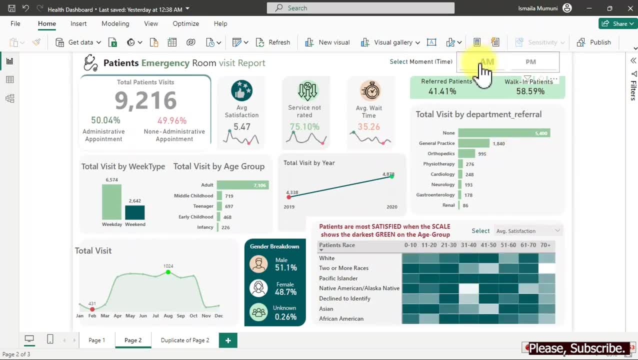 different. can you see it now, beautiful huh? so we can decide to check for people who visited the hospital in the morning, or we use the pm to check people who visited the hospital around evening and stuff like that. so when you click on this, you can see our dashboard changes and respond. 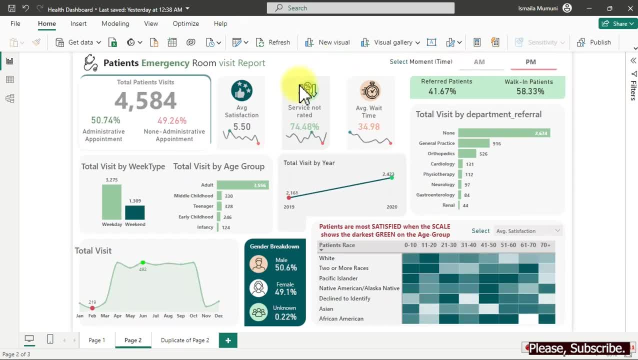 to filter exactly the way it should be. you get it, so this is exactly how it is. so we try as much as we could to highlight the most important part here, which is the month we have the highest and the amount we have the lowest visit just to make sure our line chart look much more beautiful. 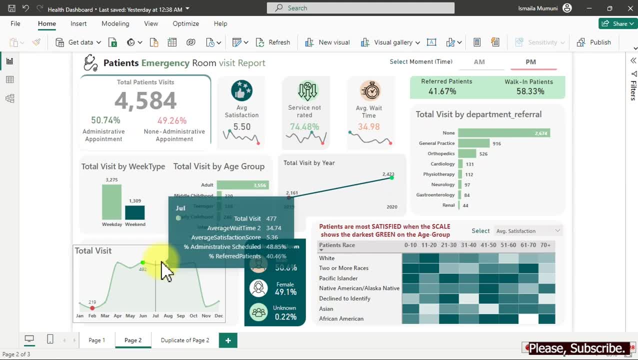 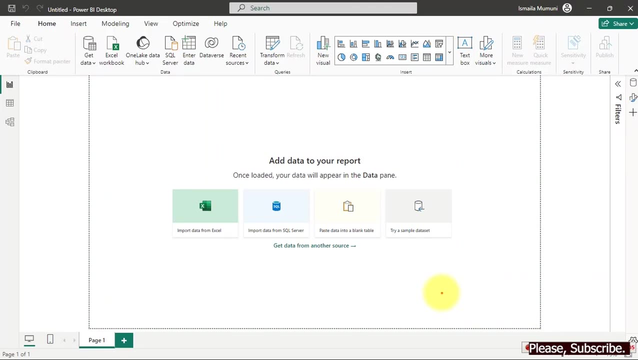 and out there. so enough of this talk. let's do the creation together. so don't forget to subscribe, hit the like button, share and leave a comment. let me know what you feel about this. all right, let's go ahead and get our data so you can actually use this particular. 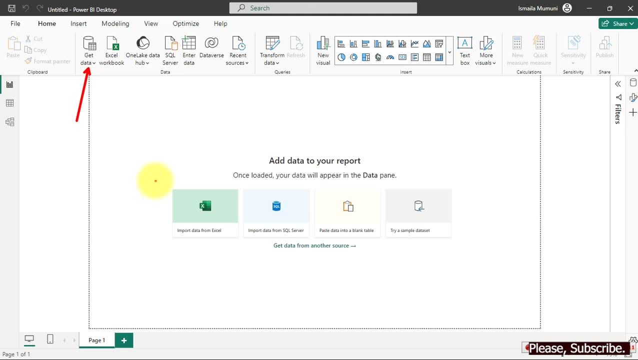 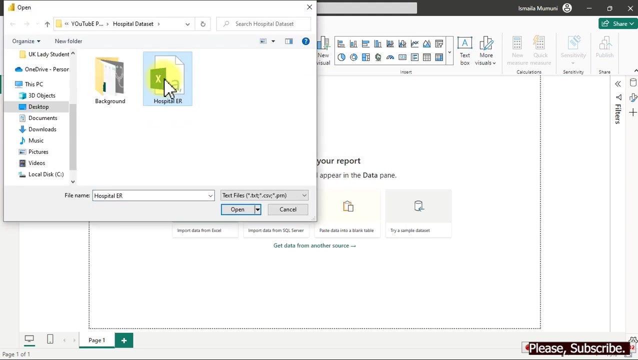 part to actually fetch the data you want to use. so if your data is actually part of those ones, so you can actually use either of those ones you have writing right now. so we are looking forward to getting data from csv so we can actually go into get data and here we have text slash csv. click on it so it lands you here. so here comes the data we 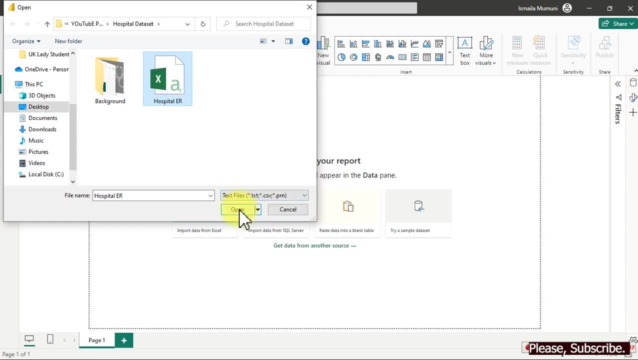 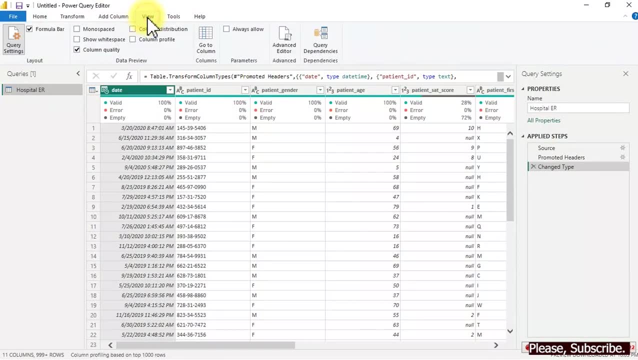 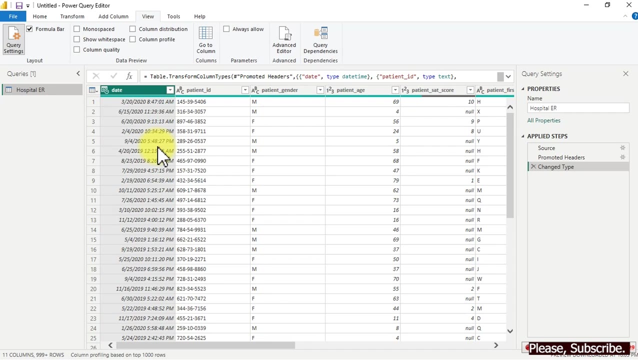 are going to use for this particular project, then i go ahead and actually click on open. all right, come to the parkery environment. this is where you have your data cleaned and transformed. so the very first thing you're going to do is to actually investigate your data and see the 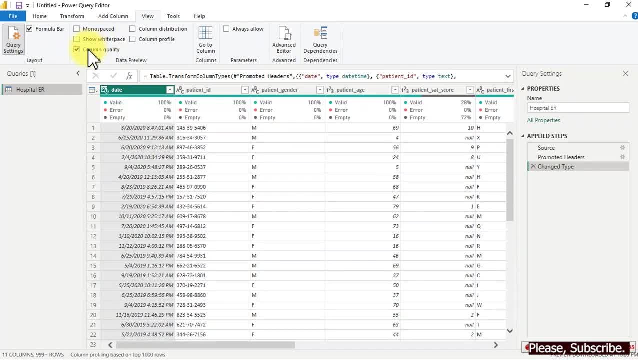 quality of your columns. that is where you actually go ahead and turn on this particular column quality. so that would be under this view here. so now, what do you do with this? if you actually look around, you can see here it's giving you 100 percent, which means there is no error. 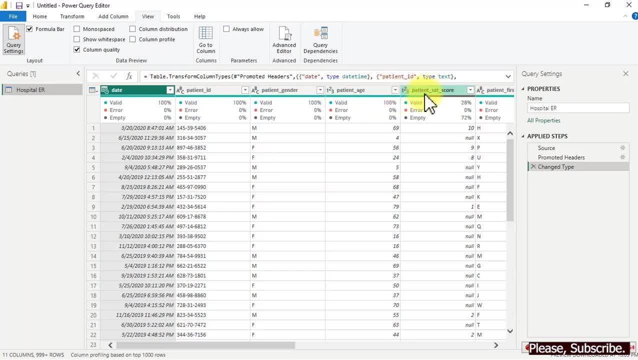 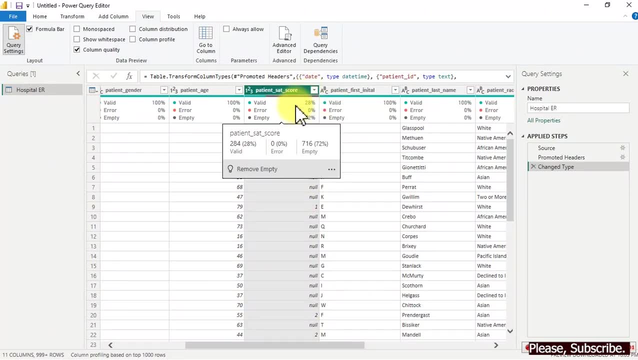 and there is no empty. you can just look around and see what it is. let's just look at this particular part here. this part says we have 28 percent valid and no error, but we actually have 72 percent- you know- empty. so the question you might have in mind is: what am i going to do today? is to make it some. 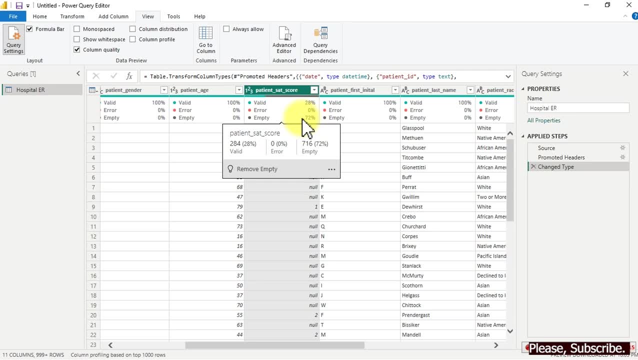 kind of 100. there is nothing you can do. leave it the way it is. don't replace the null with anything. that means this is actually a patient uh satisfaction skull. so it means 72 percent of the people that visited our hospital did not rate us, so we're gonna leave it like that. 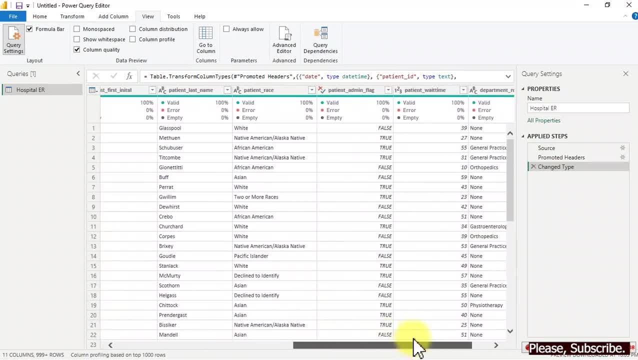 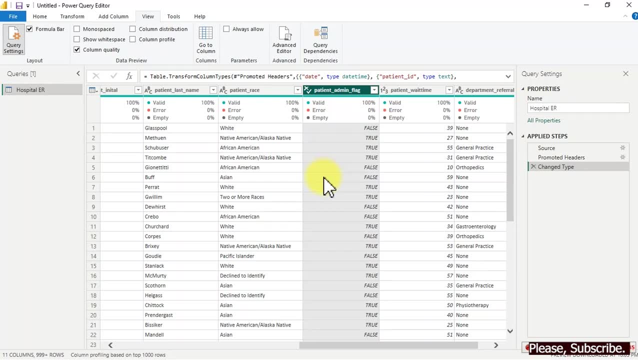 so, scrolling to this particular end again, i will definitely have. we have this here where it says patient admin flag. so this is what you might be having issues with when working with data. specifically, if you have not worked with this kind of company before, it would be hard for you to read all the columns to understand what is going on. 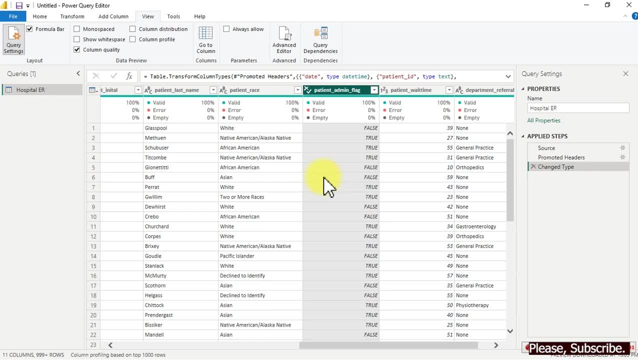 we have 100 percent valid, but what is the meaning of true and false? so you have to communicate with your manager or whoever is involved, a client, to tell you what each and every column is, or you have a data dictionary. so let's say we don't have anybody to actually assist us with that. 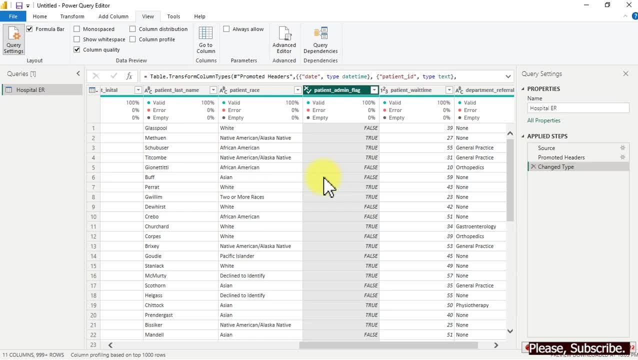 i'm going to actually help you now using ai. so what do we do? we can actually use ai to tell us what this particular column is and what we can get from it will be easily, you know, derived. so how do we do that? we're going to use chat gpd, so chat gpc does not actually take in huge amount of data. 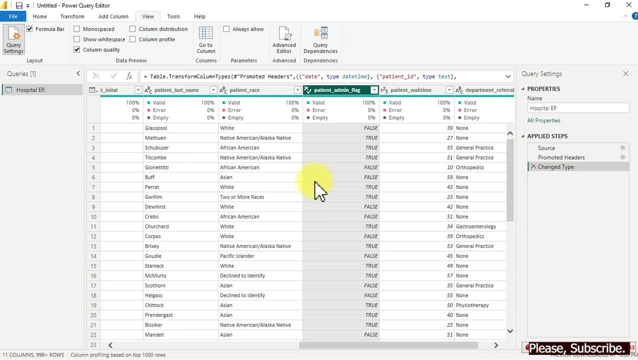 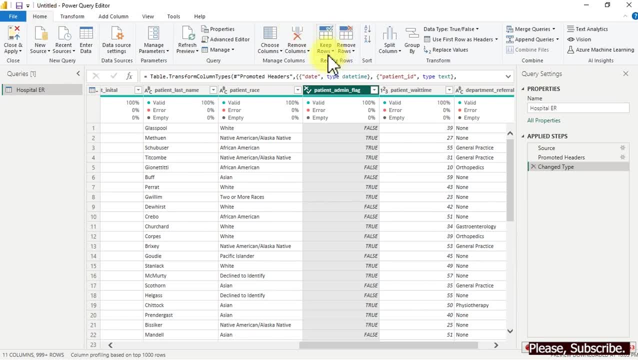 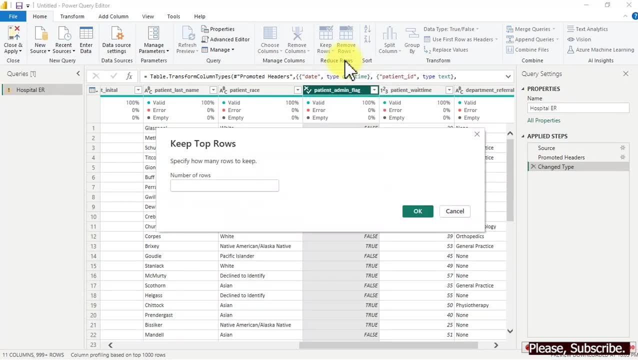 go ahead and click on home and from home you see where it says keep rows. then use this particular, keep top rows. so we have to specify how many rows we want to keep. we want to keep 10 rows. don't be panic, we're going to bring the remaining rows back. 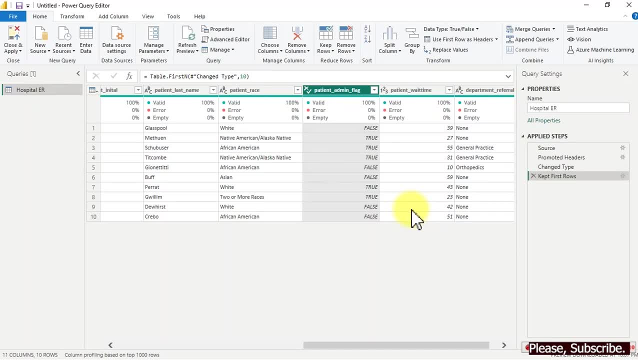 so once you have this, what do you do? you ctrl a. so once you ctrl a, it highlights everything for you. then we ctrl c to copy. we've just copied this to call clipbuild. then we ctrl c to copy. we've just copied this to call clipbuild. 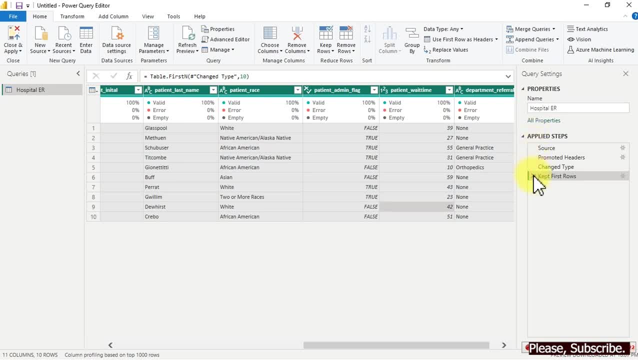 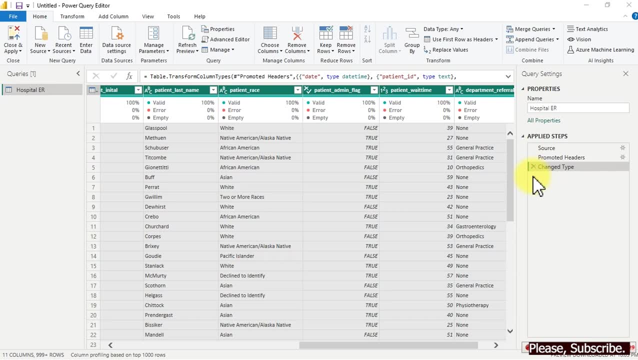 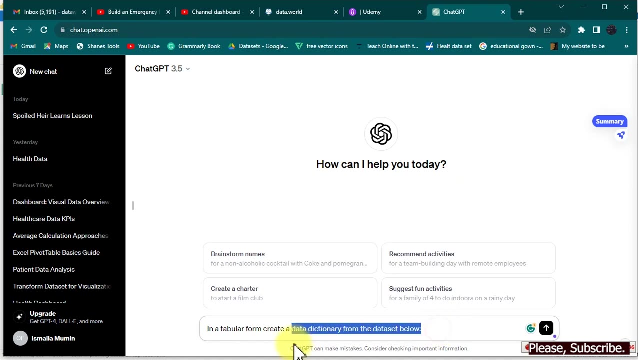 we can release this. so remove under applied step. just remove this particular keep first row, then we have all the full data back. so it is the time to head on to par on the gpt. all right, here in gpt i have a prompt already. the prompt says in a tabular form: create a data. 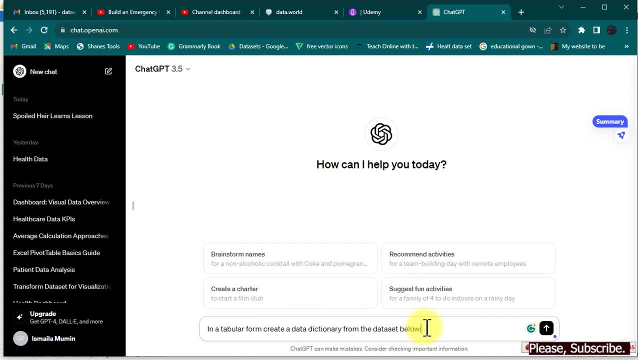 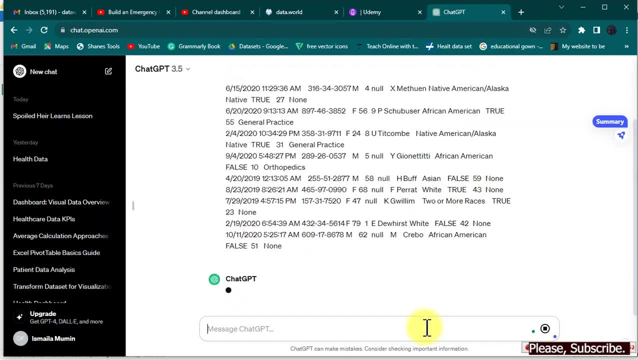 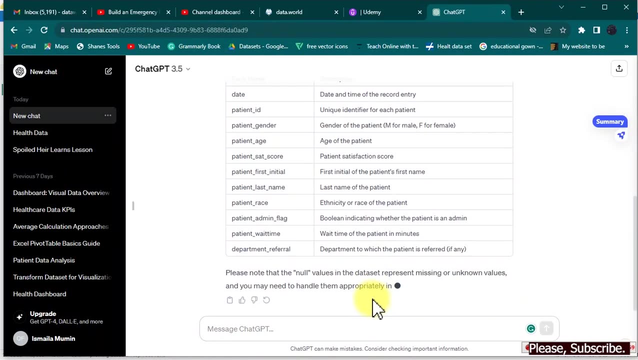 dictionary from the data set below. so what am i going to do? i'll hit shift enter key to paste in the data i have copied. then, if i hit my enter key right now, this is going to help me to create a data dictionary from this data that explains what each and every one of this column is. 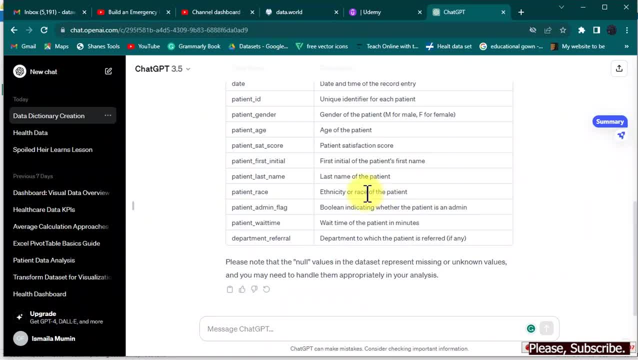 so if you look at it here, it's giving us everything we need to know about this. so this is where we are really much important interested in. so it says boolean indicating whether the patient is unadmin. you got it now, so what are you talking about here? 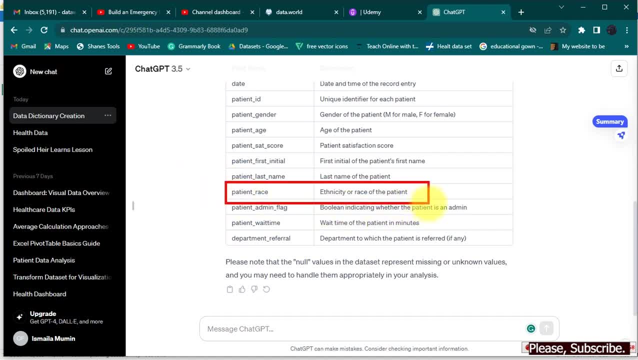 so this is the part we are trying to actually on this. okay, not this part. this is the part you're trying to understand here. so what it is saying? it says: patient admin flag boolean indicate whether the patient is an admin, which means whether the patient is a staff of the what of the hospital. 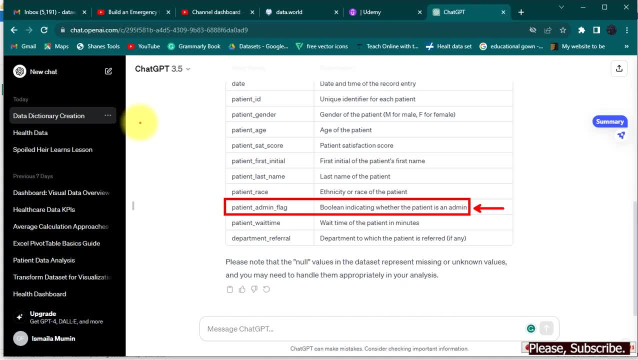 so in my country we have a hospital that is actually a custom, a custom hospital. so this custom hospital- if you're a custom staff, even if you're not a direct staff- maybe, uh, your father is a staff, or is a staff, or is a custom, or is actually part of the 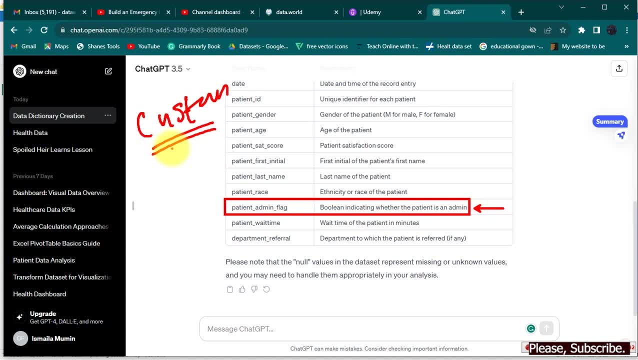 health. you know um individual right there, so your cost will be lesser compared to somebody who has no any connection to staff, you understand? or if you're actually part of nhs. nhs is just like an organization that actually gets your money every single month to help you subsidize your hospital. 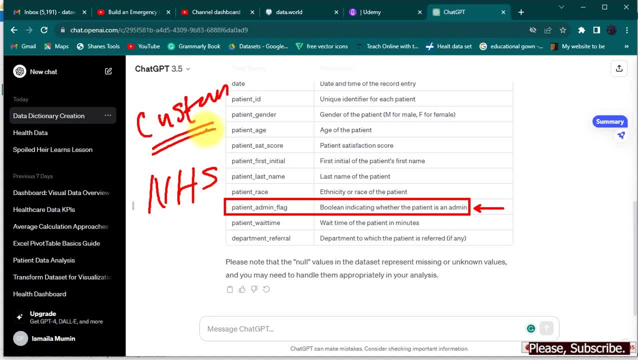 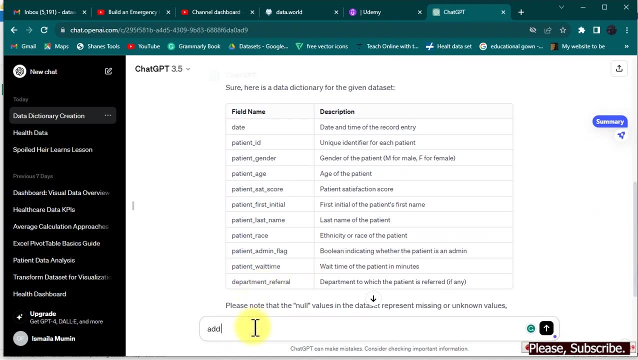 bill when anything happens. that is what nhs is. so this is exactly what is particular, particular heart is talking about. so in case you're not some kind of satiated, you know, with what you have as a data dictionary, you can further prompt the system like add a new column. 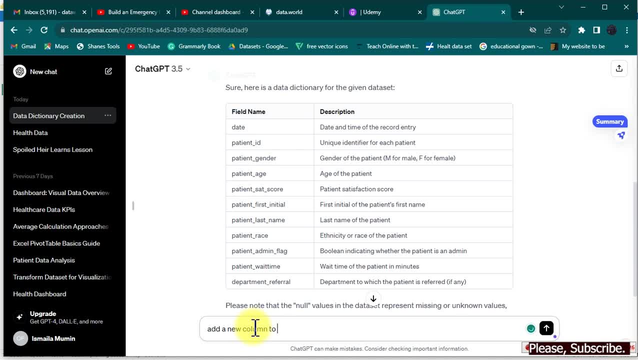 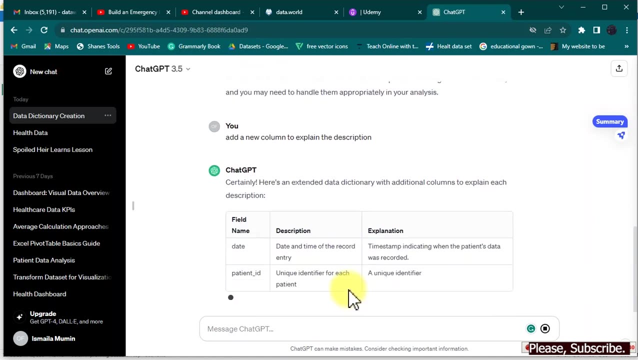 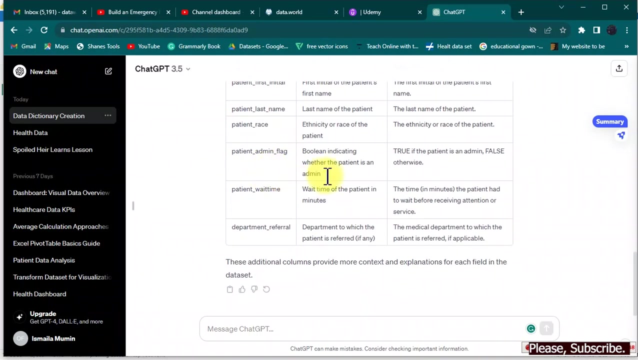 to what? to explain the description. so this is going to actually add a new column to this description to explain, to further explain the description you have here, you understand, so that you can actually have much more understanding than what we had, just what we just looked at. so now it's. 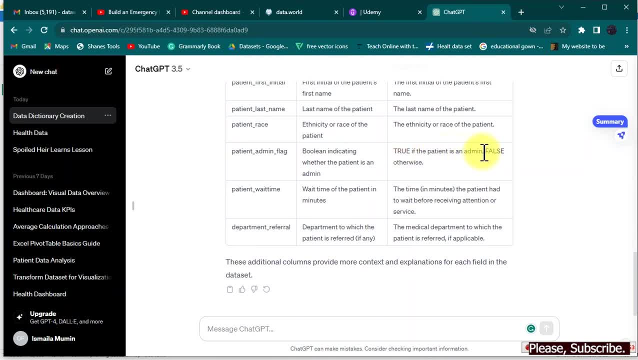 telling you: true if the patient is an admin and false if otherwise. so if the patient has admin privilege, it will be true. if the patient does not have admin privilege, it will be false. now we have learned this. how can we use this is very important. so, on that part, you should actually consider looking at and understand what. 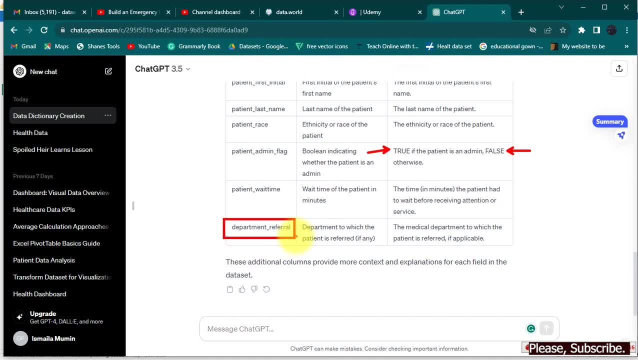 it is. it's actually departmental refer here on that. this department refer is actually telling us here that departmental who's the patient is referred, if any. so the medical department to which the patient is referred, if possible. so it depends on what brought the patient into the hospital maybe, uh, you have eye problem. so 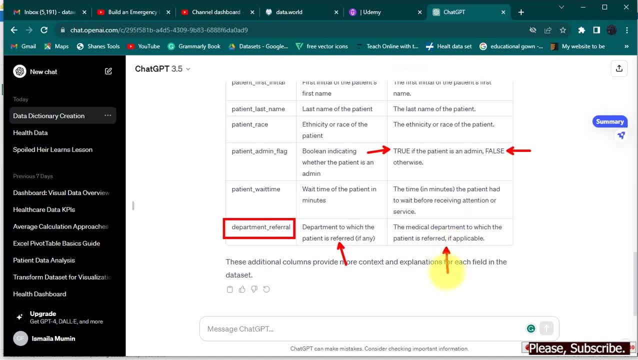 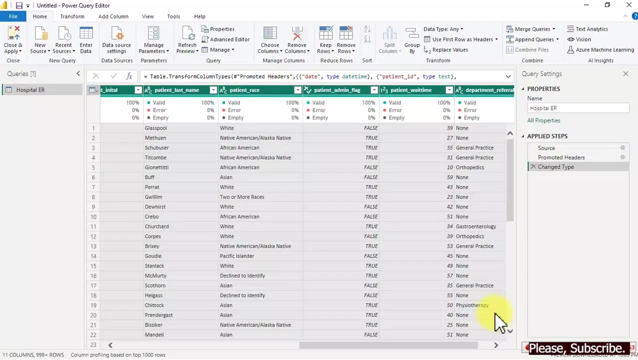 you have a speech impediment into the hospital, so you have to see a doctor that is specialized under that particular, you know condition is what it is. so, in order to have looked at this here, it is time for me to head back to Power BI and specifically Power Query to start looking at. 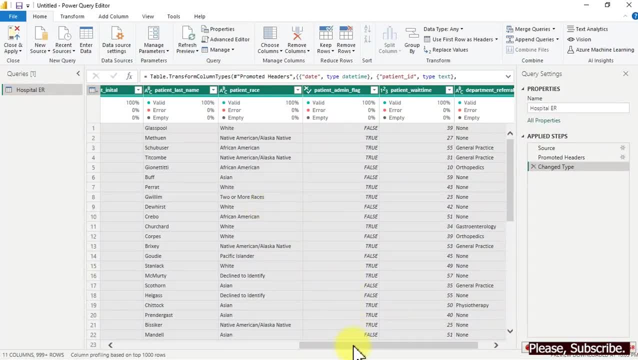 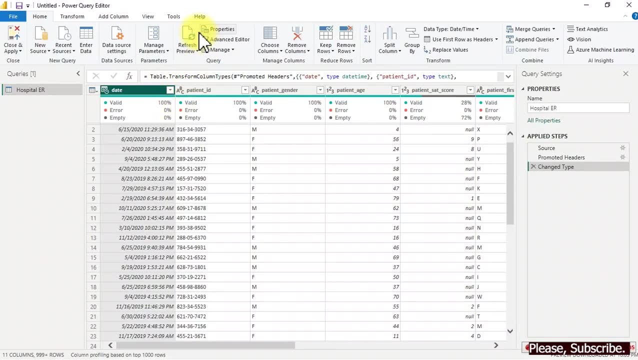 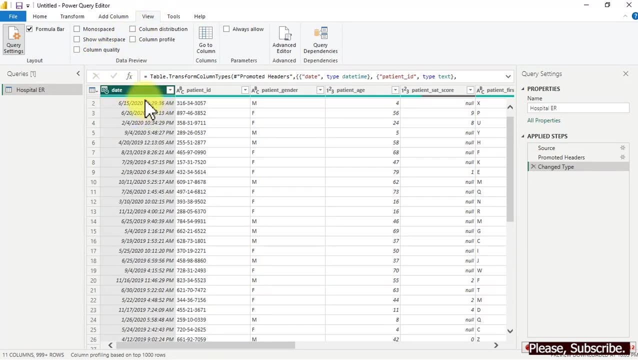 how to transform the data. all right now, if you look at here, we have this column that contains date, time and the PM and the AM. so we don't actually want the time, we want the date. but before we actually format it to what we want, we want to extract a particular part of it. so I'm gonna actually click on my add. 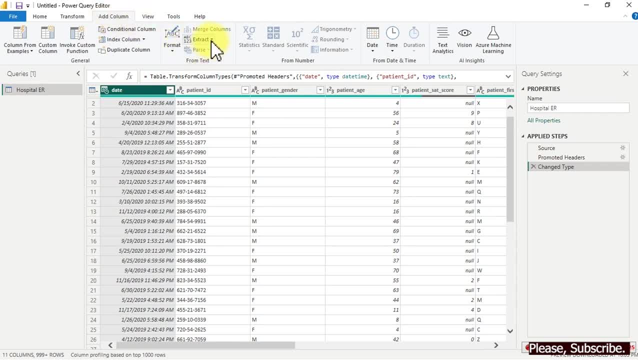 column here on the add column I go to extract. so before you use this particular part of it, you have to be very sure that your the what you're going to actually extract is consistent. so what am I talking about? my AM is two characters, so so PM. so if we have like VMC, so now we cannot use this particular. 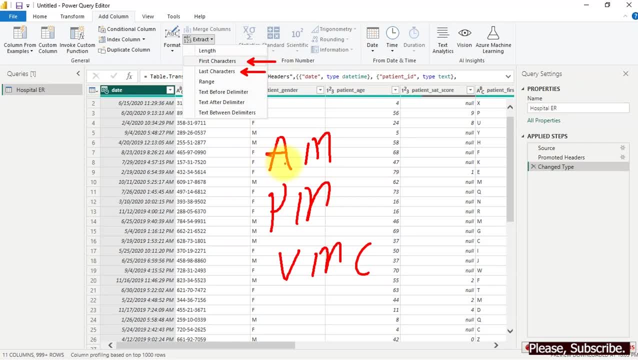 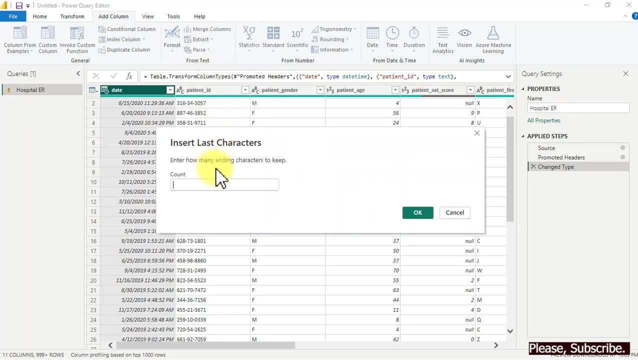 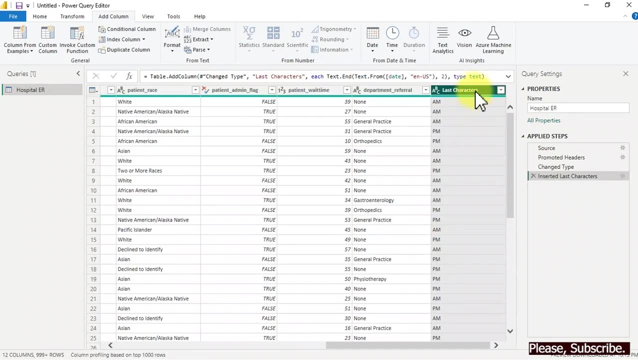 one and this one to extract it because there is no consistency. so understand that. so I'm gonna choose last character. so for the last characters, I want to retrieve this last two characters because it's consistent. then I'm gonna click on this. here we go, we have it, the AM and PM. so all we just have to do is to rename it. 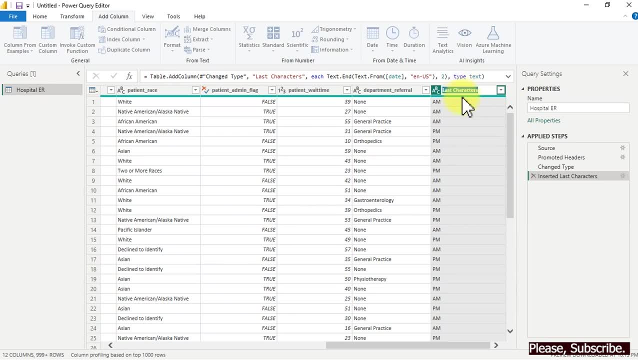 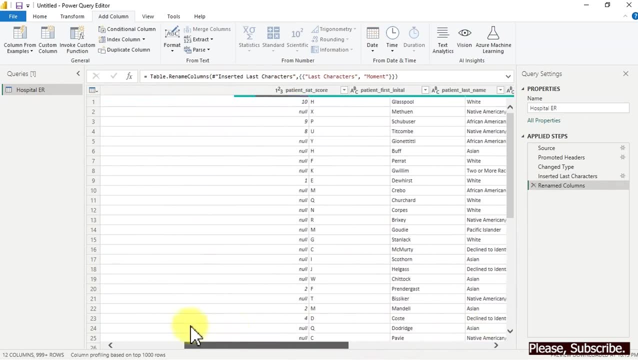 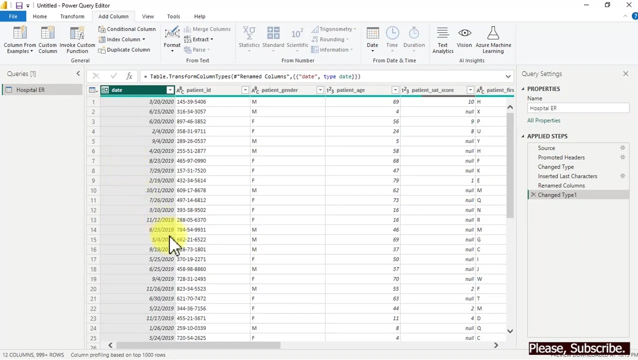 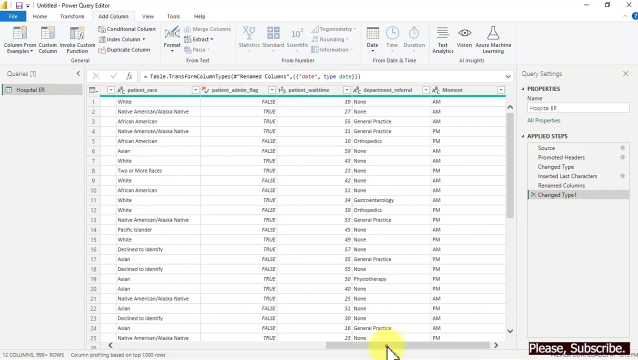 to something that would actually make sense. so we're gonna choose moment here. then I can go all the way back here and now turn this into a date instead of date and time. beautiful, we have it. I think there is nothing more to be done here for now. we are cool, we are good to go. we can start going. okay, one. 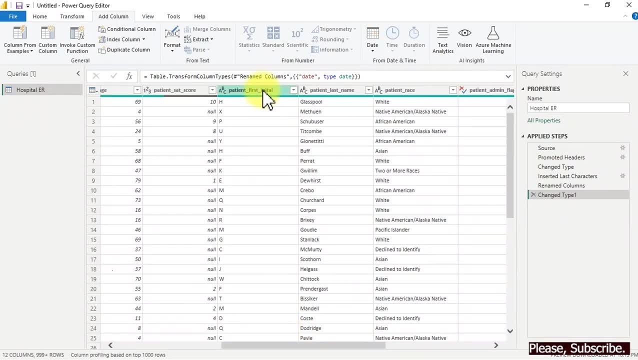 Martin, before we go, what if you want to analyze with the patient name? we might have one patient named John in the last name. so what can differentiate that particular default John from the second John and third, John is actually the initial if you don't have the first name. so what you can do now is to actually 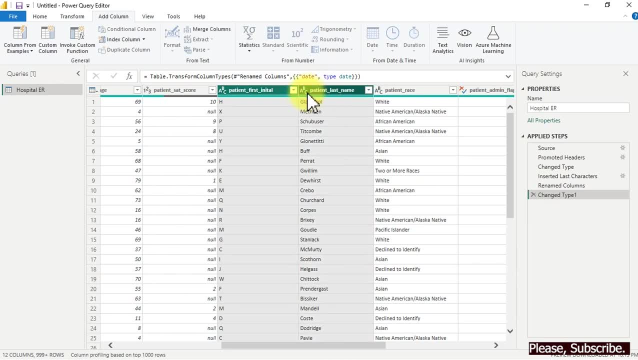 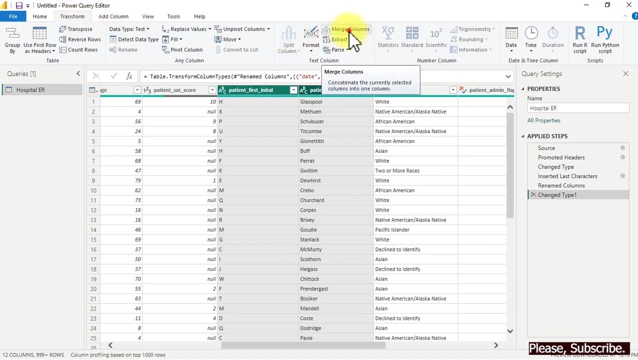 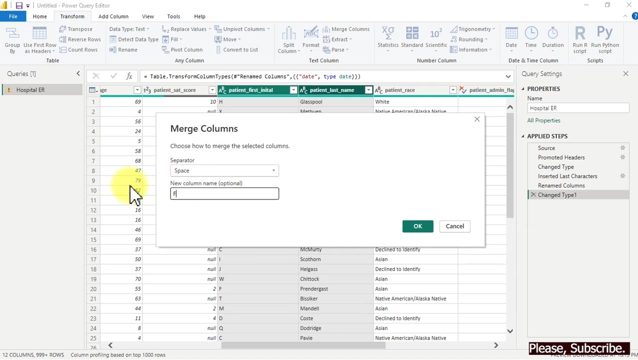 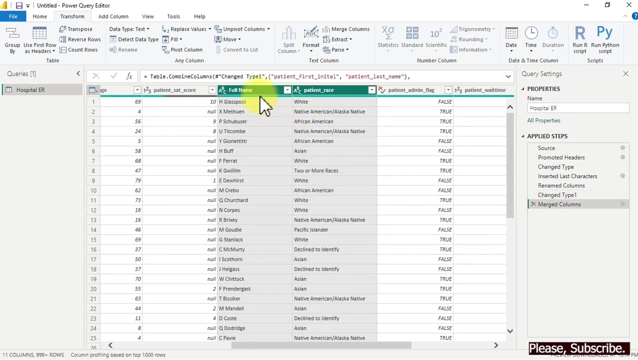 make sure you actually combine them together. to combine them, don't do it on add column, go under what, go under transform, and you're gonna see where it says merge column here. so for the delimiter you use space, and over here we type what, we type full name. then we can click on OK. so there we have it all. 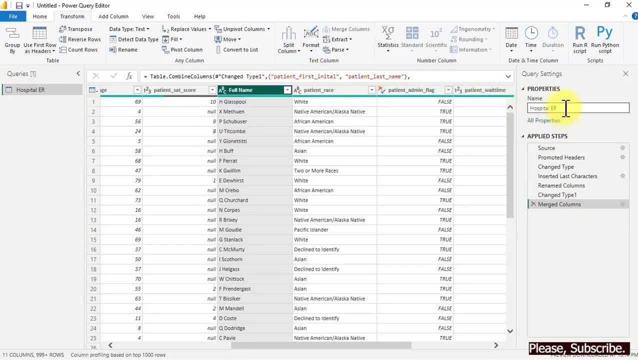 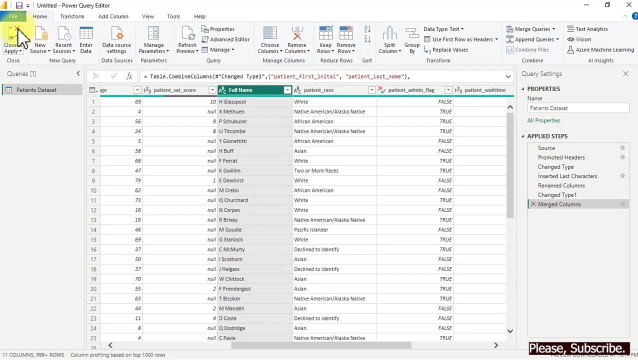 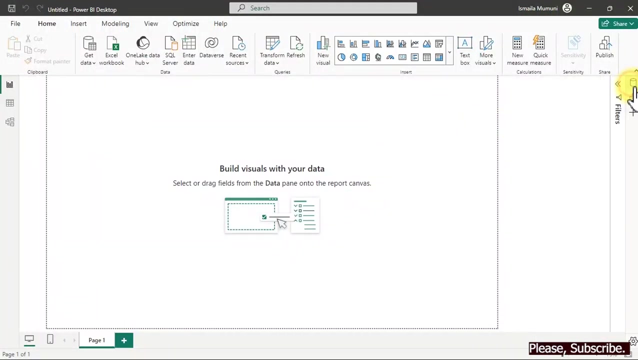 right with all of this, we have one more thing to do before we go. I don't like to keep my data with this kind of name datasets, so I have updated it all right. the next thing is for me to actually click on my home and close and apply. all right, now we have our data right in here. 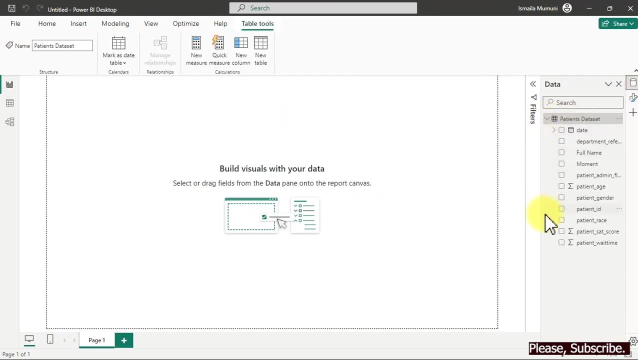 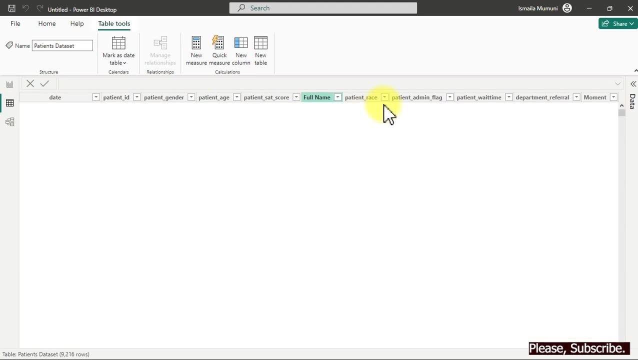 for us look at it. if I open it up right now, we have all the columns, and if I come right here, you can actually see the physical table. you can actually see the physical table right in here. so this is exactly what it is that we are looking forward to. 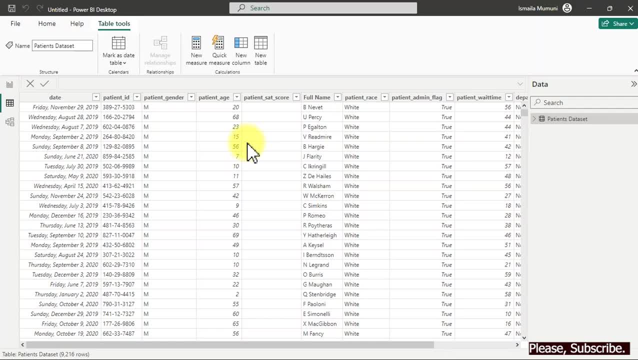 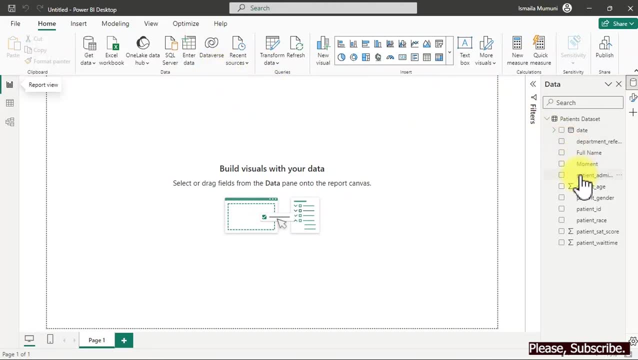 saying: okay, very simple data. what do we do? first we need to actually create a table where we can store all our measures. right then we start actually combining our measures in this table, so we click on what we click on enter data. you can decide to actually create the measure, to create a table. but this is 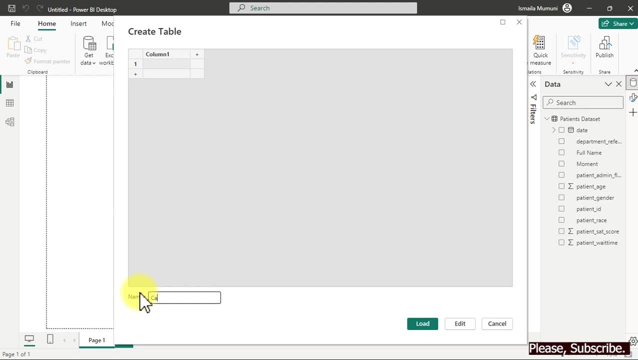 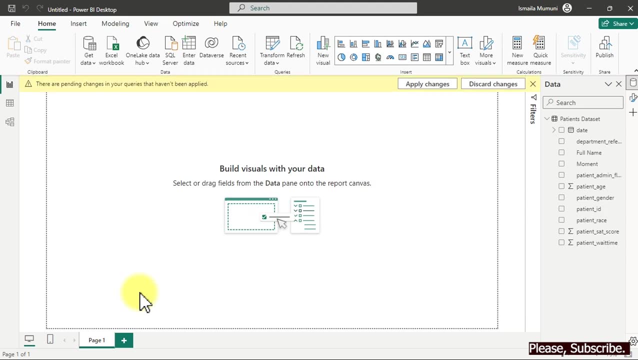 actually much more easier, so I'll do calculate. so now we just bring it into Power BI, so we have a table that is actually a disconnected table from this. it does not have any connection. all we just want to do is create in our measure in it. okay, what is the first measure we want to? 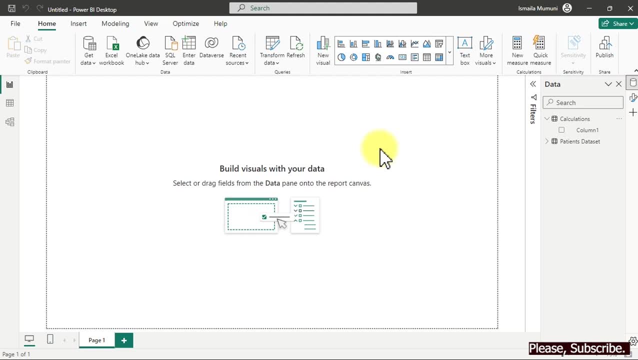 create. the first measure we want to create is actually counting how many patients that we have over time. all right, so we click on new measure here. so with new measure being clicked on, we are going to name this. so let me just zoom closely for you to see. 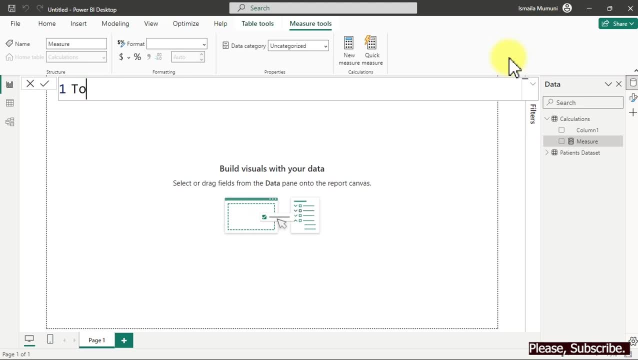 what I'm doing. so we just name this total patients. so, with total patients, all we have to do is to count our rows, and which rows. we're counting the rows inside our full table. I'm talking about a patient data set, so if I type patients here, sorry, if I want to do that, I would have to use a. 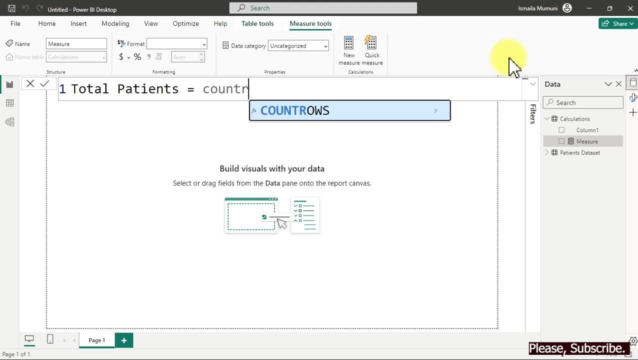 function, and the function is nothing but controls. so the controls function would be looking for what we'd be looking for: a table. if you're just joining this particular tool, like you're actually using Power BI for the first time, this is where you have to be paying attention, pay attention to the intelligence here. so 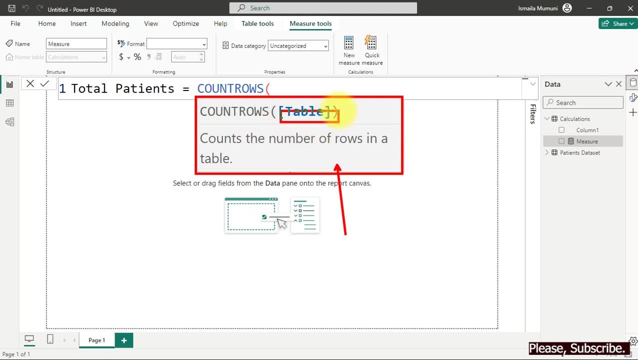 that you can know what is the set number, and then, if I want to do something like that, you will have those set numbers over here, and so what it is you have to supply to count rows. before count rows return what you want to return, and if you read this particular part, it will definitely give you the idea of what you would. 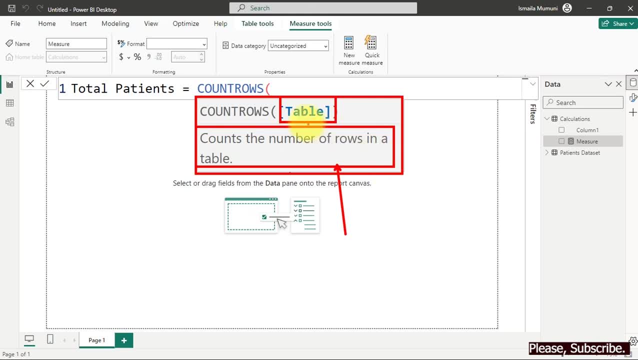 be having back. when you actually provide to it a table, it will give you the count of rows in your table without any exception. all right, so what is the table? the table is actually patient data set. here we go. so i'll go ahead and click on enter so that creates the numbers of my 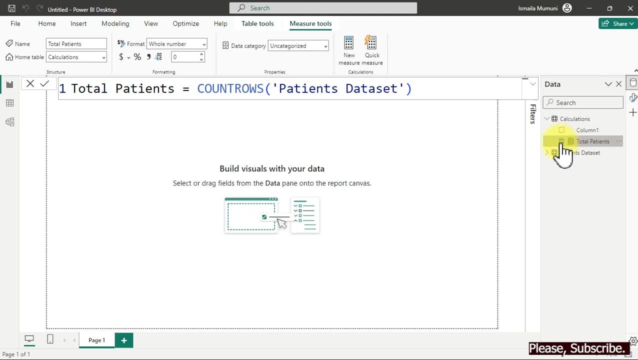 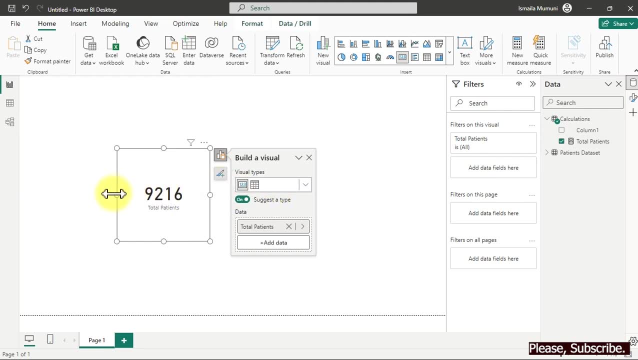 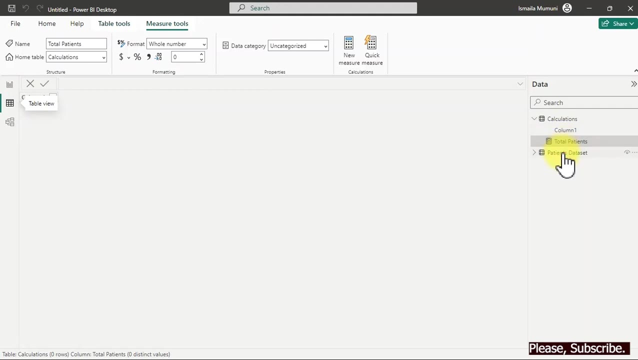 patient for me, then we can push this into a card. if you look at it now, it's okay, we have the numbers. if you want to verify this- we don't have huge amount of data- we can always go back here and we click on this so we can see. we have the count of rows. can you see beneath here? 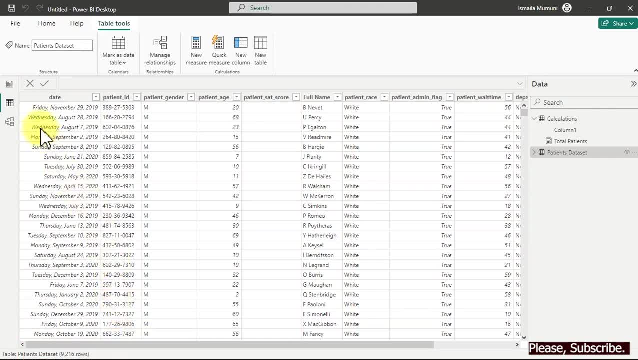 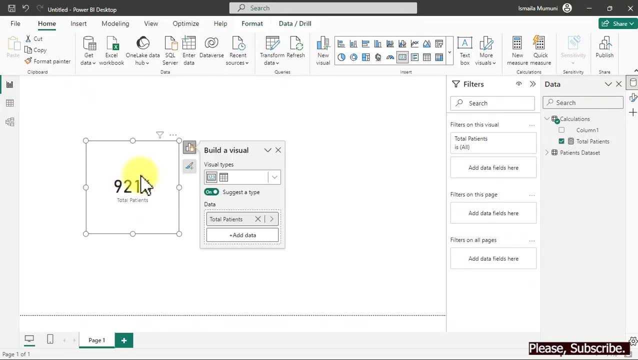 this is where we have it. so if what you have there is different from what you have here, which means what you have written as a DAX code is wrong. so there is one more thing: we need to actually add what. we need to add a comma separator. to do that, go back and click. 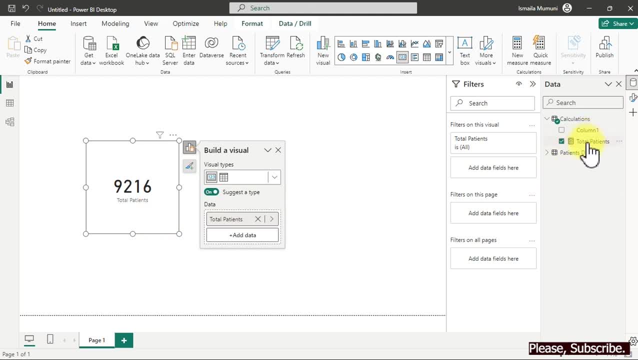 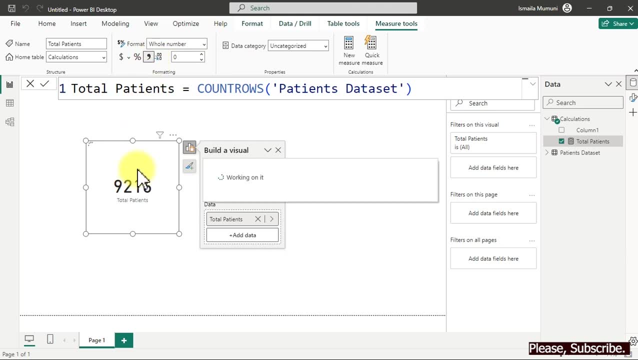 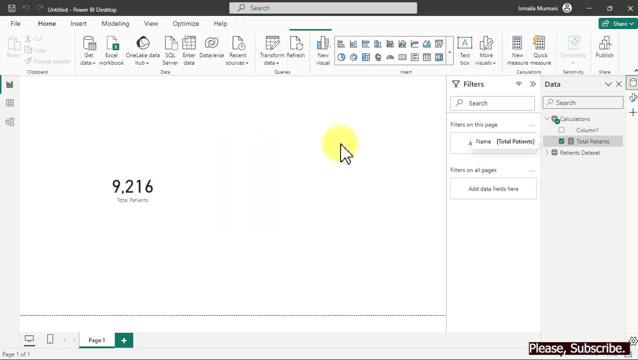 on the measure you have created. so once you click on it, you're going to actually have this particular part. you use the comma separator on it, then that will definitely separate this for you in thousand. all right, remember that particular true and false that we have. so it's time for we to make sense with it. what are we trying to do? so we're 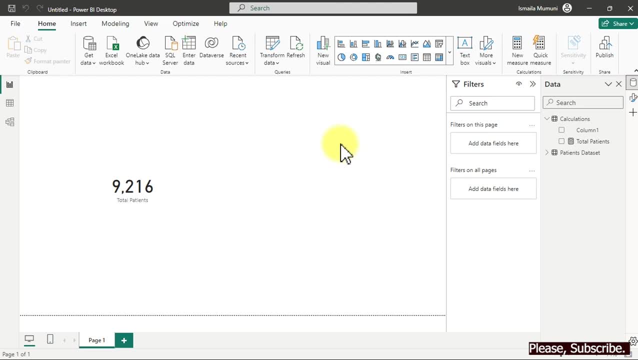 trying to actually look at those people that actually have admin privilege and those people that does not have admin privilege. so how do we do that? so, for example, we have a new measure. so first of all, let us just make this some kind of stay here, then we add a new measure. 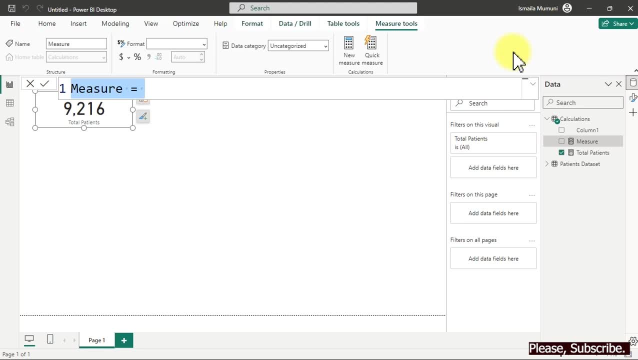 so we are not looking forward to showing the numbers. instead, we want to show the percentage of people with admin schedule and non-admin schedule or privilege. so what i'm going to do is actually say here: percentage and non-admin administration, administrative rather schedule. all right, so here we go. so what i'm going to do right now is to actually divide. 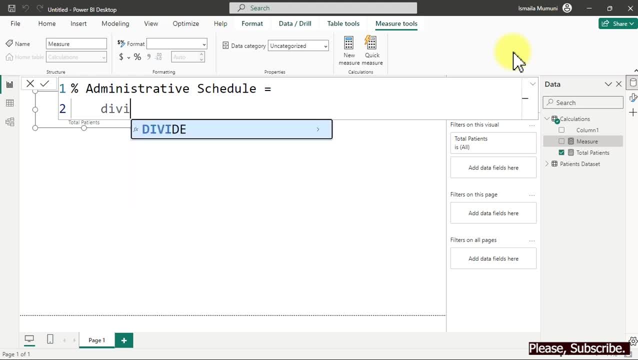 what i'm going to divide. so inside my division, if you pay attention, now i've told you always pay attention to the intelligence and now i'm going to divide what it is that you need to for the numerator. here i'm going to actually filter my what i'm. 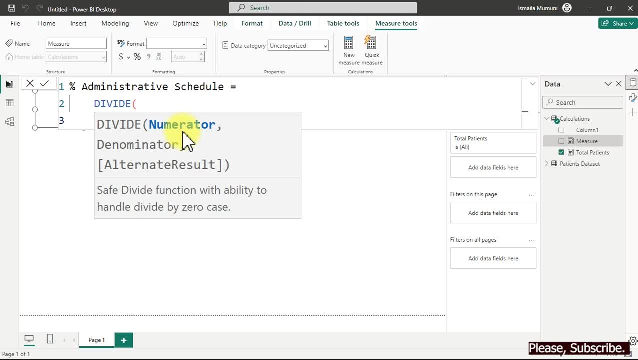 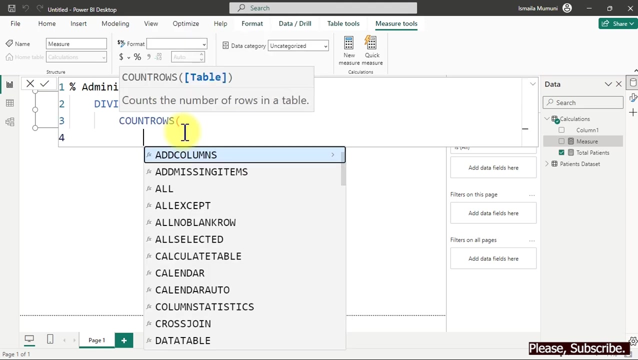 going to filter my main table and when i filter i want to actually count how many people actually have administrative privilege or where schedule under administration, wherever. so that is where we have true and false. so i'll use count roles inside these controls. i'm going to actually tell controls that you're going to count this particular table called. 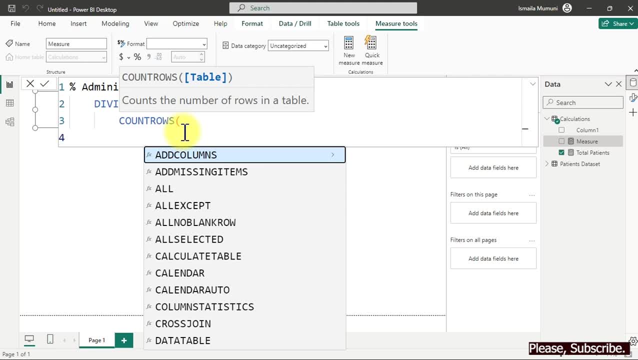 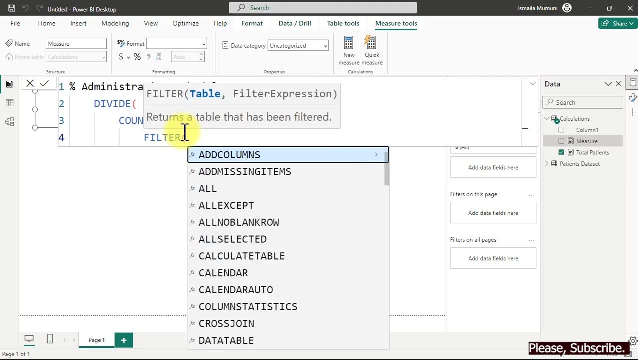 patient data set, but not all. you have to actually make it a specific row or some specific rows. i'll use filter to filter how many rows i want to count. so filter, okay, and then after that you'll be asking me for a table. if you read interlezans here: 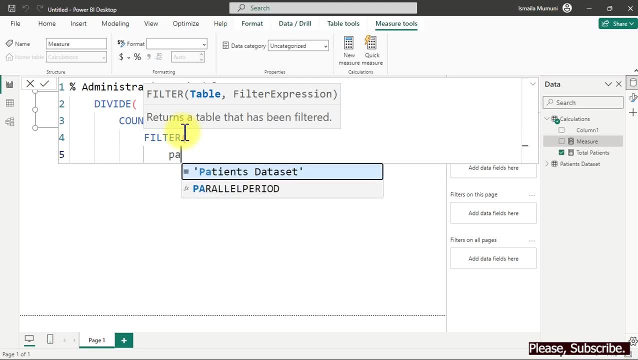 it says it's a table, so i'll put this patient here. so the second one is the filter expression. please always use this part to guide yourself through what you need to provide next. okay, that is the expression. the expression now would be a column. and what is that column column will be our patient. 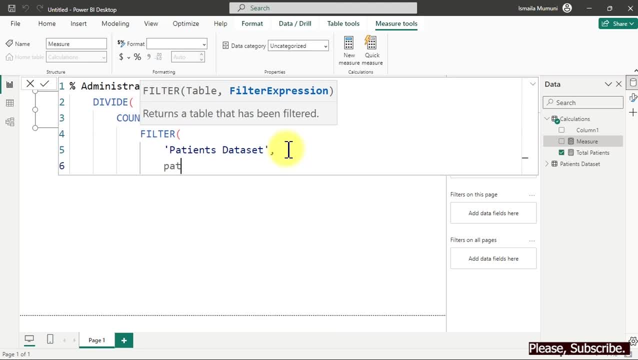 ının, our client floor, and he has the ordering and organization. no, we set an opening that was to be created. then, frame area icon: those quienes indicate we set words. i'm going to make this as a so here we go, patient admin flag here. so we wanted what it is equals to true. so if you 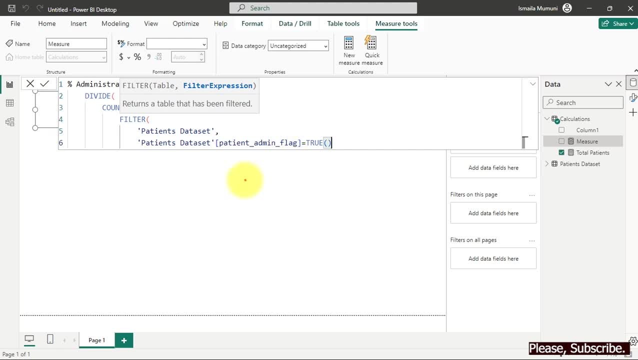 look at it. I did not place my true inside quotes like like this. that was because you know power bi is able to understand true and false without placing them inside court. otherwise, if we are trying to actually find maybe male gender, we have to please our male or female inside the. 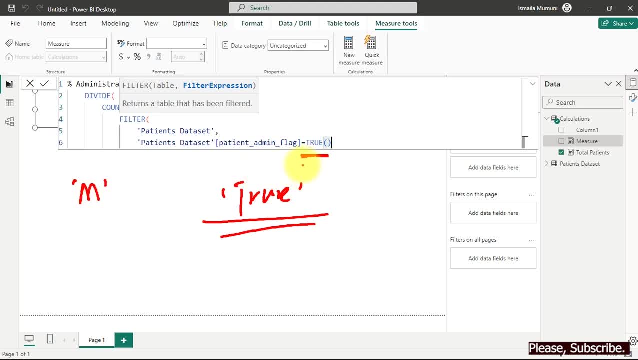 bracket. so here you don't need to do that, just type in your true Isaac. so once we have done this- now this is actually gonna be closed here- then we put a comma. sorry, we close this first of all. we close for our filter, now we close for our controls and we place a comma. so 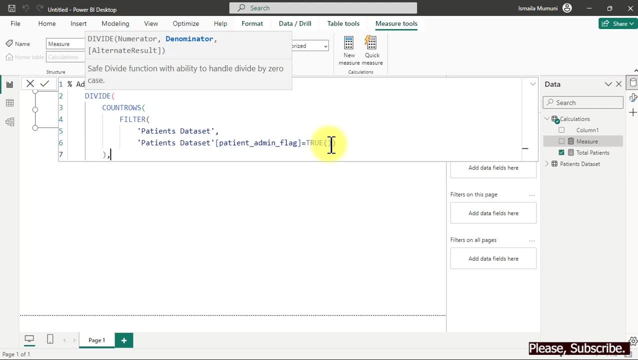 this denominator now would be the whole of our patients which we have before. that will go to be our, a measure we've created, which is the total patients right here. then we go ahead and close for our divide. so this will definitely create the administrative schedule. so I'm gonna go ahead and control C to copy. so I've copied this I have. 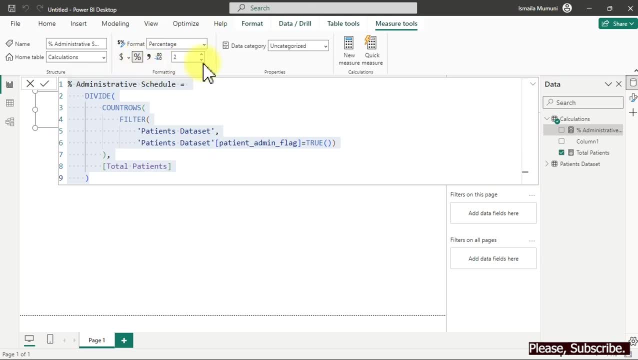 to format this one into a percentage. then, quickly, before we actually look at what we have done, let's go ahead and create a new measure. so inside this new measure, I will have this paste in, so instead of me having administrative schedule, I will have none admin certificate like this: 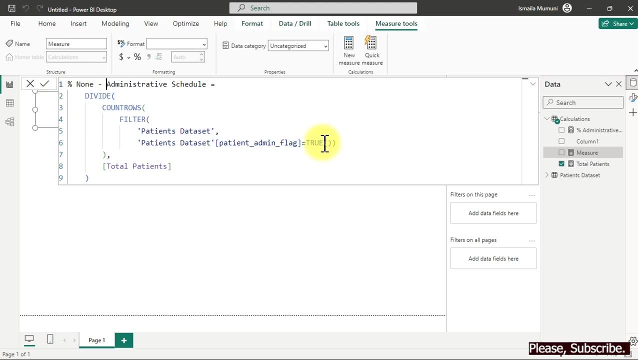 okay, then instead of we having true here, we'll be having false over here. so you get it. that is all you just need to change. then you hit your enter key and convert this into a percentage. all right, it is time for me to bring this into a card. so if I bring this in, it's going to show in a percentage. 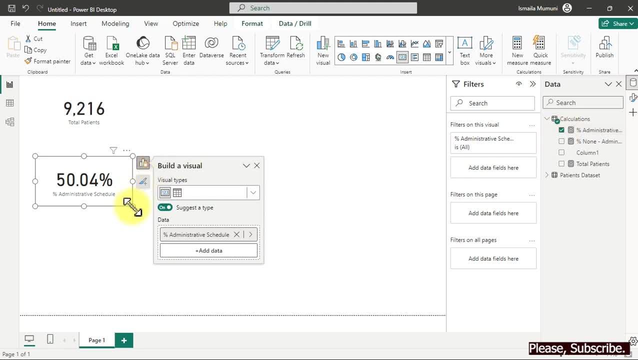 you look at that, so we have 50.04 percent of people under administrative schedule. then we bring the second one, which gives us 49.96 percent. can you see it now? so, before we start making this look much better, before we start making this look much better, 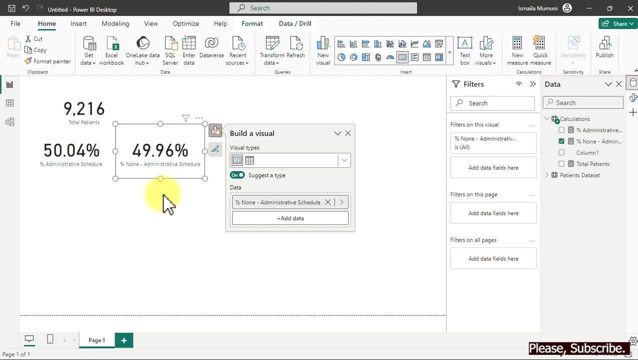 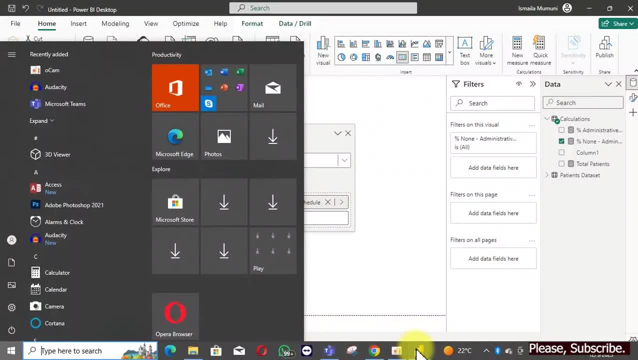 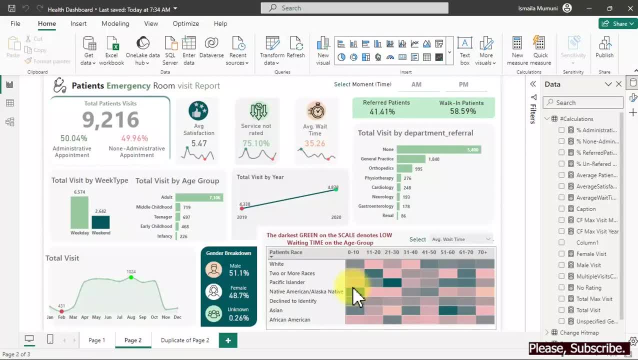 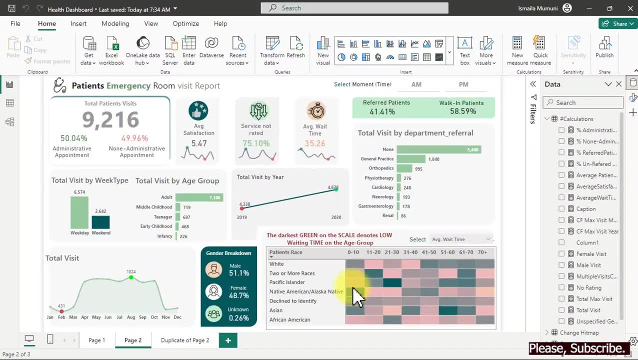 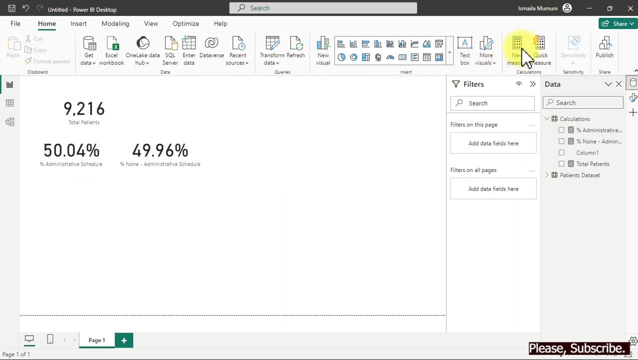 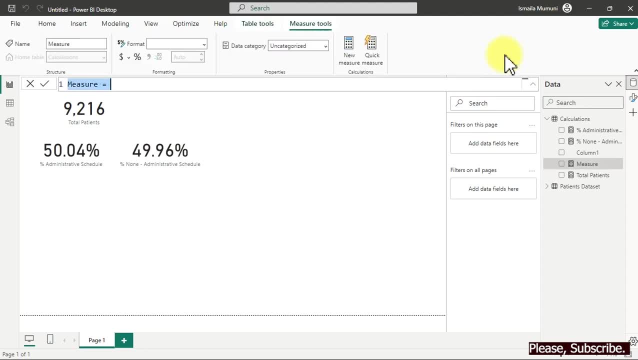 we want to actually look at our average. you know satisfaction very important, so understanding our average satisfaction is very important. so what do we do? we just use a DAX function that actually help us to wipe off all the blanks is very important. remember we have blanks. let me be done writing this particular 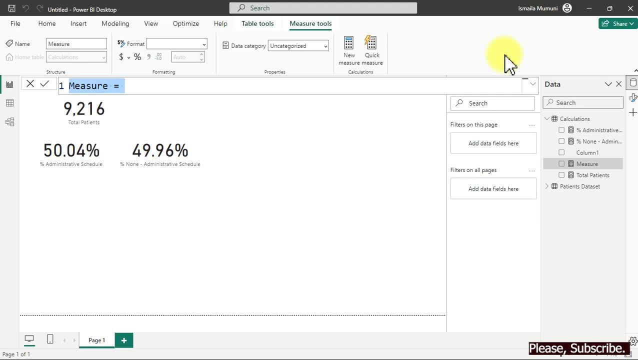 DAX code. I'm going to show you the column involved, how it looks like and why you should do what you're about to do. otherwise, you can just use average and average the column and you're good to go. so if I do average satisfaction score, so I'm going to do equals here- then I'm going to use 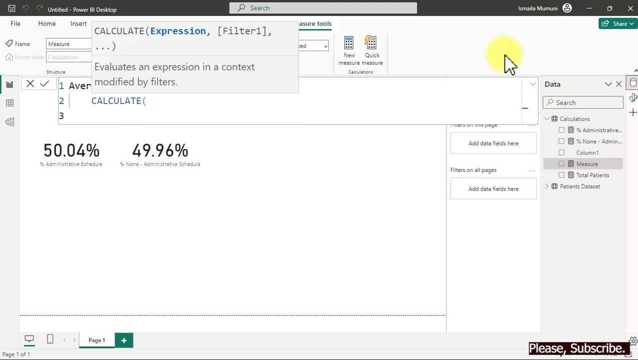 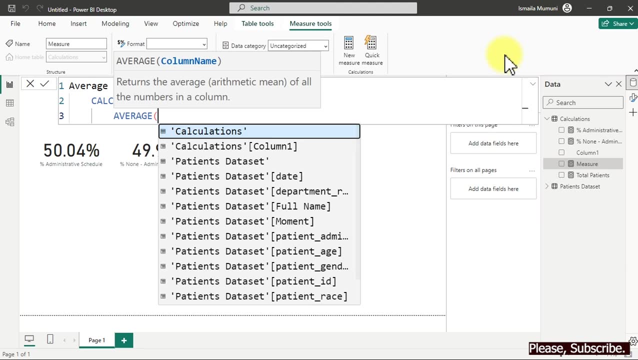 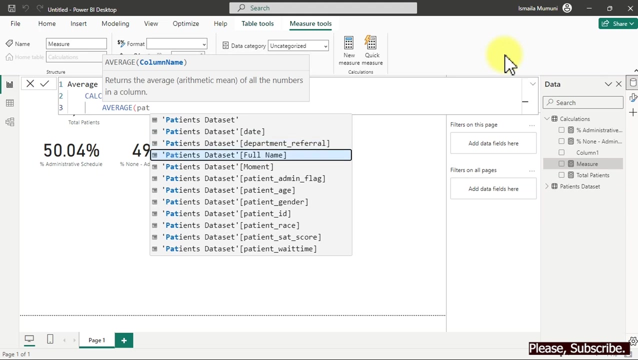 calculate function to actually have this done. then, for the calculate function, the expression- I will skip that first and I will use what I will use: average. so the average is looking for a column. what do we want to actually average? we want to average this particular patient, so it's going to be patient average. that. 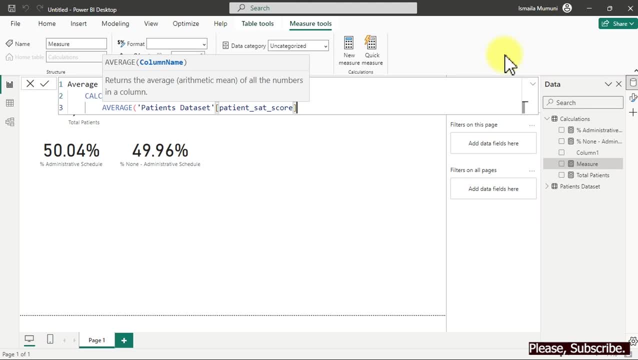 is resscored here. patients off satisfaction score here. so I'm going to close this and place a comma. so he's asking us for filter. that was where we have the calculate here. otherwise this particular part has actually done the job for us. this line here has done a job for us, but because we want to filter, this line. we want to recommend that we now DustB 매数 as a closed line, but from this lean line has done a job for us, but because we want to filter this line, we want to filled her. this line is actually for respect to my data is just a linear. 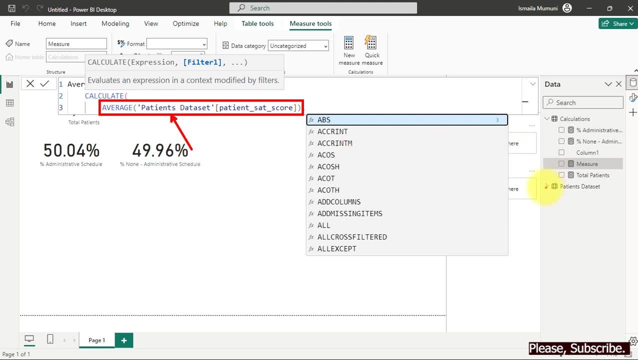 so let me do a bad email. no, I'm just going to find that shake video. let me particular patient data set table. i mean this whole table right here. so for that we need to actually use the calculate function if you know the functionality of the calculate function inside. 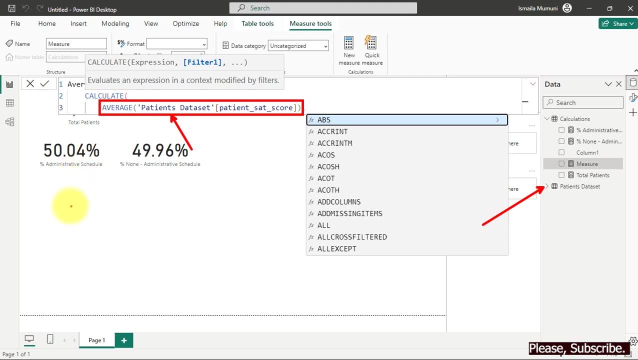 the dax measure, you wouldn't argue this because it actually helps you to change the filter context. so what filter context are we trying to change now? we're trying to remove where we have blanks. we don't what. we don't want to some kind of average it. so we want to remove where we have. 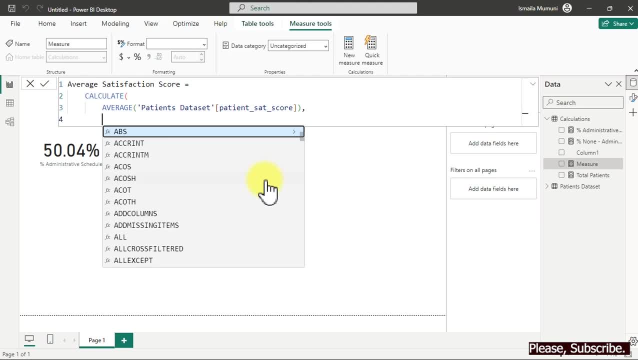 blanks. so the next thing i do is actually say: okay for my patient. you know, satisfaction score here we want only where we have values, so i'm going to use this as not, which means where it is not blank is where we want to average, i'll do this. so i am going to do this and do the other one, so, which means i can just copy this: 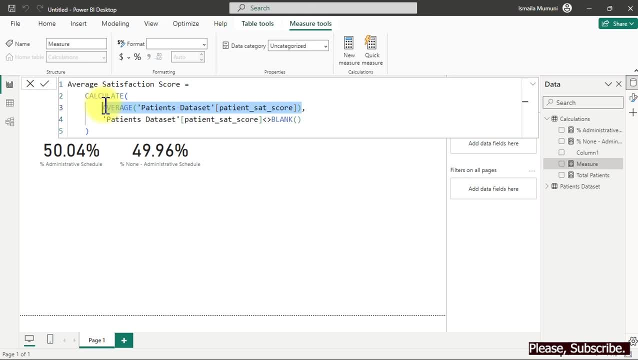 particular one here and ctrl c just to show you the difference between this one and the other one we're going to create. so once we are done, we can hit our enter key. we have just created our average. what average satisfaction score of our patient, how satisfied they are with our services. 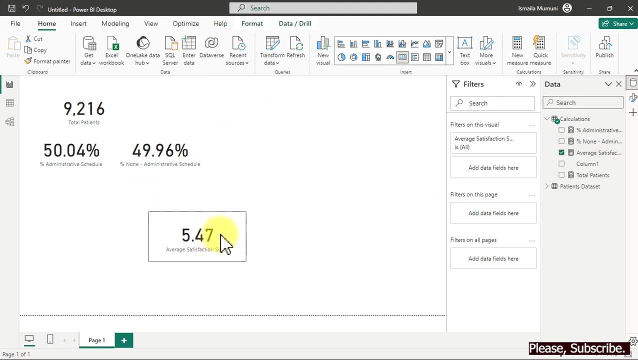 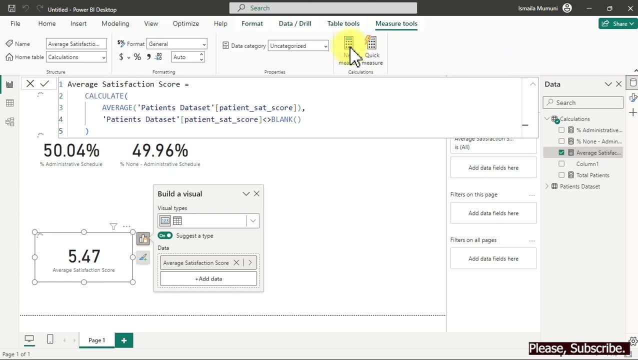 all right, i'm going to bring this in to a card. this is what we have. please look at this and let's go ahead and actually create a new measure. i don't give this measure a name, but it's going to do this, something similar. here we go, so i'll hit my enter key. 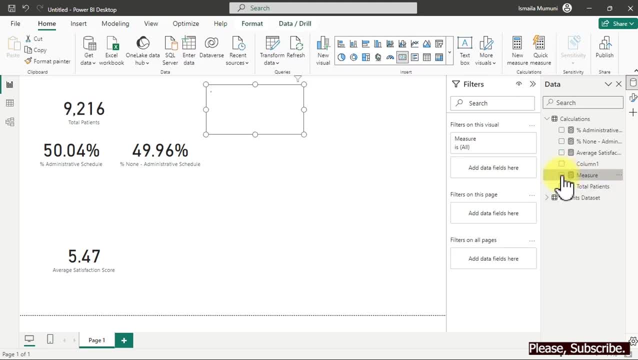 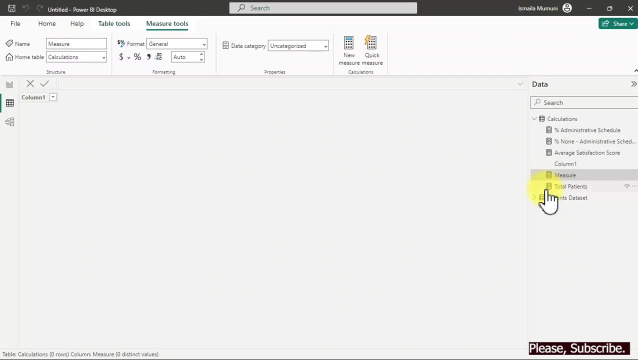 then i can push this into my card again. so can you see the difference now? now, let's go to the table view and take a look at the table. now let's go to the table view and take a look at the table view. let's go to the table view and take a look at the table view and take a look at the table view. 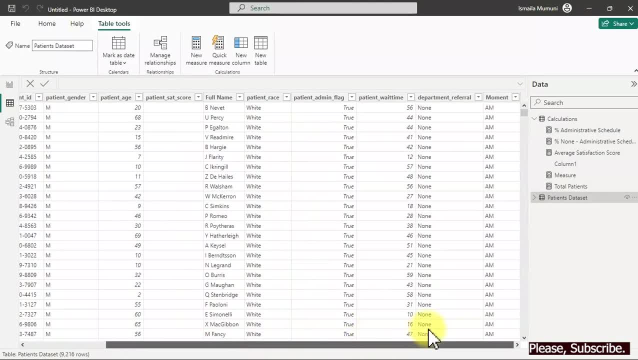 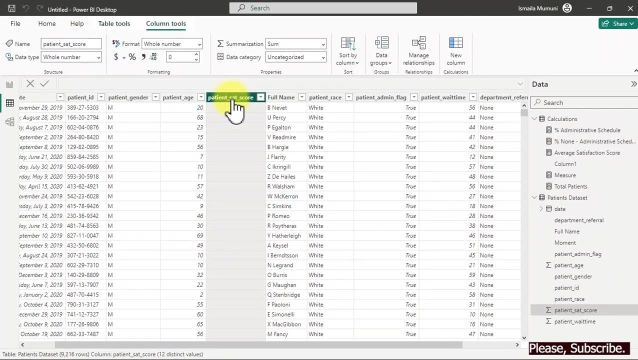 involved. Inside this particular table we have a column which is the average patient satisfaction score. If you look at it with what you are seeing now, the column seems to be some kind of blank. but it's not totally blank, We have some. 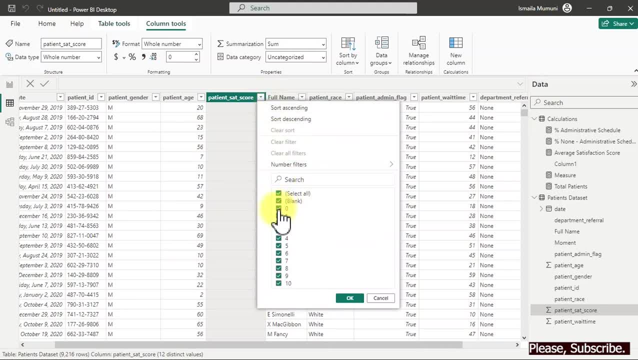 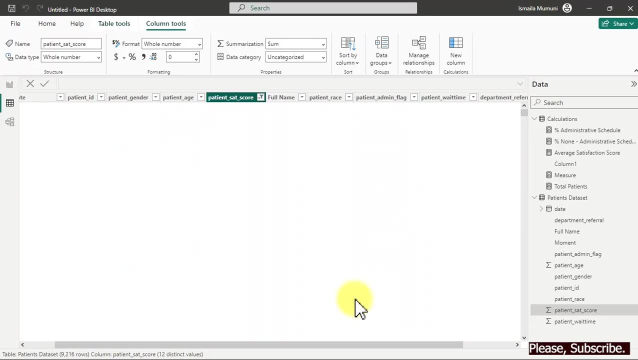 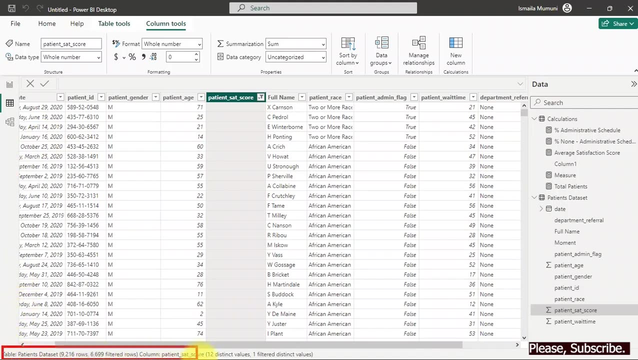 values here. So this call starts from 0 to 10 and we have blanks. If you want to see the blanks now, I can actually go ahead and do this, and here we go, we have blanks. So look at what we have as some kind of guide to our blanks over here. So 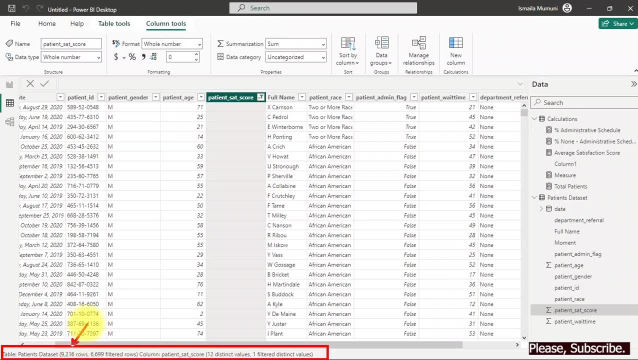 we have over 9,000 rows and here we have 6,699 filtered rows, Which is the blank that we have. Can you see? That is exactly what it is, So we don't want to account for the blank when we do our average, So for that we 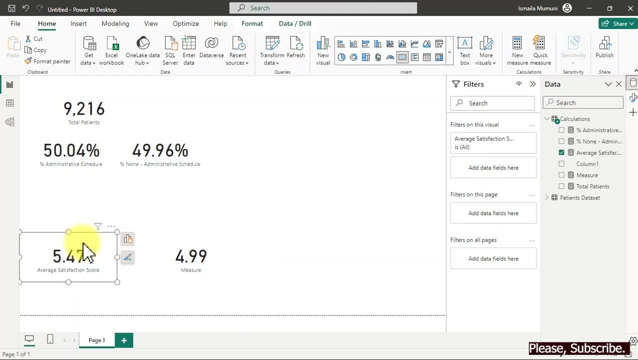 have to filter it. So we filtered it in here and it's giving us 5.47.. So the one that does not use filter of blanks away is now giving us 4.99 as an average of satisfaction, which is not correct. So can you see that now? 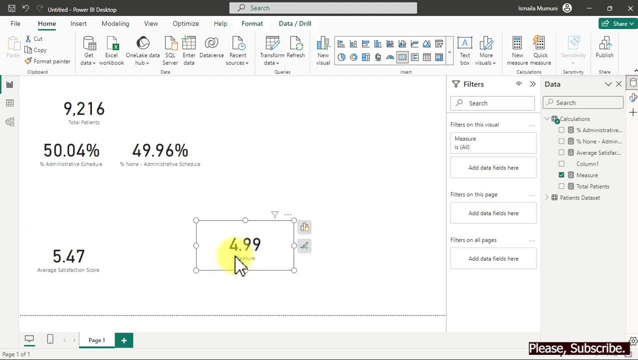 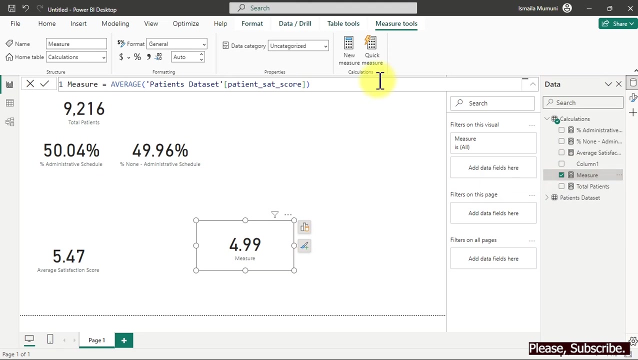 Okay, We want to now get how many persons did not actually rate our services or when they visit the emergency room. So we want to actually account for them and what we want to do now is actually showing the percentage of people who did not actually rate before the leave. So I'm going to come back to the here Now. we 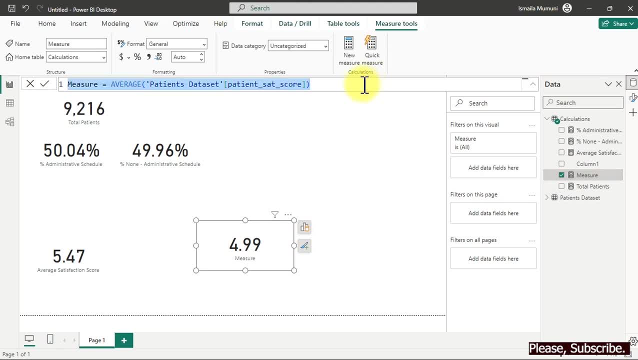 don't need to keep this, I can just get it off. So I'm gonna say percentage plus 100% and then, by the bottom line, 50% and executedorean F: quantity before they leave윈. So I'm gonna come back to here. now, we don't need to keep this, we can just get it off. So I'm gonna say percentage before the leave. So I'm gonna 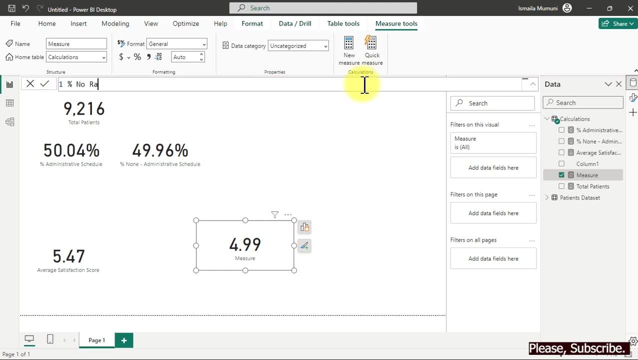 of what? of no rating. so for the percentage of no rating, what I'm gonna do now is type in a variable here inside a variable. I'm gonna name the variable no ratings. okay, so for this: no ratings. what I'm gonna have is using the calculate function here to find out who are those people. that does not, or that. 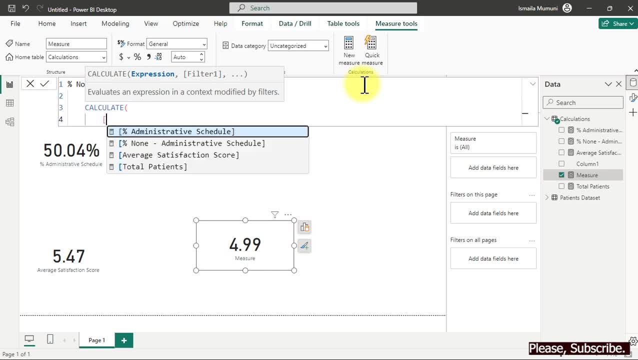 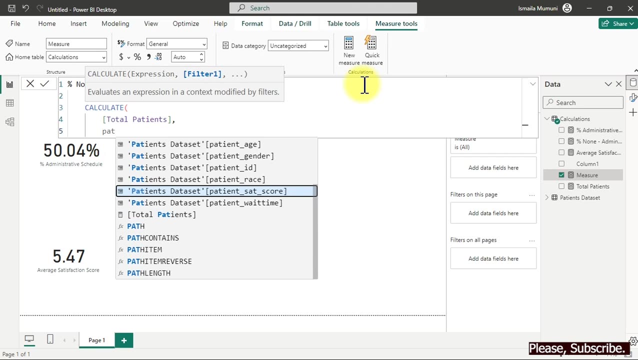 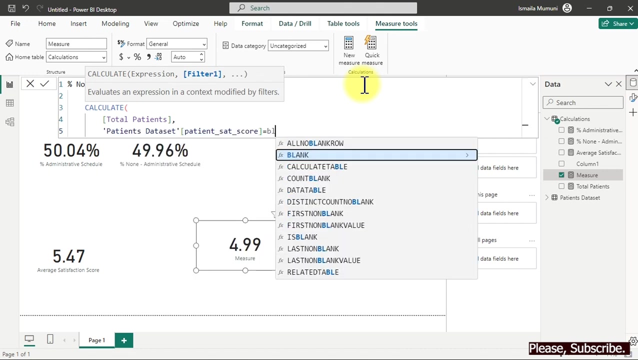 do not rate our services. so I'm gonna calculate what calculate the total patients. then, when I calculate the total patients, I will change the filter context by filtering for my patients where we have the average- sorry, the patient or satisfaction score to be equal to blank. so we can now come back and close for our calculate that is. 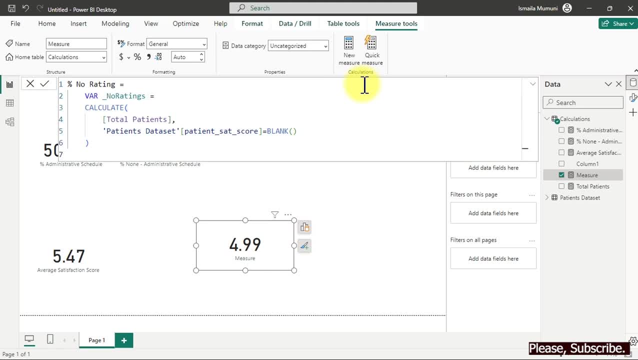 that, so we can now do return. so for the return, we can do divide, so we divide what we divide, our variable, which is number of no ratings, number of ratings, so yeah, number of no rating. we do that by what? by total patients, or we can call it total visit, visits or visiting wherever it is. so 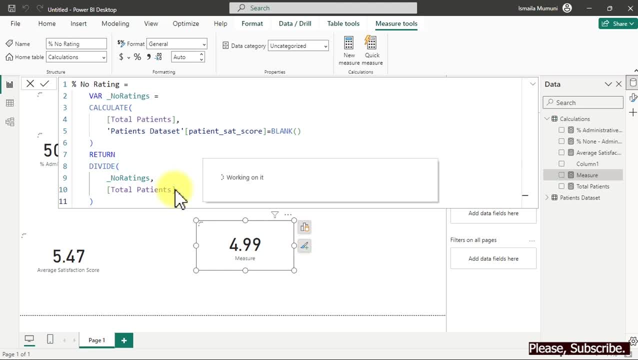 here we go. this gives us like 70. what, based on what we saw on parkery, I think it's 75%. just go ahead and format this into a percentage. can you see that? now? this is the numbers of people that did not actually rate us. 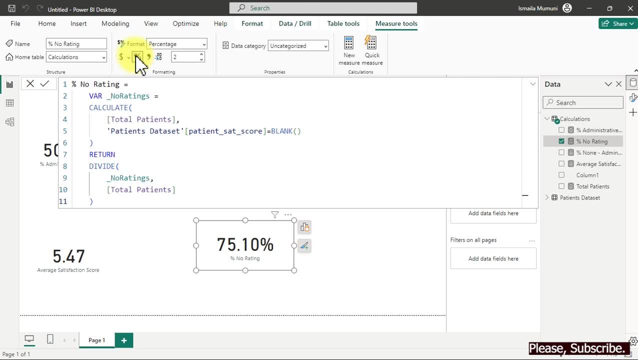 so we don't know why, but we're gonna find out why in no time and see which. where are they, where are they from? so there are so many things we can actually put into consideration while doing this. so do you see this now? so the next thing. 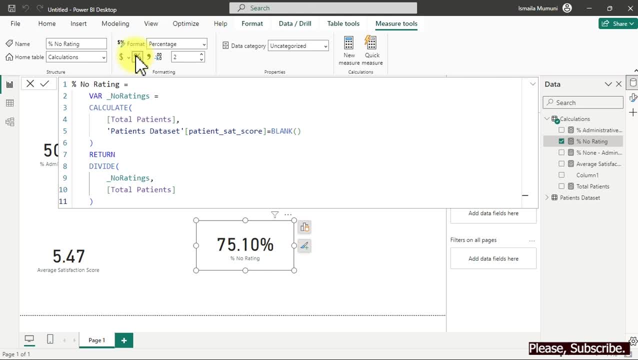 we have to go with now is to actually check the average wait time of those people that actually visited us. do they stay longer before they were attended to, or not too long? so I'll come over here and create a new measure. so in this particular column there is no blank, so all we have to do is to 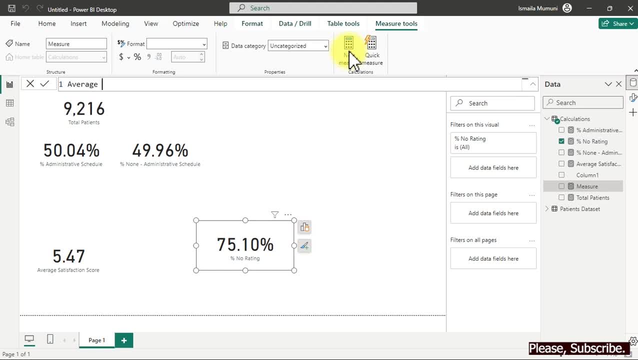 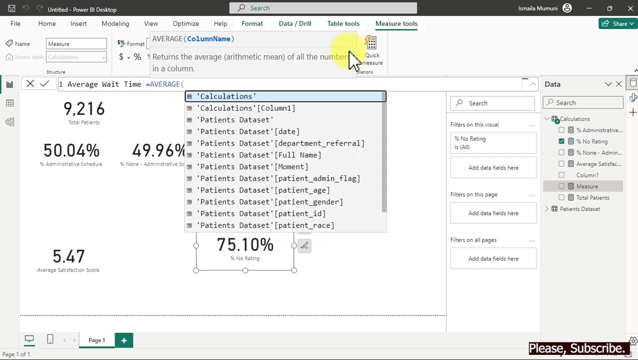 actually type in here average with time. so what we need to do is just to use the average function here and we average patient. you know that is gonna be. oh no, this is it here. we just flopped it. let me see. do we have that column? average wait time? oh sorry. yeah, we have it here, so we have a column that can. 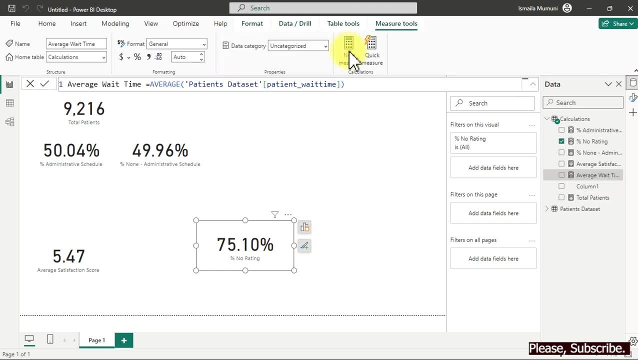 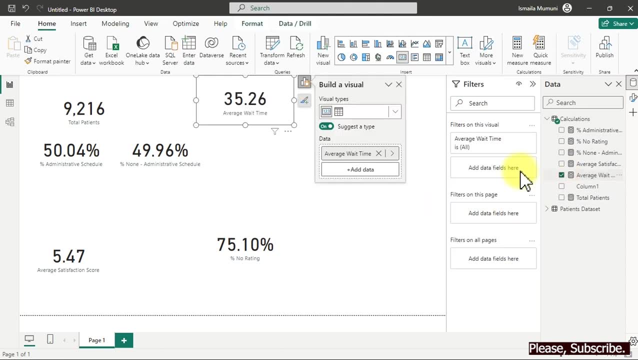 represent that that is the wait time here in minutes of our patients. so if we bring it into a card now to look at what it is that we have, we're gonna have something like this: ice: 35 points, 23 average minutes. they waited in the emergency room before the話. 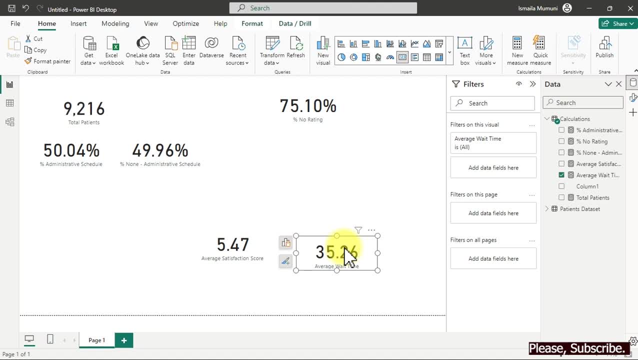 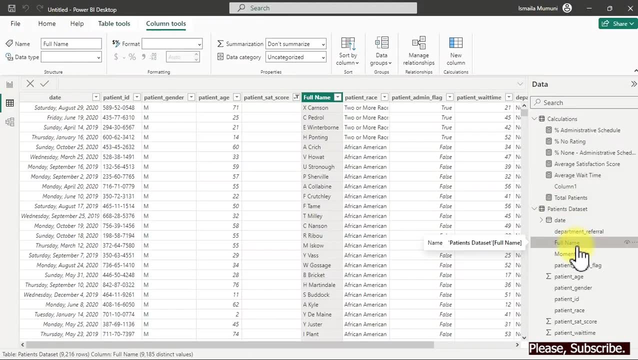 the satisfaction of our rating, which is average satisfaction score here and as way time here. what are we trying to investigate? we have a column. this column is called patients race. so the patient's race now is: if the patient is black, the patient is actually um talking about. 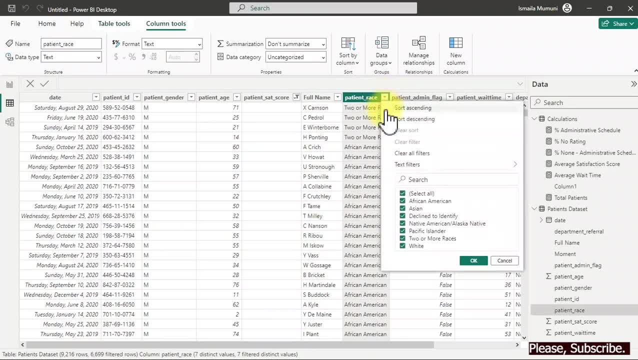 this one here. so if i open it up right now, you see this. so the patient is actually african-american. asia, you know, declined identity, which is those patients that did not feel that particular part to identify where they are from, and all that. so we want to know. where do we have high rate of? 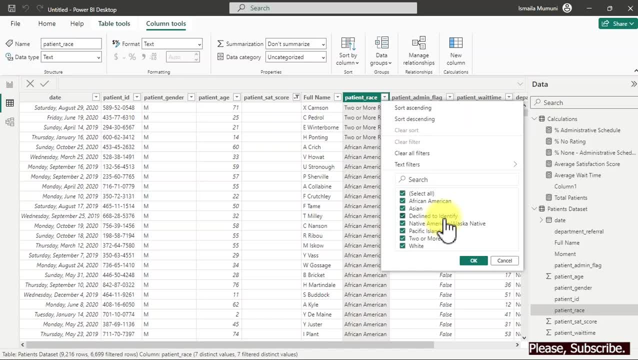 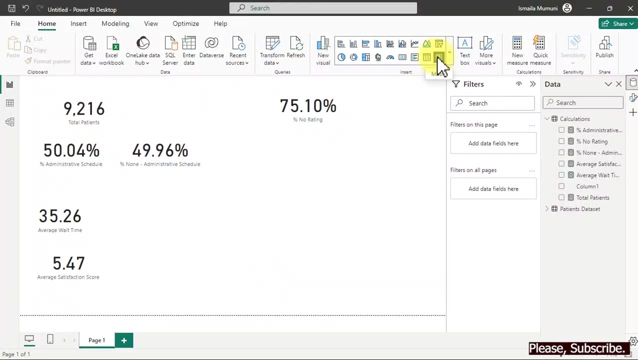 satisfaction and low rate of satisfaction. and as well, where do we have, you know, high weight of high rate of weight, of average weight, time or whatever. so we go back here. so now we are here, i can actually create a heat map for that. so if i click on this, this helps me to create a heat map. 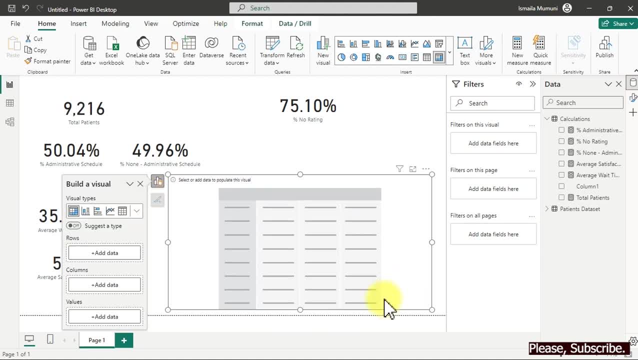 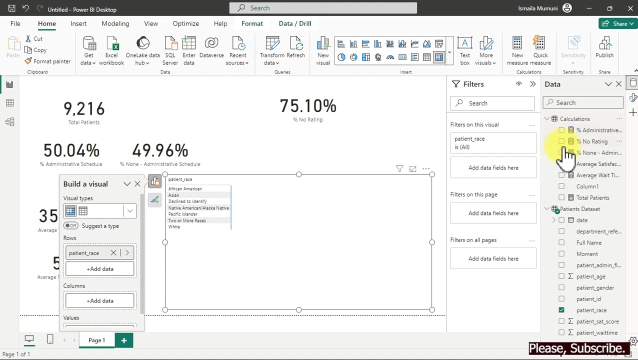 so which you can drag over here, make it as big as you want for you to actually look at it in detail. so in this heat map, the very first thing i'm going to do is to actually bring in what bring in my patient's race. so i have my patient race here. so what we want to look at first is actually the average wait time. 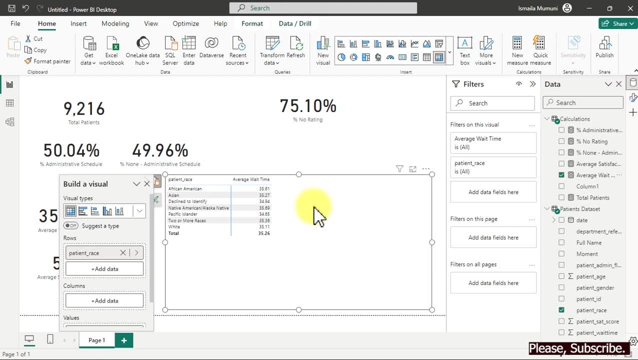 so for the average wait time here is not making a lot of sense for now. we need to actually add a column. so what will this column do? this column would look into which particular age group has the highest average with time or the lower, the low average wait time. so we need to actually add that. we don't have that here right now. 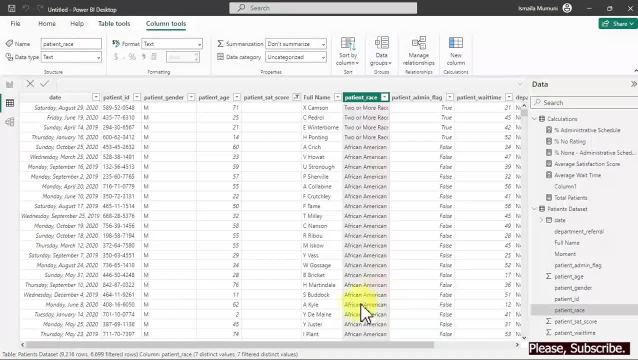 okay, let's get back to the back end here of our data. so we have this particular column called patient edge. we have our patient edge here. we can't use it. it's going to look some kind of awkward when you try to use it. so what we need to do right now is to group this edge. 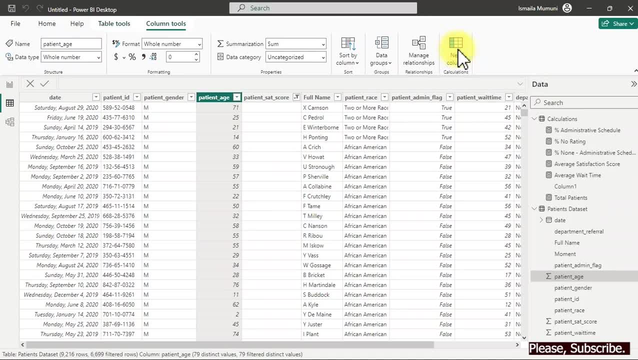 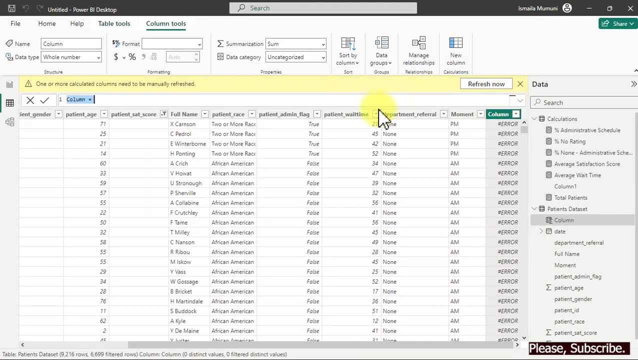 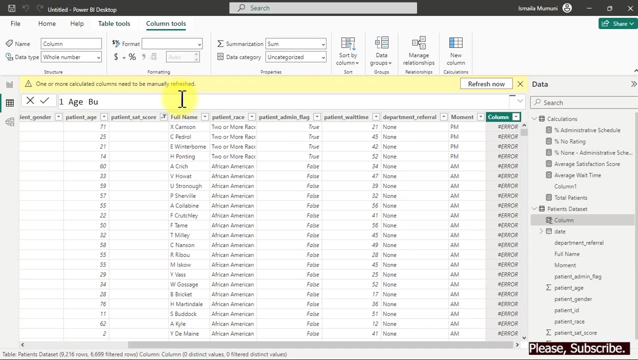 so to get that done, click on new column. so this will definitely add a new column for you. the column is giving us an error, don't worry about that. all right, on the new column. here i'm going to actually call this age bucket. so for the eight buckets i'm just going to straight up: use what. use the switch function. 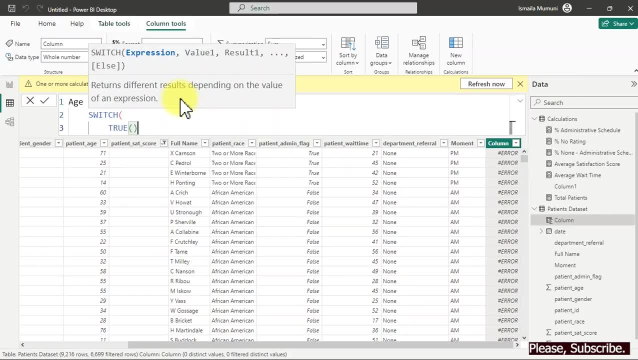 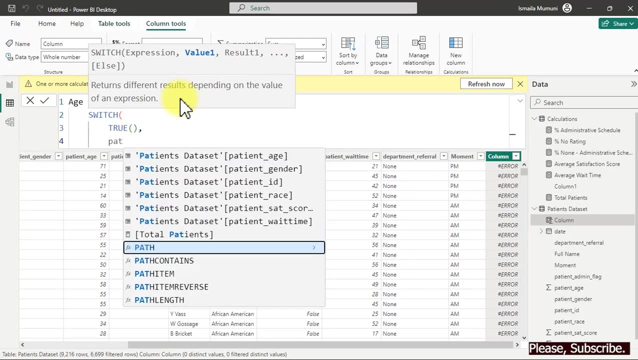 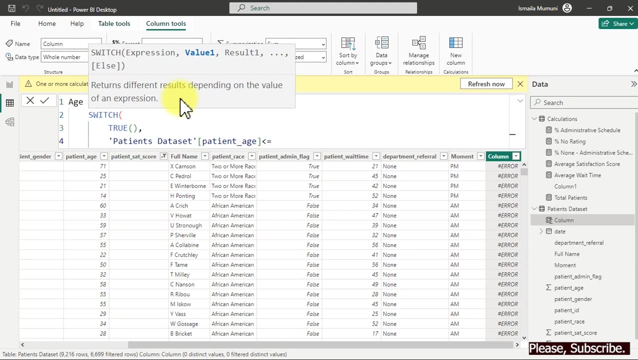 so it's going to be switched through, so comma. so what we're going to do right now, we're going to say the patient um age here if it is less than or equal, to try to find what the error is: 10. so what do we do? we want to categorize them into 0 to 10. you get it, that is 0 to 10. so please. 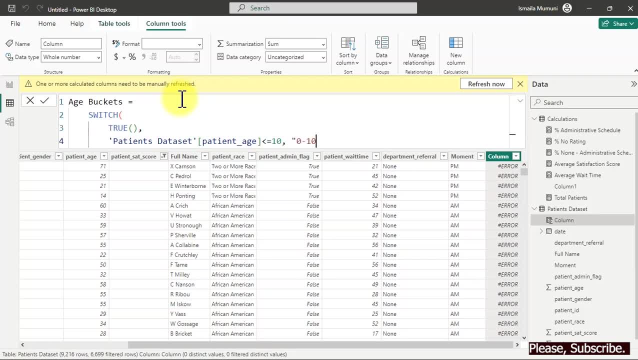 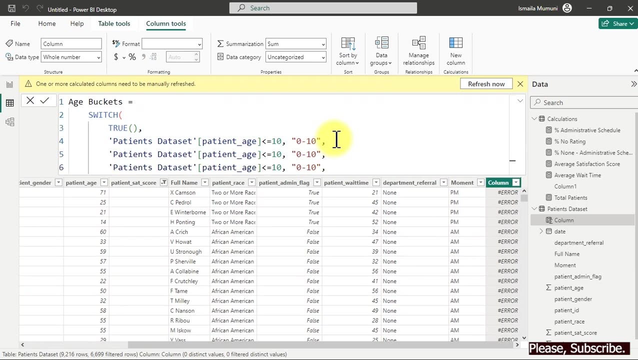 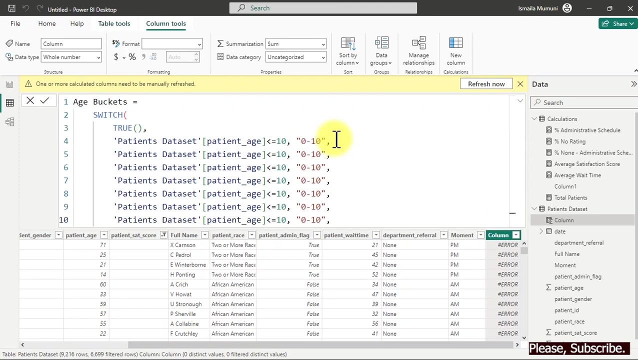 place it inside quotes 0 to 10. then, to avoid writing this over and over again, i can place my comma here and just go ahead and copy this. so just recycle through this, okay now. what we need to change now is this particular part. here we make it 20. 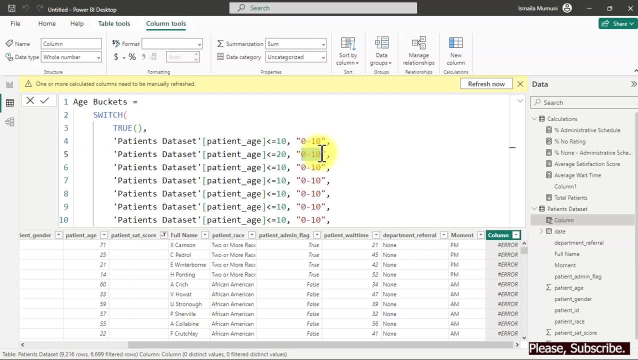 so we can make this one 11 to 20. so, right, here, we're going to make it 30, which means we have 10 interval, right? so we're going to make it 30, and then we're going to make it 20, and then we're going to make it 20. 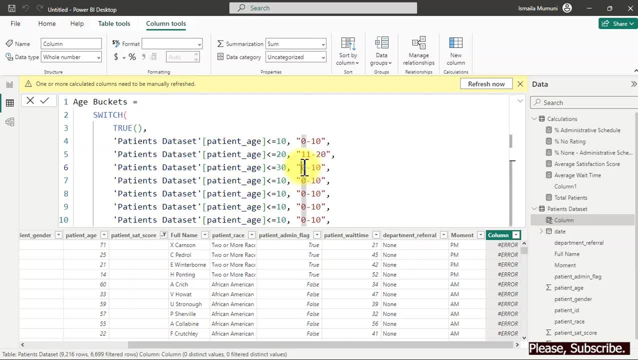 so we're going to make this one 21 to 30. all right, this is what we do. we have just done this- and anything that is not between this particular from 10 to 70 here. so we're going to categorize- you know anybody on the data- to 70 plus. 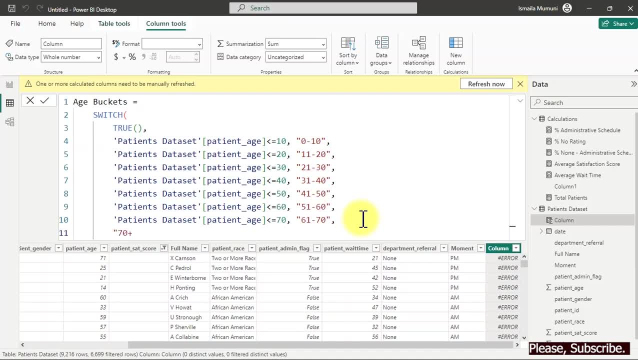 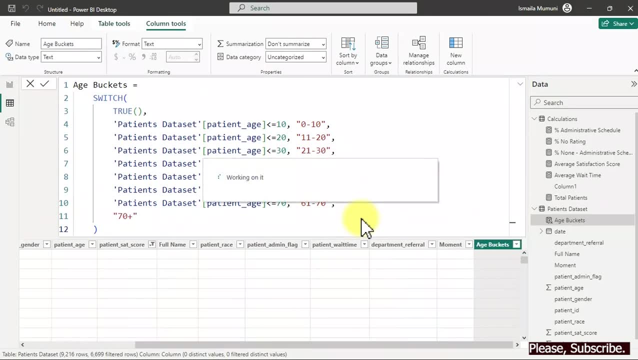 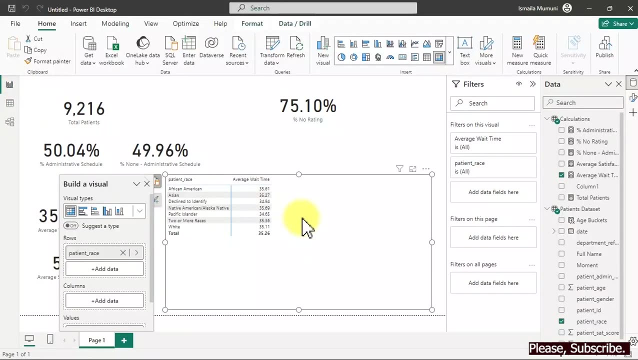 so we go ahead and close our switch. so we're going to make this one 21 to 30. so we have actually, you know, grouped the age. now, here we go, so we can now use this inside our dashboard. so what do we do? we have to push this particular eight buckets in the column area here. 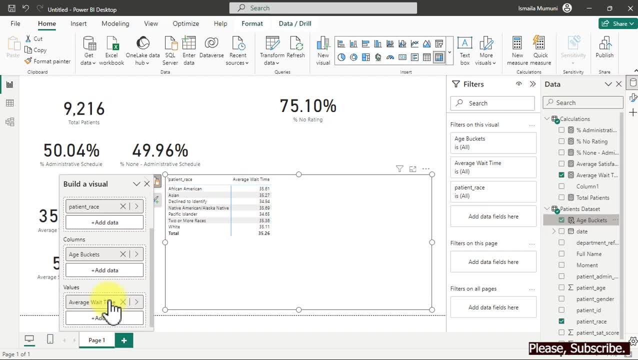 so go ahead and move it here. so can you see it now? so there you go, you have this all right. the very first thing we're going to do after this is we're going to do is we're going to make this one 21 to 30. 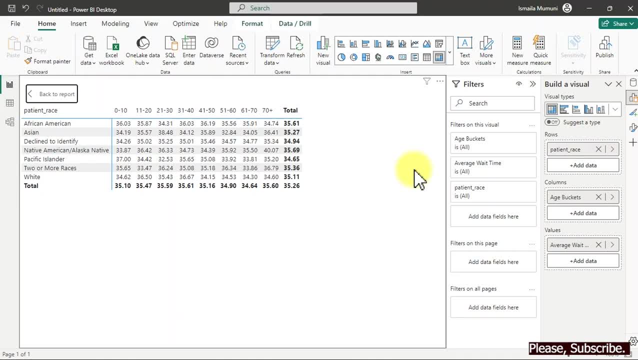 all right, the very first thing we're going to do is we're going to make this one 21 to 30. so after i've gotten this done is to some kind of make sure we use the color to tell the story. but one thing is this: i want to be able to switch between my average satisfaction and average wait. 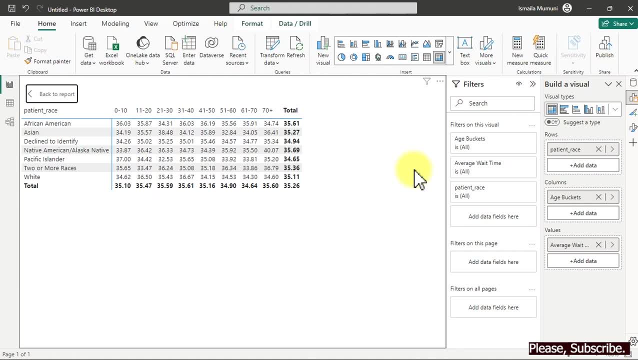 time. in that case, what do we do? which means we can't use this measure. we need to create and damage it, but we don't have to write a single measure. but we don't have to write a single measure, but we don't have to write a single. 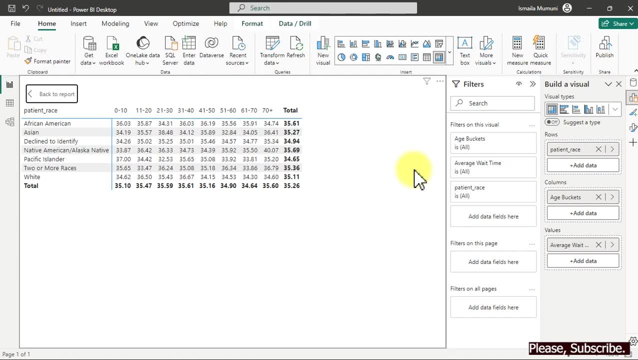 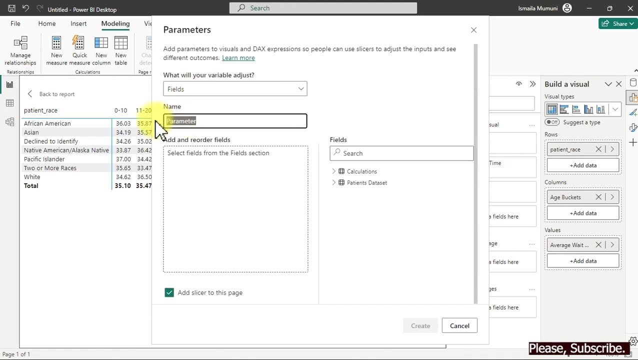 DAX code to do that. so we can actually allow the system to help us do that. go to this modeling here and click on this new parameter. from there, click on fields. so you're going to have this. so you can name this one to anything you want. so I might leave it to parameter. 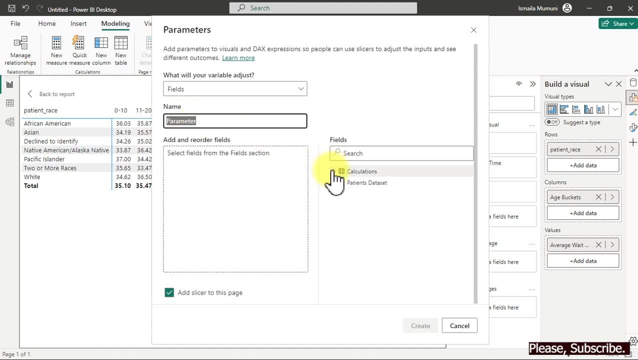 because I'm not going to create many of it so you can rename it. I've just said that. so when we go here now we have the average satisfaction here. it's now in this box where we have add reorder fields. then we want to keep in. 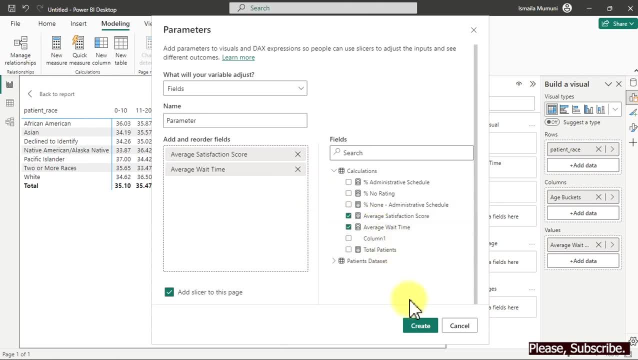 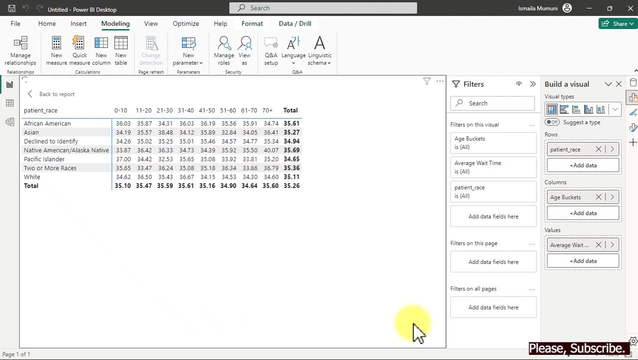 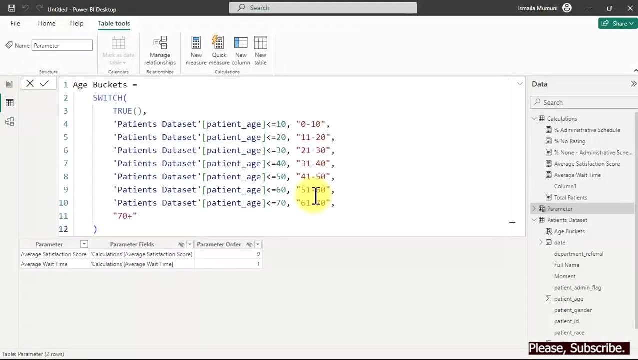 our average wait time. so with this now we can add a slicer, so it has been added for us before we can see it. let us leave this particular view automatically. it brings us here, so we go back to this particular part here now and let's go ahead and take a look at 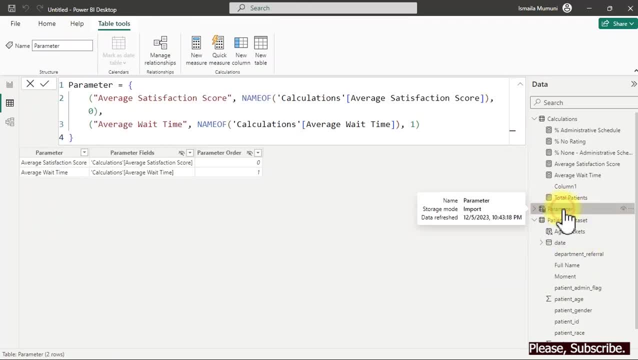 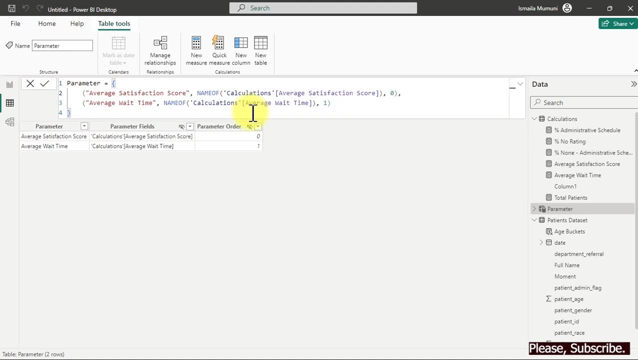 what we have done. so here is it. so this is what the system generated for us automatically: a measure with a table at the same time. so I want to- actually I want to change this. I want to remove this particular part. so, for the average, I would love to use this avg for average. 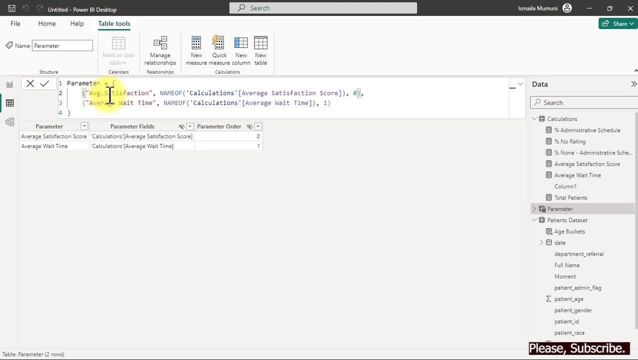 you get it there, I will come over here. I will use the same thing to make it short. so here we go. we are done. we can hit our Enter key. so in this table we have parameter, which is the name of our measures. so we have parameter fields, which is what the 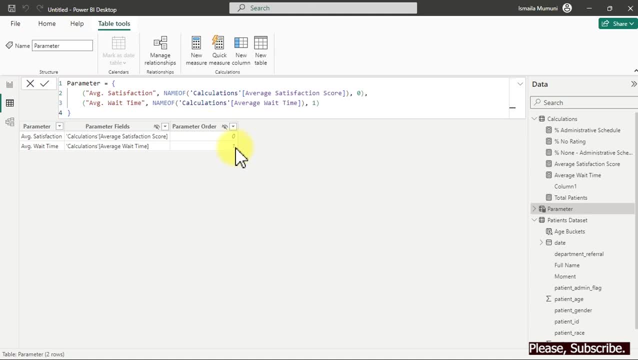 measure we brought in and we have order, so we're gonna use this particular 0 and 4 in subsequent time to come, but for now, let's just go back and take a look at what we can do with this. all right. now that we are here, we are going to update. 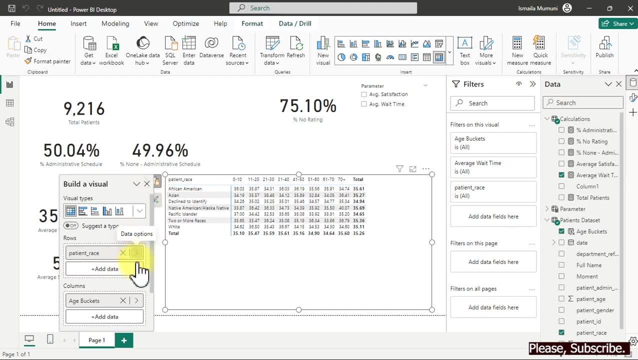 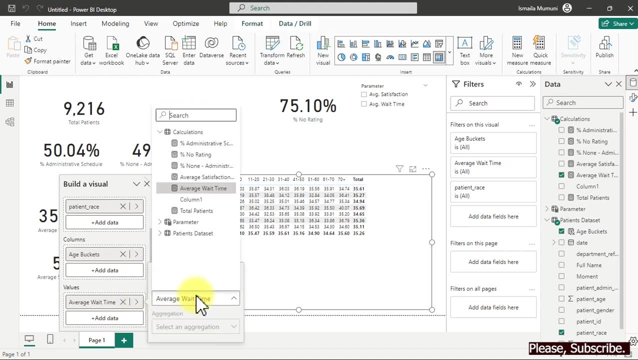 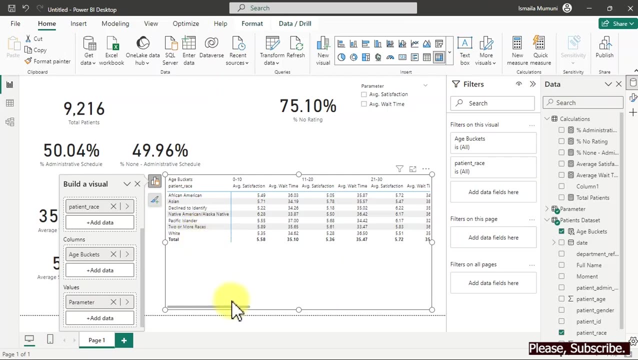 this. just click over here and update your patient's average wait time here. so update it to what? go to the parameter and bring in this particular parameter here. so now it's looking ugly. can you see a lot of it? so why do we have this? that was because we have. 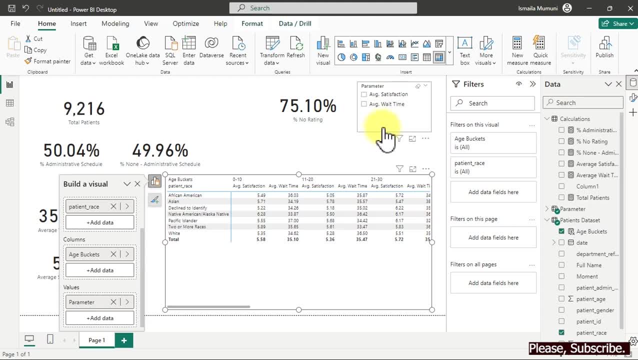 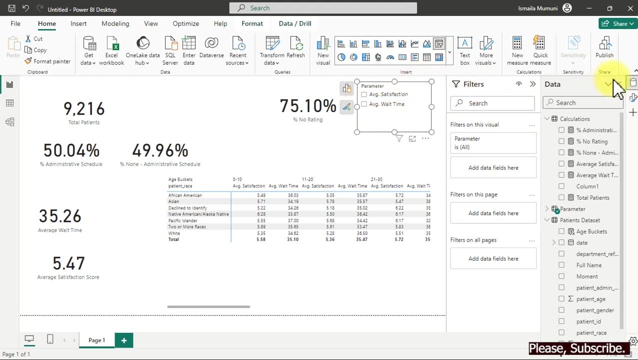 not made any selection, so we have to select one of it. so for you to avoid this particular kind of view, what you have to do is to click on your- you know- slicer and go over to here under format. then you go over to slicer settings and 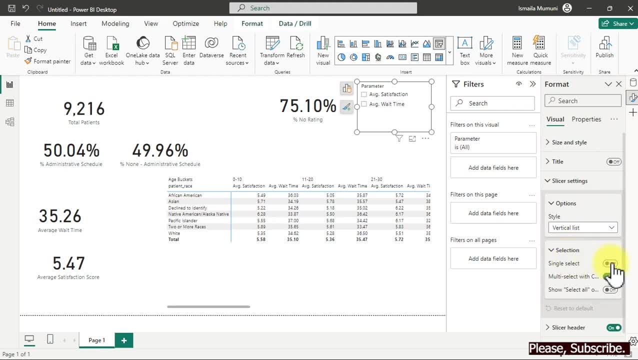 you go to selection, then you actually make sure you check this particular single selection automatically. it select one for you, select one for you. so we have the different colors that we can choose between the color codes we can use for our report. so let's go ahead and select. 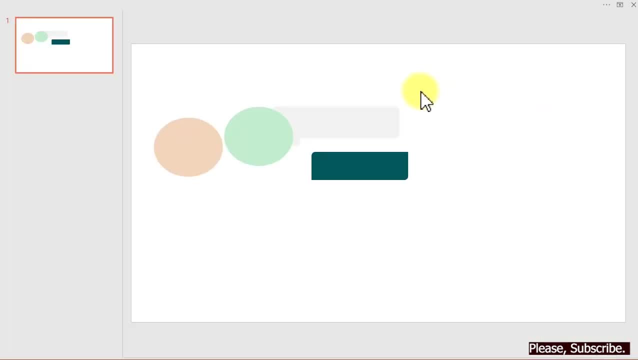 that, so we can switch between that and this. do you get it now? so right here we have the color we are going to be using. so here is colours we're going to be using for our project. so all I'm gonna do is actually copy the color code from: 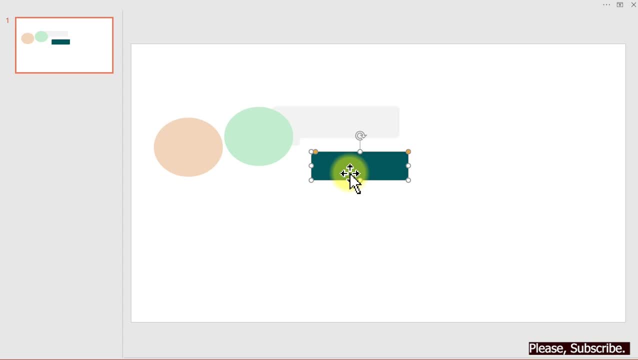 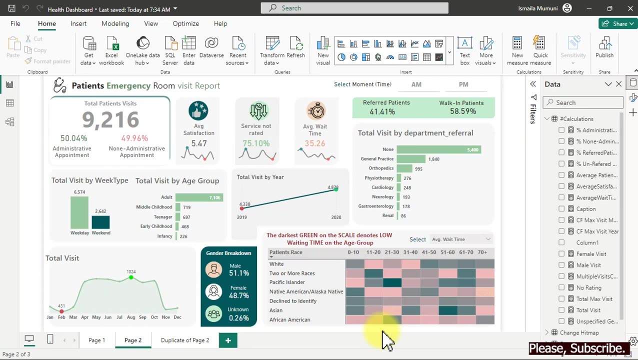 here. you need to see that. so you're gonna actually receive this. you can decide to choose a different color. to create your own report is your own choice, but create our chart. so, on this particular chart you have here, we call it heat map. so when we select, 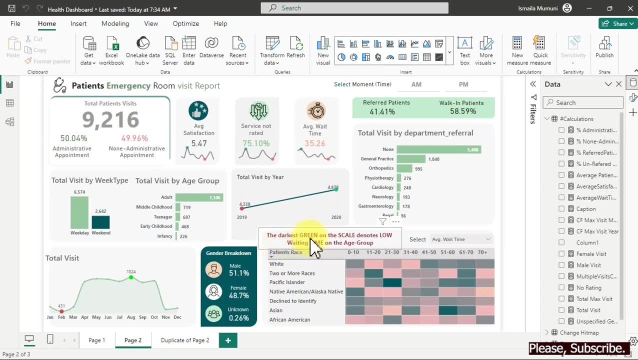 average weight time. you can look at this. it says the darkest green on the scale donates low weight time. on the age group and as well the what the race you understand. then, when we select this particular average satisfaction here, it changes to what patients are most satisfied. 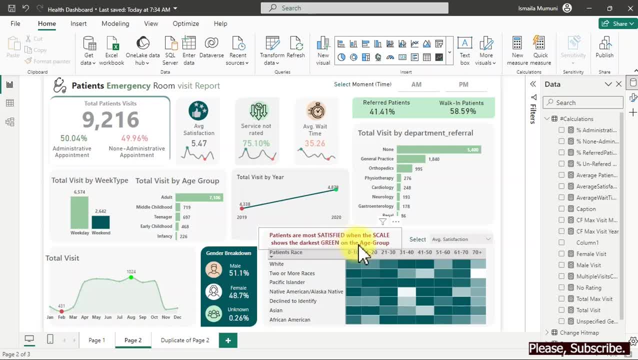 when the scale shows the darkest green on the age group, you get it. so now, which means when we come to white, the white race. so we have from 31 to 40 and 41 to 50, then 61 to 70 to be highly satisfied, followed by this. now let's go to african-american. i think they are actually. 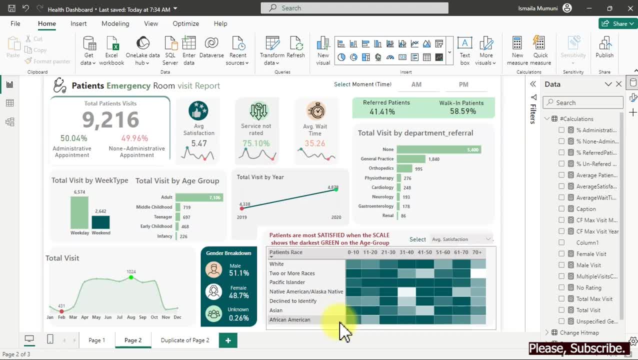 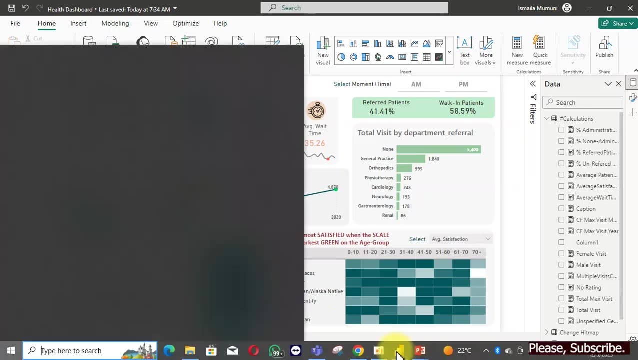 more satisfied with what i'm saying now. so, which means the average Satisfaction has nothing to do with rays and all of that. So that is what this is telling us. We want to actually replicate exactly what we have here right now. How do we do that? Okay, first off, we go all back to here. 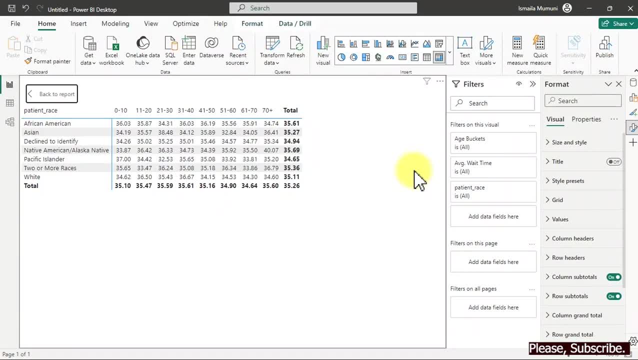 So we are right here. let me give you this view. So, with this view, now the very first thing I'm going to do is that I want to remove my row and column total. So we have them here and here. We don't need to keep them. 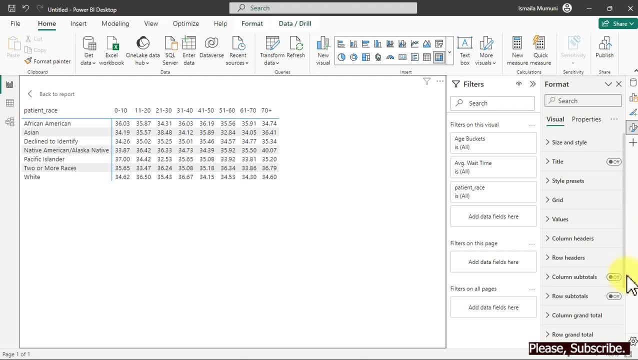 So we are now left with this. So if I scroll a bit down, So I will see where it says cell element. I'm talking about this one here. Click on it. So now that we are here, we have two different measures. We are actually on one. We only see this when we switch using the parameter we created over here. 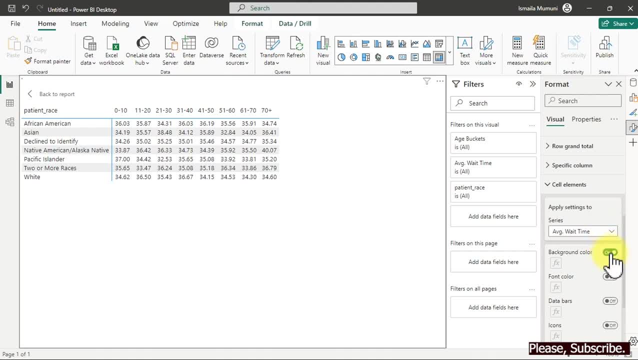 So now that we are here, we have two different measures. So now that we are here, we have two different measures. So I'm going to turn on the background color. I have something like this, So I'll go to fx here, Then come right here. So what are we doing now? 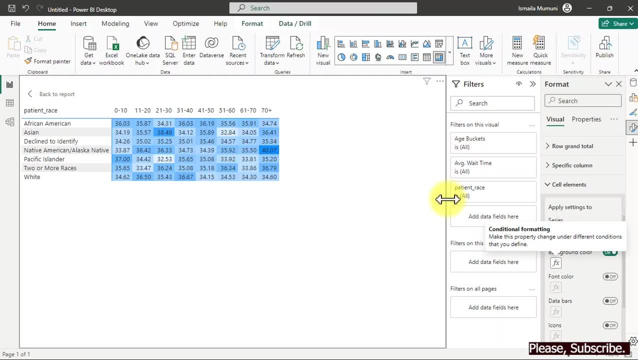 We are doing the average wait time. So, for the average wait time, what do we actually want to show? How do we want to format it? So what we want to do now on the average wait time Is that for the average wait time, we want the darkest scale. 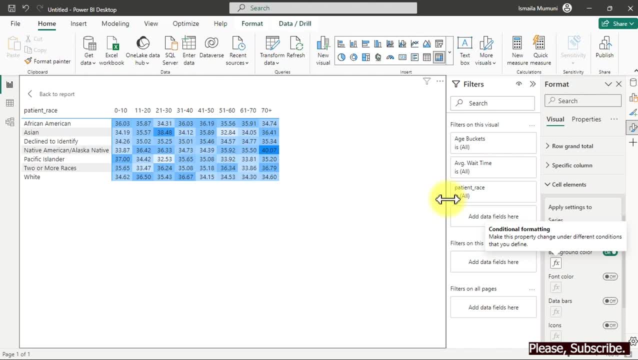 Or the darkest green on the scale to donate low wait time. I want to show in that color that actually signifies Any way you see that color to be. Those colors represent where we have high amount of wait time. You get it now, So click on this particular fx here. 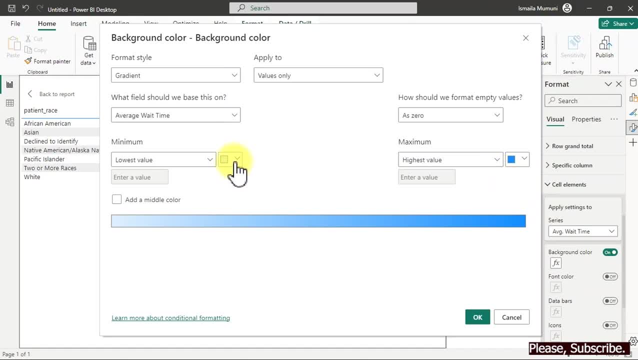 And it brings you here. So for the low, we're going to click over here And click on the more color here. So we have our color code to be this, Which is going to be: 01575c Is the kind of color we want to use. 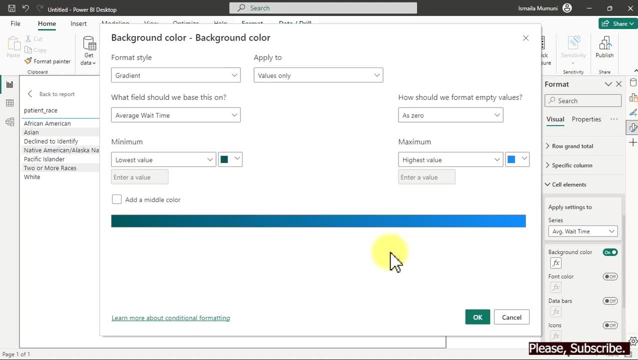 Just like what you've seen previously. So we go with this. So we want to add a midpoint, Which is this one, This one here in midcolor, For the midcolor. now We're going to select this one For where we have high wait time. We click here. 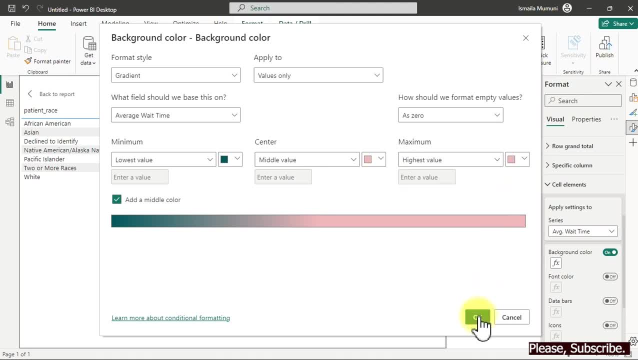 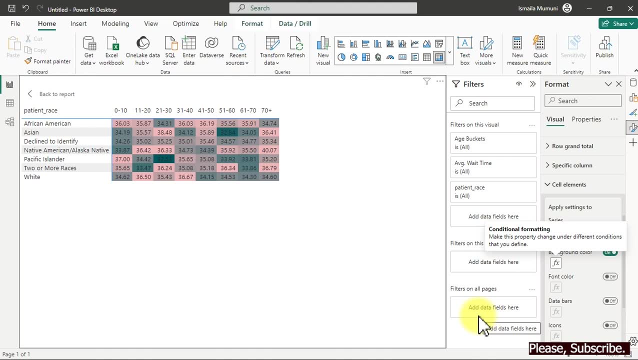 We select this one Where we have high wait time. Then I go ahead and click on what? Click on OK. Do you see it now? So anywhere you see green, Which means we have low wait time. Let's compare it As in the lowest wait time we have is actually 32.53 average wait time. 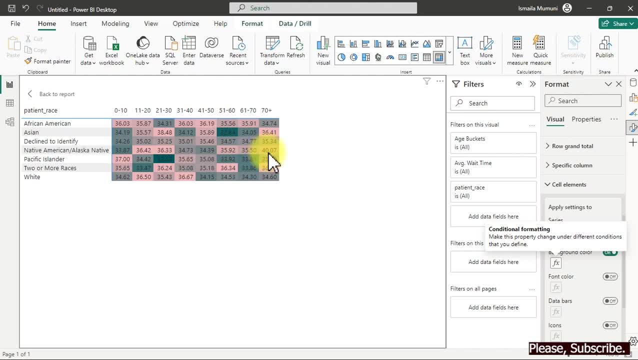 So the highest wait time we have is actually 40.07, Which is this one here, Under 70 and above. This is what we want to create. So once we have done this, We are not trying to show the figures, We are not interested in the figures- 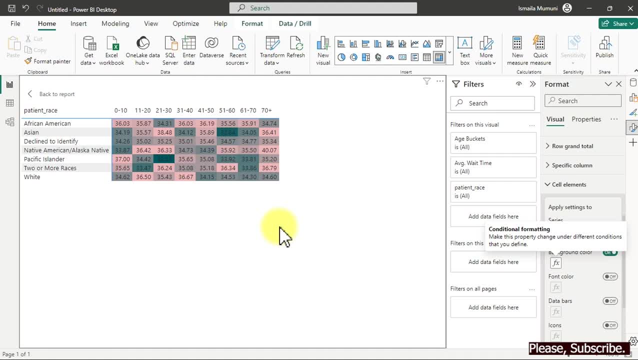 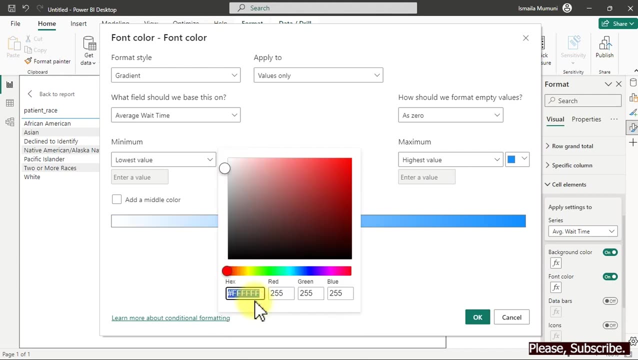 We are interested in the patterns, Mostly the scale of the color. What do we do? We click on what? Click on font. When we click on font, we go right here. We choose the same color, Starting from here. Go to more. That will give you 01575C. 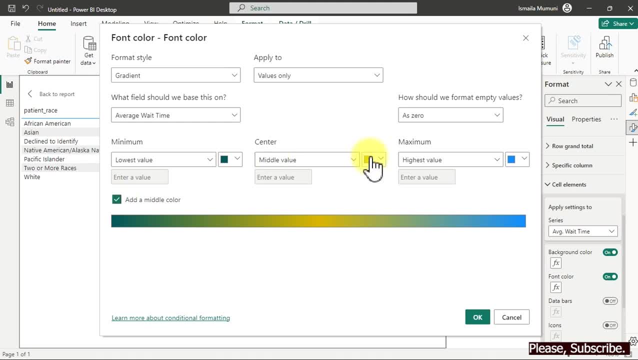 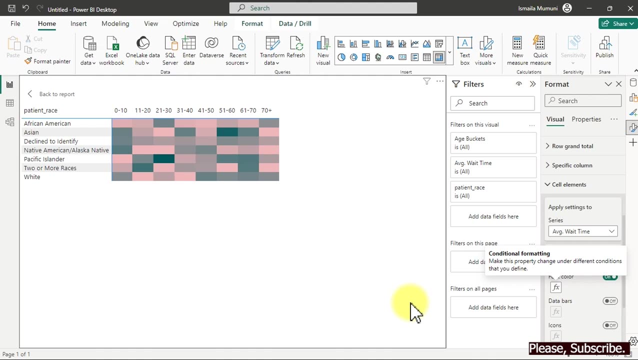 Then we add the middle color again, We choose this same color. Try to remember the colors you're using. Then this would work better. Then we click on OK, Now this is what we have. So anybody can actually come to this now and look at like: Where do we have the highest wait time? 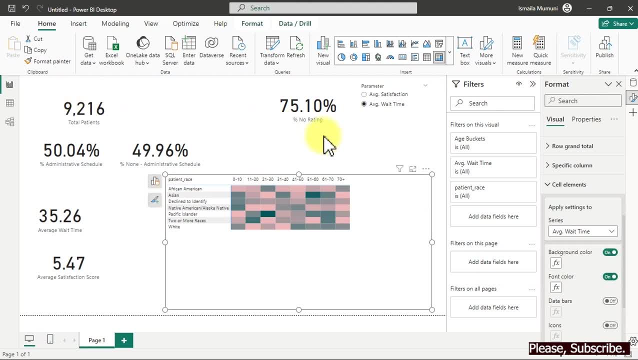 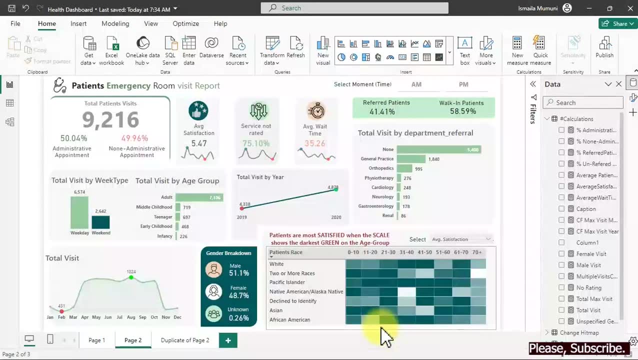 But nobody can tell what this is all about Until we make it some kind of much more readable. And how do we make it much more readable? That is why we have this part to guide us through. So whenever we make any changes from here, Specifically if I change to average wait time- 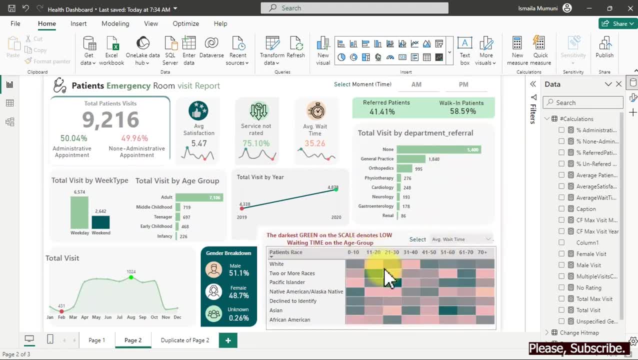 Here now. So it's telling me the average wait time, What it is. So the darkest green Which is this one? This one- Anywhere we have green That is not of this particular color here, So shows what Shows low wait time, Which is good, You understand. 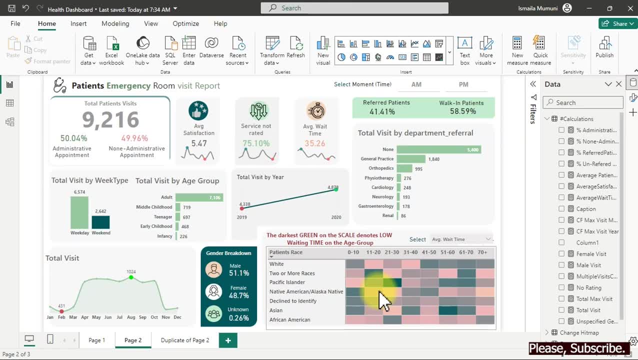 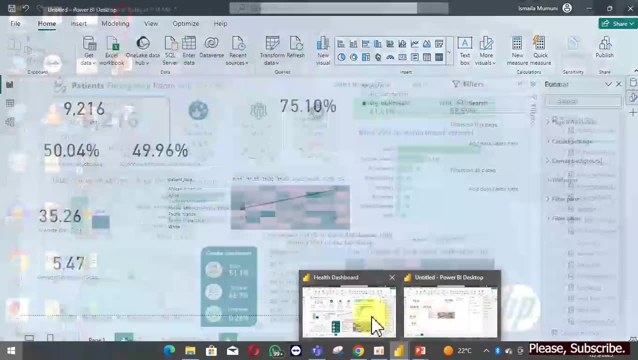 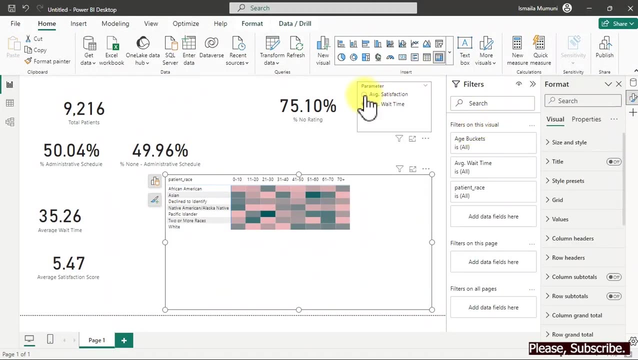 So we don't want to go to the hospital And spend like the whole 24 hours Before we get you know to see the doctor. That is what it is. So we go back now. All right, we're back here. Now. with this, We want to choose our average satisfaction. 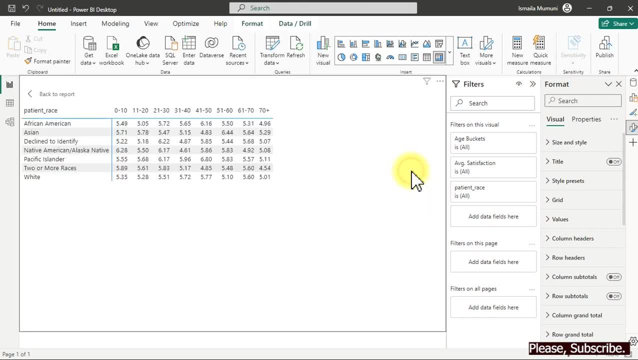 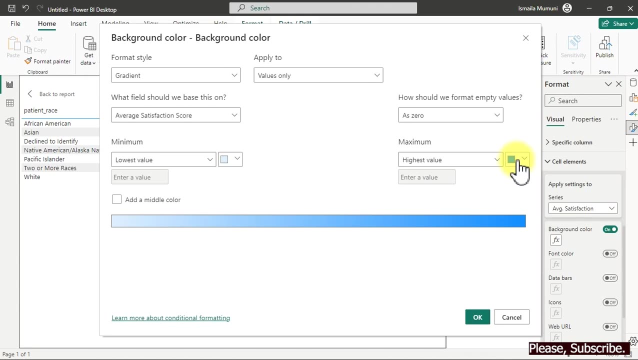 So for average satisfaction, This is what we have. So for average satisfaction, We just have to scroll all the way down And we turn this on. We go right here, So we do. now We want to see where we have maximum average satisfaction. This one is not going to be under low. 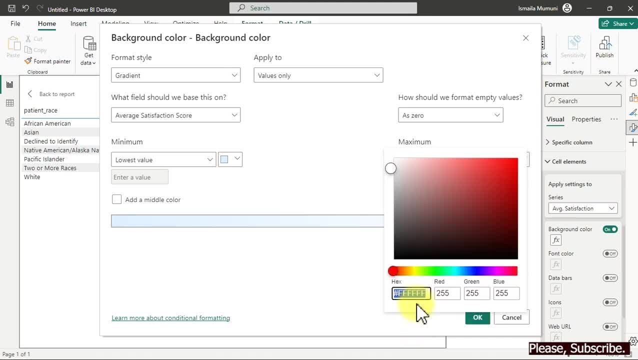 So we click here And we do the same thing. When I say we do the same thing, I'm talking about the color we want to use, So it's going to be the same color: 015756 75C. Okay, This is it here. You can copy it if you want to reuse it. 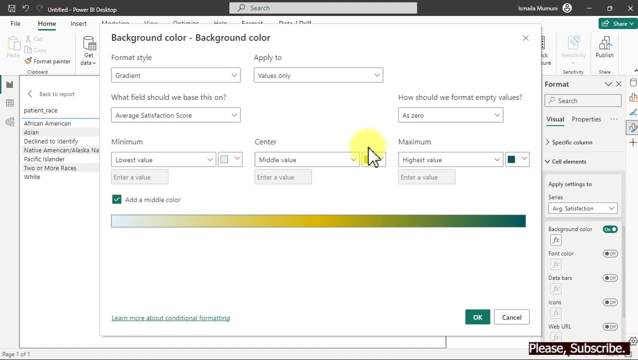 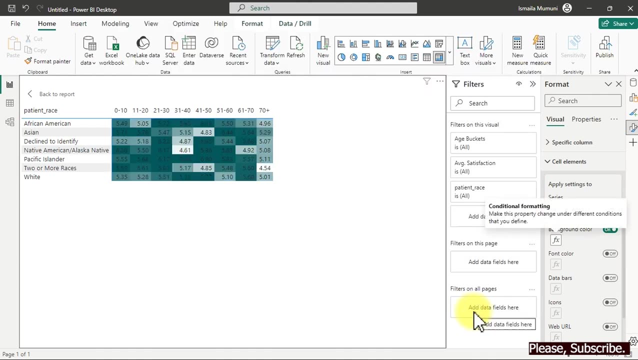 You know what it is. So we want to create a midpoint. That midpoint should actually carry the same color. So here we go. So over here we want to donate for it. white. Let's see, Let's find out. This is how it looks like. So anywhere you see the darkest green. 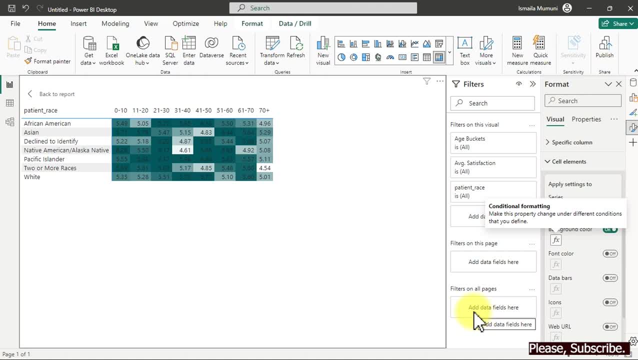 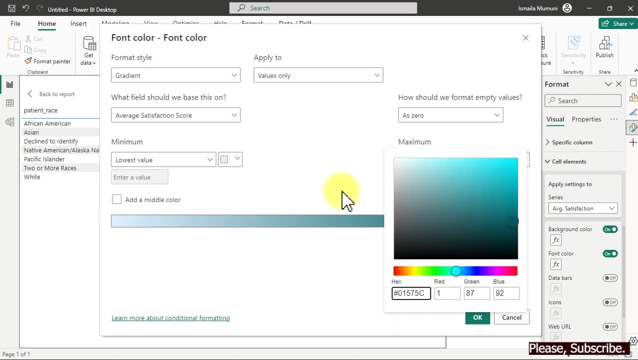 That is where we have the highest average satisfaction. So remember, we have to turn off the numbers, So we just use this part here, And when we click on here We do the same thing. So we have the color copied before. So we come down to here: Add a midpoint. 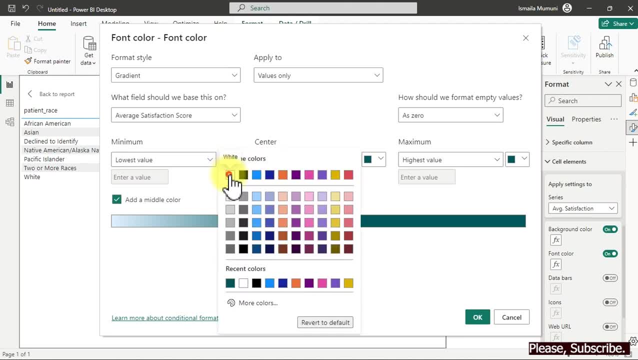 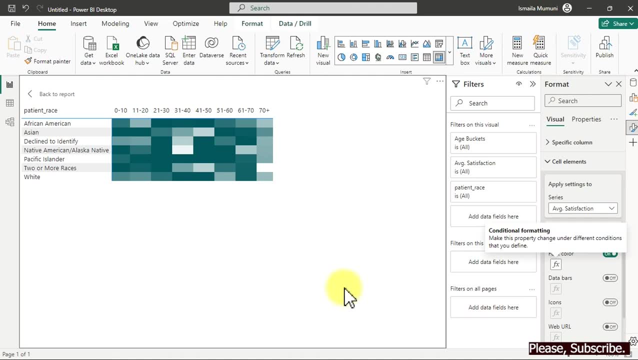 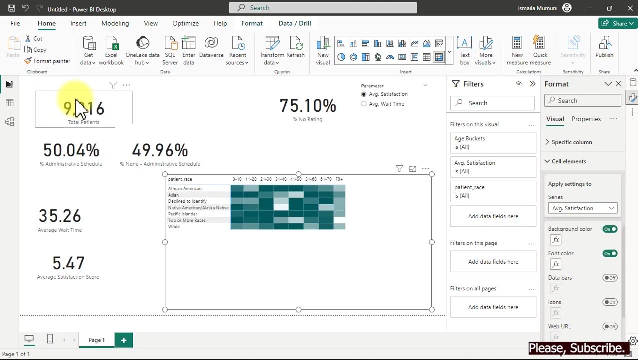 So we get the color Then for this here, We choose this white, Then we go over here and click on OK. Then we have this. So do you look at this now Before we start brushing up this? For now we're going to actually have this here, So we'll actually be cleaning up this. 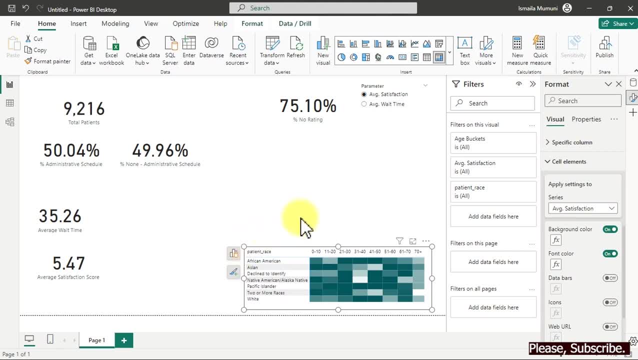 And making it much more beautiful And stand out in no time. But this is what you should actually do. You know what I'm saying Because you really know how to create For the first time. You understand? All right, We want to create one other chart And this chart would look into different kind of people we have. 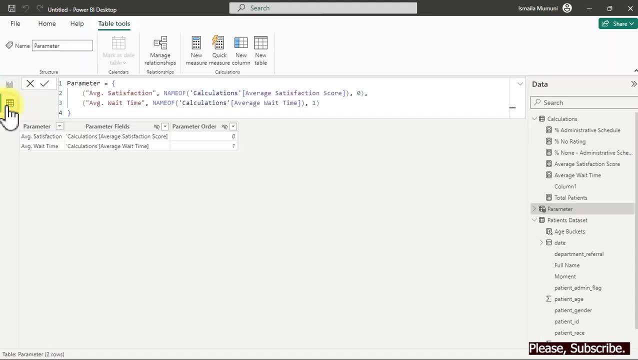 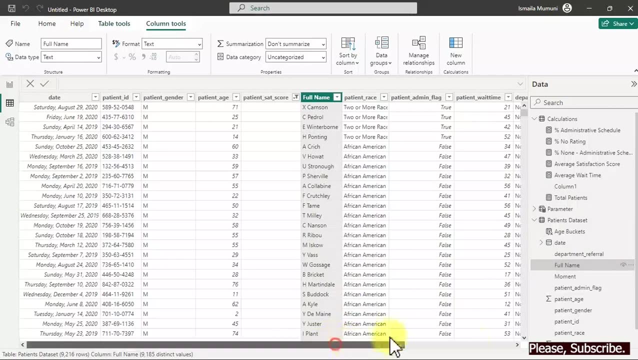 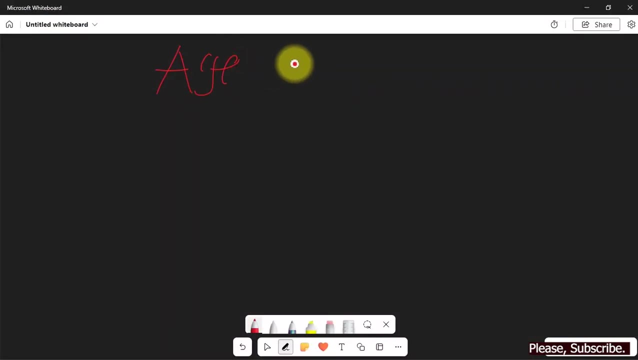 So I call the previous one age buckets. This one I am going to call it age group. So we group our age in different ways Other than this. all right, what you're trying to do on our age group, we want anybody who actually visited our hospital that is actually less than or equal to two to be categorized into what infant so anyone? 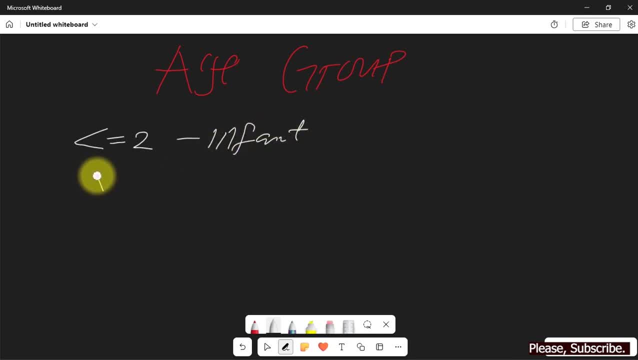 that is actually less than, which is gonna be less than or equal to six. so we want to categorize them on early, you know childhood, early childhood, so if anybody is actually less than or equal to 12, so we want to categorize them into middle childhood. 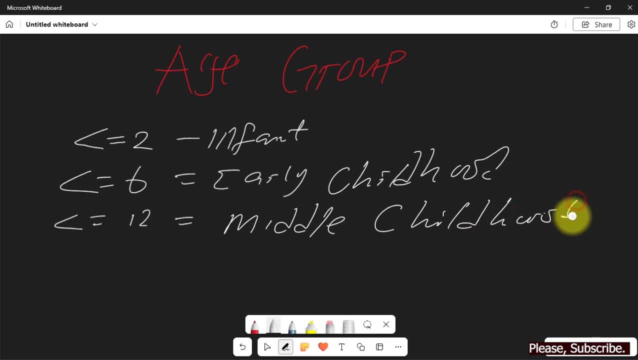 then anybody who is actually less than or equals to what 18 you know, or you know what it is. so they are gonna be categorized to the teenage. otherwise, we want to categorize any other persons into what? into adults. so we can now know this does group of people. how many of them do we have? 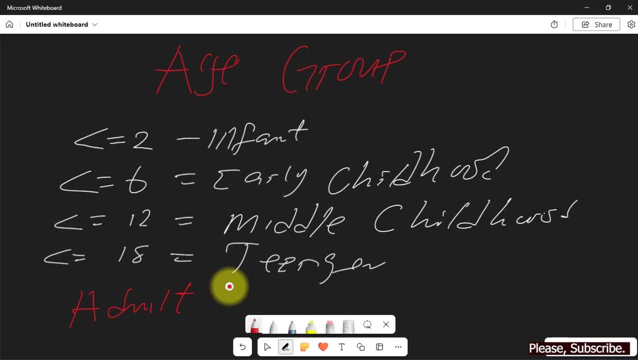 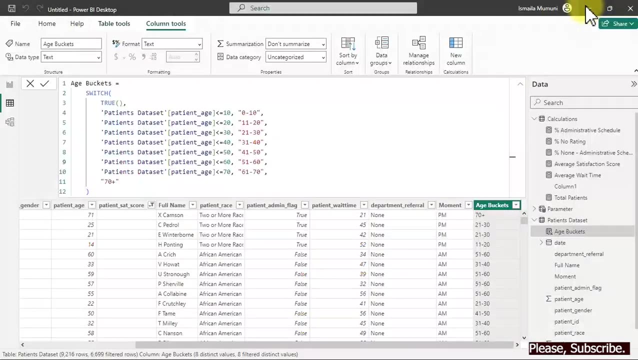 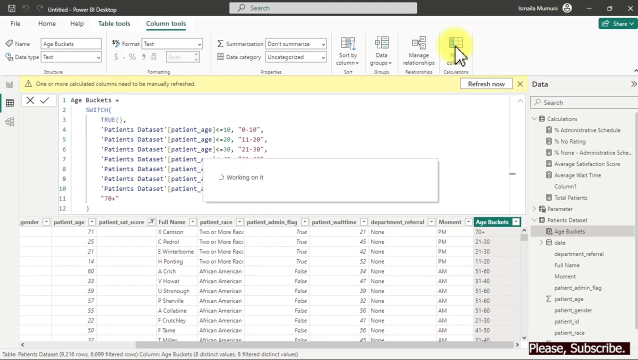 coming into a hospital. we can further use it to filter our data to know their satisfaction rate and their average wait time as well. you get it, so now let's get back to our main part of the work. we're right here. we add a new column, so we're going to just use some couple of switch, or, if either of it will go, 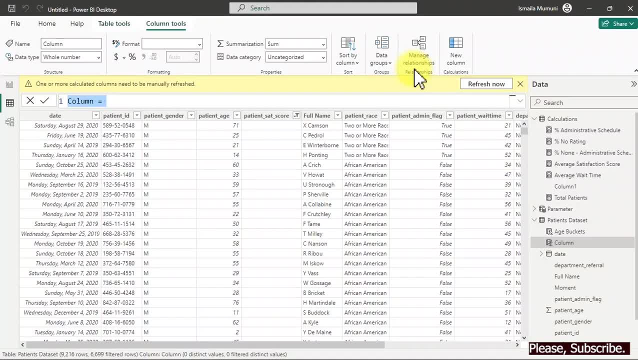 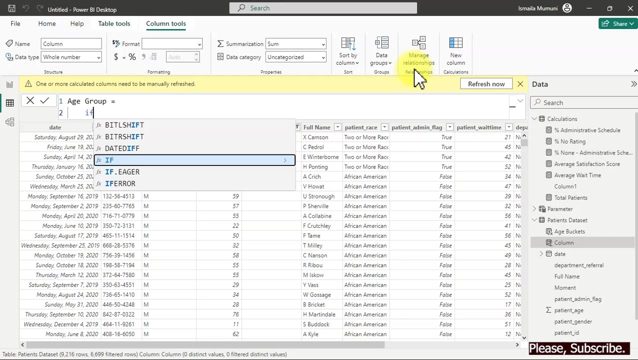 so I will name this one to be my age age group. so for the age group here I would use: if so you can just make it some kind of a bit more weird to refer back to it. so make it something somehow simple, for we just stop, you know, or? 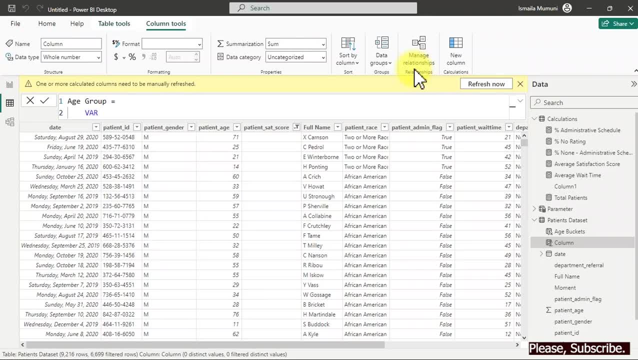 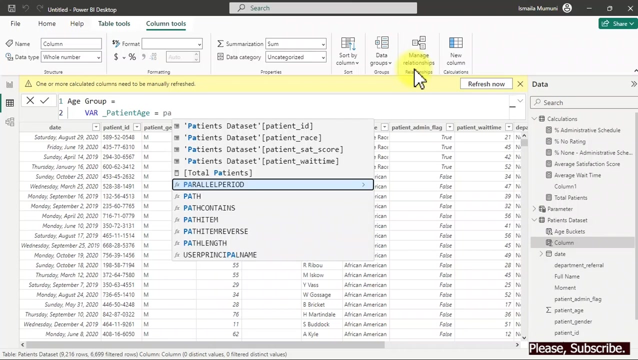 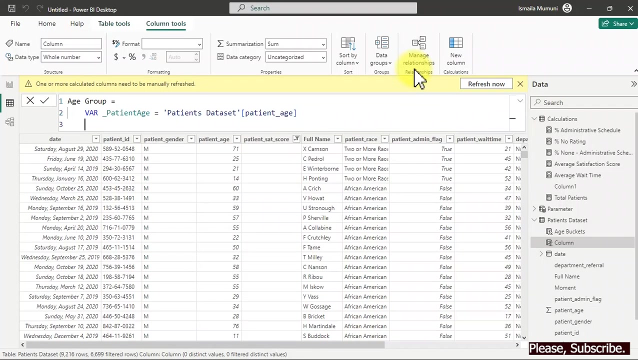 using table over and over again. we can store our column inside a variable, so this variable will be um patient. you don't underscore patient. what age? so equals here. so I'm going to use patient age. so here we have it. so we have stored our patient age there, so we can now come down here now and say: if 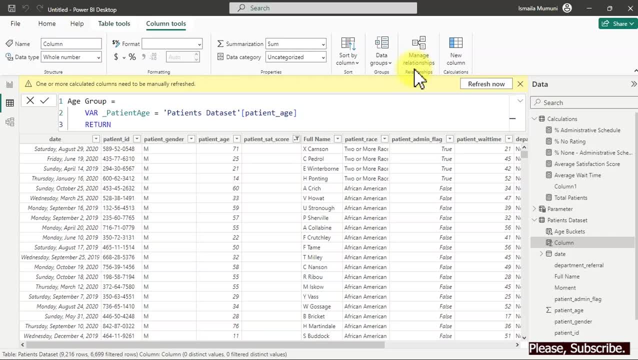 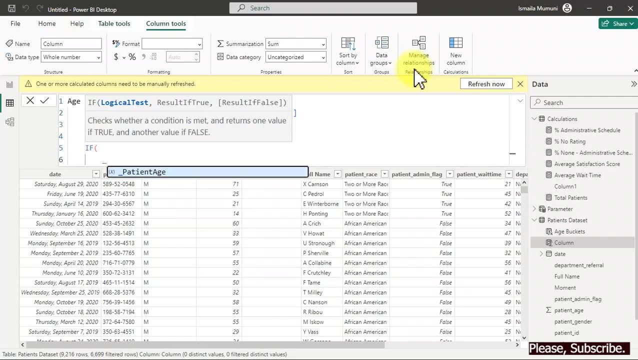 so before we do this we have to return. so under the return here now we can use the if condition to say: if underscore patient age is less than or equal to two. so we want to categorize anybody in this bucket into what? into in funds or in fancy. 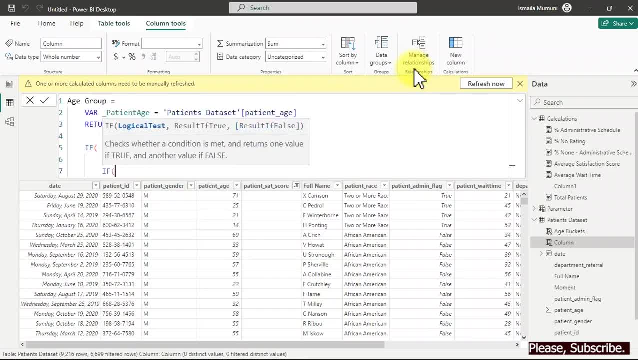 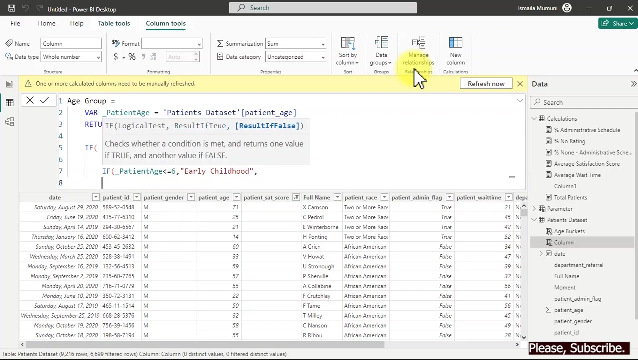 then we put comma. so we nest under if again. so we say if underscore. patient age is less than or equal to six. so we categorize anybody under this particular age bracket into Ellie child hold. so we place a comma, we type in another if. so we say if underscore. 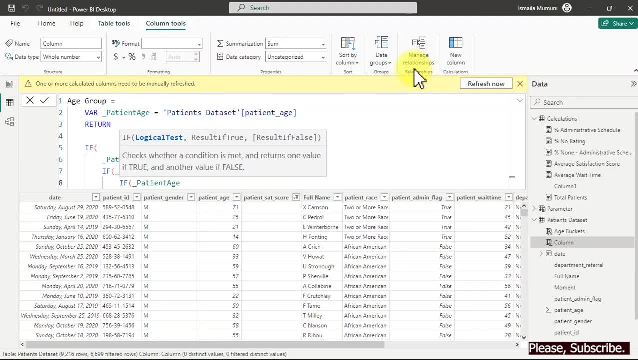 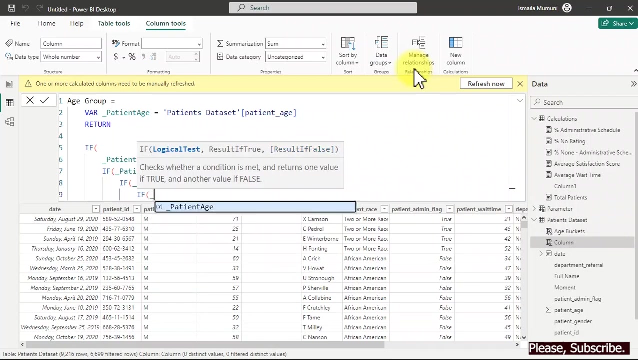 age. patient age here is now less than or equal to 12.. that will give them their mild who so middle childhood. then if anybody again is in, the variable created is less than or equal to 18, so those are going to be our teenagers. so otherwise we want to categorize the remaining one into adult. 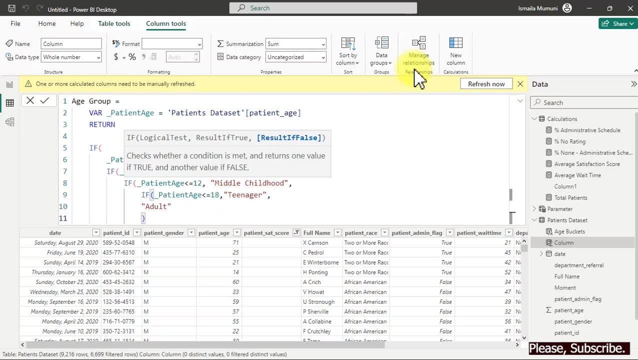 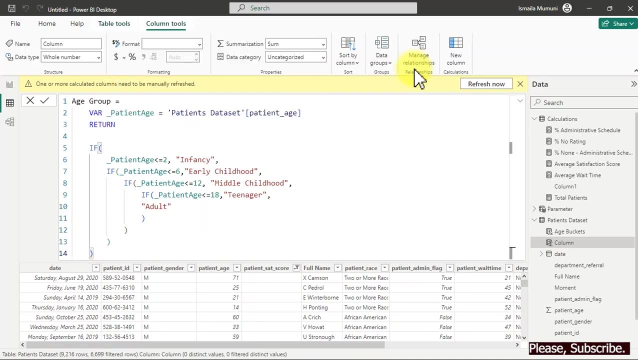 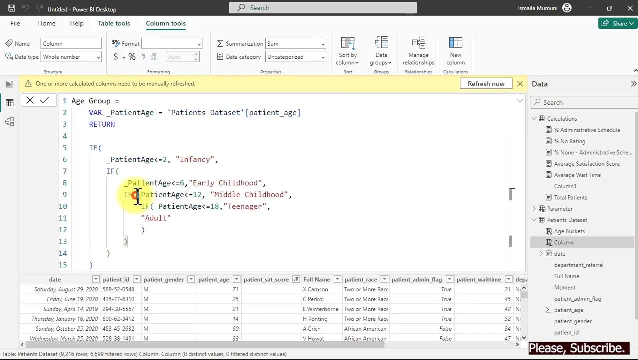 so we close for this. if we close for this, we close for this. I will close for the first. if here we go, so you might. there are different ways to actually invent this. I can just drop all of this. you just drop all of this. it depends on how you want it to go. so this is much more readable. 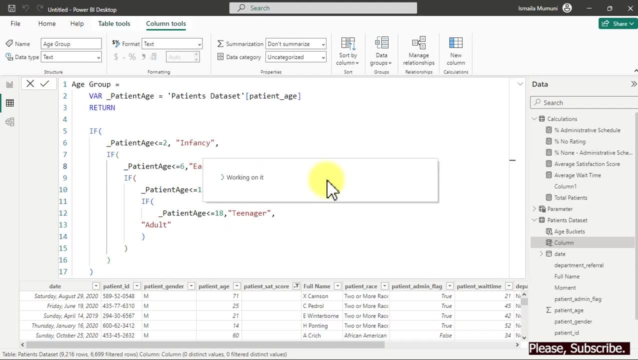 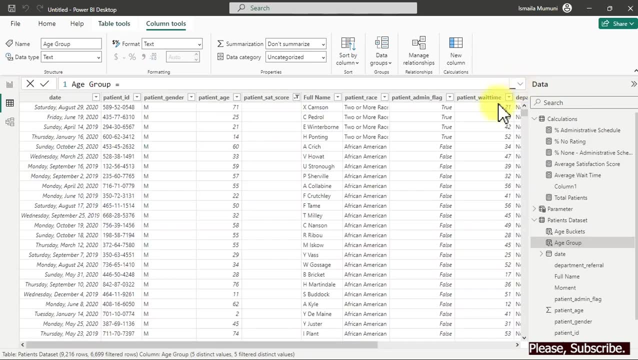 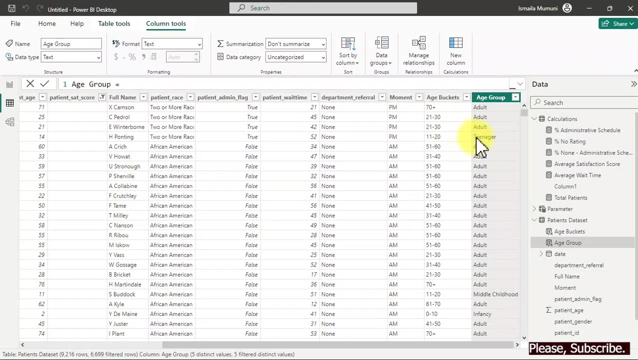 can you see that now? so if I hit my entire, this helps me to create and group all of those people. so you can see now, if you look at here, 70 plus on the adult 11 to 20 is on that teenager- you get it now 11 to 20.. so if you want to get it, 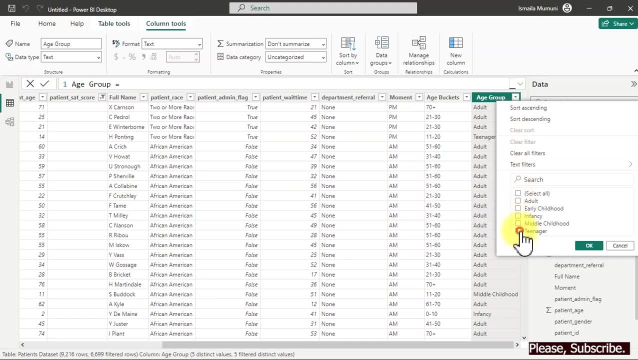 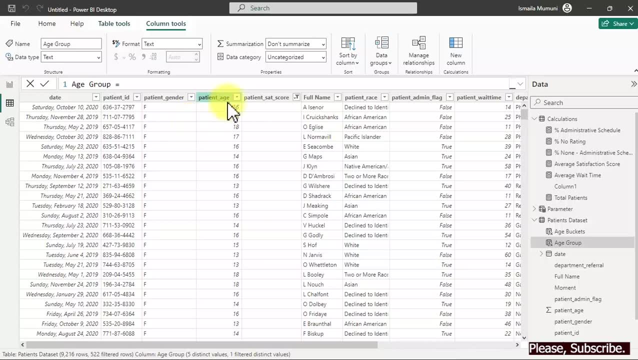 right. so you actually go ahead and filter teenager here. then you go to the age for our teenager under age we just see is 13 to 18.. that is correct. so we've just done that. so before you do this you have to do your calculations to. 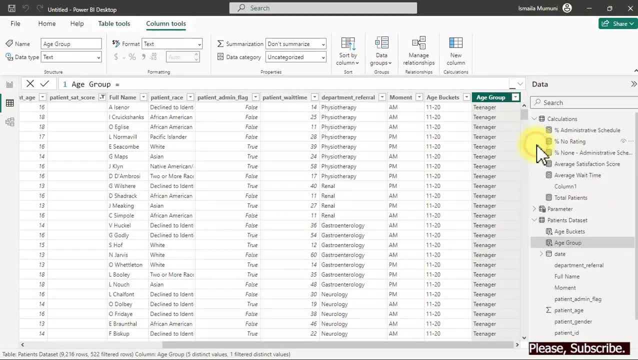 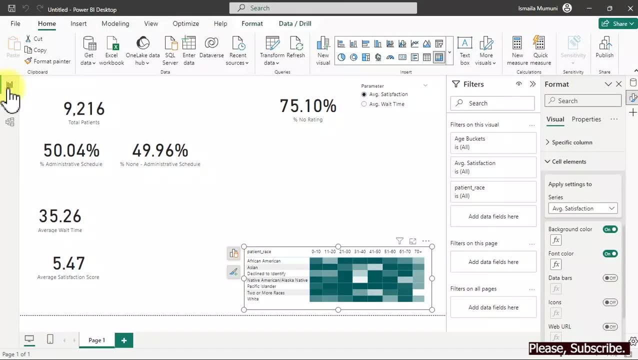 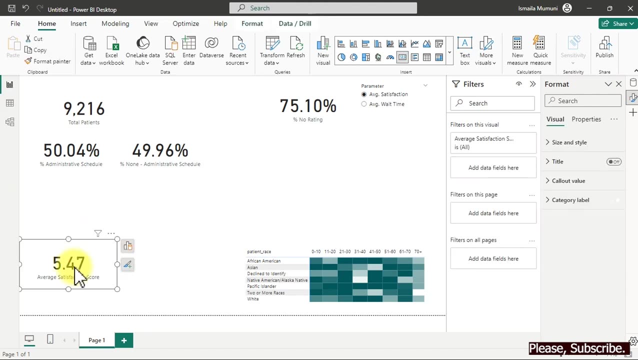 know how this should actually fall. you don't just start writing and it will come the way it is. no, you have to actually do your calculations. so we've done this. let us look at what we can use this for. I would definitely remove this. I'm going to remove this for now. 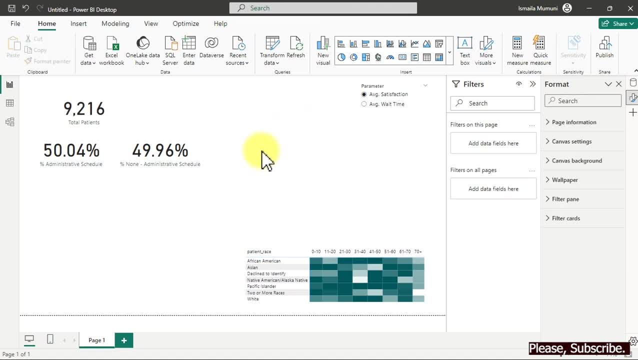 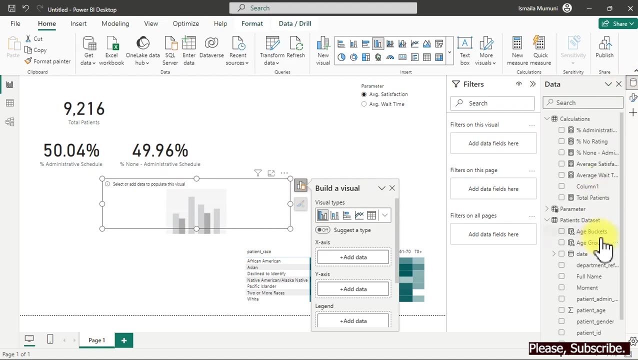 then I'm going to get this off for now. so we create a chat with that. so the chat we're going to create, if we want to go with this chat, let me tell you the disadvantage of using this chat to actually visualize something like this. let's go over here and I'm going to go. 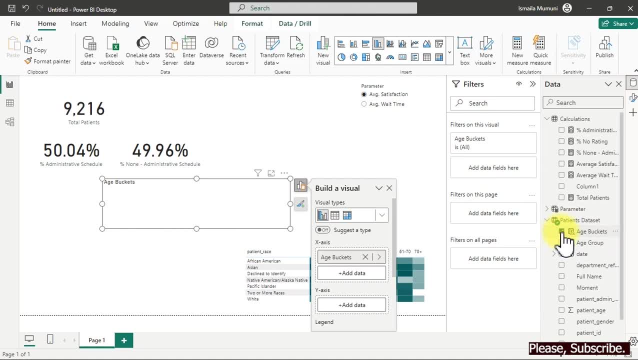 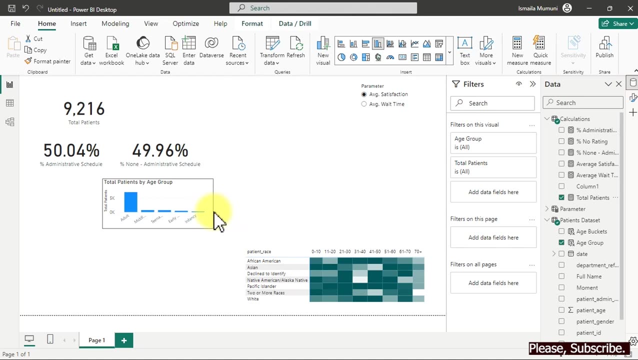 to each bucket this time, or the input eight buckets. I think that is going to be our age group. so here is our age group and I want to say it by total patients that we have. so now, if I want to make sure it actually occupy this small space, 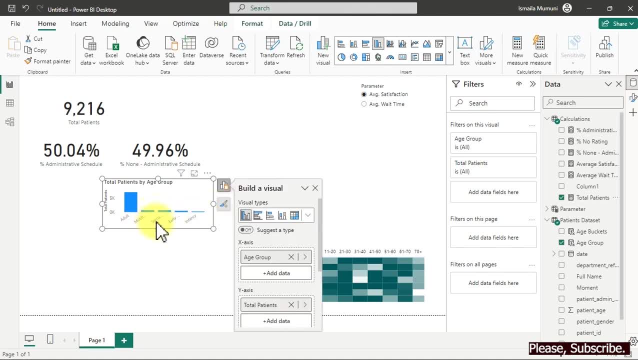 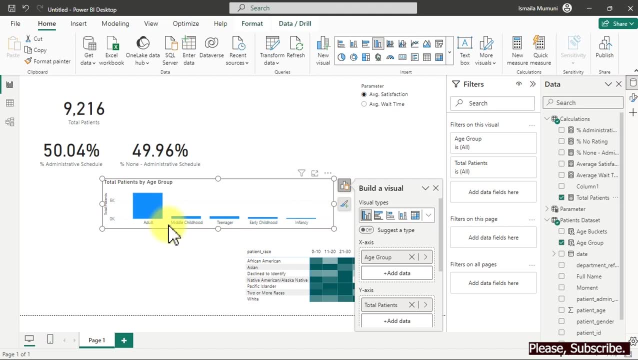 here. so our x-axis is not going to be readable, so it has to take up to this level before we can read what is here. so we want to actually use a small space with this in order to have other charts, you know, sit in the report. then definitely, if I compress it, it's still not okay. 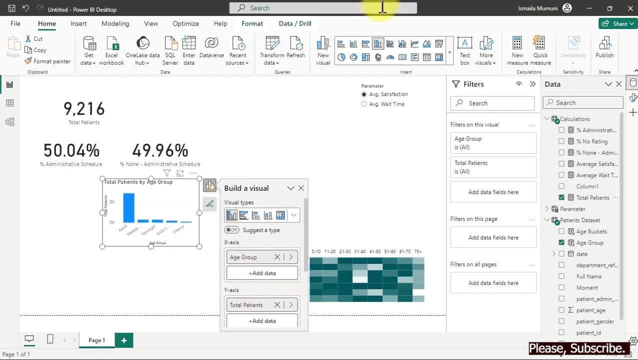 so what do I do? I would rather use this chat to convey my message. so this looks beautiful, but it's not looking nice at all. what do we do? we'll clean it up and it will definitely look okay. watch it. so I click over here. if you're still watching and you have not liked, please hit. 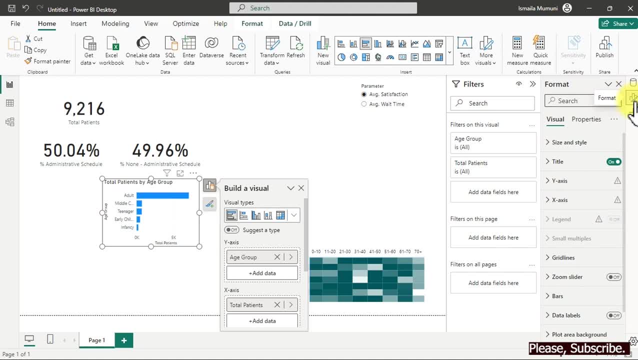 the like button. it's very important to me, and if you're not subscribed, you might want to consider hitting the subscribe button right now. so leave a comment let me know what you feel about this. on a continuation, we can actually come over to the y-axis first. 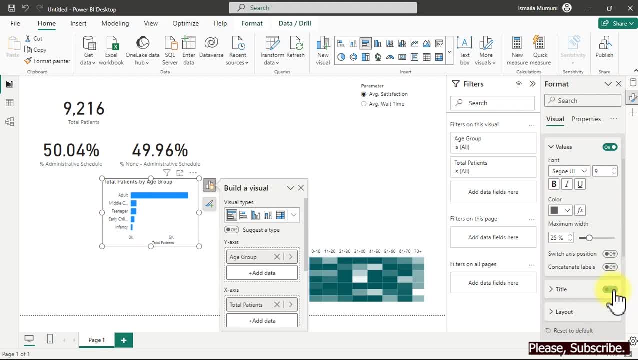 and we scroll down a little bit, we actually turn off the title. so when we scroll back up we have the x-axis here. for the x-axis we have to turn up the title and as well the value. so it's looking much more okay, but something is still wrong. if you look at. what is wrong right now is: 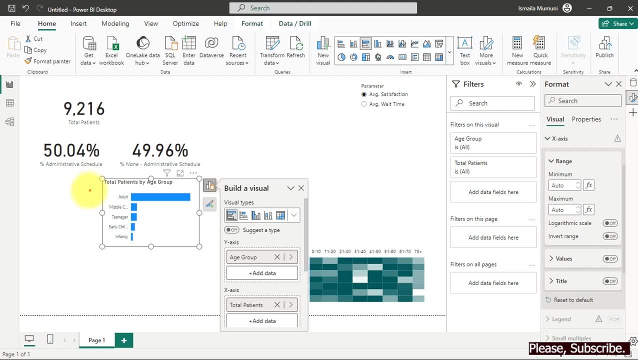 that this particular y-axis here is not in any way somehow readable. so how do we fix this? we have to fix this under the y-axis. let's find out. as long as we are here, we can bring up the y-axis. so what you're going to change is this one here. 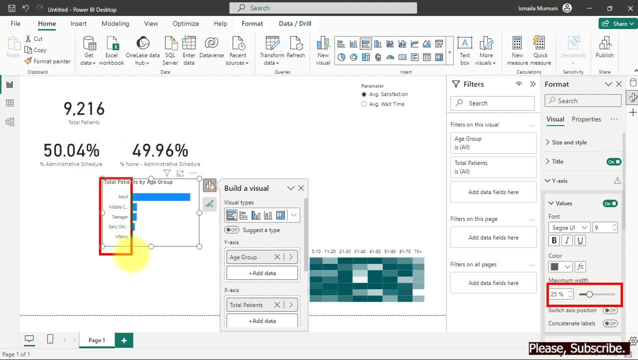 in order to correct all of these that are not appearing. well, let's do it. so just move this to 50. if I bring this to 50, what you have, if i bring it to middle, you still have something a little bit weird. so bring it to. 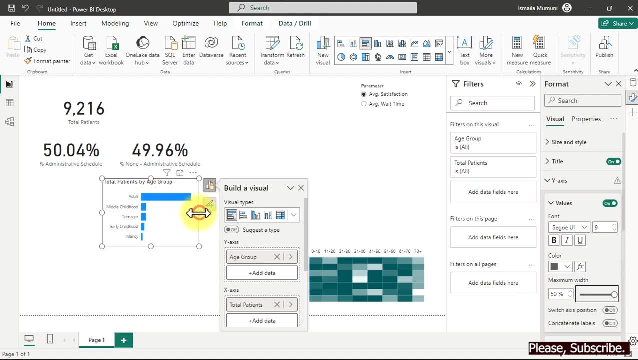 50. so with 50 now you can see when we move this now, before it affects this. how is some kind of cool? so it will take time. this is what we want to have on it. can you see that beautiful? so you might want to stretch it a little bit and make it like this: 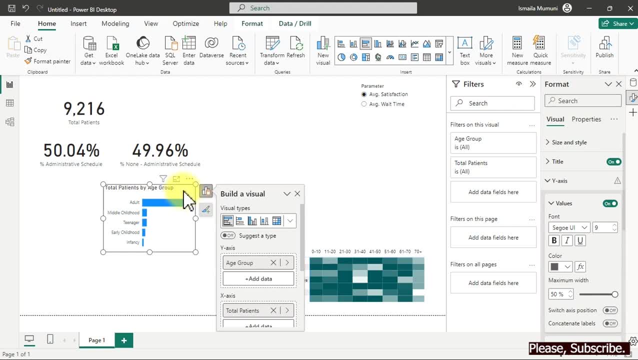 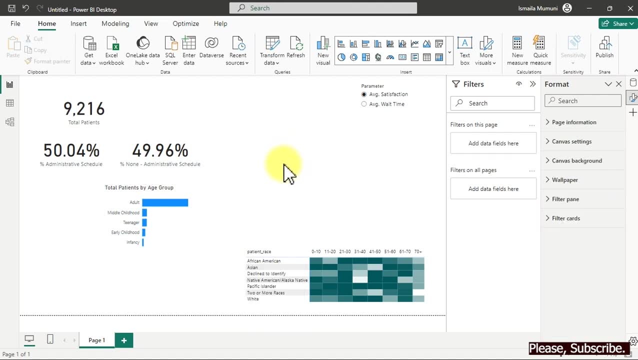 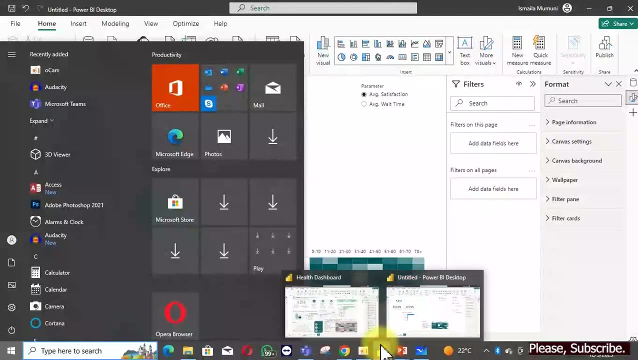 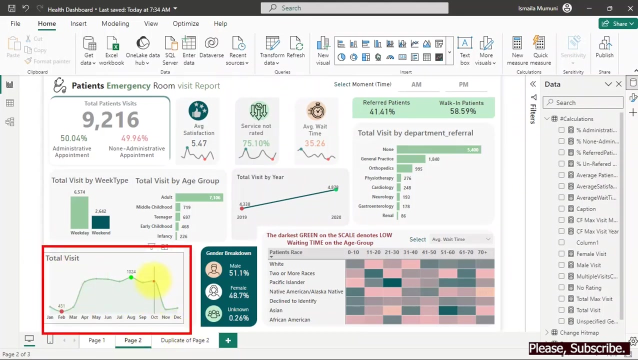 so, after having this, now we want to have a line chart that displays our visits, our total patients that we have every single month. over here we can see the conditions that we have of line charts that we have displaying our visit and my most important part is marking this: 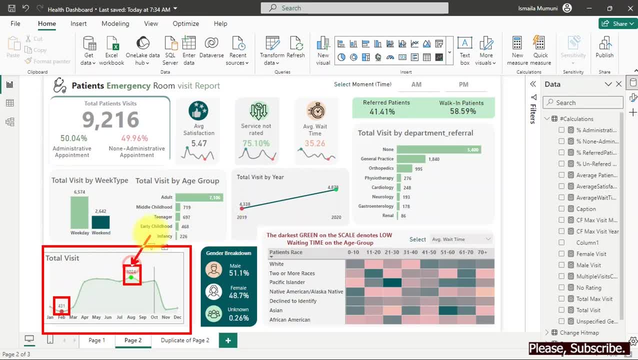 particular part. so this part here, what is it showing? i'm talking about this very part here. this part here shows the highest month we have more people visiting us or visiting our hospital, we have more emergency and this is the lowest month. so we did this to be able to draw people's. 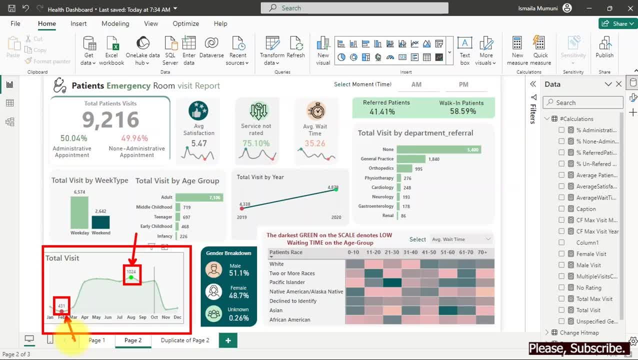 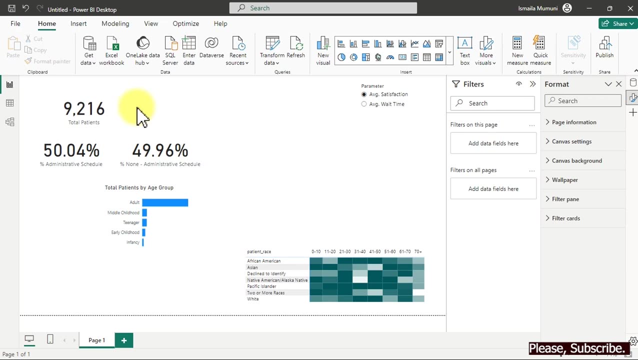 attention into those particular two months. this is not just a line chart. you have to customize it using dax. this is what we're about to create right now on our project. let's get it. in order to create that, we need a simple date table. if i talk about simple date table, we don't have to spend much time. 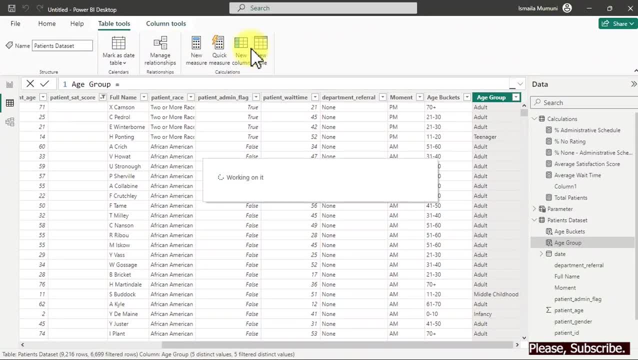 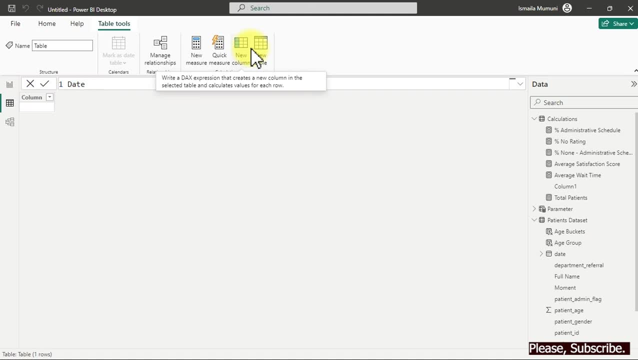 so we just have to create a table and in this table all we do is just to create what? to create date. so i'm going to come right here and just edit. so inside my date, i'm going to use calendar auto. so this calendar auto helps me to generate my date. so if i hit my enter key now, let's see what. 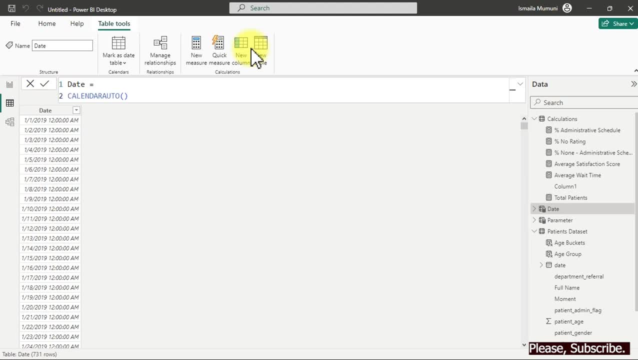 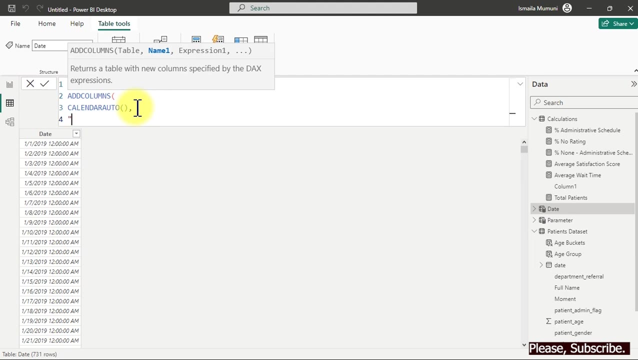 calendar auto has done for us. this is what we have. then we need to add some columns to our calendar auto so we come over here and use the add columns. so when we use the add columns above calendar auto, we put a comma right here and move down and we say we want to add here, inside this square or inside. 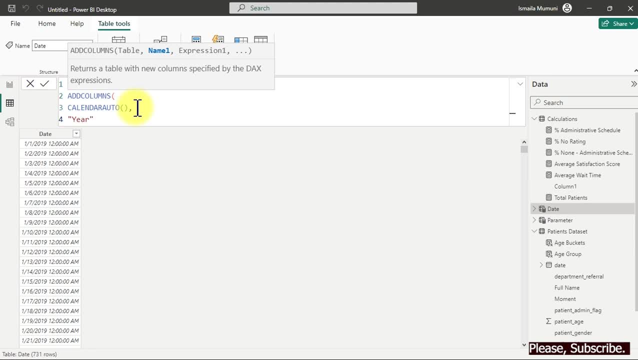 this particular quotes rather. so we type in here to extract the year and comma. we use the year function and date. that's going to be the date column. so the date we have here now, if you look at it, is different from this particular, you know date. this date is actually a function. 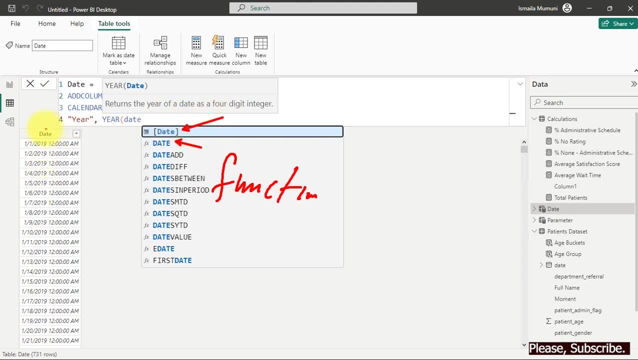 so this one here is actually a column and this is the column we have just used here, so which is the one inside the square bracket. so we have a date here. so i'm gonna grab this. i'll close it. the next thing i want to do now: 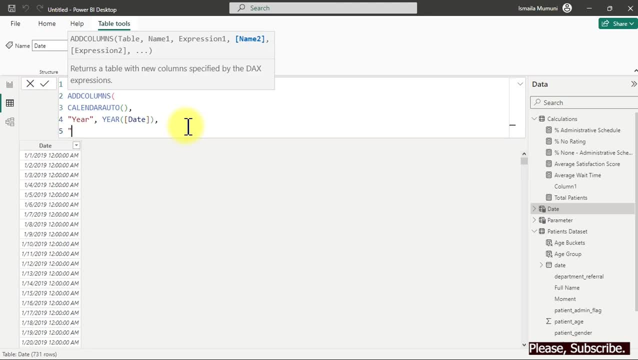 is to extract my month. so. so i'm gonna do what to extract my month. what i need to do now is to use format. oh sorry, do this format. and for the format now we need a date. so we want the month to be a short format. so we use mm, triple m. then we are done with this, i can close my format. 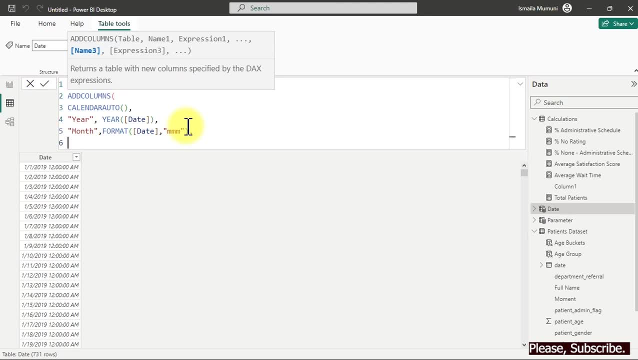 i'll place in that comma again. i will now actually do for what do i want to actually get my weekend and weekdays? how do i do this? so i'm going to type in here with type. so, for the week type, what we're going to do right now is to say if 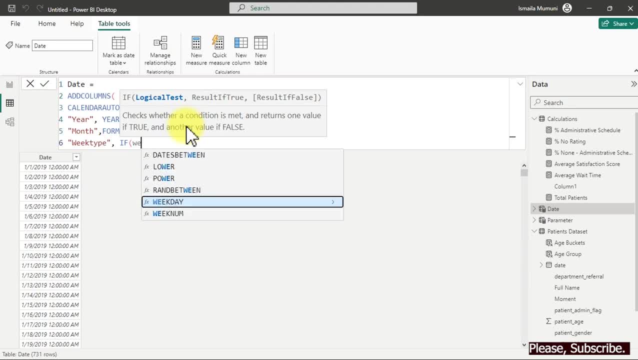 so using the if function. so we're going to actually ask the if we have what to call weekday, the weekday returns numbers. so those numbers would actually range from one, two, three, four, five, six, seven all of that. so one is always a weekend and seven is a weekend. 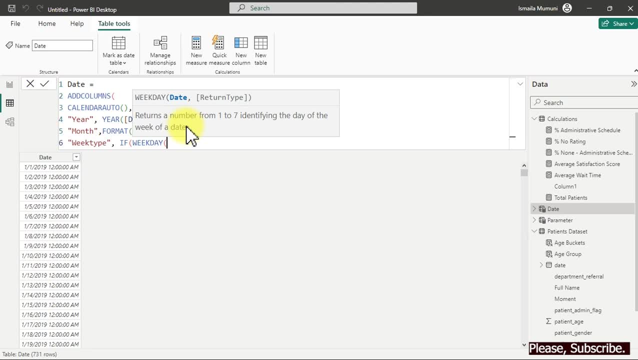 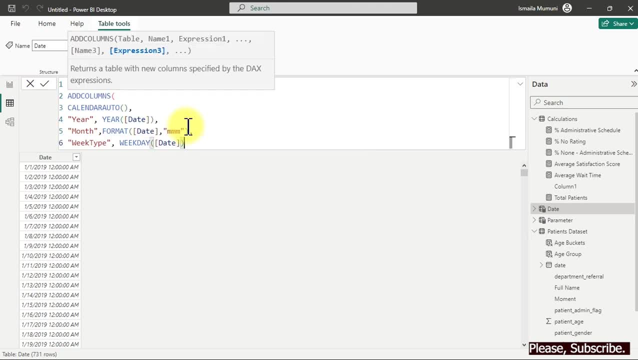 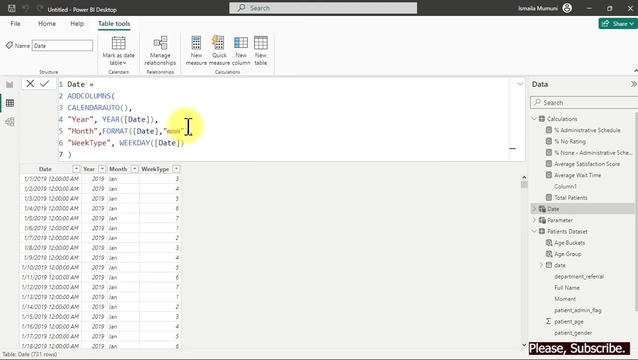 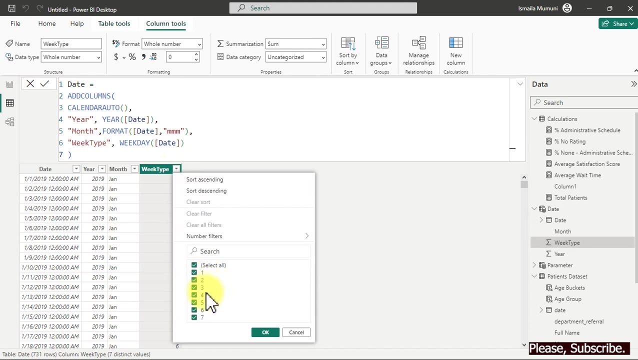 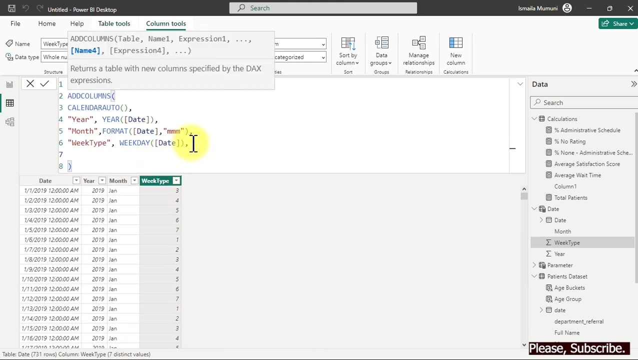 and i will go ahead and close it. so now i'll close my add column. i'll hit my enter key to extract this first before we move further. so if you look at my week type here now, it's telling me that i have one, two, three, four, five, six, seven. you get it. then i'm gonna extract one more. so 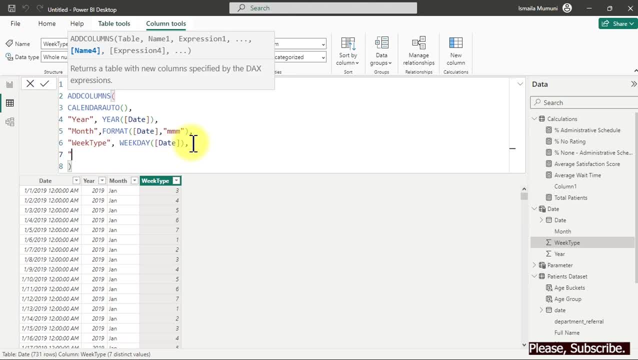 this one will be my weekday. then for my weekday now i will use the format. for the format, we need the date right here we do the day to have the shutter form, so i'll hit my enter. so let us look at what every one of those numbers are attributed to. three is for tuesday, then seven. 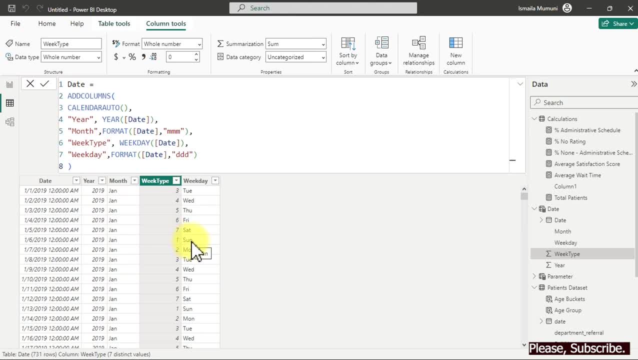 is for saturday and one is for sunday, which is weekend. we're gonna use seven and one to actually customize our week type here. so for our type here, we don't want to keep it, we don't want to keep the numbers. instead we just extract what extract the week type, either weekend or weekday. so we 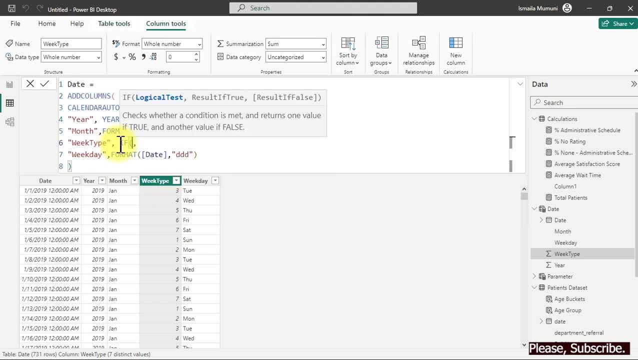 gonna use if over here. so we're gonna say if calling the function weekday here, if the weekday, how do we extract the weekday? we extract the weekday with date is equals to one. so we have to close our date first, close the bracket, so now it's equals to one. so what do you want if that is the case? we want weekend. 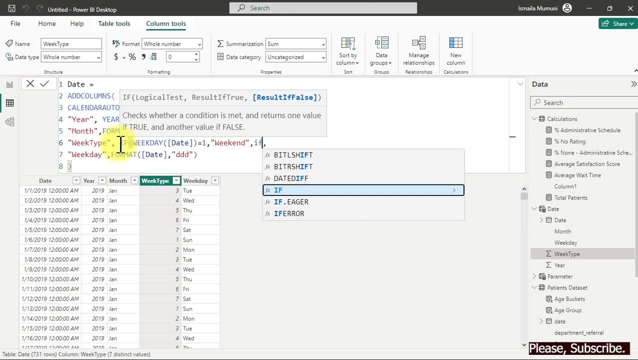 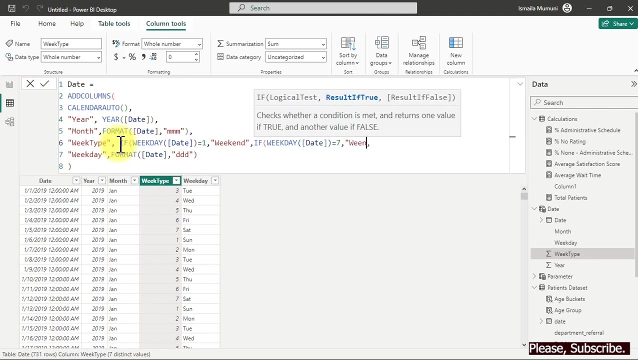 then we close, then comma, so we nest on that. if again, if weekday the date, so we close, and now it's equals to seven, so we still call this what we call this week end, otherwise it will be what it will be: weekday. so the person let's say that we closed one, we will close the last one. 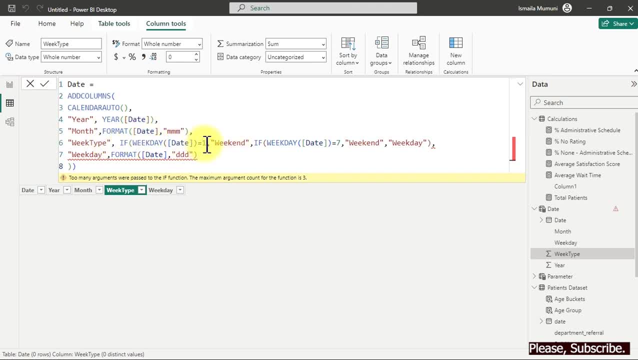 so look at it. oh no, we have an error somewhere. let's see where that falls to equals to one. that gives us this. so if the week that is equals to seven, we have this weekend again close the last. if so, we have to place in the bracket here and now hit our enter key that. 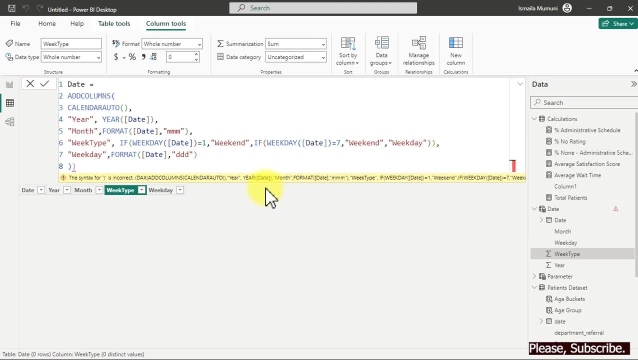 would definitely correct this for us. it doesn't- yes, it should be, so we have to remove this one here- that the system automatically placed here. the system went ahead to help us close it, but it did it in the wrong direction. so now we have two types of week here. either it's a weekend or it's 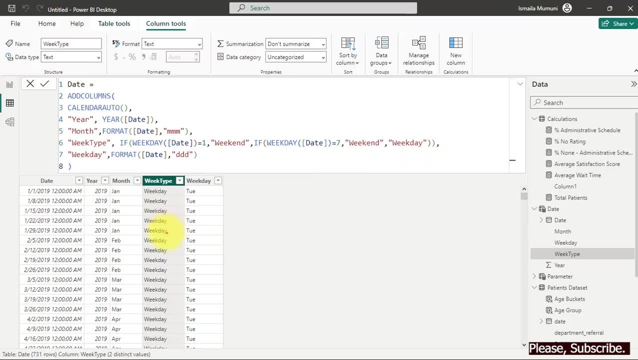 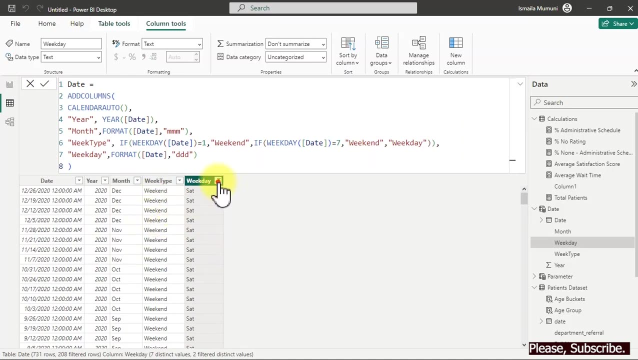 a weekday. so for our week end- let us try to look at that. so we have weekend to be sundays. so if i come over here now and just do saturday and sunday here, so it falls on the weekend, which makes it correct, so we can clear the filter from here. clear the filter, so let us go ahead and take. 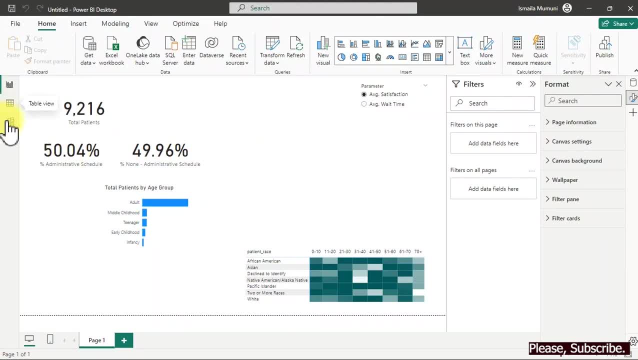 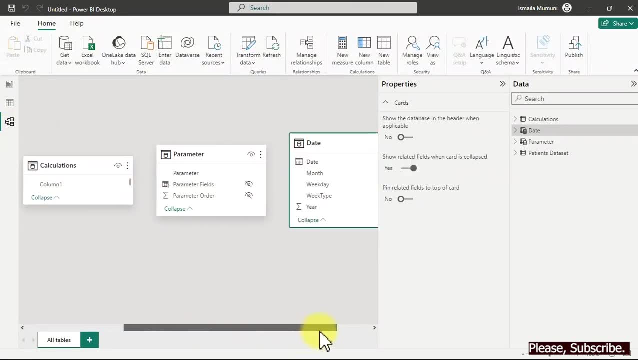 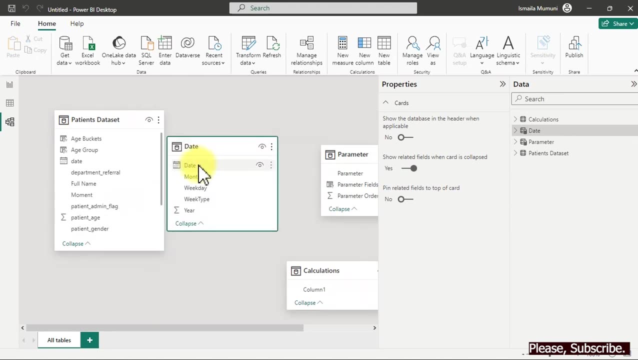 a look at what we have done here. first of all, before then we have to go all the way to the back end and try to connect our tables together. let's move the table here. those are the two tables that can have connections, so we're going to connect our 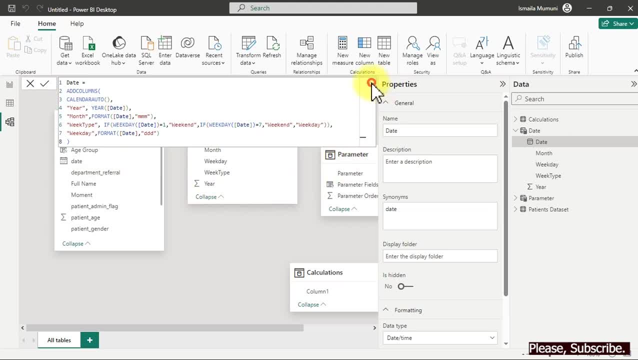 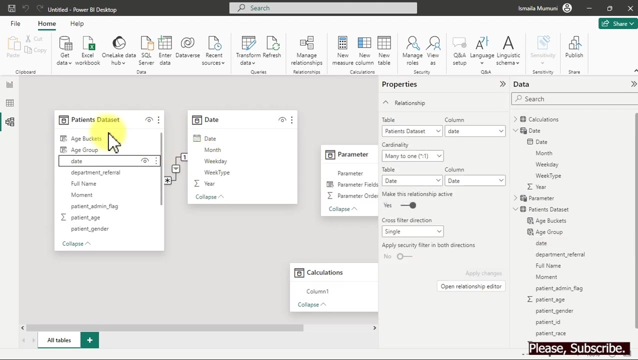 table, which is this very one here. now to this. so we have the date column here on our main fog table. we can drag it and put it on top of this particular date. so we have created one to many relationship, or many to one relationship rather. so we come over here now and we're going to connect our table to this table here. 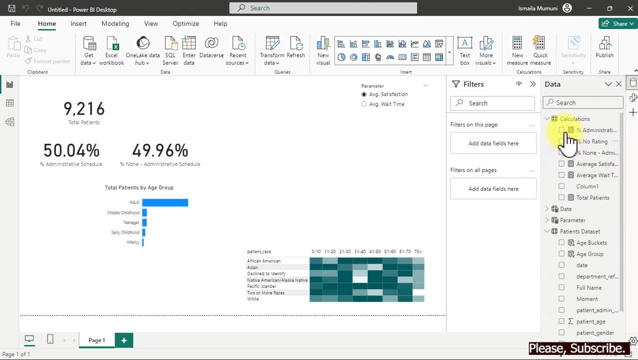 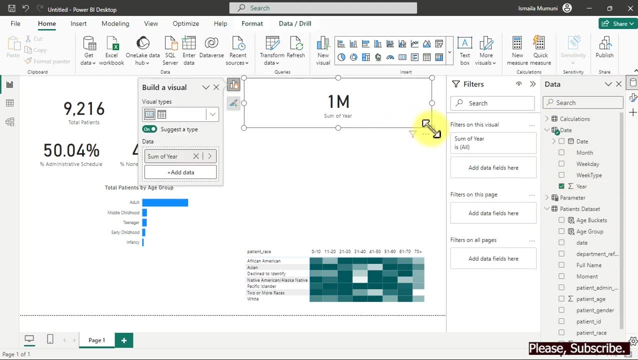 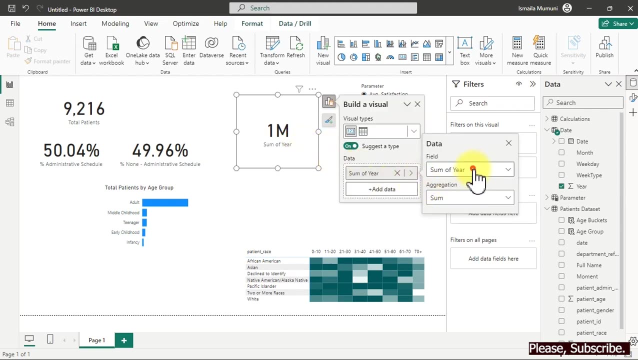 let us bring in something like going to date. so we bring in the year, so the year is summarized for us, so we can now choose this particular sum and we say: don't summarize. so it's giving us two years of data. we can now try to look at it. 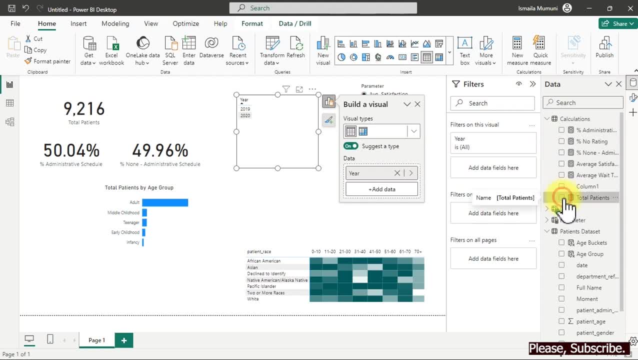 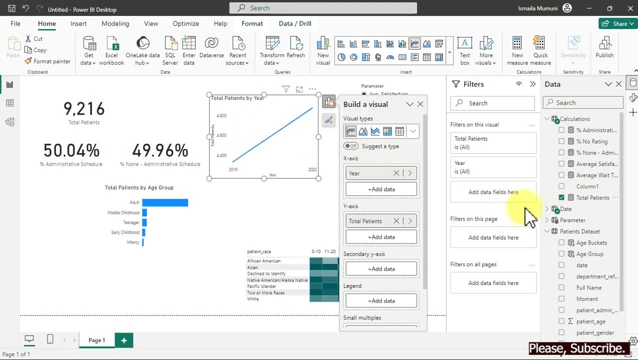 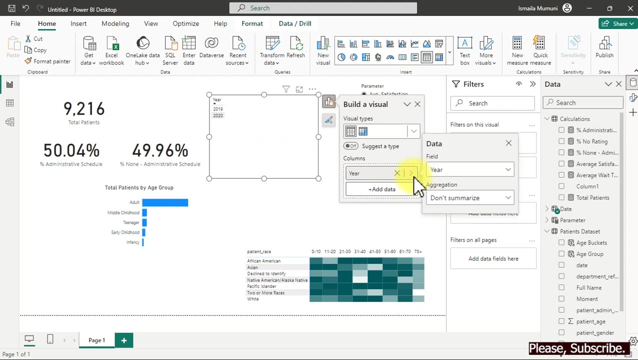 if this is really correct, we pull in our total patients, so it gives us this. can you see it now? beautiful, but something will happen. i'm going to remove this now and convert this to a table. instead of me having my year, i'll bring in my month, which is going to be this one. so if you 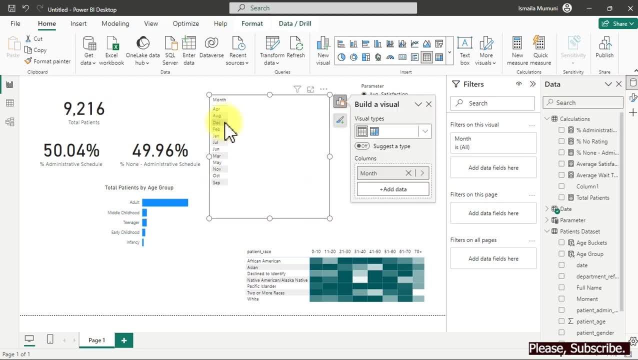 look at my month. something is a bit wrong here. so that is because my month is starting from ebry, the Chinese New Year. for when my month ends- September 2021 or 2019, or end of the year, maybe September 2021 or 2020- it means full moon, obvious and well hoop, because my month is starting from April and my month 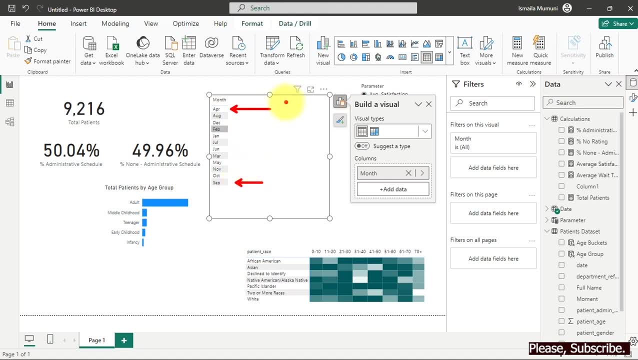 ends at what? at September, 2021 or 2020? then we have already added the month and the month is starting from June, which will be our day month is starting from September. so we are supposed to start the month and we are going to downcharge October 2019 and we are supposed to start before it gets closer and deeper. 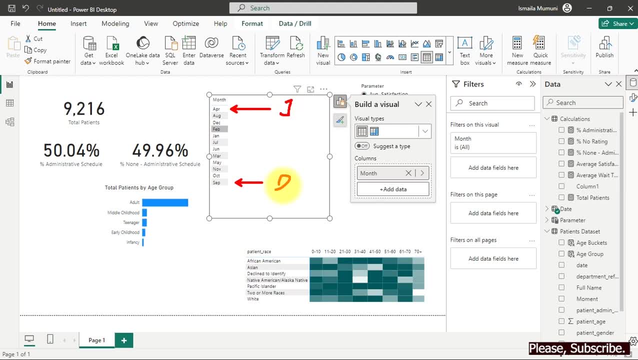 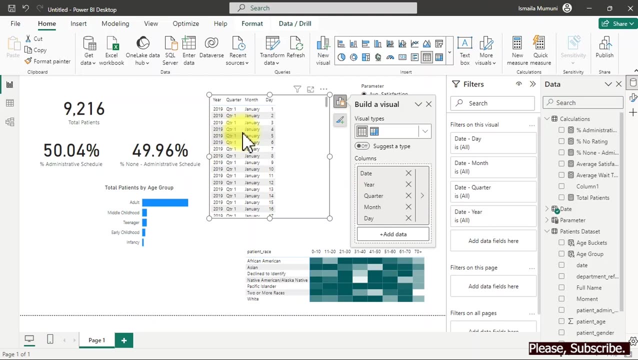 to january and the month should end in december. that is not the only thing that is wrong with this date. let me show you something else. so, clicking on it, i'll go ahead and grab my date, my main date, not the other columns, this one, so my date is still just like the default date. that 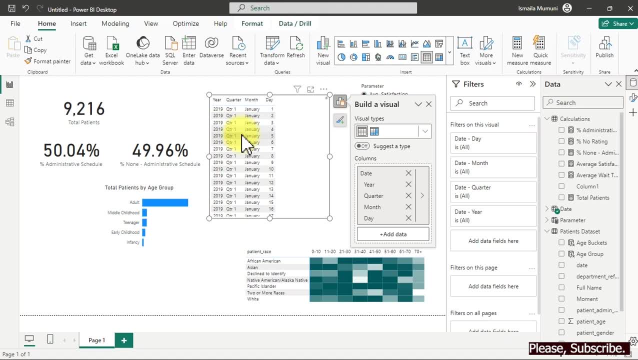 power bi has for us. so we have to change the look. how do we do it? we have not actually told power bi to stop using its own way of date format for us, so we need to do that, telling power bi that we have our own date table. so go all the way to here. so we are back here again. so click on this particular. 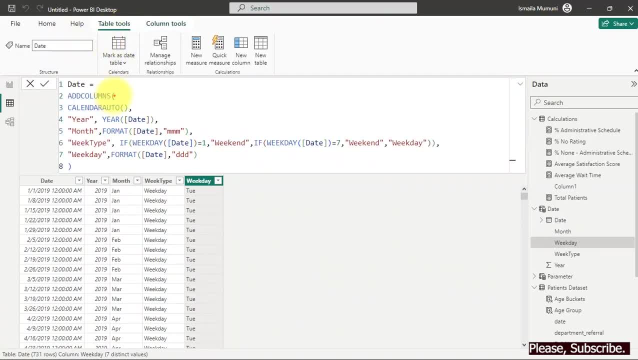 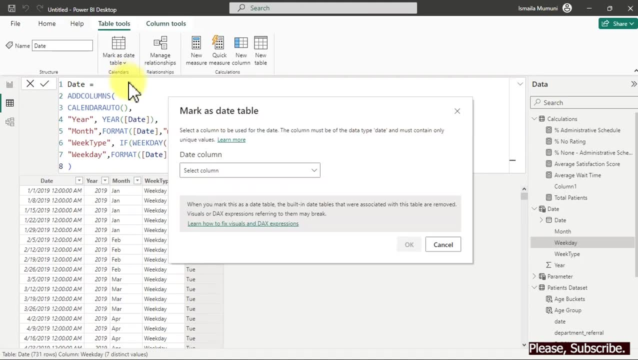 table tools and here we have mark as what you have to mark as date table. so we mark that date table and that disconnect the power bi default table and replace it with ours. just click on ok, here that problem is solved. let's get back and look at it. 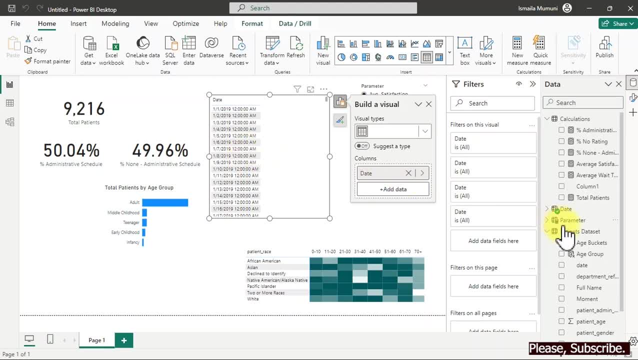 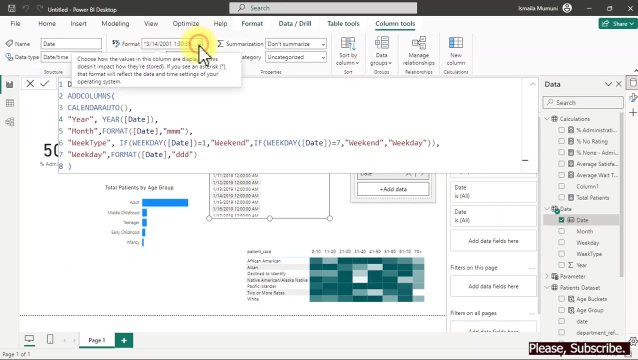 can you see it now? it's solved, but one thing is not yet done, so i'm going to come here and solve it from here. so click on the date itself here so you now see where you can actually format your date accordingly. so i'm going to use a shorter form that will clear off the time for me. 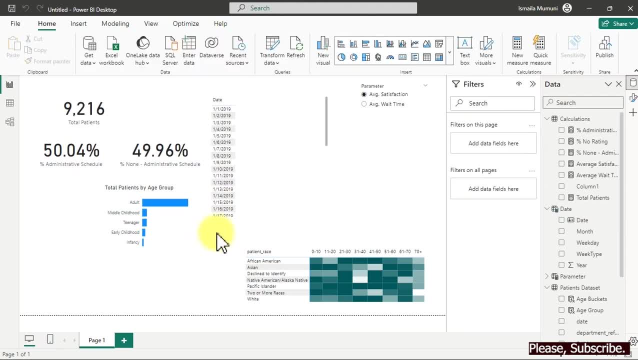 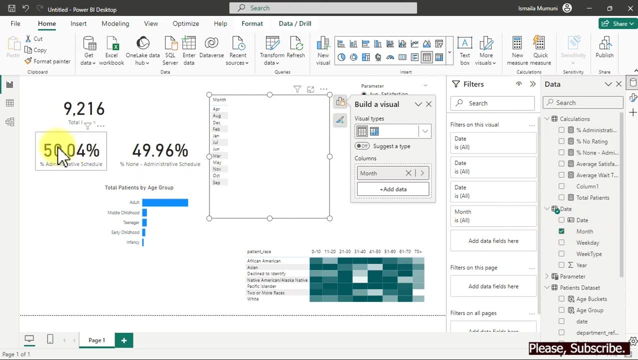 beautiful huh. okay, we have one more issue to actually solve, and that issue is the issue of the month. how do we fix the month? to fix the month now, we can be here and fix it. we don't have to go back to the data view. just click on it here and over here. you see where it. 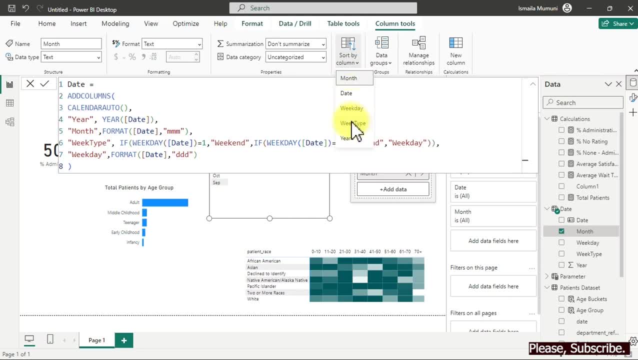 says sort by. so we want to sort this by what by month number. sorry for that, we do not have it. can we create it from here? yes, of course i'm going to add a month number here, just add a comma. so with comma i'm going to type in here month, inside quotes month. 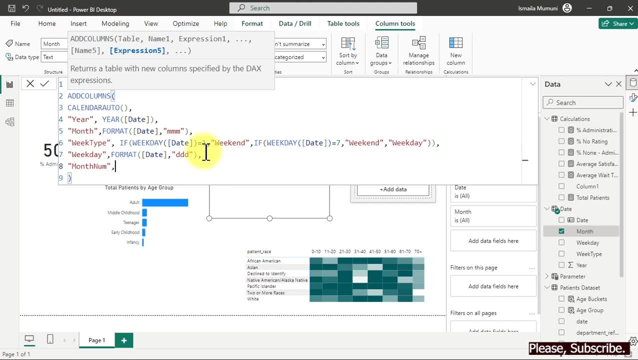 num and with the comma. i will definitely use month as a function and i'll bring in my date. that is all we need to do. we just do this and we hit enter. so let me solve this particular issue here and later, after all, i'm going to show you to. 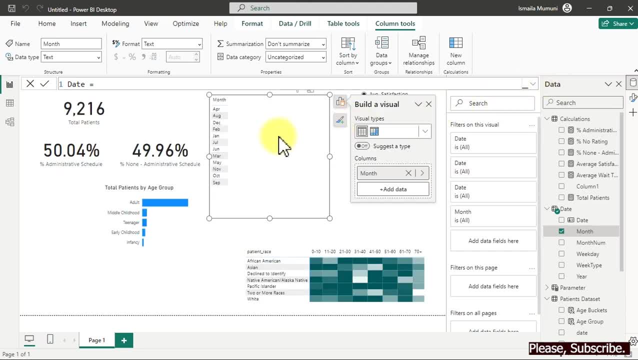 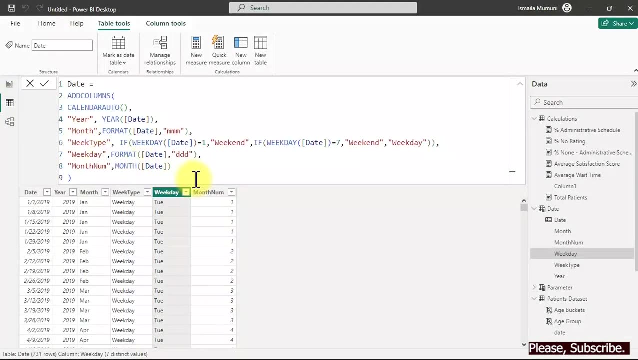 actually, you know, satisfy your curiosity in case you want to know what this is going to do. so click on the month and click on sort by column and go to month number here, and this will definitely start from january and it will stop at december. beautiful getting back here right now. 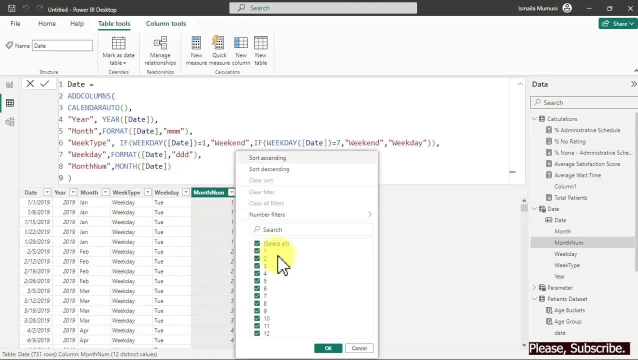 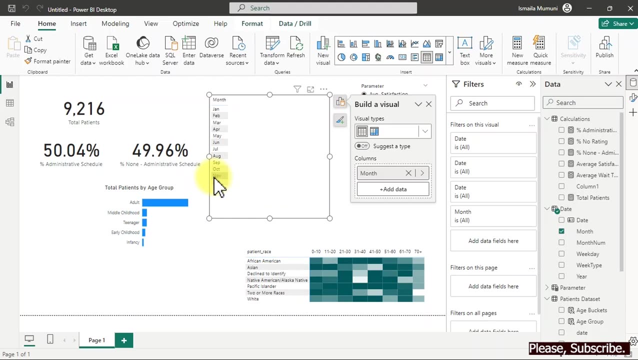 we have the month number we have added and we have 12, from january down to december. so we use this to sort this particular one. you get it, so let's get back. so we have gotten what we wanted to use, so the next thing now is to start creating exactly what we want. so 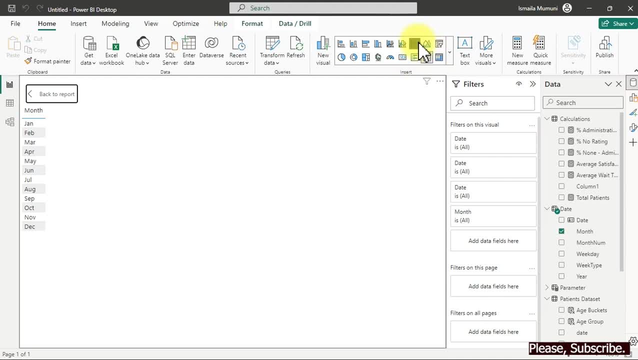 i'm gonna have to give you this view. then i'm gonna convert this into a line chat. converting this into a line chat, i'll bring in my total patients into it. this gives me patient trend every single month. so now it's fine, we can easily talk about the low west month. but can we some kind of want to be some kind of like. as soon as we see our chat, we will just put theminutewest station and oures coalition, and i will just envelope this to that code, هanton, and i am going to push filter, so, and that gives us the min, not. so we are going to put this trend down again. we cr onze, so you can. 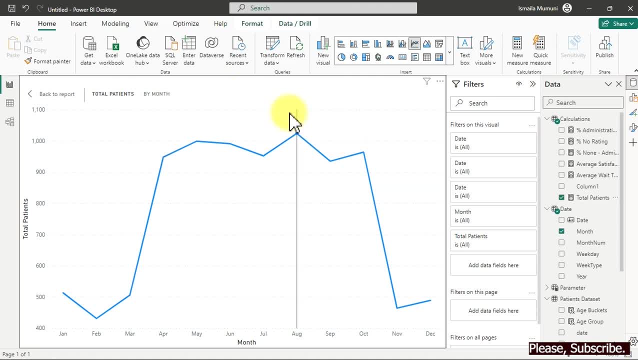 we see our chart, we want to tell where the max falls to now. if we have to tell where the max falls to now, we can be some kind of like: maybe here, maybe here. okay, maybe we might get it right here. so where does the mean fall to? is it on this one or on this low part here? so we want to avoid. 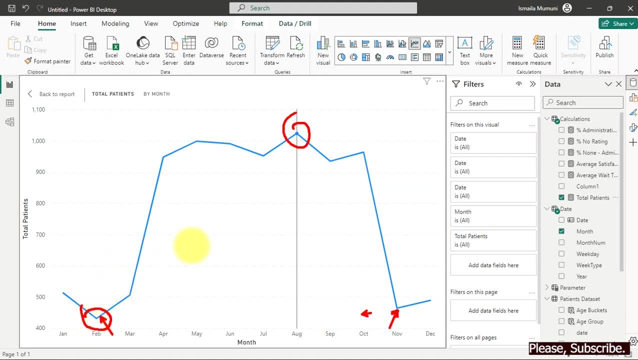 guessing we're going to actually mark this particular part as our mean. so this is going to be dynamic. when we play the filter, that filter will start shifting it to different months based on the availability of what of it. you get it now. let's do it. we don't have a default formatting. 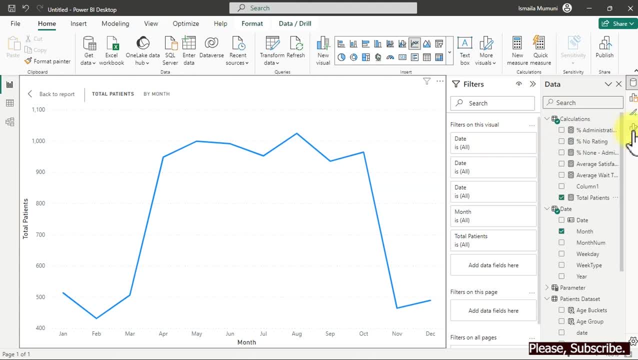 for that? what can we do? let's try it. come over to here so you will go to line. you have an online chat. we have markers for every part of it and our aim is to turn those markers for the max area here and the minimum area here, so which means 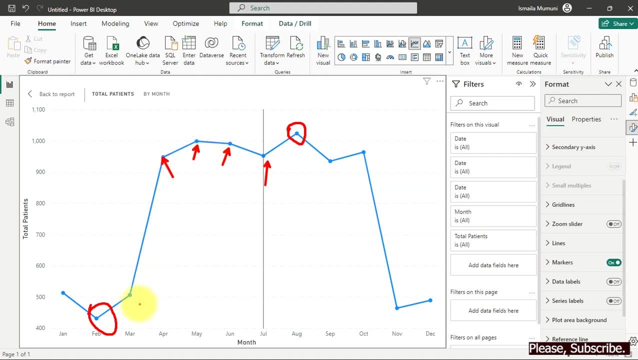 those ones are some kind of wrong. how do we fix them and make those want to disappear? we don't want to see them, we only want to see where we have circled, like this one and this very one here. to have that done, we have to create a custom measure for that, but it's very important to turn on this particular. 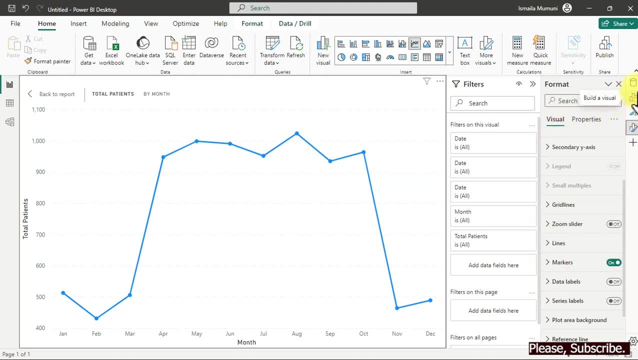 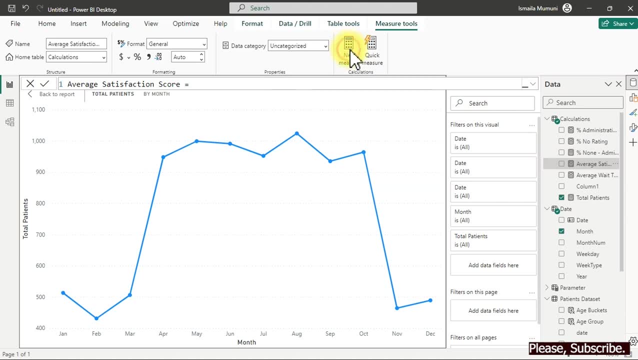 markers here. okay, to do that. now let's go over here. in the click in here, under calculations, add in your measure. so i'm going to show you every step of this measure, what it is that you should be expecting or what it will return. so inside this measure, i'm going to name it um, conditional formatting, c, f. so max point. 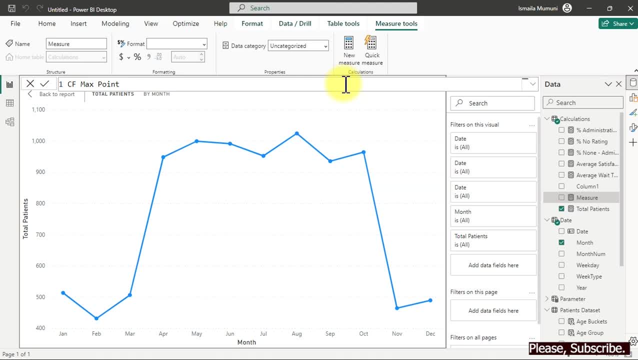 so equals. so i'm going to indicate it as month inside brackets. i'll type month, then close it. now my equals here. so, um, you might be tempted to use the maxx function to do this, which would definitely be okay, like if we try it. let's try that, because 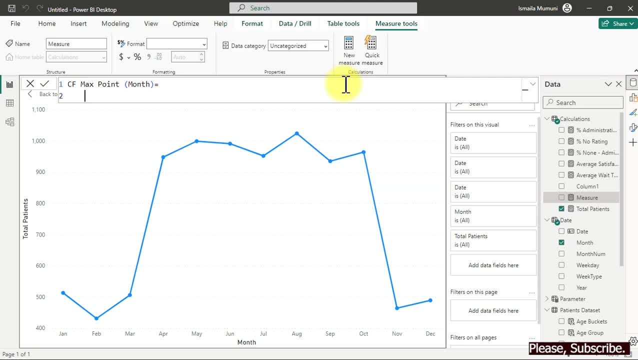 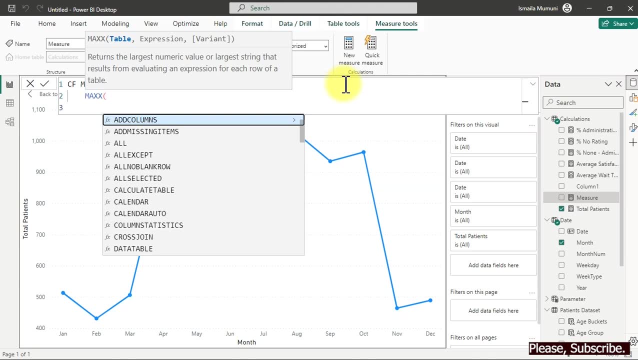 that is what everybody might be thinking of. so over here i'm going to actually use my max x here inside the maxx. the maxx is looking for what it's looking for: a table and that table. i want to remove filter from it because i want to have a straight line on this so you can use the all. 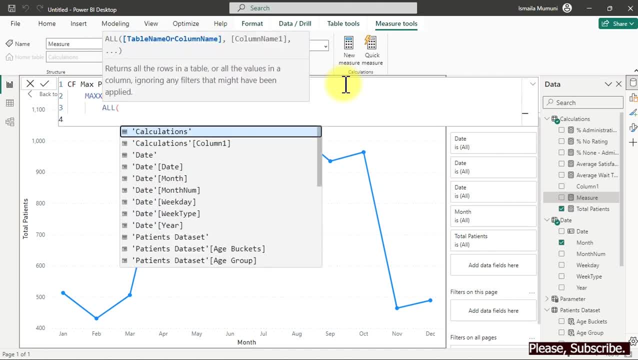 function inside the all function is looking for the table function, and then we can define the max x in the table function of the table function of the table, and then we can define the max x, for we are going to use the date, so using the date now. 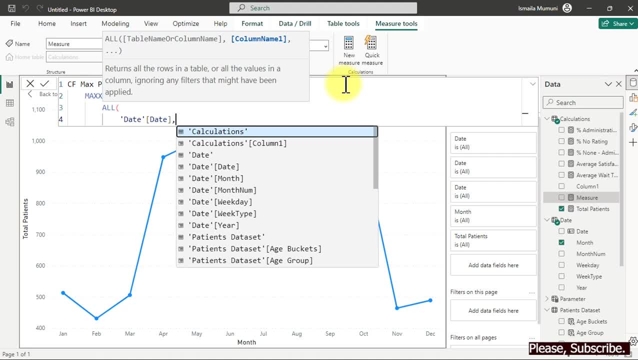 we have a comma here. this comma is asking us for a column, so the column now will be sorry. we are using just the date table. so with comma we use the column over here. the column will be our month dates and we use the month. so we close it. 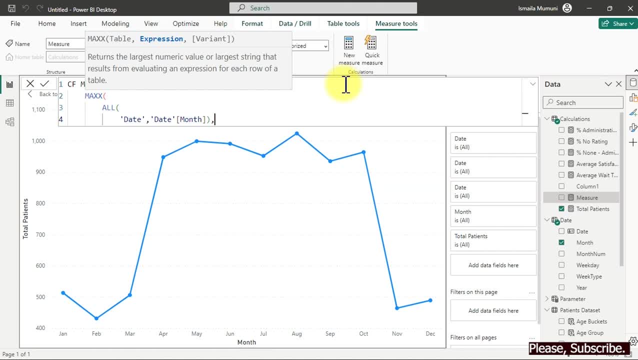 for comma. now our expression, our expression should now be the measure we are trying to use or we have used on our line chart that we are trying to find it marks. that would definitely be total patience here. then, once we close our marks and hit our enter key, 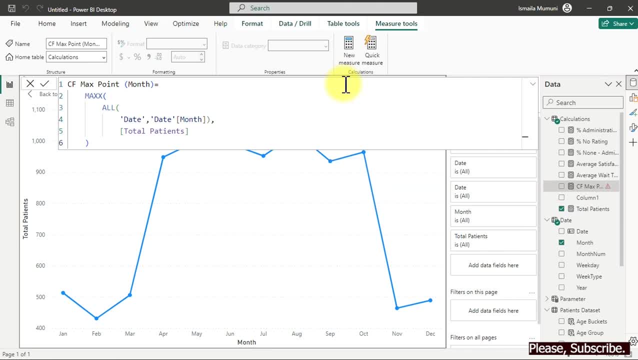 so we are expecting to see a straight line because first of all, ok, what do we have? we have. ok, let's remove this. I just have column there, then hit enter key. that should actually get this done for us. so we have cleared the error: no table, we just used the column. 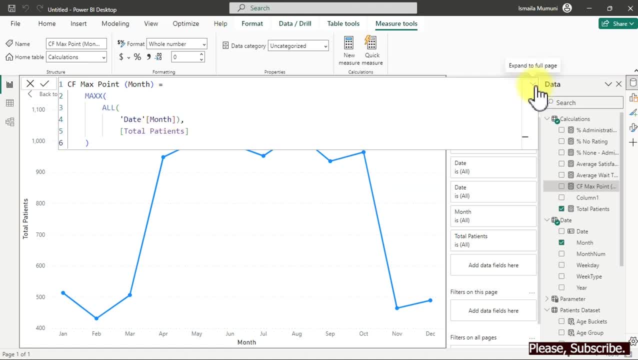 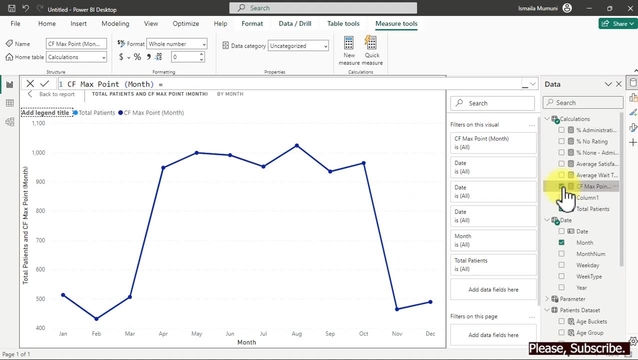 so we are expecting to see a straight line when we drop this into our line chart and we go ahead and bring this in. so it doesn't give us that. so when we hover over it, it's giving us cf, which is conditional formatting marks point. it's giving us the same value all through. 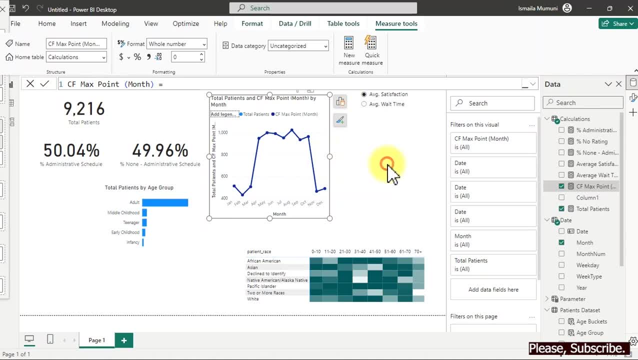 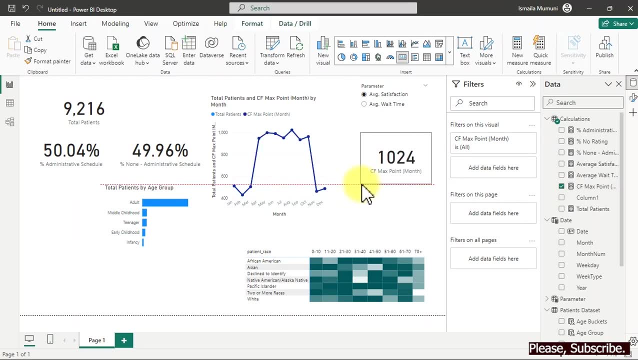 but let us verify something here. what if we bring this into a card? what is it giving us? it's giving us this value, so different from this value here, so different from this value here, so different from this value here. so what is actually going on if I hover over here? 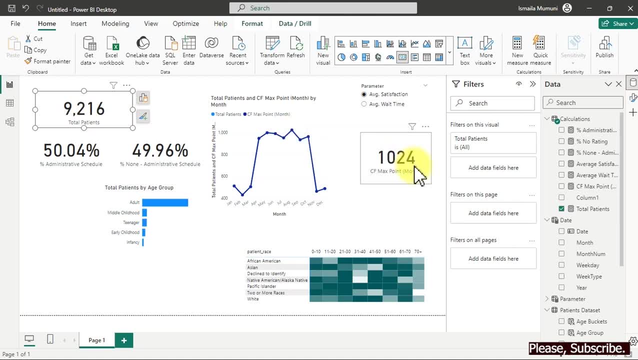 this is my marks point. it was able to drag in and bring in my marks point. look at it when I hover over it again. the marks point fall into August, but it's not giving us what we want, so, which means we cannot use this approach to do it. 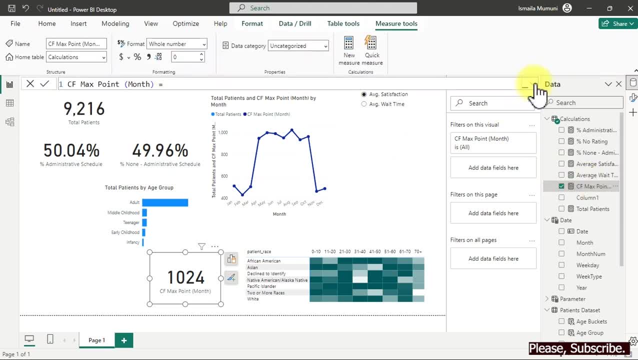 let us go ahead and do the rightful thing. so now I'm going to wipe off this, and we start off by creating a virtual table. and we start off by creating a virtual table. so to do that now we have to write a variable. so this variable we call it. 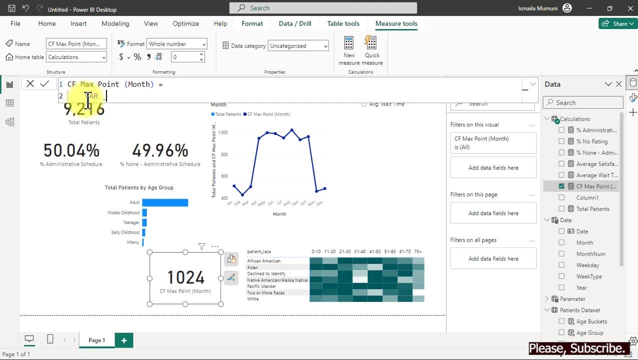 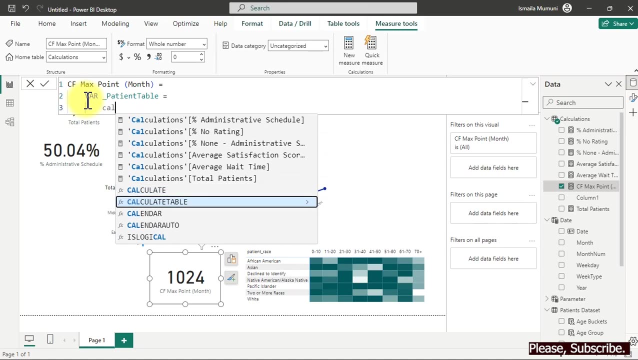 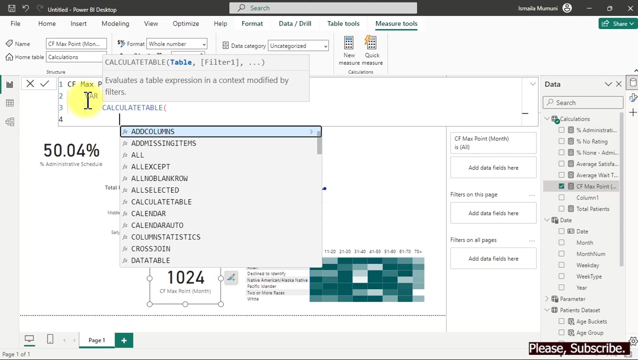 patient. we call it patient, patient table, patient table. so for our patient table, we're going to use our calculate table to create the table we are looking for and inside this table we want to actually have our month, so which would be summarize. so for the summarize, it's looking for a table. 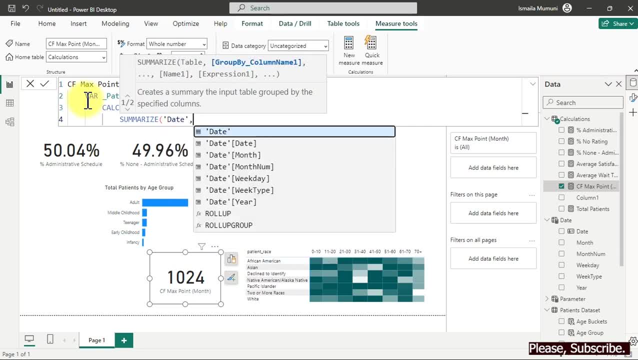 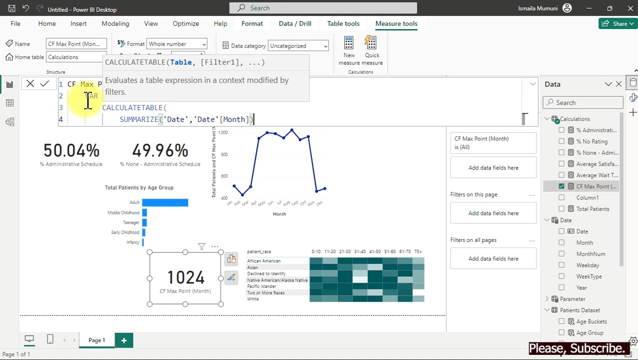 we have to give it date first, then comma. now we want to group this particular date by month, so we bring in our month here, then we can close this when we have closed this. this is okay, we want to group this by what. we want to group it by the. 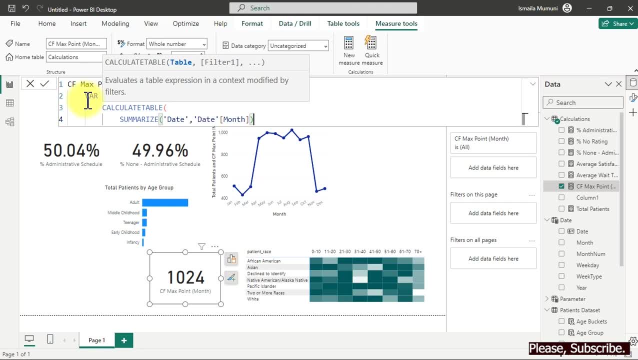 total visit or total patients that visited our hospital. so, which means we need to add another column to this, to add a new column. now we have to go above summarize here and we use a function called add columns. so with this function add columns, we come below here. 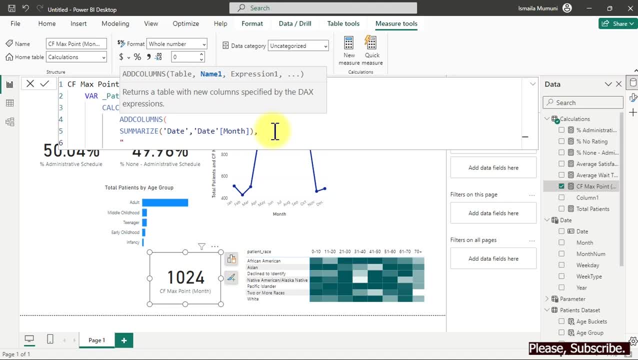 so we place a comma here and go here and we want to add a column. I'm going to just say add, to differentiate it from my other one. I'm going to say total patients. so you get it. then I'll do this: total patients. so if we have an issue, 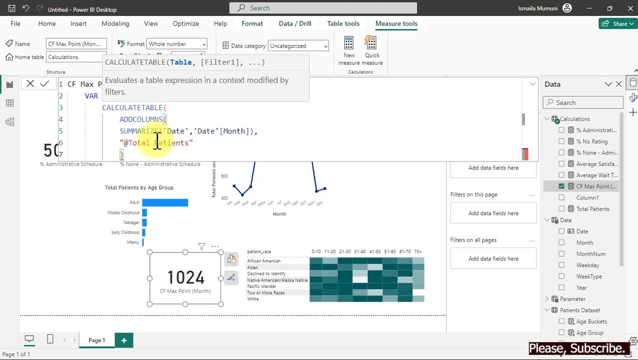 that issue should be. what should be our space. let's solve it. can you see, if I put in my space and I come down here, I have this underline on the bracket: I've closed. so by the time I go there and take off the space so I can use underscore. 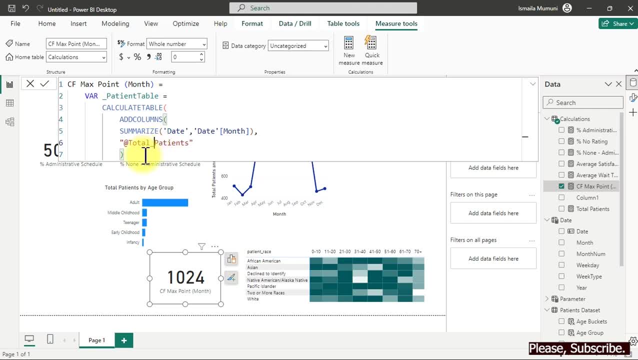 if I still want to have space for readability purpose, you have this. so now we still have that. what's wrong with it? let's remove it again. okay, that means we have something different wrong with this, let's see, let's see. okay, fine, that is good. so I'm going to actually have my 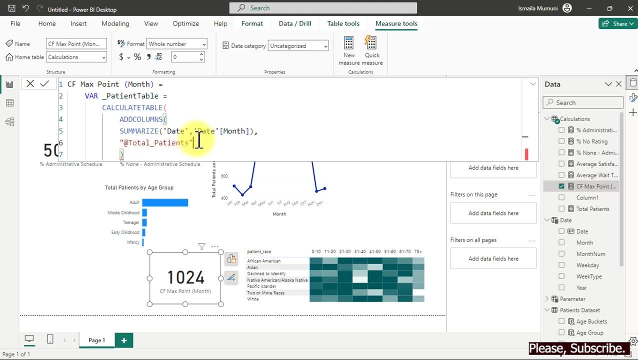 underscore here. I have forgotten to actually place a comma here, to actually give it an expression. an expression is a value and that value is going to be nothing but our total patients in here. so what have we done? this is actually a column on its own. we have thought in this column: 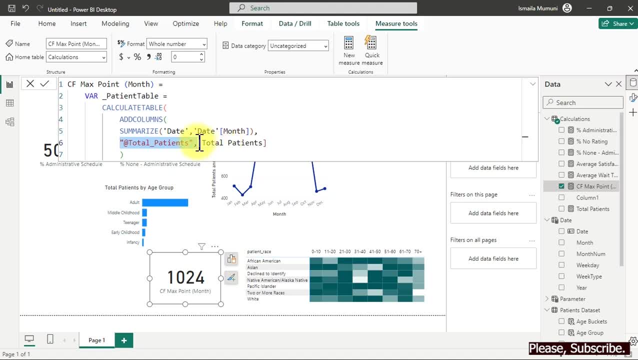 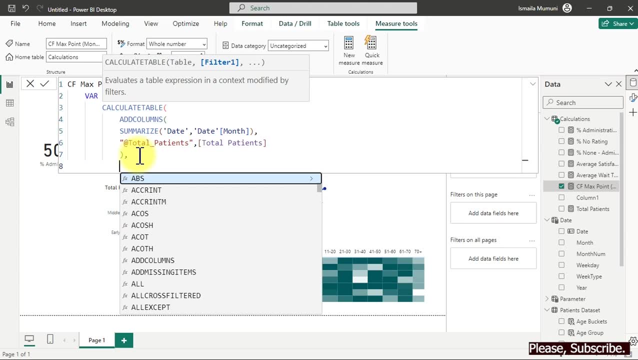 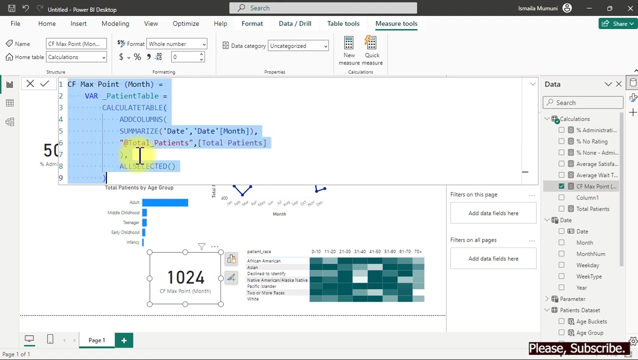 this particular patient, what patient or visit? so at the end of this we want to actually say: all selected right. so we're done for you to have the full understanding of what we have done here. I am going to just copy this particular part here. I'll copy it. 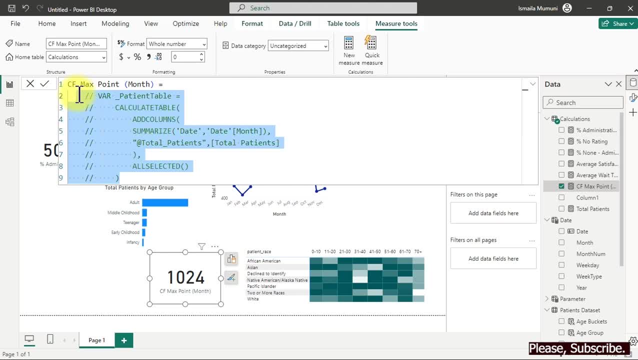 so once I've copied, I'll comment this one so that I will not have an error if I hit enter and step off from here. we don't have any error to do a multiple comment. you hit your control key and the slash on your keyboard- that where you have the question mark. 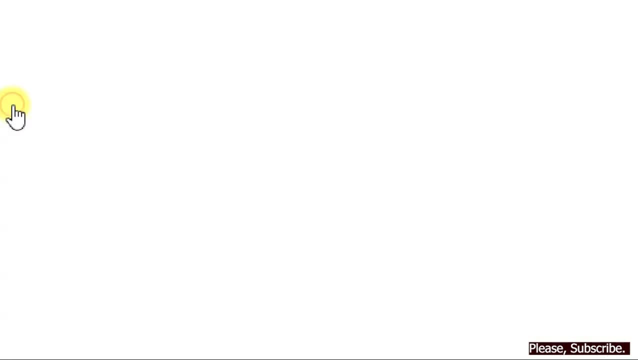 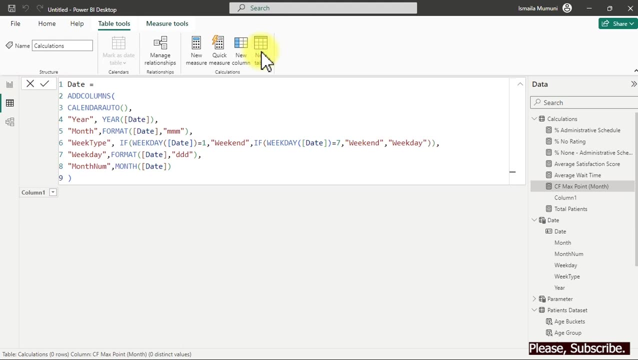 right then, that is all. let's get back here. now. we create a new table, so inside this new table, I will go ahead and paste in the DAX code we have written here. so we it's in a variable, we need to return it. so what do we return? 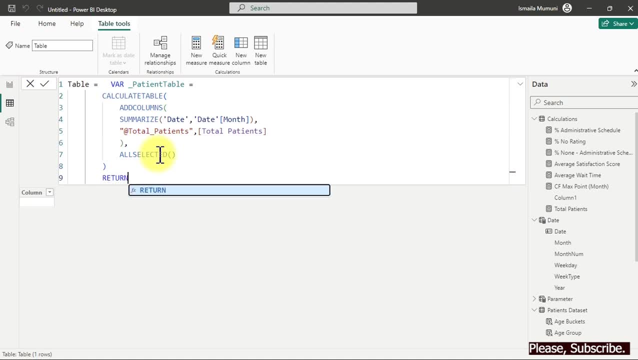 we return underscore, so we return what return underscore- patient table. and if I hit my enter, it should create a table for me with two columns. this is what we have. so we have summarized, we have brought in our month, which is using the summarize here. that is the first. 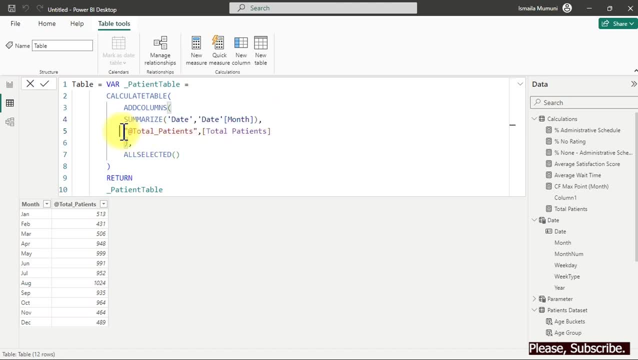 column we added then the second column is this particular one over here that populated this particular number, as you can see, at total patients. so this is what we are going to use to actually identify the marks and the main point let's get back to here and now. 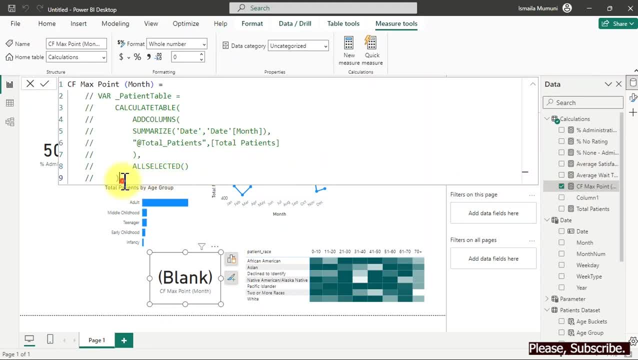 we have to click on the conditional formatting. so the next thing we have to do now is go in here control, then we hit the slash key. so you see on your keyboard, when you have to click on the control and a key that goes this way, not the one that 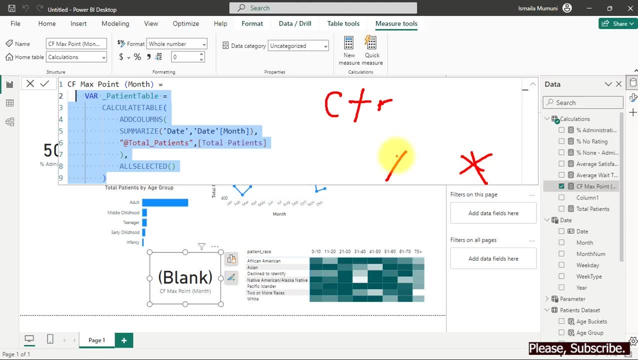 goes this way: no, not this one, but this one, right? so once we have this done, now we're going to actually add some other conditions here to actually set exactly what we want. so we create a new variable inside this variable. I'm going to call it underscore. 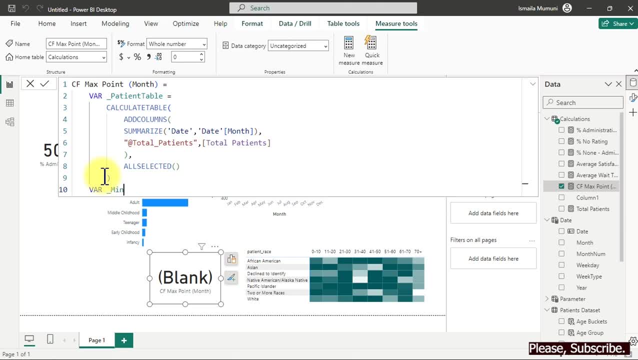 mean mean, what mean value. so it will be equals to what to mean x. the mean x is going to actually say: okay, my table which returns the month and the values. we've just seen the physical table here, so we want to find the mean inside this particular column. 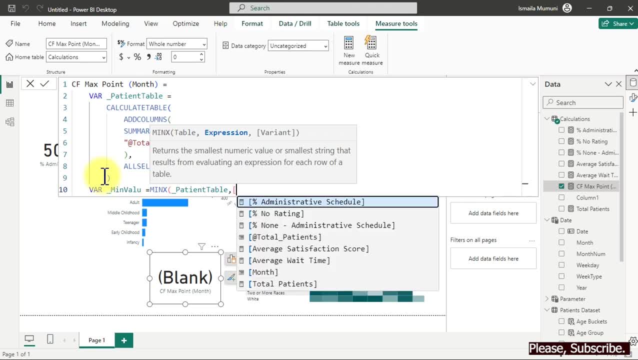 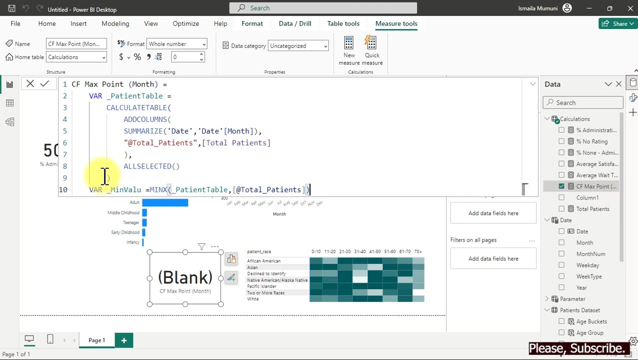 that is going to be the column with the at this one here. that at is not really important. we just put it there to be able to identify our new create head column. so we close it right, so we create another variable, so this variable will be underscore max. 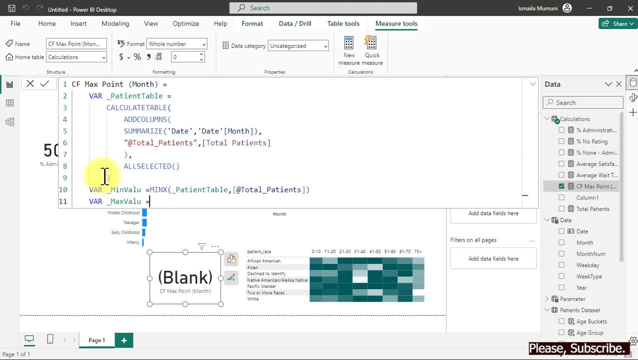 value for the max value. here we're going to use max x. so with the max x we actually call the table name again. so with comma we bring in our total patients. we close it. so individually. let us look at what it would return if I return this. 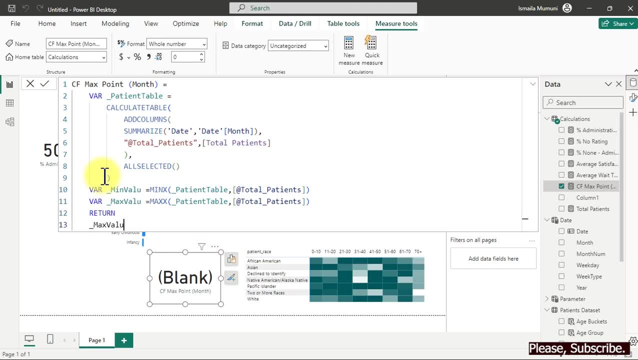 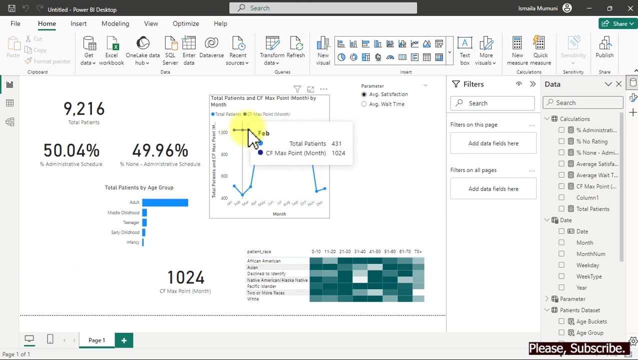 underscore max value here. what should we expect? we should expect that first value we had when we did that particular- I'm talking about this one here. then let's go ahead and verify. can you see it now? can you see, because we have it over here. it's now marking. 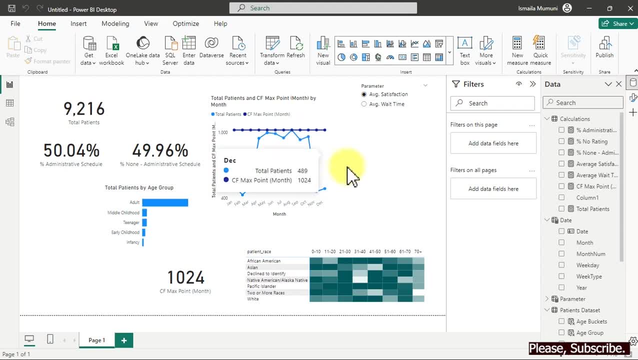 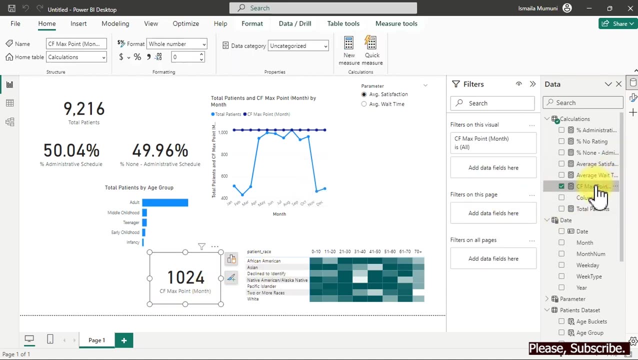 it for us. but this is not what we want. we want to. we want something a bit different than this. so we have the max point here now. so what about the min point? let's try the min point. so I'll go over to this. I'll return. 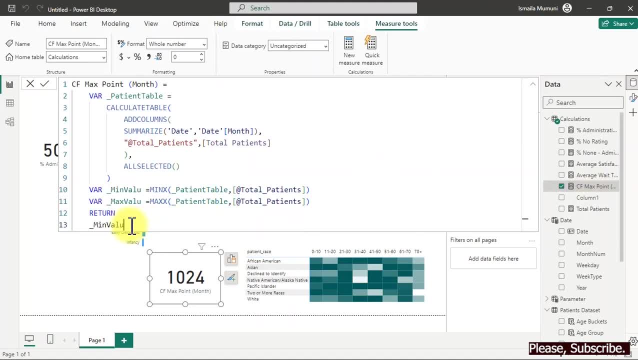 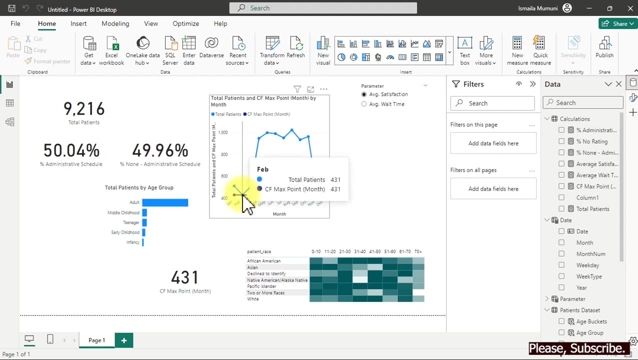 the min point for you to see what the min point will give us. the min point, so the min point will definitely give us this and that particular lines move down to this and this is our main point. four, three, one, do you see this now beautiful? okay, let's. 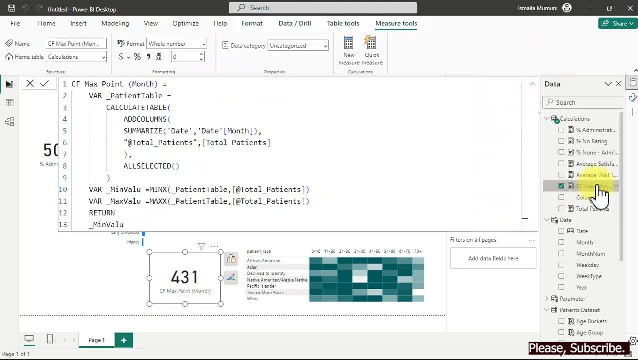 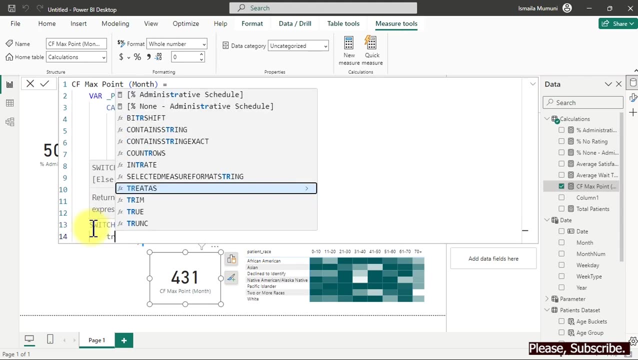 spice, see this up a little bit. so we come under the return here. instead of first returning this, we are going to do switch, and you see, true, only true comma. to switch this now, what we want is actually like: okay, you know what if underscore? oh sorry, we have one more. 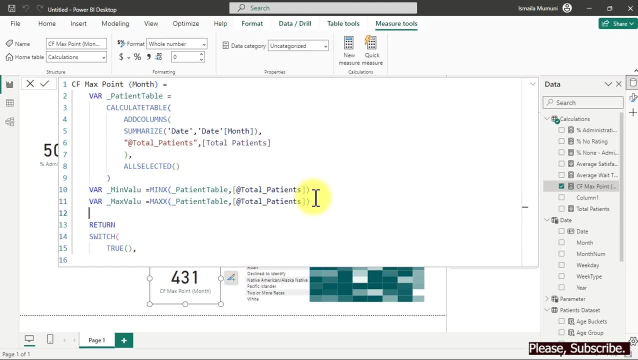 variable to create. that variable will be our total. that is going to be variable underscore, total patience. so which is going to store in our main measure called total patience here, then this total patience would be used to compare, like compare the min and the max. so only when. 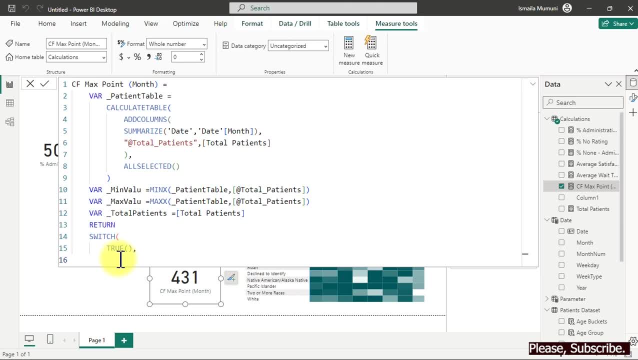 the min and the max is equal to a particular value we have in the total patience measure that it would return something. otherwise we don't want to return anything. so we're going to say: underscore total patience is equals to what? to min value here. min value, I think our value. 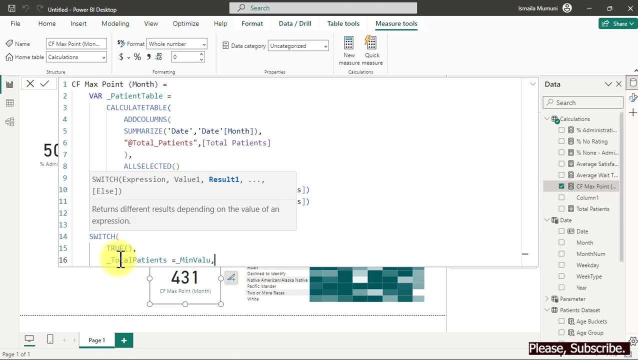 should have. e sorry for that. so min value here. so what we want to return? we want to return one, or first of all we want to return that particular min comma. so underscore total patience here is equals to what to underscore max value. then if that is true, 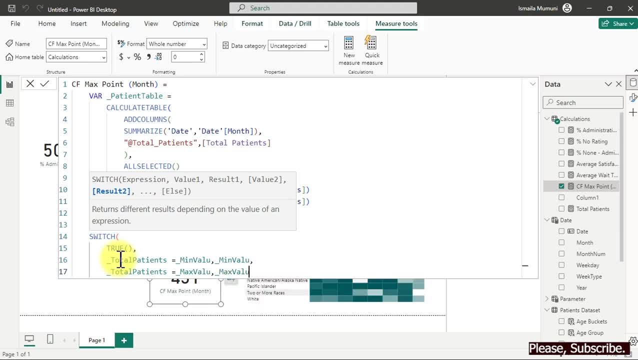 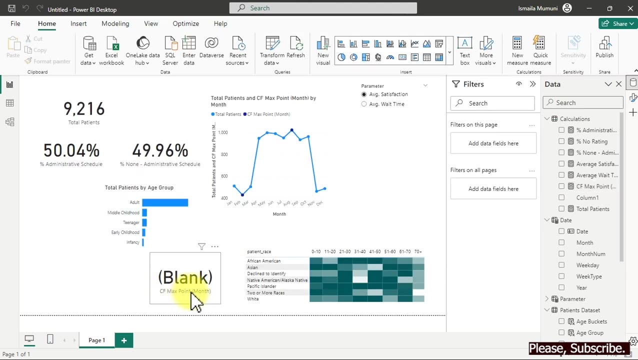 return the max value to us max value. so we go ahead and close our switch function, switch function and let's see what we have. so this is returning blank and it has worked here. it has worked here. so what happens if I go over here now? so let 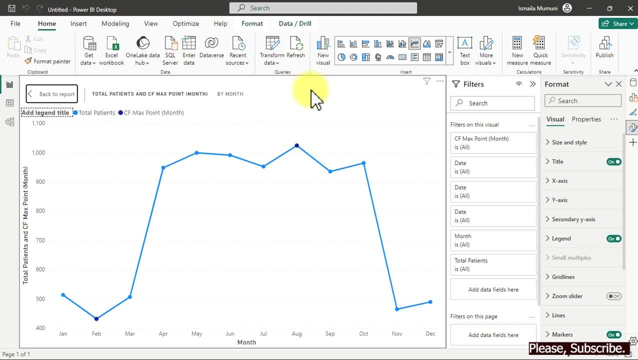 me just put it on the focus mode. so now we have marked here with a different color, a different color, so let's see if I go ahead and turn off this. can you see it? now that has given us this particular highlight beautiful. so with this, now just go ahead. 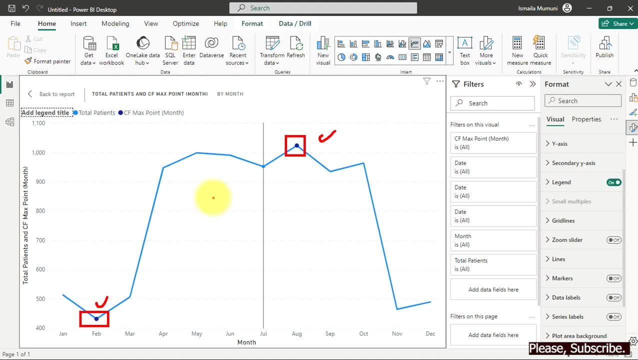 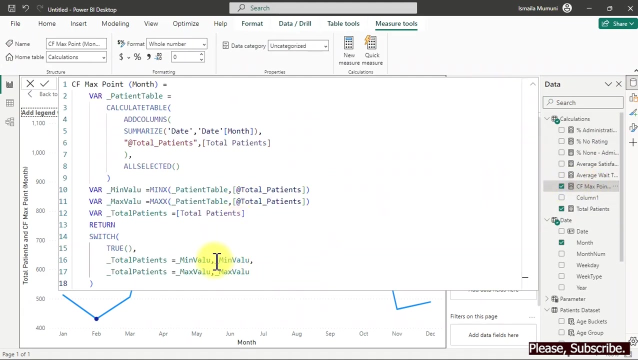 and hit the like button. share this. we want to actually have a color here. so for the max value, we want to have like a green color that signifies high point and a red color that signifies low point. what do we do? how do we do this? because what we 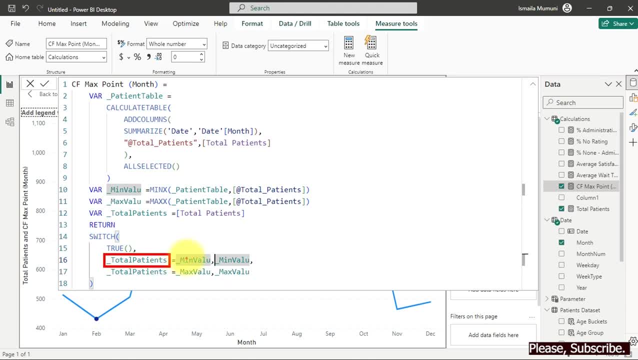 said here is if this particular total patience has value that is equal to remember, this one is returning one single value. so this particular one single value, it has here a particular number that is here in the max, is found here anywhere, is found in the month we want. 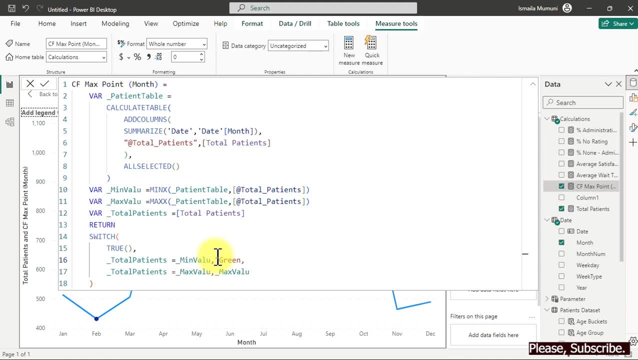 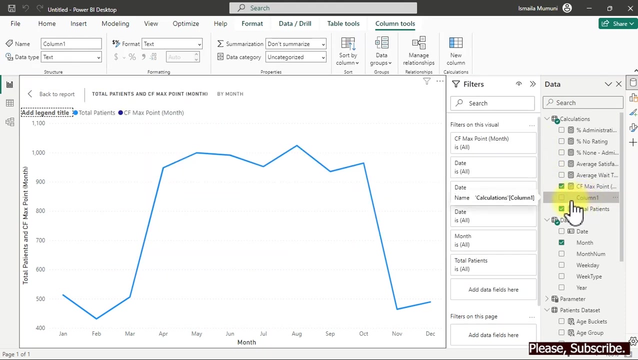 to give a color, so let's do that. so what if i use something like in the? in double quotes i'll use green. okay, my red should be just one e. so let us hit the enter key and see what this would look like. now, that doesn't. 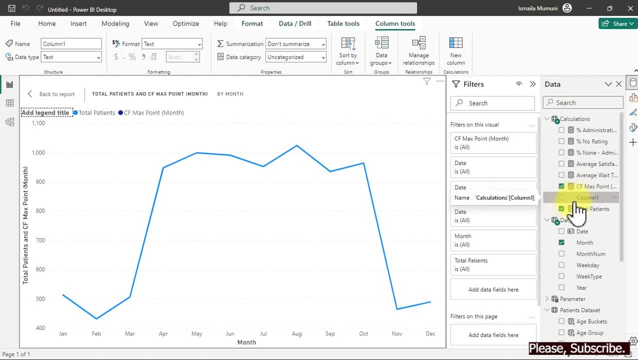 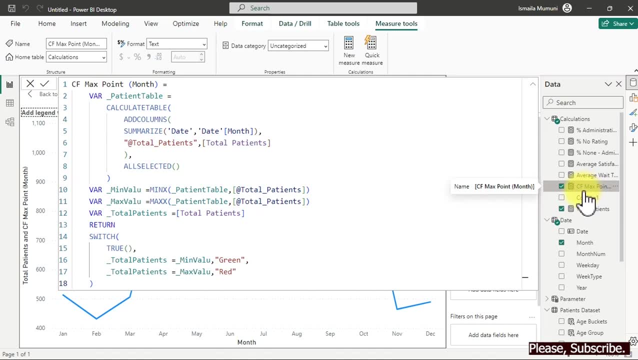 work. instead, it moves it off and our aim is to actually create this and make use of it. if it is mean, we want to display zero here, so power bi understands number, we just put here zero. otherwise, if it is max, we want to display what we want. 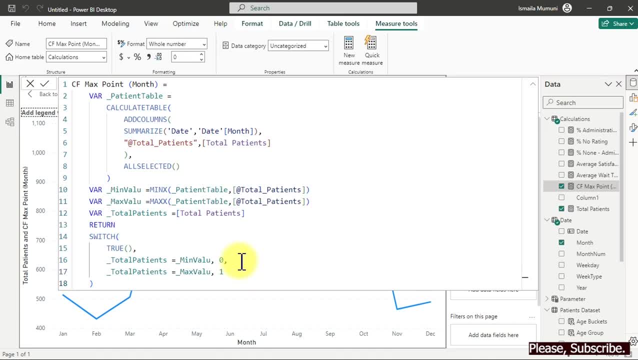 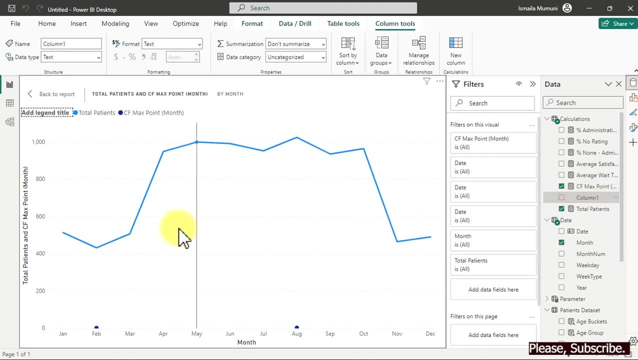 to display one. we just move this off. it's making our chart look a bit ugly now can you see? they both fall under here and here. we don't want this. for the time being. let us leave it the way it is right. now we're going to. 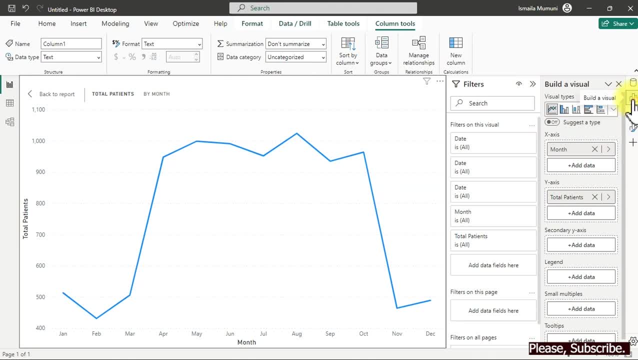 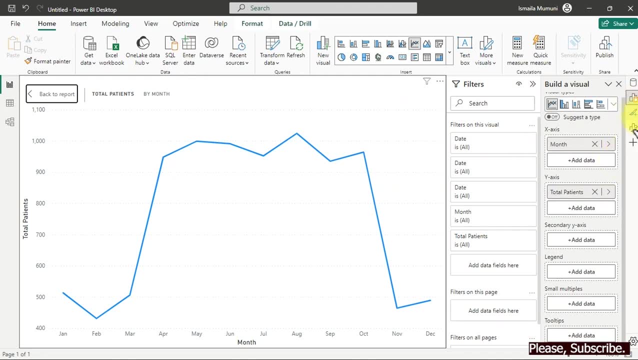 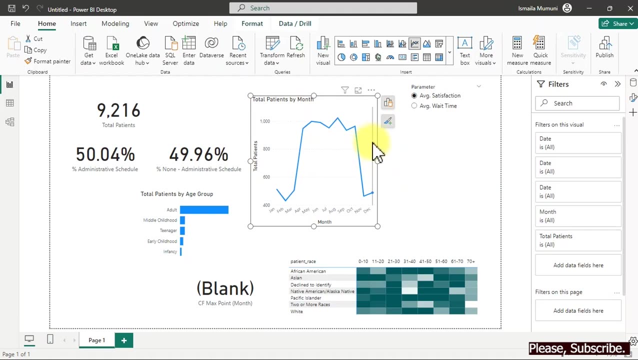 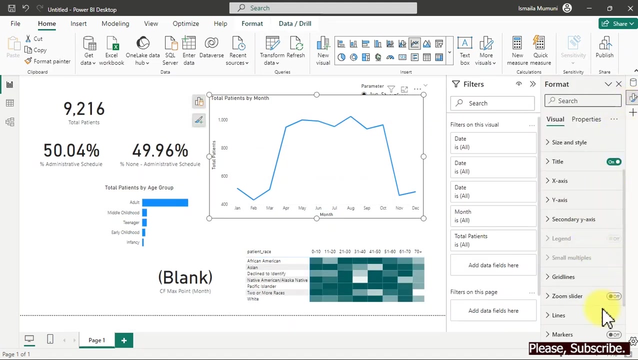 go ahead and come over to here. make sure you're still clicking on this. so under the formatting here we go for. so under the formatting here we want to actually make sure we mark the point. so that is going to be under markers. we bring this up, so we convert. 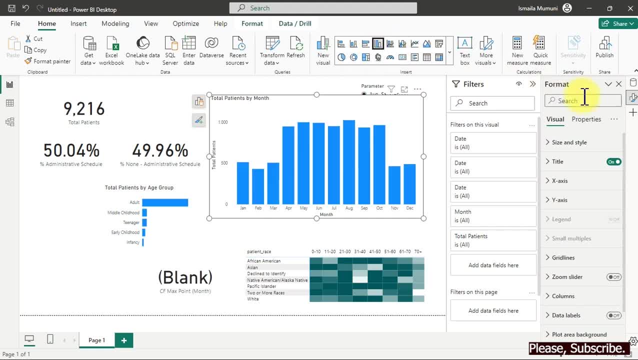 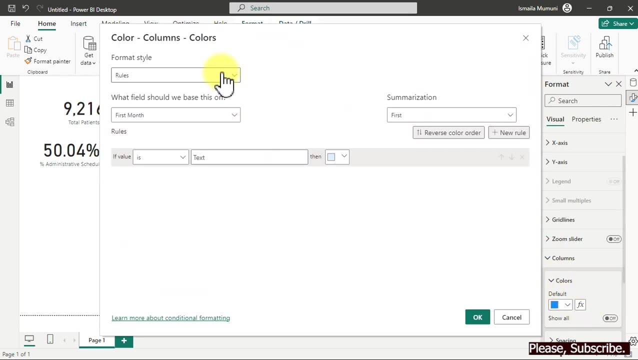 it to what convert from here. we now go down straight up. we go to this particular column here, then we click on the fx. so when we click on the fx, we use the rule to do this. so we come over here to select the measure under calculations we use. 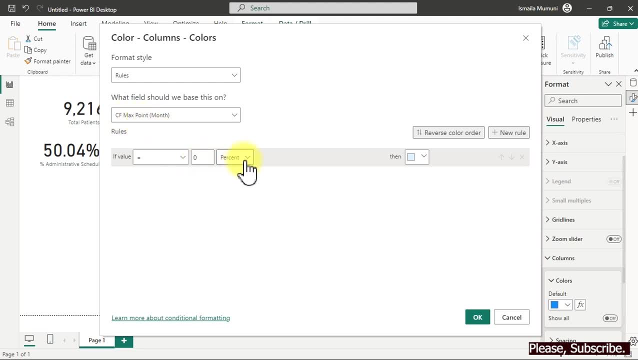 this particular one here is equals to zero. we change this one to number, then what we want to display is red. then we add a new rule: if it is equals to one, what we want to display- change this one to number- is actually a green color. there is. 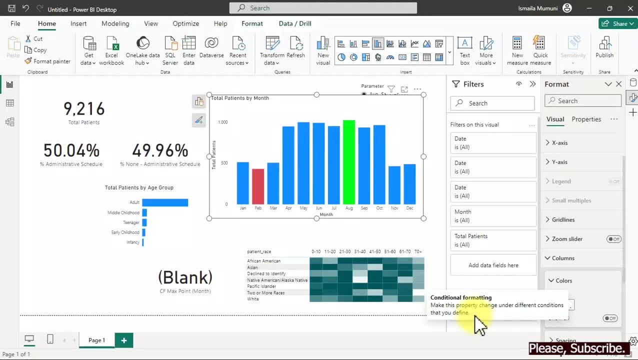 no green color. now we can see this. now this is what you have. so it has actually marked this as the highest and this here as the minimum for us. so this actually switch when i now add dot child hold. can you see this? so you can see it's. 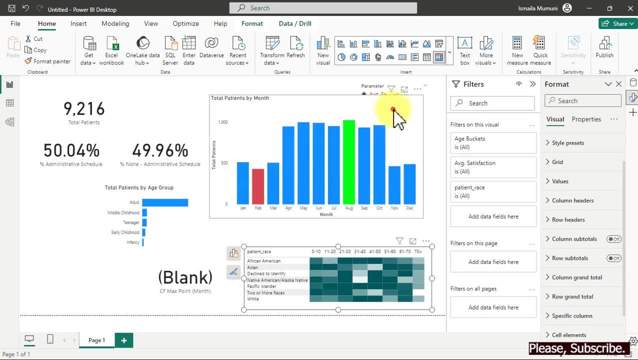 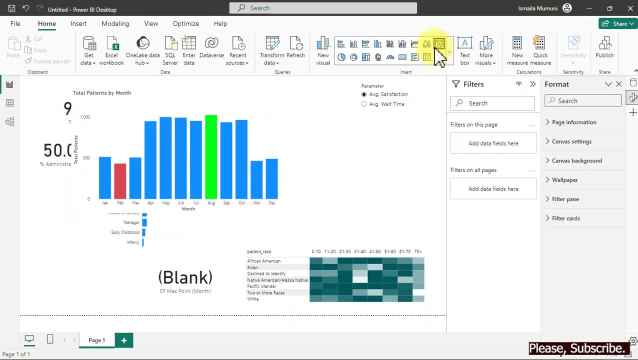 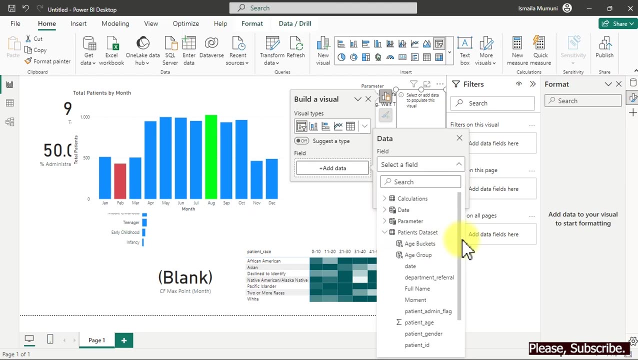 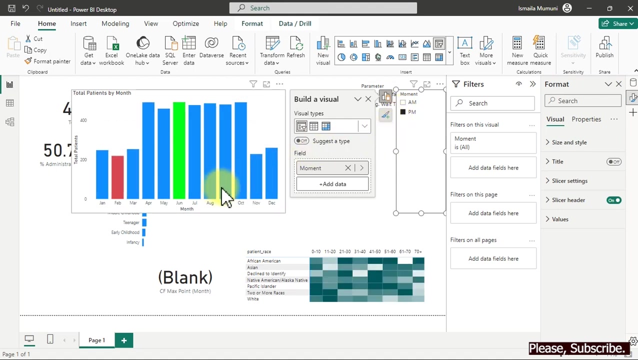 dynamic. all right with this. now what if, for example, i bring in a filter here, this filter is going to take in the moment we created inside inside power query: am my max switches, from where it is to june if i go to am now it's in may if i select it. 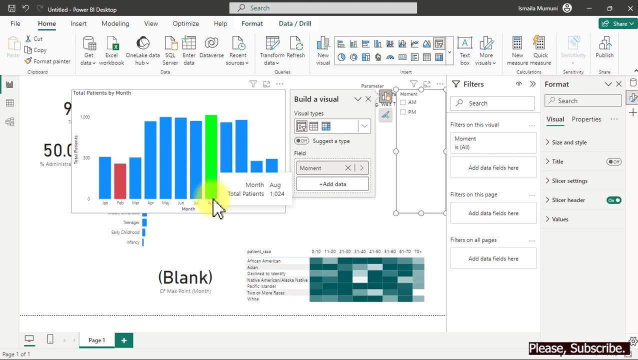 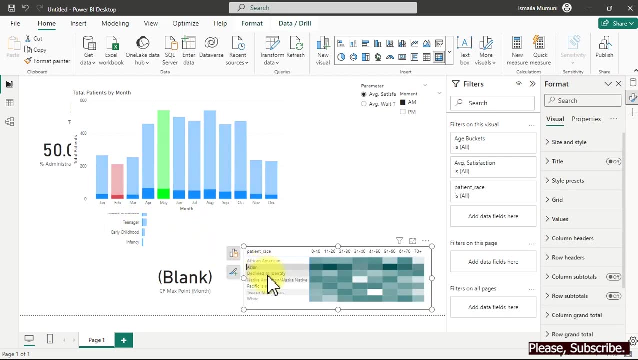 it's going to be back to august, which makes it movable. it's moving according to where it sports the maximum and the minimum. it responds to your slicer, as i've said earlier. so we are on am, so you want to see based on this issue. so now, very dynamic. so how do we have it as a line chat? just, 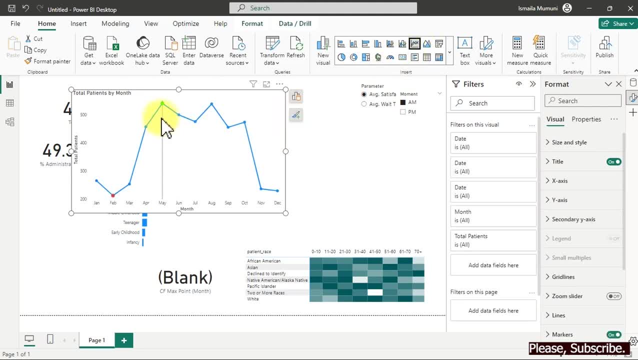 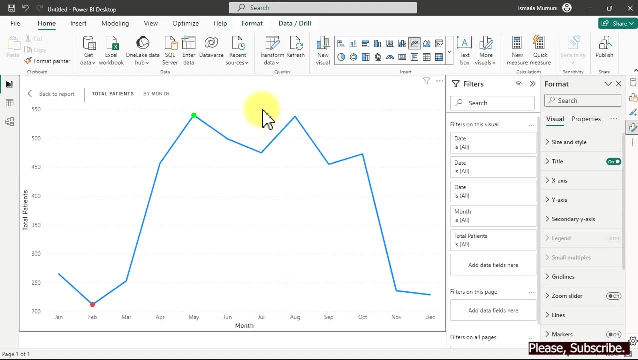 go ahead and click on your line chat. it's up, it marks it for you. then we can now come to the marker here and turn off this marker. so what do you see? so i want to use this chat. i click on this chat. you can still have it. can you see it now? your marks. 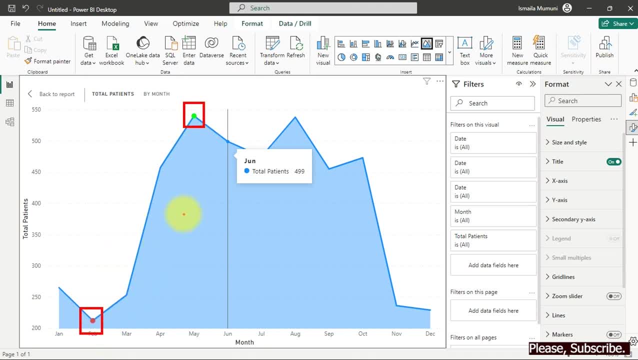 you can see it now and your mean it's been marked. so all right. the next thing now is that i want to show the value that is peculiar to my max and my mean on top of them. how do i do it? very simple, let's actually give a line chat first. 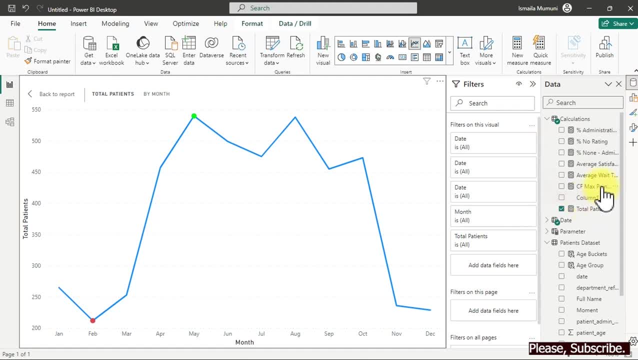 we have this. okay, we come here and we click on the conditional form. i'm going to show you how to do it. so i'm going to show you how to do it. so i'm going to show you how to do it. so we're going to show you how to do it, so i'm going to explain it to you. 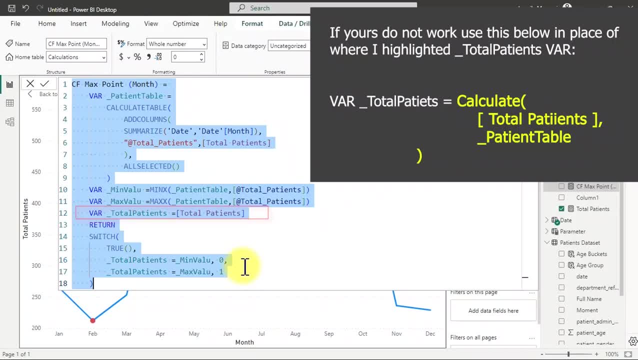 so i'm going to start off with a value, and then we're taking our value and then we're going to apply the conditional formatin here. we have to go ahead and copy this, so create a new measure. we just make three changes, just three changes. we paste it in. the first change is the first among the three changes. here is: 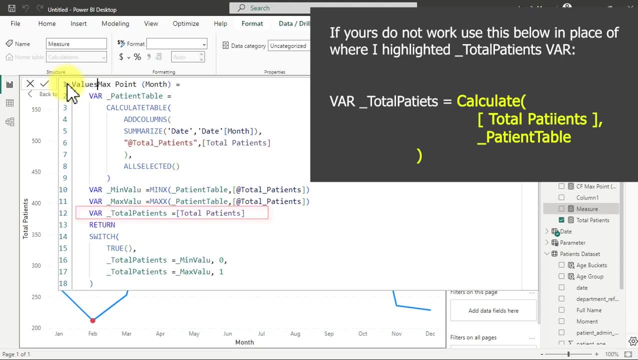 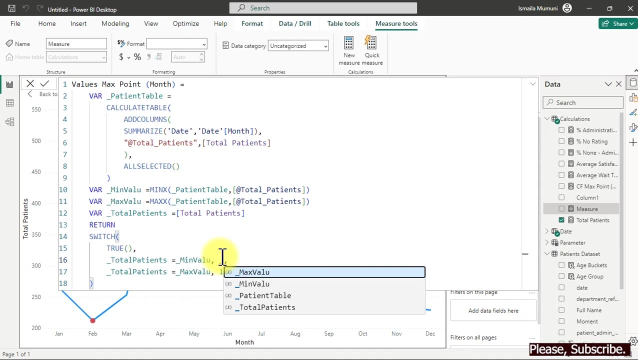 not more conditional formatting. this will be value, values, max point. the second one is value and the previous one is value. Second one here is to return underscore mean Yes, I return underscore mean If I return underscore mean this wouldn't do it, It will only return the max for me. 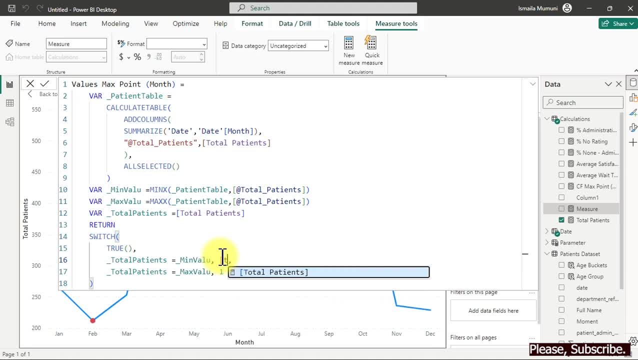 And I want to return what. I want to return my measure. It's going to be total patients Here. return what, Return the total patient as well. So return the total patients. So I'm going to hit my enter key for now. 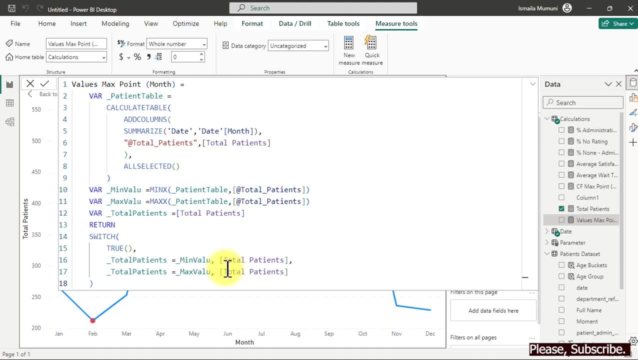 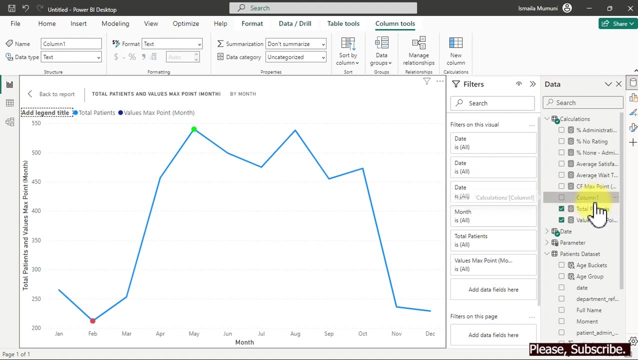 So how do we actually display this? Should I just move it in? Does it work? I guess no, It doesn't. So we need to find a way to bring this in. We find a way to bring it in, So let's remember. 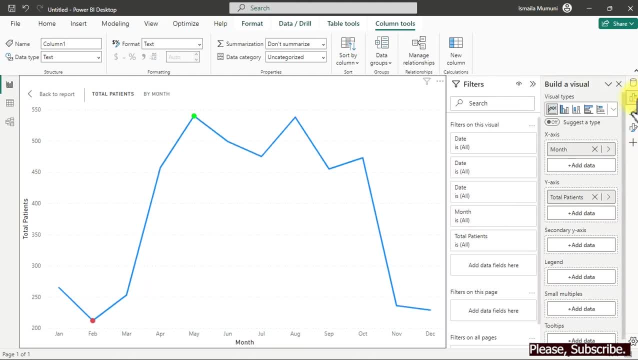 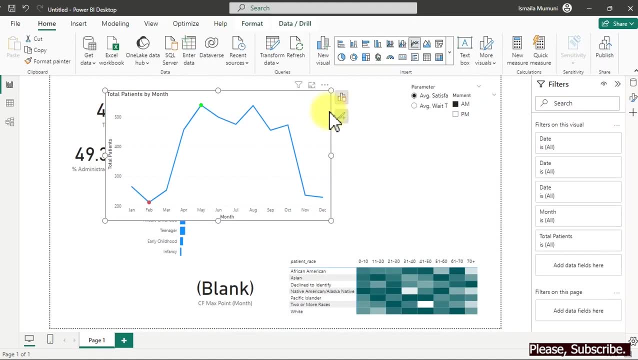 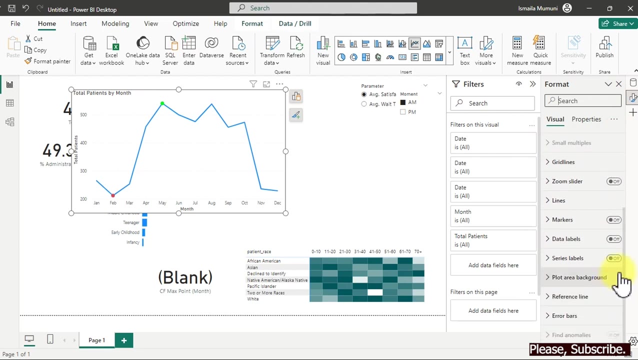 I'll click here. Click on our chart. Let's click here. Now let's go to detailleable. I'll turn on detailleable over here. I'll open it up. If I open it up, my detailleable has just this. 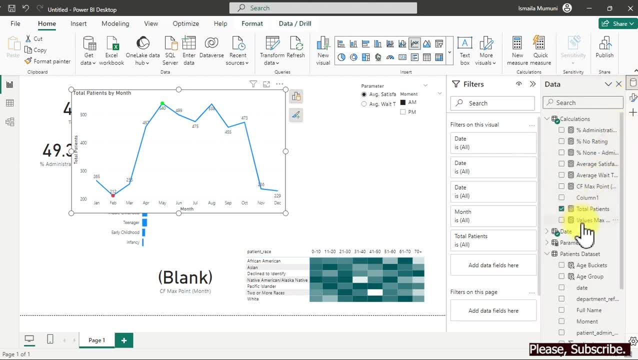 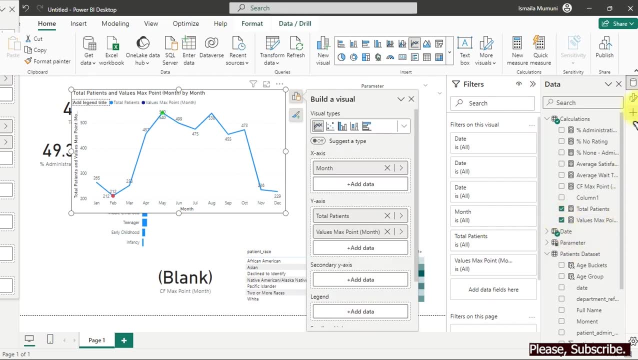 It's giving me all. So I'll now go here and bring in my value max point here. So if you look at it now, we have gotten it. So we now go back here. now, Under the detailleable, we go ahead and choose this particular total patient here. 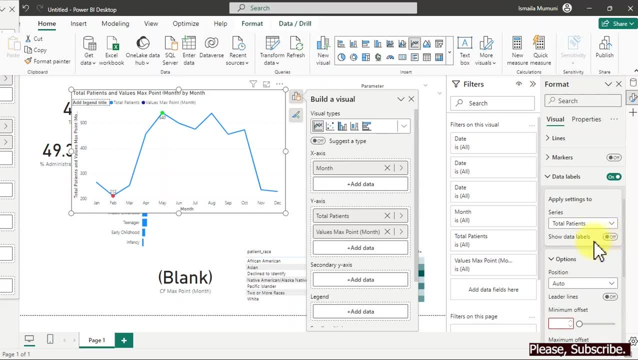 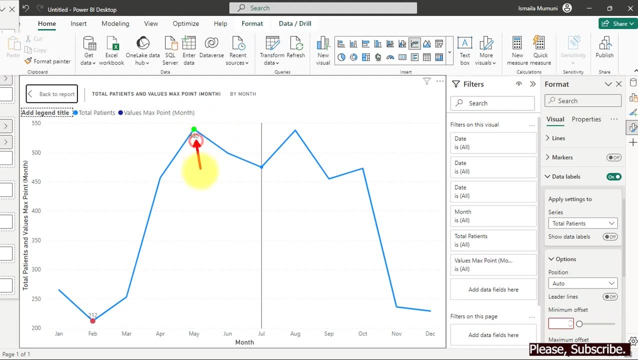 Then we turn it off. The magic has happened, Can you see it? So we now have The value that is peculiar to max and to what to mean. What we need to do now is that the one downside is we can some kind of format it nicely, the way I want it. 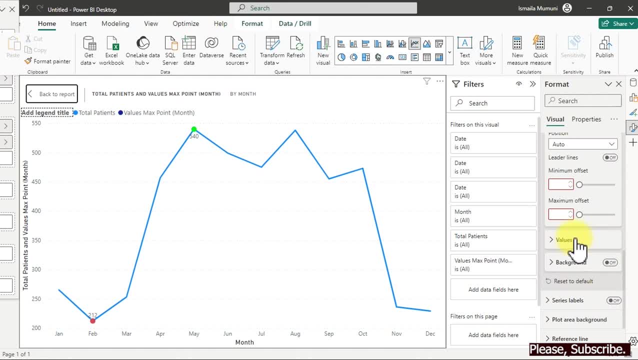 So I can just go ahead and move down to value. So I'll go to what to auto, I'll click none. If it is in Tarzan, I want to show it in Tarzan. I don't want it to have K or whatever it is. 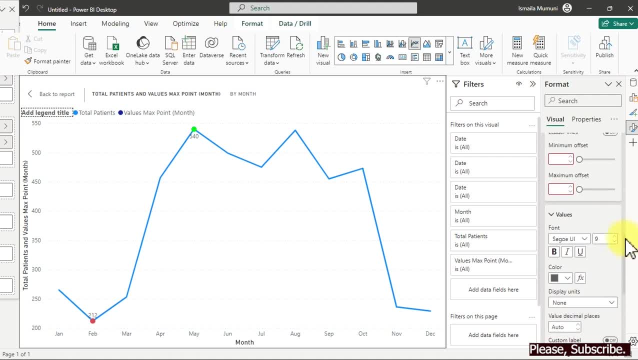 So if I actually want to change the color, I will. So if I put it on bold or I decide to crank it up to look more, much more- you know bold it doesn't really reflect on it, So I'm going to leave that one like that. 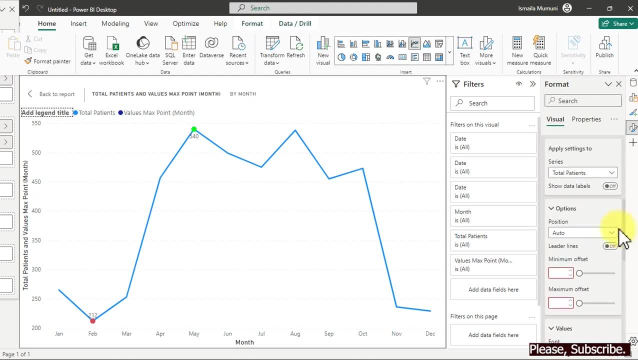 It's OK. So now, where do I display this? at the position. I'm going to put the position at the above. It doesn't actually respect that, No problem. So position no Doesn't work, So don't worry about that. 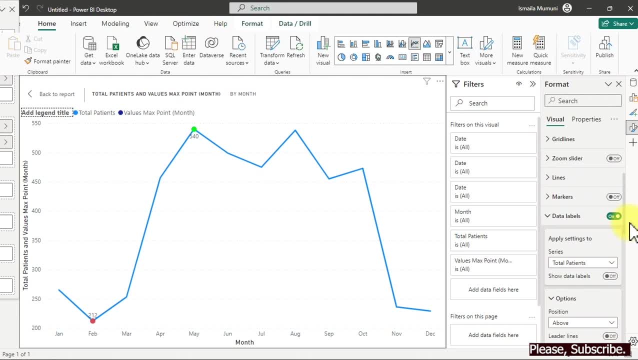 So we've just achieved this, And what is next for us now is that for our line chart, we go to line chart. So here is our line chart here. So we actually moved down a little bit. For line chart, we have line type. 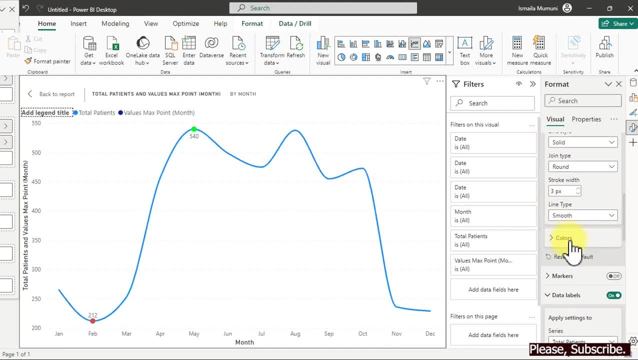 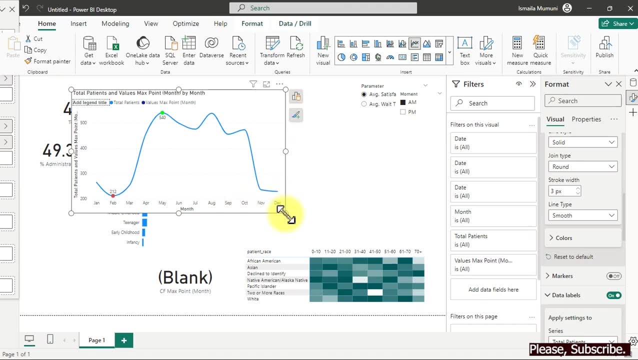 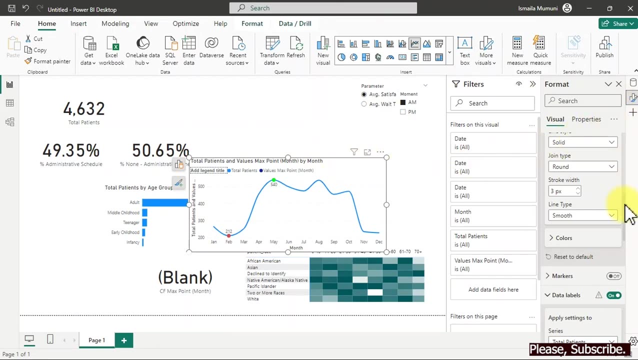 Want to use a smooth line That makes it much more looking good. All right, We have just created this and it's looking nice, So all I have to do is to update my title. Come here And for my title, two-top patients is what I'm going to have. 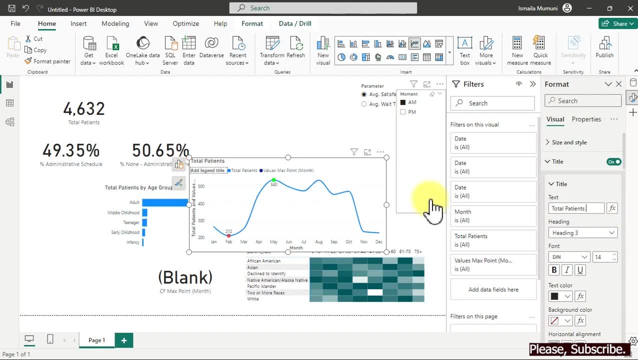 You can type in two-top visit, So I'm going to do two-top patient visit. So now the next thing to do is For the legend we have, we don't need to keep the legend, We turn off the legend. So we have to actually format our line chart. 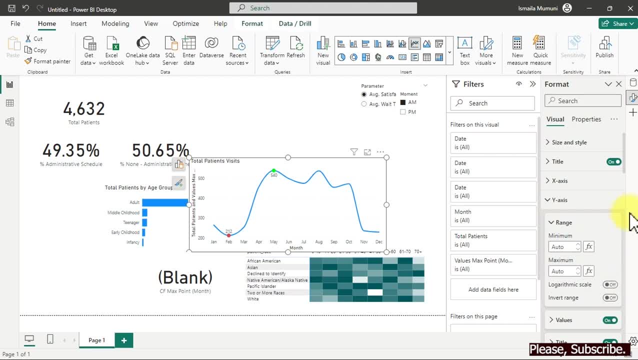 So we go for the Y axis here quickly. For the Y axis, what we have to do is to turn off the title, Then turn off the what, Turn off the value from it. Then for the X axis, what we're going to do right now for the X axis: 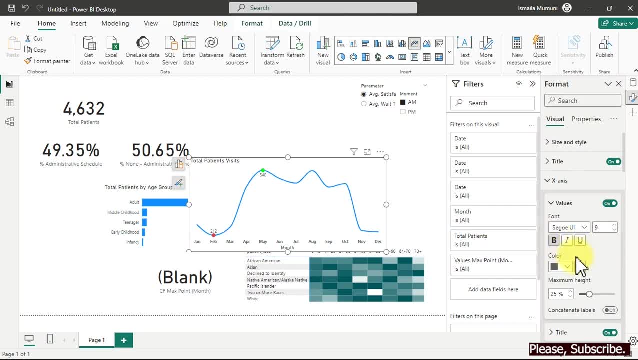 we want to make it bold. We want the month to pop out. Then we turn off the title For the month axis, So we have something like this: Can you look at that? So we don't have to keep this any longer. 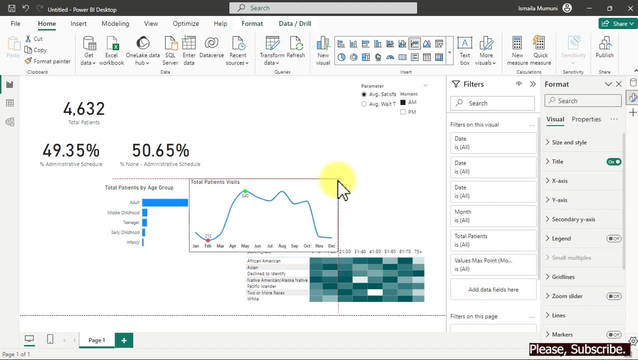 So we've just done this and it's beautiful on this, So I can just make it a bit smaller And push it over to this particular angle for the time being. So what about this? This calls for celebration, right, And the celebration is you hitting the like button. 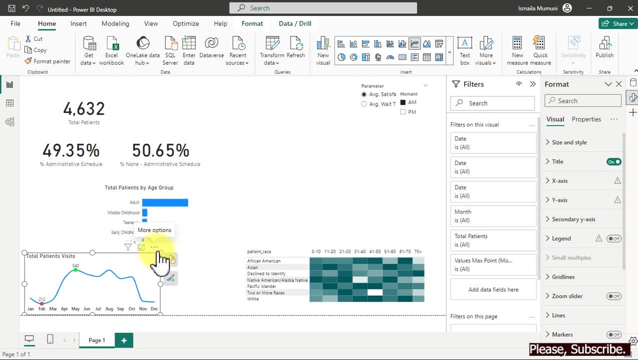 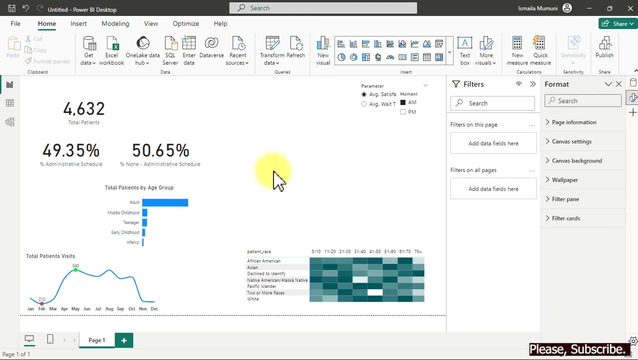 If you can do it a million times, I would have been happy, But just leave a comment. Let me know what you actually feel about this. All right, So I want to actually show the year, So all I'm going to do now is to actually just go over here. 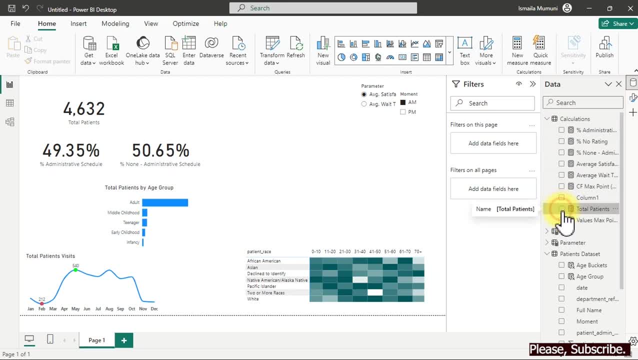 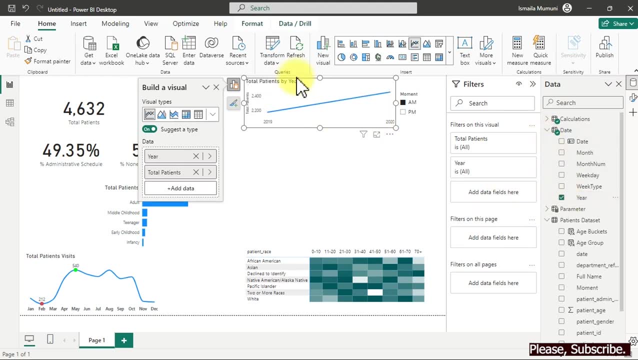 And I will get my total patience, So I'll go over to date. I'll bring it in which is my year, So my year will do this. So if it is important for you to actually still do the same thing, I've done. 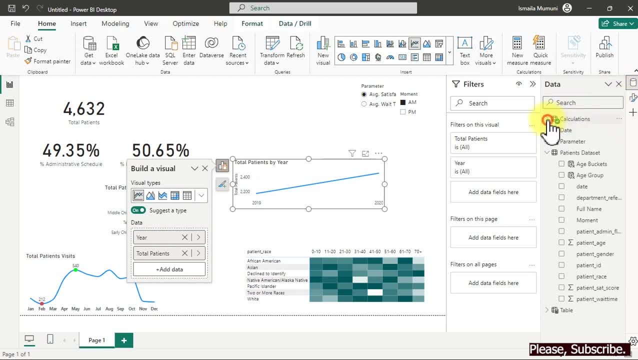 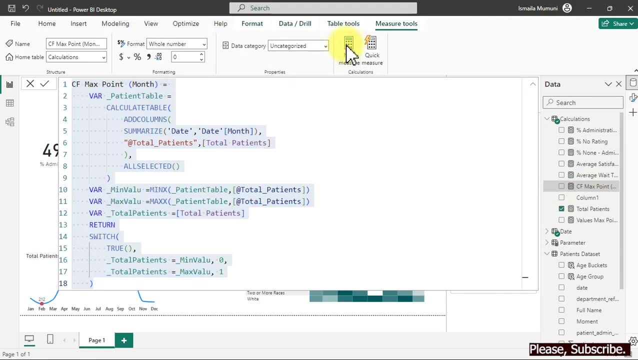 So all you have to do is not much, It's going over to here and This particular conditional formatting here. You just do ctrl c to copy. That was why I identified this one as month. The next one can be identified as year. 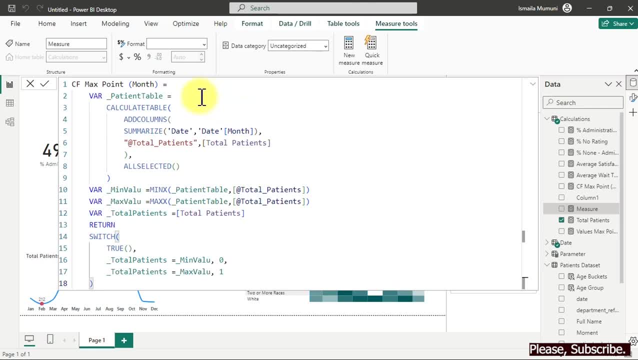 So all we have to do is just do one single change, And that is going to be this one. So, instead of month, we do the year. That is all we have to do. We don't need to do anything. Okay, Sorry. 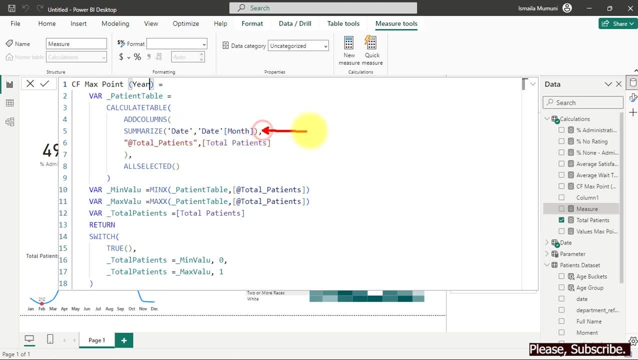 One more thing: We have to make a change of this Here. So the column we want to have here now is going to be the year. So I'm going to clear this. I'm bringing the year instead of the month. I'll show you how and why. 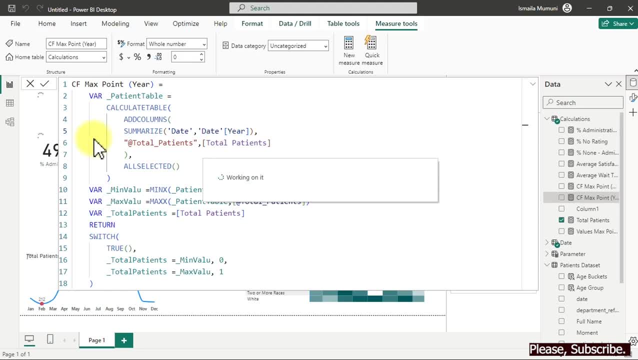 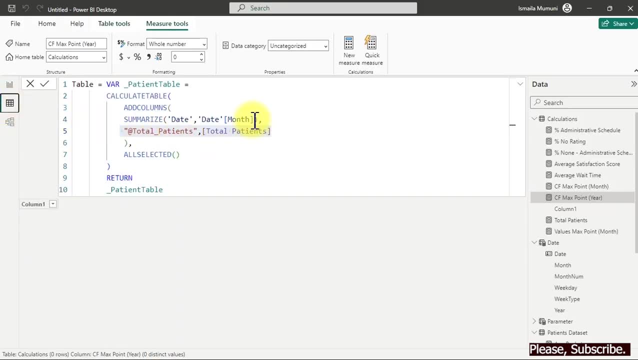 So I'll hit my enter key. I have made that change. Let's now go to the physical table that we have actually shown the other time Clicking here. So here we have the month This month, this place- Um, what the heck is it? 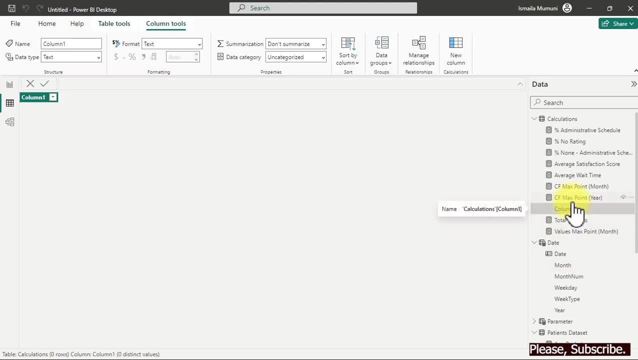 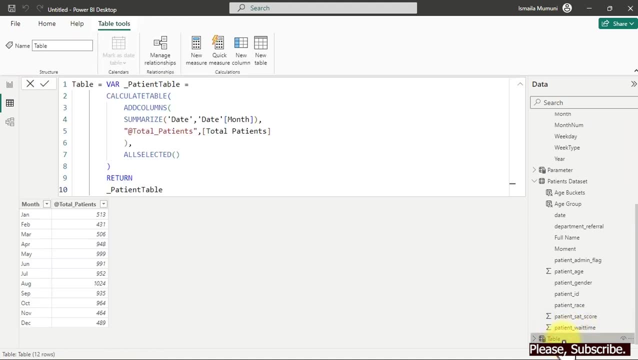 That is going to be column Max year. Sorry, sorry, sorry, I can see. Okay, This table. This table displays this. If I change this one to year, let's see what we're going to have. So I change it to year. 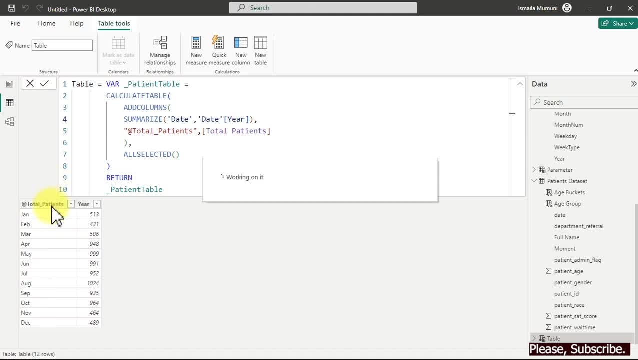 If I hit my enter key where I have month, would give me what The year Can you see? So we have the year here, so we have a total right here. This is what we have done. Then the system will be smart enough to look for the max. 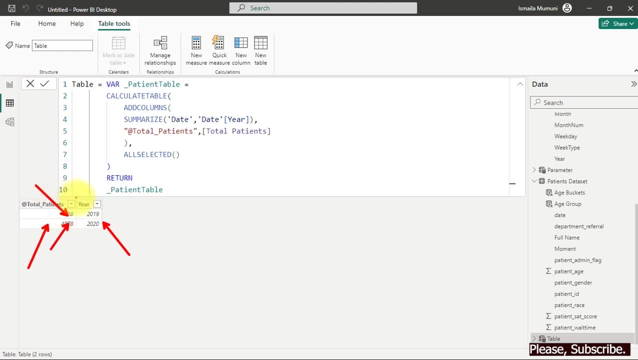 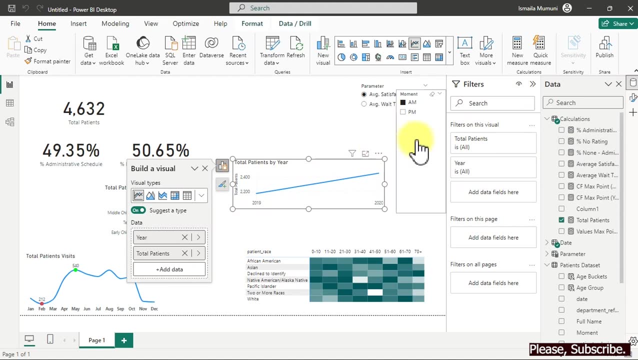 So to push this one as our max and this one as our mean. Very beautiful Now that we are. we have done that. you know the rightful thing. So we just go over to here. Why can't we do it over here? 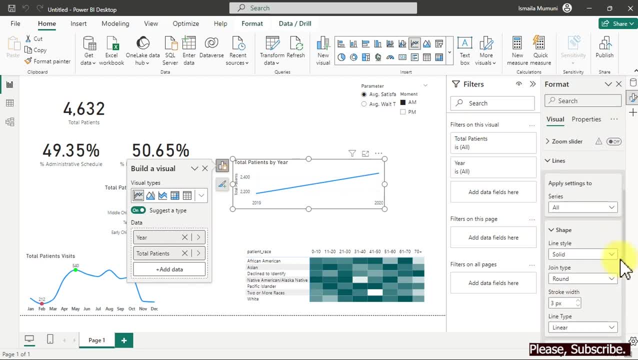 When we go to our line chart we just go to color and click on the FX inside our line chart. We have a color but this color does not have that particular. you know F? X that we have. that we'll click done to do the conditional formatting. 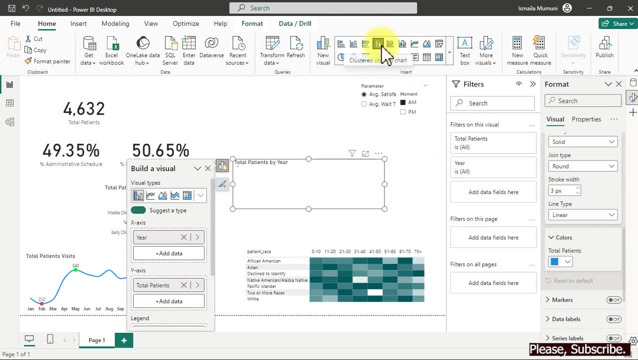 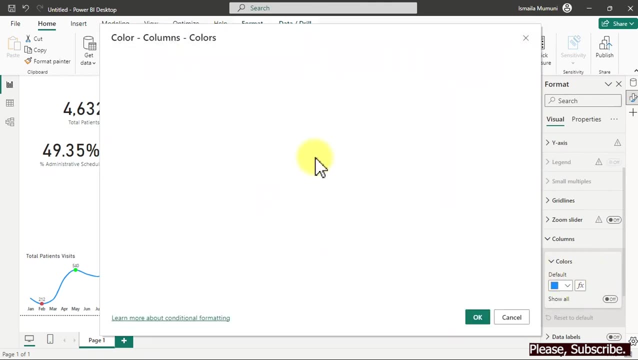 That was why we always go ahead and turn it into this particular kind of chat. Once we have done this, we click on the column and quickly you are going to spot what spot the FX here. So once you click on it now we choose the column. 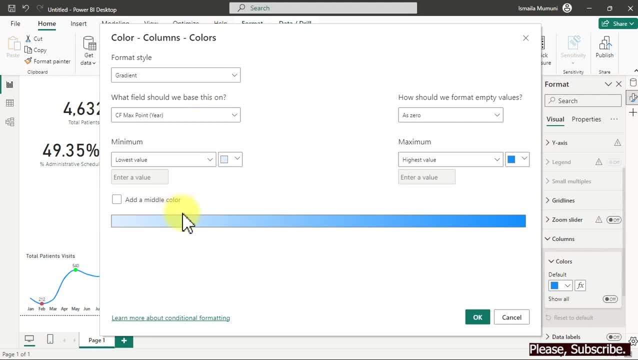 So which is the one with Ear? So when we choose the one with the ear, we can now say, uh, not great, but rule. So, where it is equal to zero, we make sure it's equal to zero, We change this one to number. 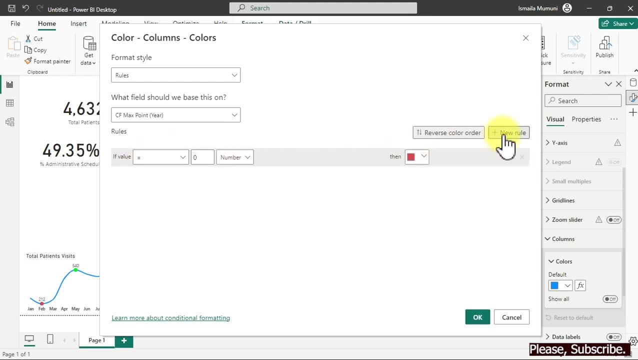 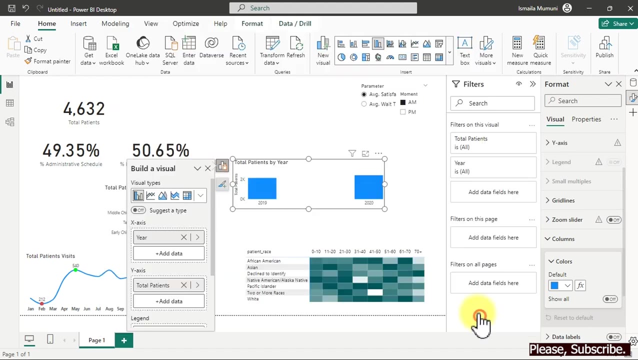 So we come here and we use red. So we add a new rule: where it is equals to one, We convert this one to number and we change this one to green. So we just select here to select the kind of green we want. Then we click. 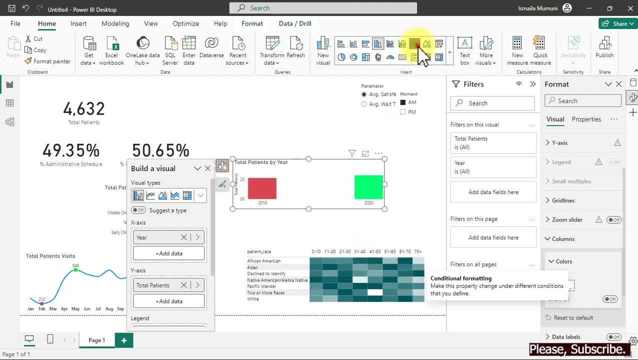 Okay, now we have it, So we convert it back to a line chart. So, despite that, when we actually come to a line chart, you cannot find that we still have this the way it is, but it has actually marked this particular point for us. 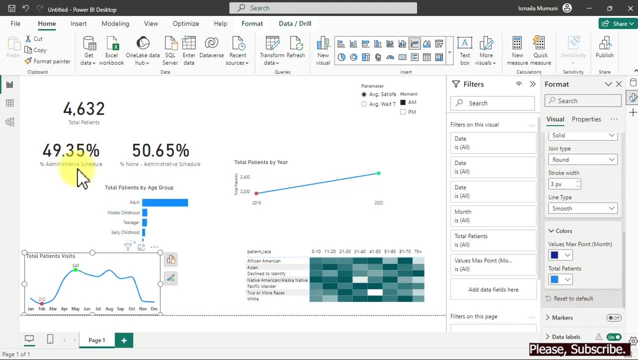 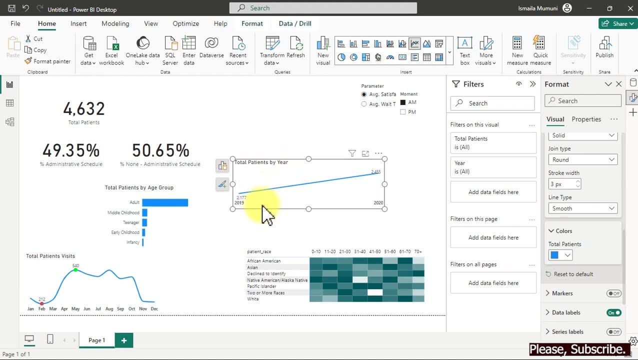 So now your aim is to actually format it this way. All you have to do: click on this one and easy format painter here, give it this, So you have this. Oh, now it's rubbish it for us. It doesn't really work, fine. 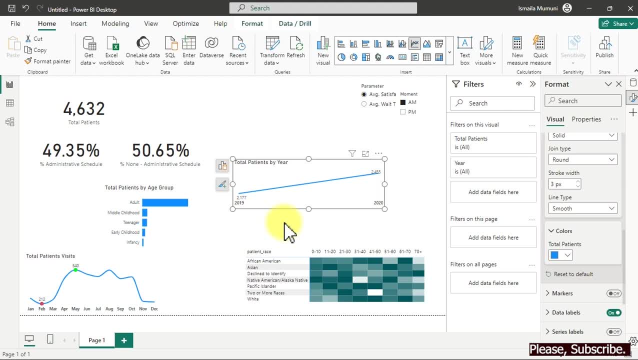 So it has taken off the condition of Martin. We have any. we have to fix this. just control Y to take it back. So we have this back. So we manually do our formatting here. So we turn this off. Then, for the X, we just make sure we go to the value area and open it up. 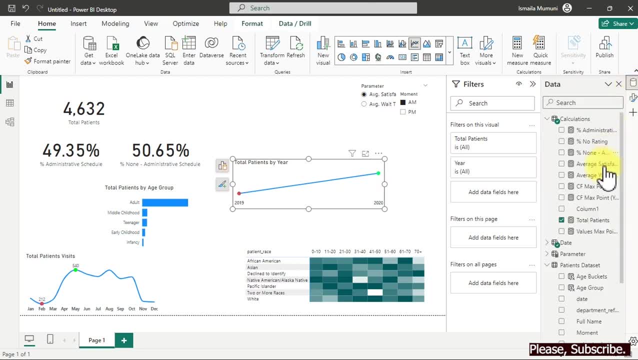 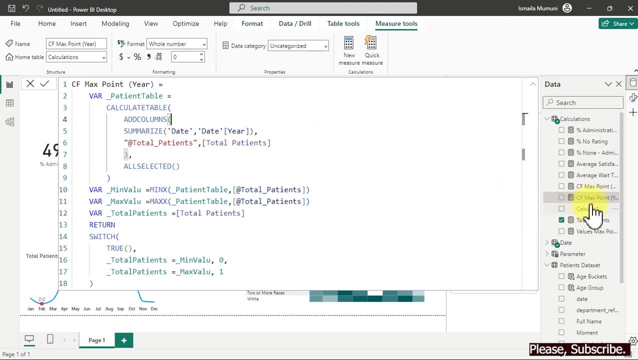 Ball. This one is fine. So we go back here and now. we copy the condition of Martin for year, and instead of doing this for year, let's do value max. we just make few changes. Then we click here to create a new measure. 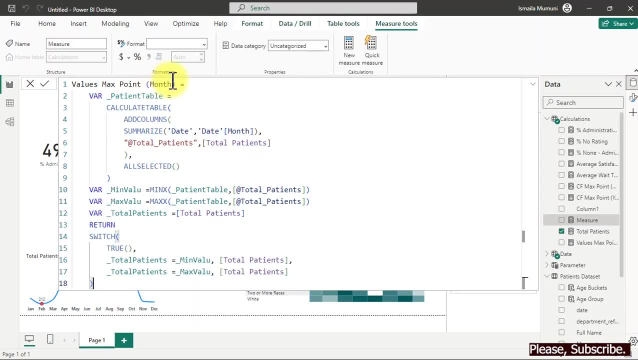 So I'm going to paste this in for the value max We put in here here To identify this. then what do we do? Just make a change of this to the year. Now we're done. We hit the enter key. This will now extract the max year and the max month, the max year and the mean year for us. 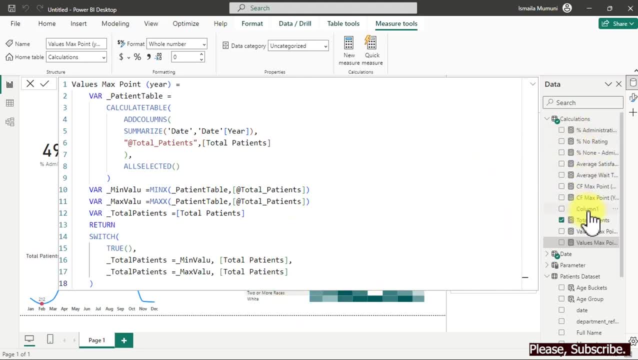 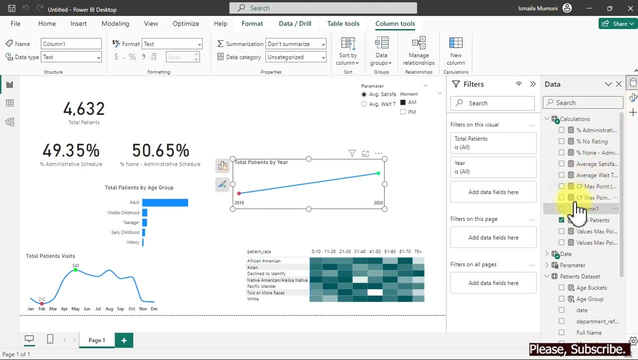 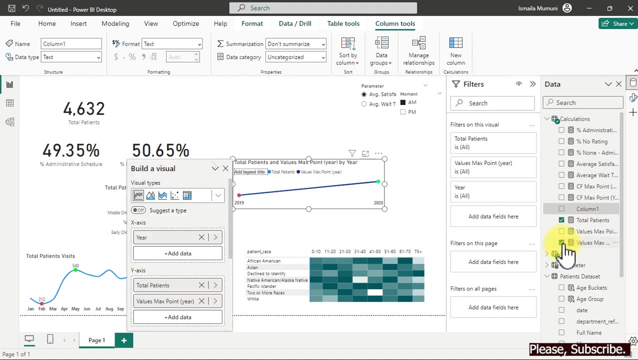 Then we go back. I used to remember how we did this. I can't remember again. Oh, I think I still remember. Okay, that means we're going to push in this particular max that has the year into what into here. This gives us this. 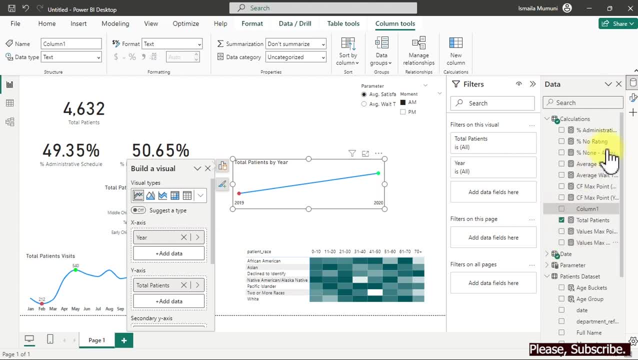 Does it sound well? I don't know. Okay, first of all, let's come here and go ahead and open data label. Where are you? Here we are, We have the data label in. Go back here and push in this particular max that has the year into it. 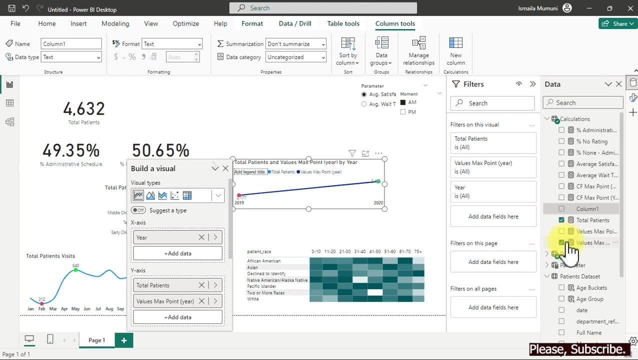 It changes the way I see it is right. It's not a problem. What do we do now? We are going to go towards to our formatting here And we go to where we have the format for our data label. We scroll down, so we choose total here and turn it off. 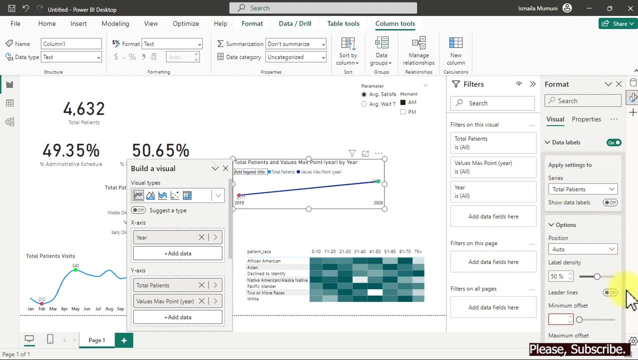 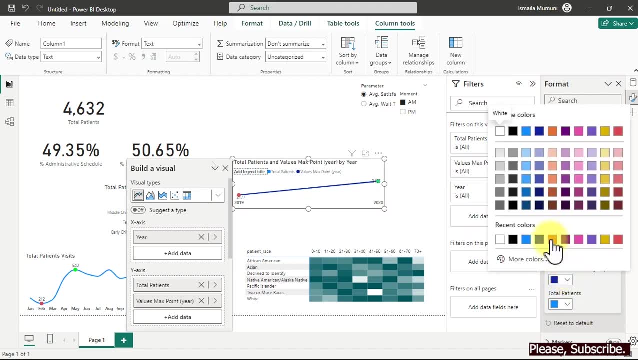 It has given us this. So once we have this now, we can now go over to here on this one and give it white. Does that make any sense? Give this one this color? That doesn't make any damn sense. Where do we flub? 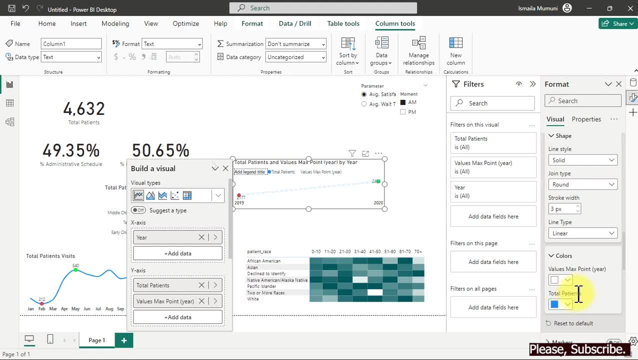 We don't want to have this color, Why are we having this particular color right away? We shouldn't be having the color. Should we be having it? So it shouldn't be affecting our visual So, which means we just turn it into the same color. 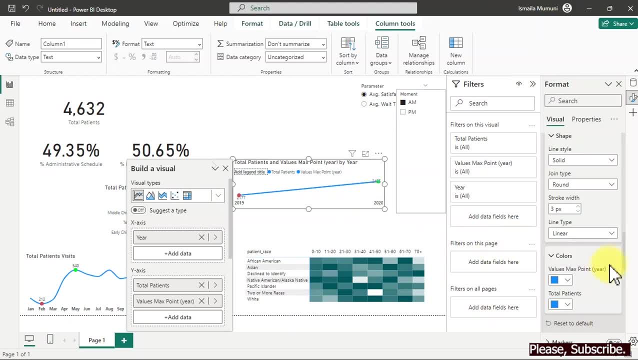 Now we have one single color for all of them. It's not a problem now. So the next thing we have to do now is to scroll a little bit up and look for the legend, Turn off the legend And make it. Make it as clean as this. 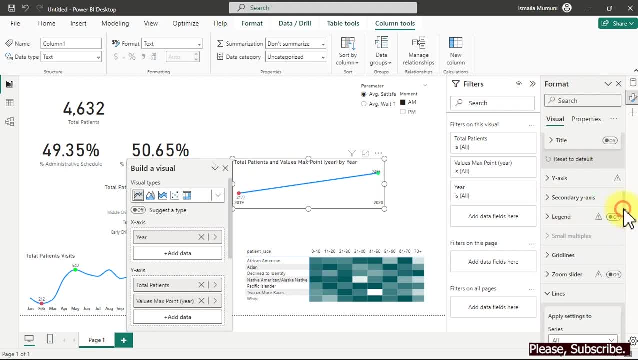 So once we have done this, now it is time for we to go to the title. Then here here, here up here, we have the title. So we come here, remove this, and we say by year, So it's going to be visit. 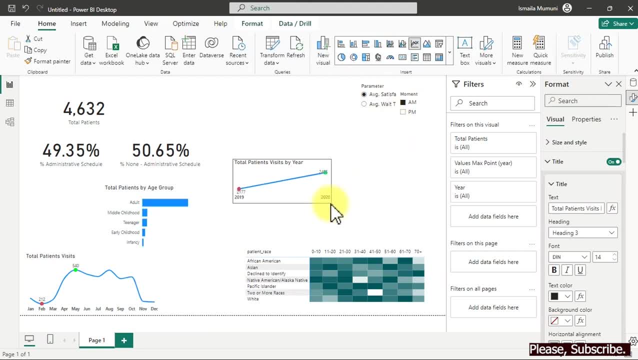 So we have this. You can just make this as small as we like. We keep it here. So for the color, don't worry. For now we are not ready to change any color we have on it. But just don't worry. 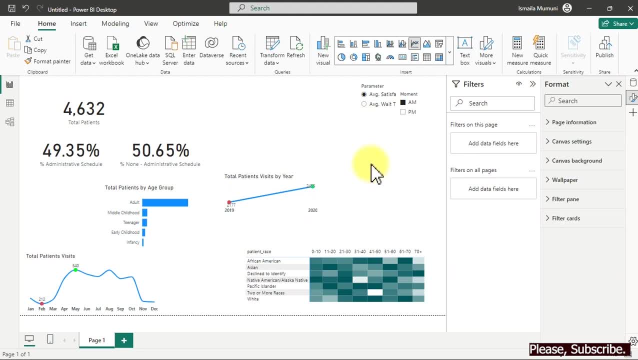 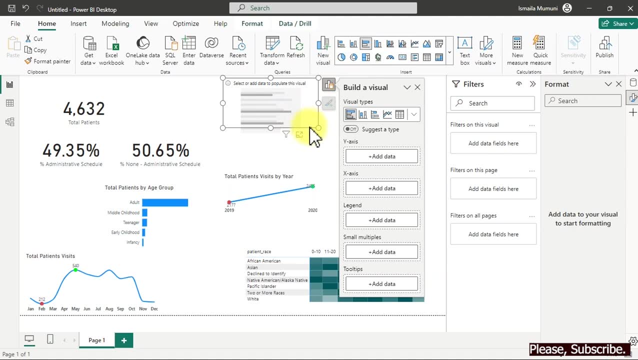 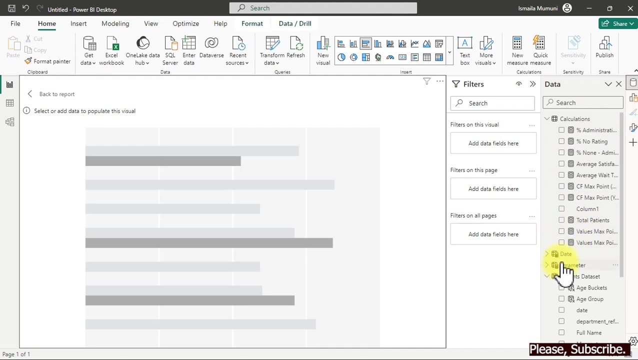 Okay, We have another chart to create. That chart will be total visit or patient visit by department referral. So how are we going to be this chart here? So, with this chart, what do we do with? We come over to here And we select our total visit from the measures we have written to the patient's visit here. 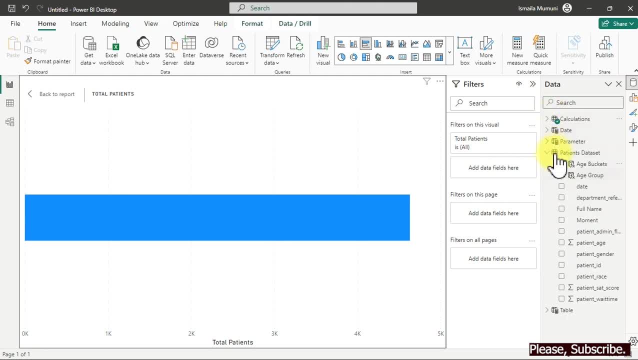 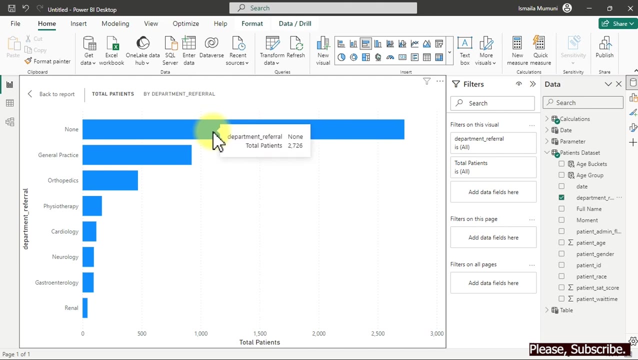 Now it's looking ugly. Let's do it. When we go over to our patient's data set, we look for the one that says department referral. Wow, That is it. So now it's showing us none here, None, right here. 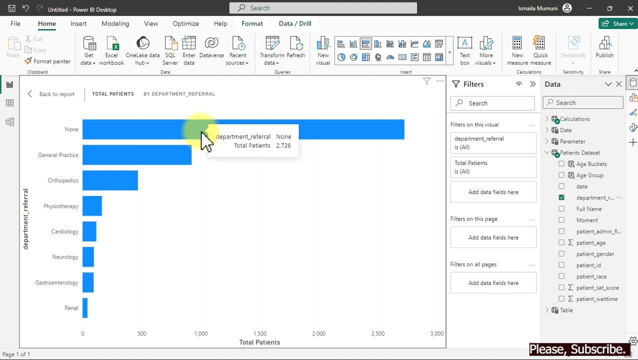 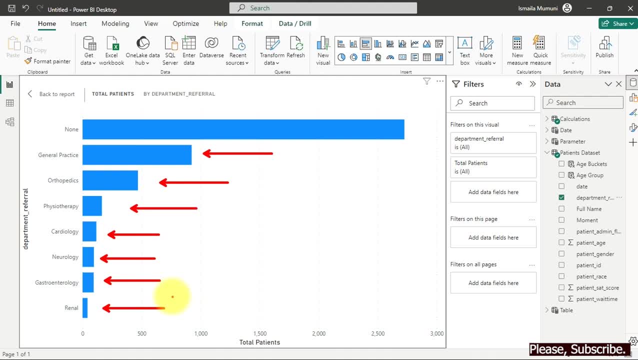 This is based on the kind of condition that the person would have before he or she visits the hospital. You understand, But what about? none Is none a medical term or a number of a doctor. We want to know because we want to use that to create something. 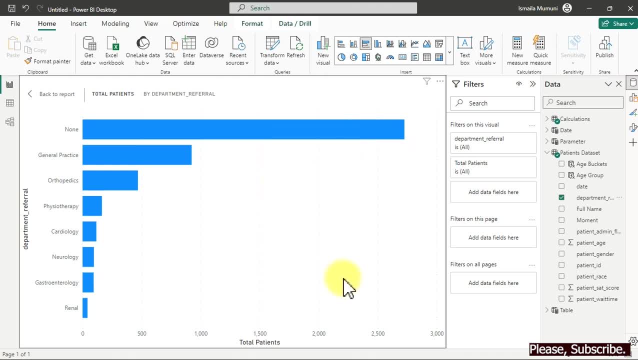 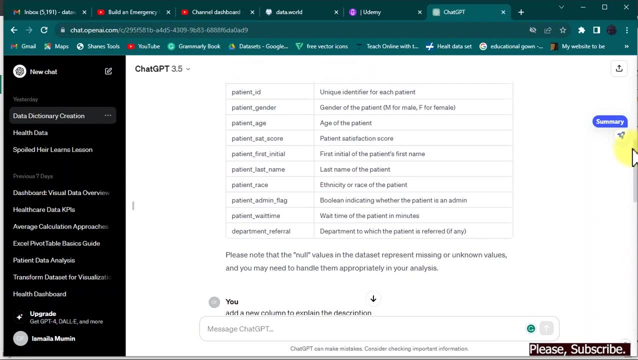 Different. So what do we do? This is the time to visit back our chat GPT, So now we have to write a prompt here. Before we do that, remember, we have the data set paste here, So you need to know the column you want to deal with. 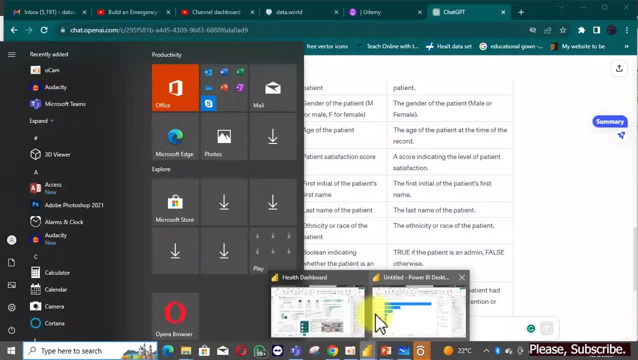 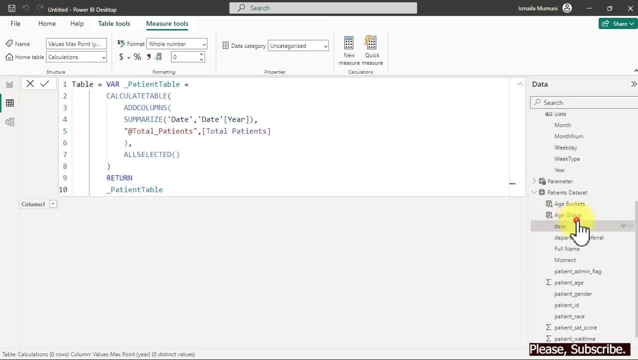 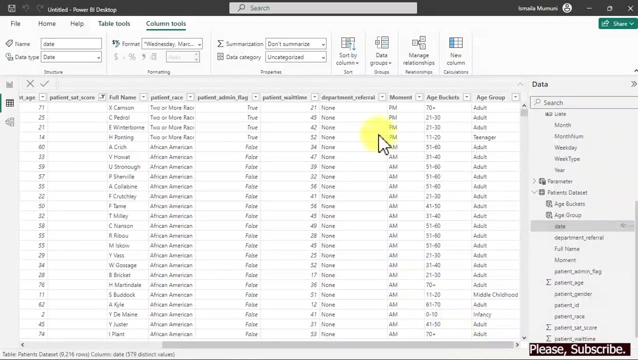 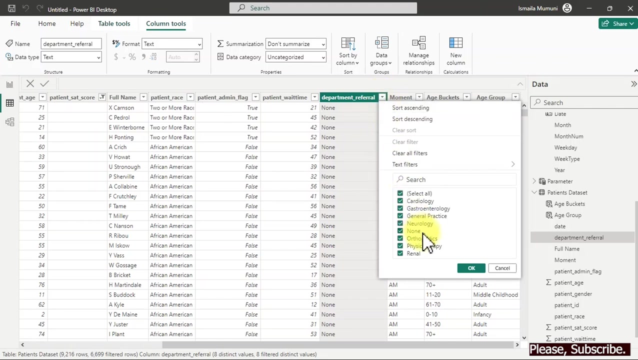 You get it. So if I go back here now and I click on my data, So we're going to have, I have to look for the column involved. So here's the column: departmental referral. So for the departmental referral, we have none and we have other ones. 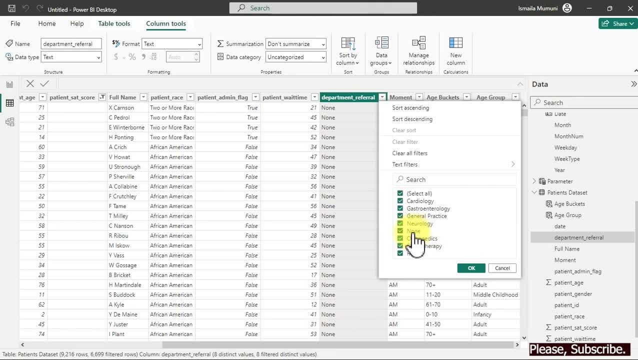 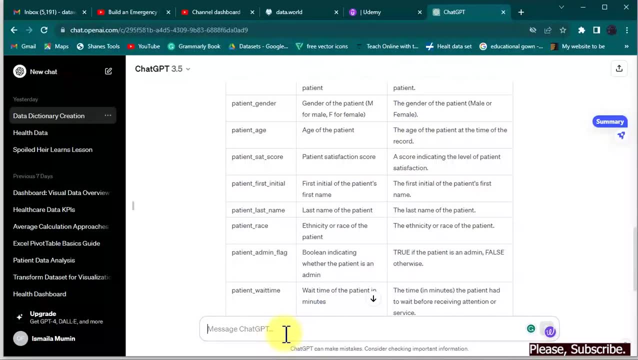 Right. So what we want to know is: what is none? Then how do we prompt it? So I come over here, I type in the: so write the column Exactly The way it is underscored. referrer. What is the meaning of none? 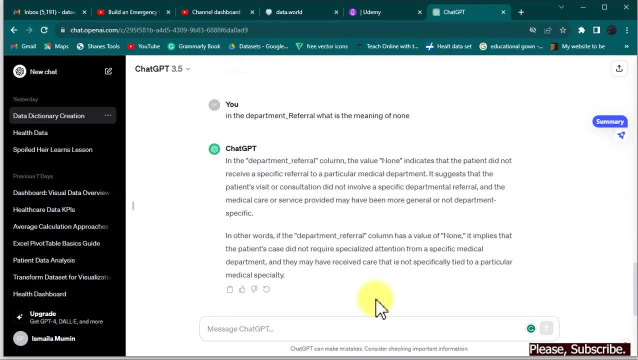 So GPT Just helped us with it. It says in the department referrer column: the value none indicates that the patient did not receive a specific referrer to a particular medical department. It suggests that the patient's visit or consultation did not involve a specific department referrer. 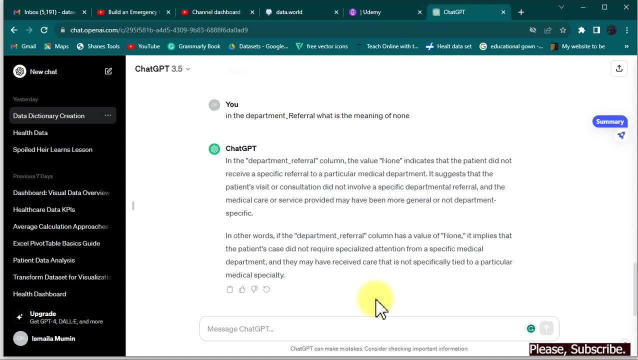 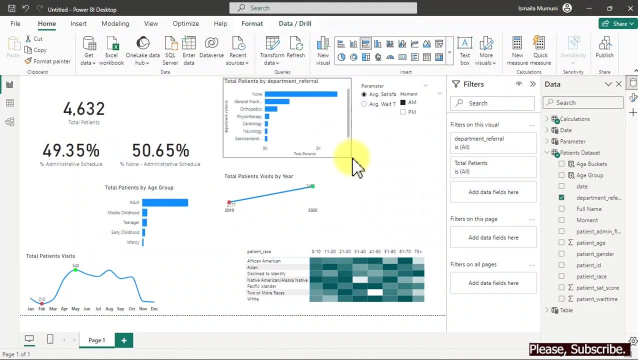 He just walked in and into the medical center. He does what it is. Now that we have known this, we are going to use this to create something very important. That was why we came here. All right, Being here the very first thing I'm going to do, let's maximize this a bit. 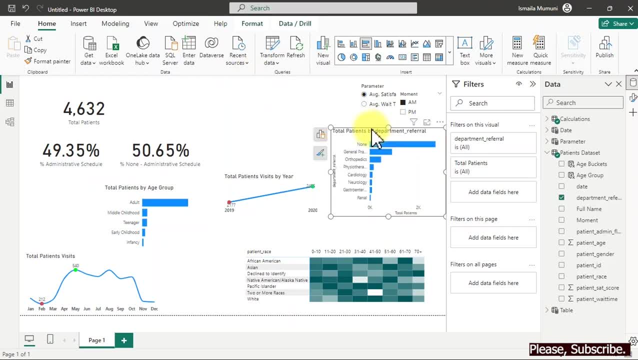 I'm going to push it over here. for now It's hard, Don't worry. We're going to fix all of this when we are done creating all our charts. Then I come over to my calculations here Inside, the calculations I'm going to actually add in your measure. 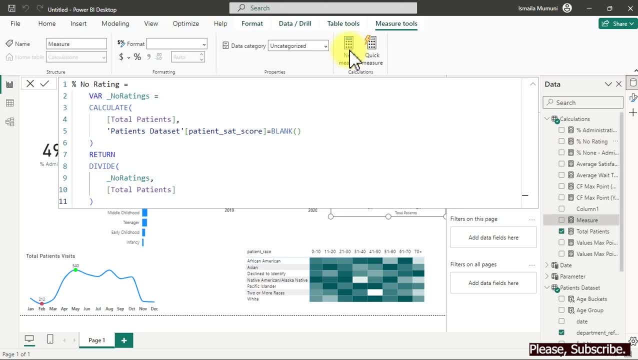 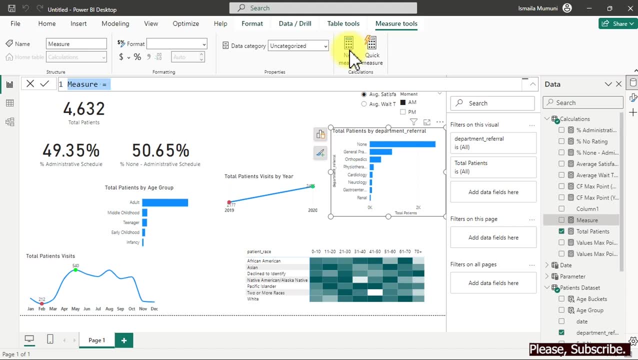 So what will this measure be all about? This measure would actually be about what I put this about: the percentage of the people that walked in willingly on their own and the people that actually got referred to a particular doctor whatever, or medical line whatever. 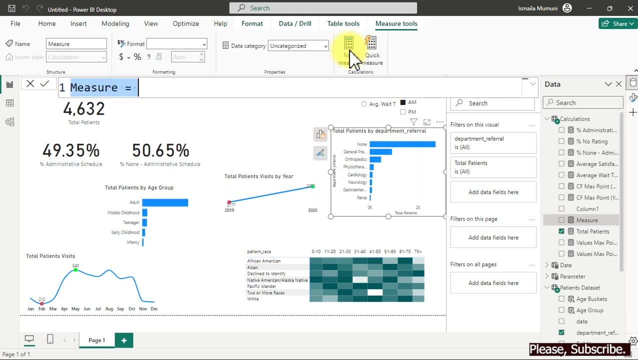 So now, what are we going to do Over here? we're going to do the percentage of the people that do not have any referrer, which is under none. So to do that now, what I will do is to use percentage of on. 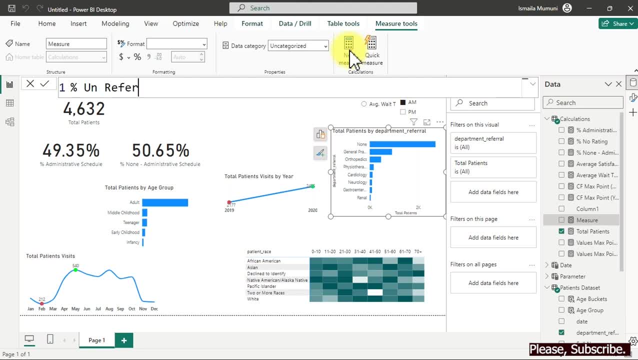 Let me use the word unreferred- Unreferred, Do I get that right? Patients. So. So we create a variable here, variable. So this variable, we're going to name it filter patients. So filter patients. So for our filter patients, now we're going to do calculate. 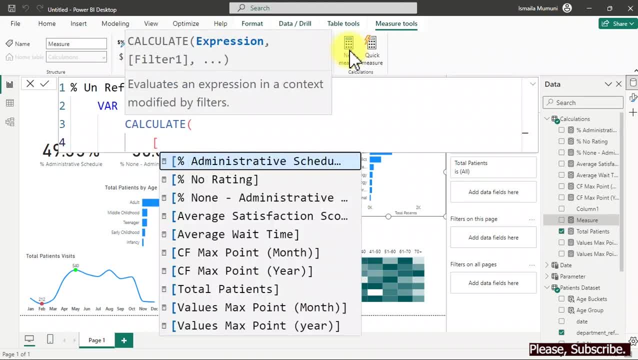 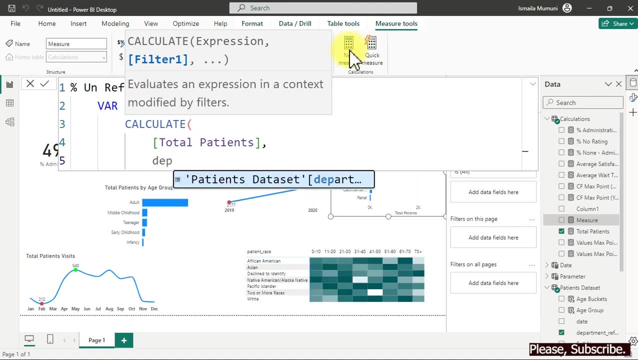 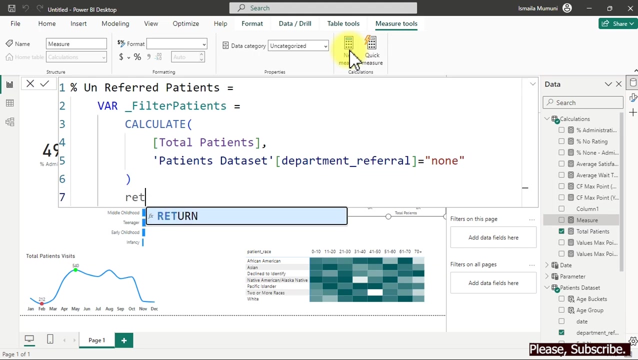 So we do all our patients, total patients- Here visit, So for that we have to filter the department. So where it is equal to none, So we close our calculate, So we come forward now and do return. So under the return we do divide, and we divide what? 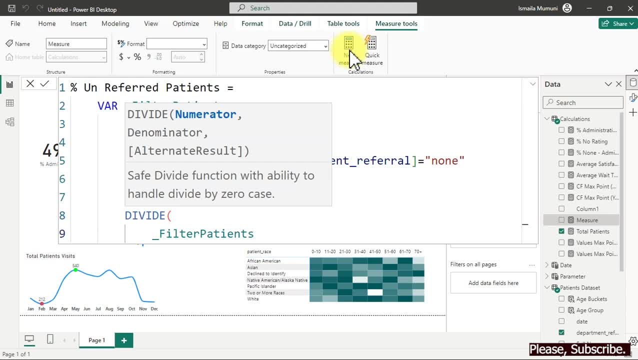 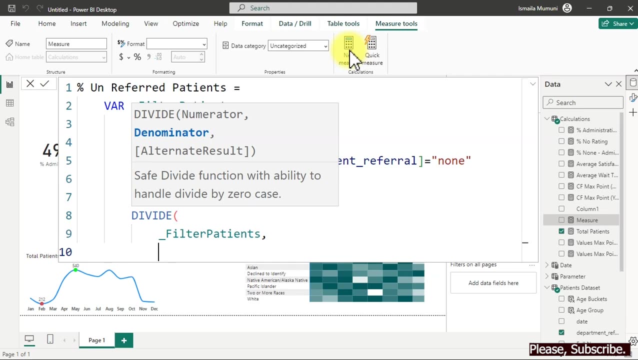 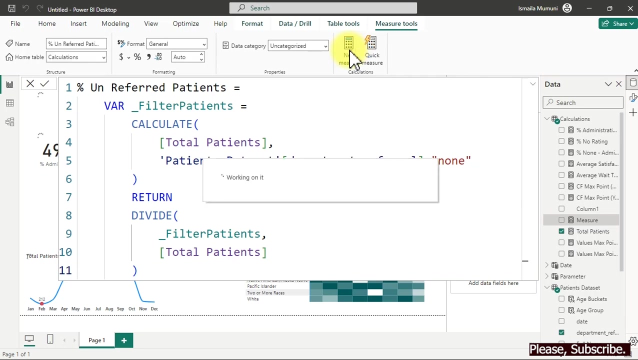 We divide our filtered patients. Remember, Inside the filter patient, we have reduced the row in the main table to just where the patients is having none Right. So we divide it by what? By the total patients that creates for all the percentage. 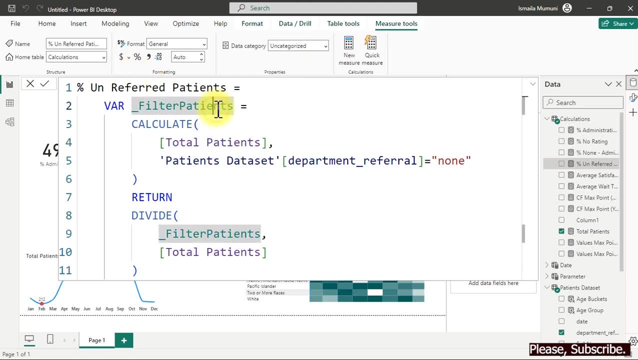 Right, Okay, We can convert this to a percentage, But before then I'm going to do control C, to copy When I control A, then I convert This into a percentage And after the conversion into a percentage, we are going to actually create a new measure and just make two changes to it. 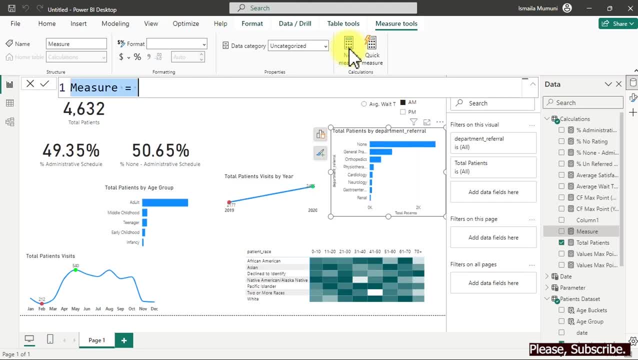 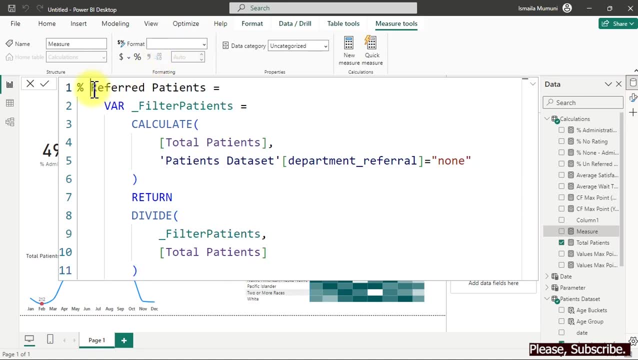 So I'm going to paste this one in here, So it will be percentage of referred patients, And over here I'm going to use: not, This is not, This is not none. So now it's going to actually create in that table that would exclude none and give us where we have patients being referred. 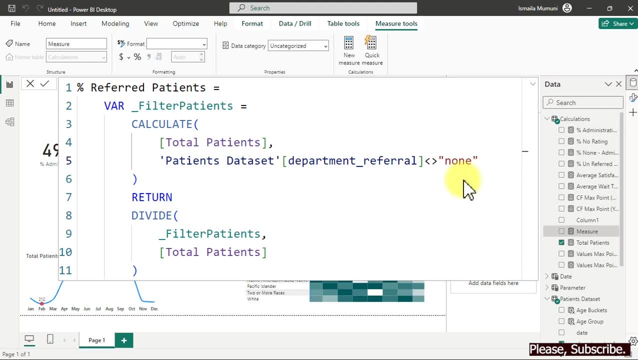 So we just do what we just do: Hit the enter key So we can convert this to a percentage as well. Now we are done from here. Let's see. Let's see what it is that we have done. I can bring this into a card. 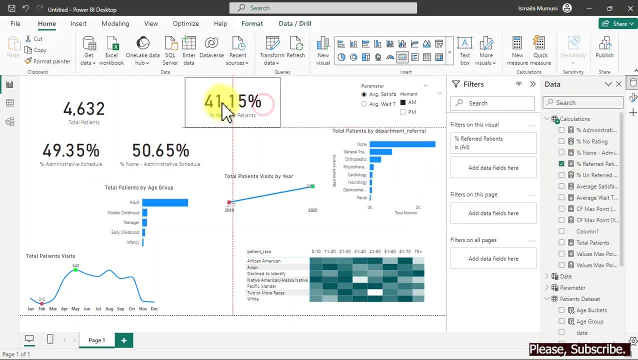 So percentage of referred is 41%. So non-referred patients gives us 58%. When you add them together, they give you the total 100%. Do you see that Beautiful? So We have just like some couple of measures to create was, yeah, maybe three different measures, or four, if I'm not mistaken? 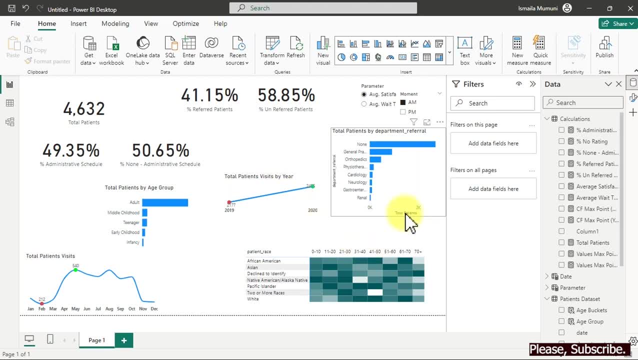 The very first one I'm going to create first is the one that affects this one, This one here, So this one has this slicer. I'm going to bring it down here. So every single time we actually move this, nobody understands what is going on with this particular patterns we have inside this particular heat map. So every single time we actually move this, nobody understands what is going on with this particular pattern we have inside this particular heat map. So every single time we actually move this, nobody understands what is going on with this particular pattern we have inside this particular heat map. 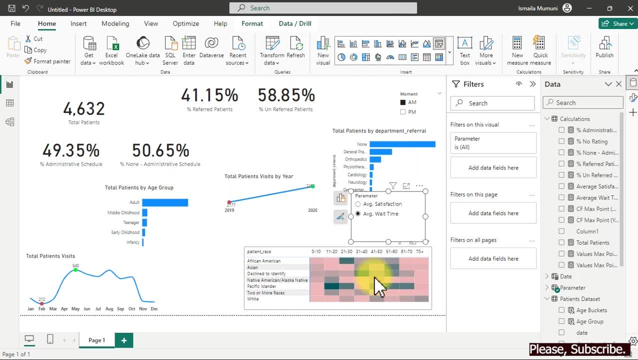 How do we make it readable? Very important: We need to know that. Okay, We're going to do something. now What do we do? Let's go back to our parameter, which is the parameter we created. So here is the parameter. 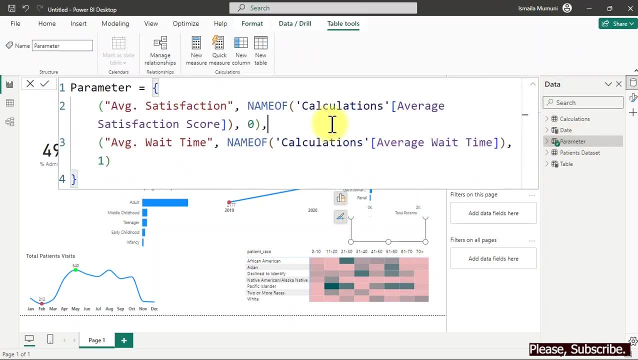 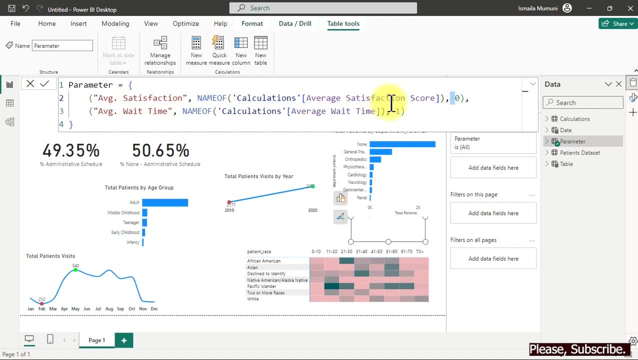 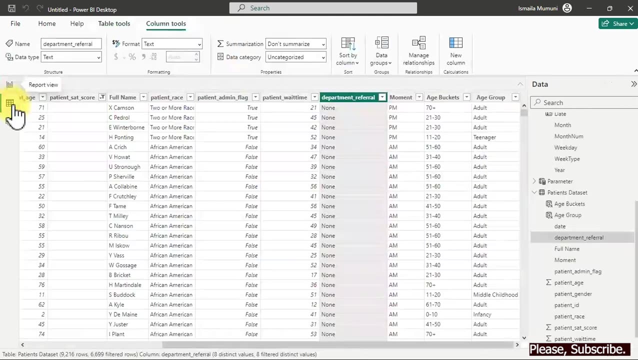 When I click on the parameter, what do I see? I see this. So my parameter actually has what Has zero for average satisfaction And one for average wait time. In case you don't understand this view, let me give you the table view. 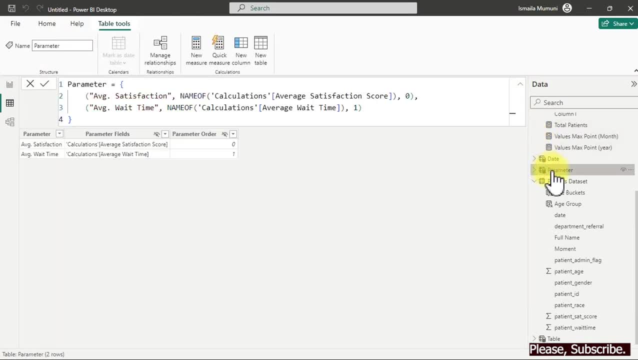 And under the table view, I'm going to go ahead and click on the parameter. So, inside the table view, if you look at it, these two are some kind of hidden. They are hidden because we don't need to use them. This is the one we're going to use. 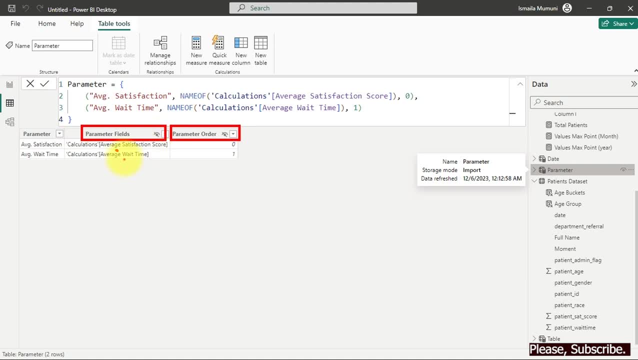 But we can still reference them In a measure. So this particular eye icon here have been checked because we don't want to see them. So right now we want to use this very column. So this column has zero and one. So zero is when it is average satisfaction and one is when it is average wait time. 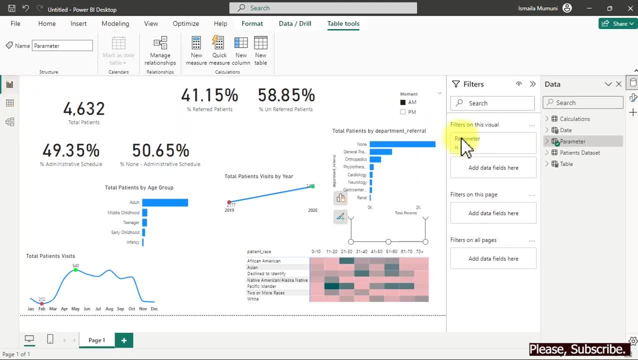 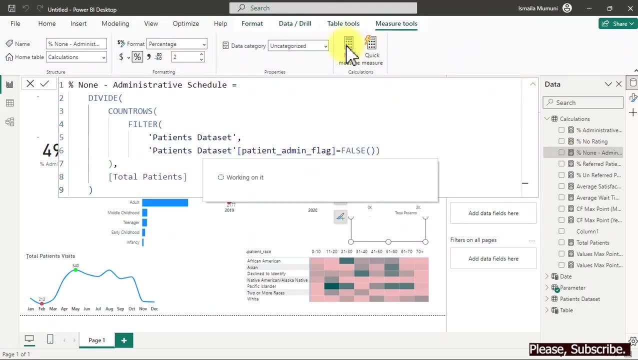 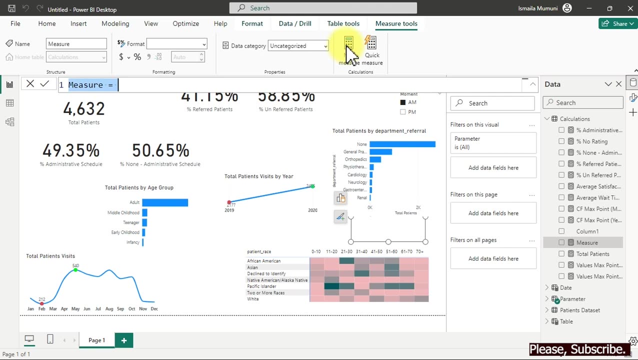 How do we make use of it? Let's do it So: we go over here, we click on our calculations and we click here, We create a new measure. So this measure will tell us what we see in the heat map, so that it will make it easy for the end users or the consumers to actually tell exactly what they are seeing, without trying to guess what it is. 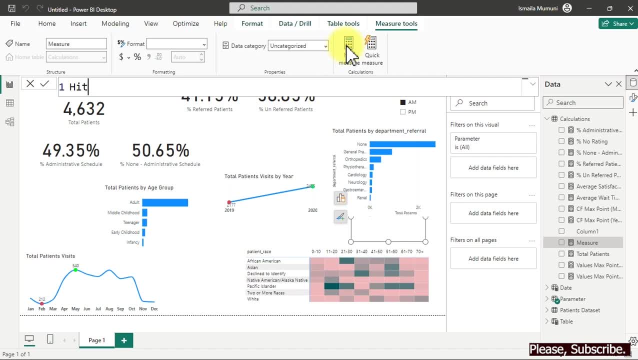 All right, I'm going to name this one. It's map caption equals. So with the heat map caption, right now I'm going to write variable, So this variable will be underscored under course. selected measure, So selected measure. it will be equals. 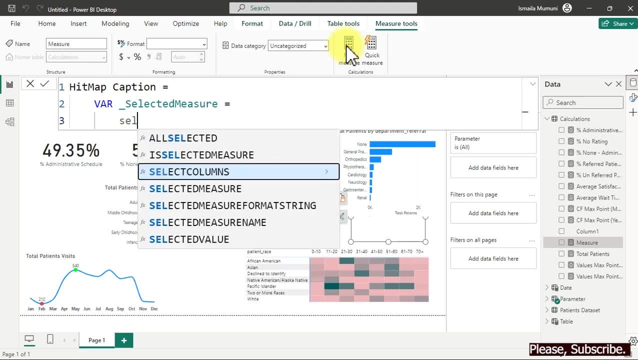 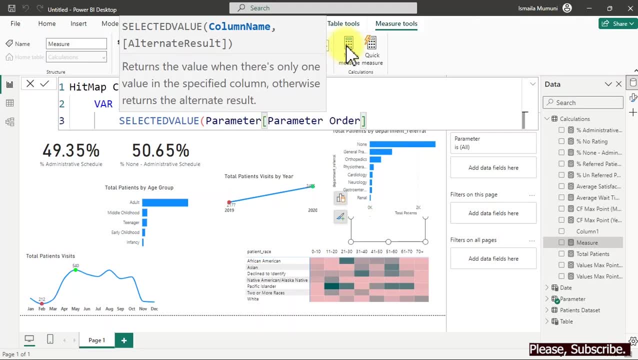 So what do I do? I want to use selected value here. So if I use selected value, I want my selected value to get in order. What is order? Order is one column among the three columns we have inside our parameter table, So we close it. 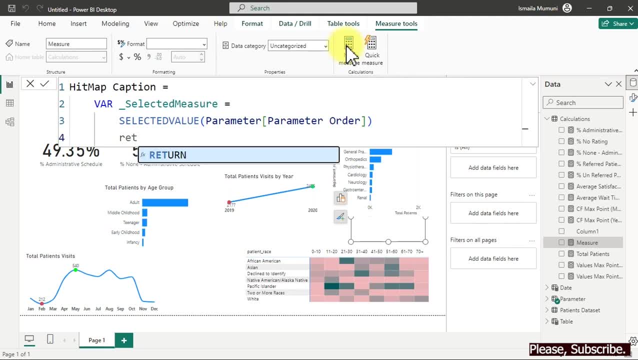 Then I'll come over here and do return. So return what Return? underscored selected value or selected measure here and hit the enter key. First of all, we want to see what this will return to the screen. All right, Let's go ahead and pick it up. 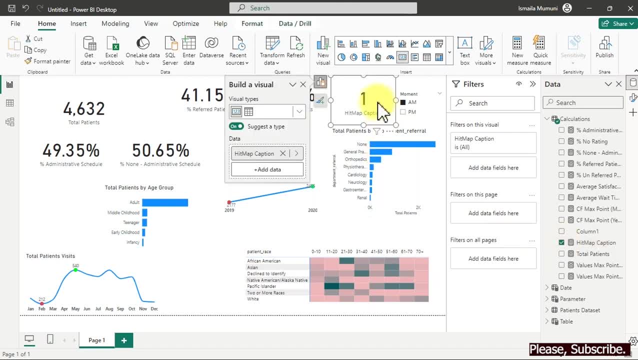 Heat map caption. So it's giving us one when we select Here we go. When we select average wait time, it gives us one. When we select average satisfaction, it gives us zero. Average satisfaction gives us zero. This is what it is. 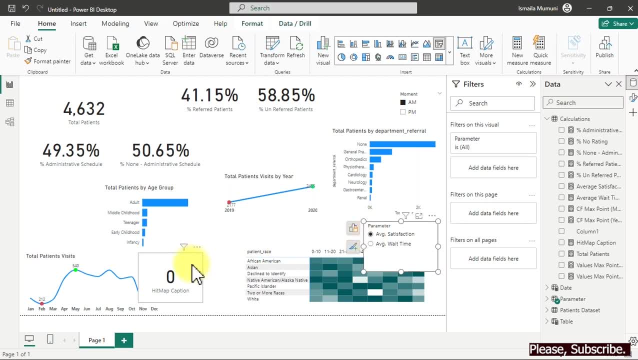 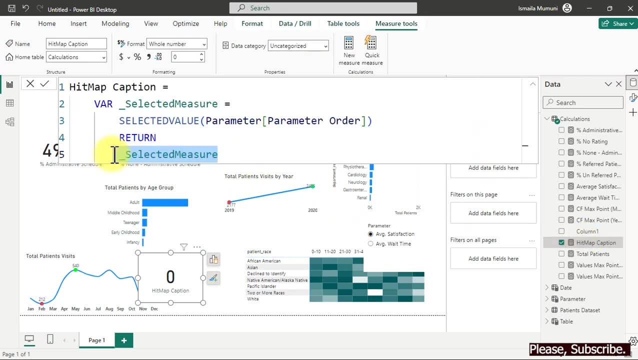 Now we can further use this to customize how we want the caption to look like. So go back Right here under the return. So we're going to type if here. So if this particular selected measure here is equal to zero, which means what is selected is actually average satisfaction. 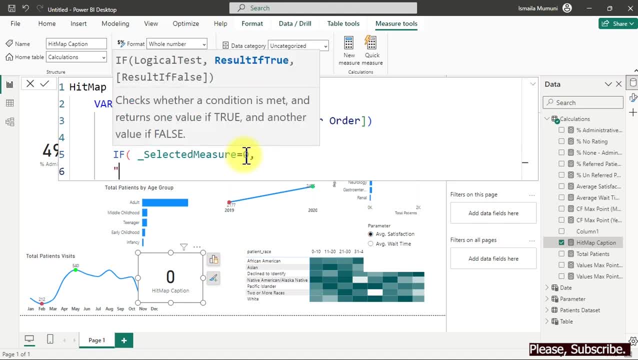 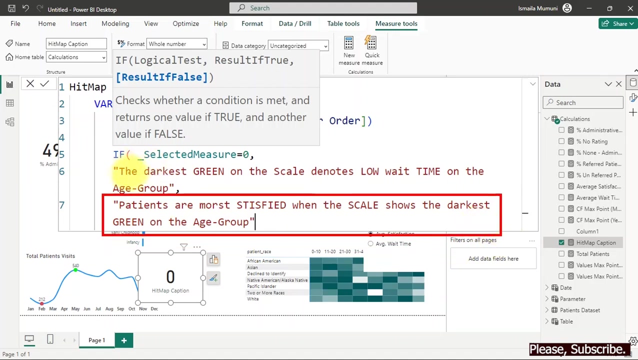 Then we want to actually show something like the darkest. So the word green on the what, On the scale, The naught, So on the otherwise, we actually show this particular message here. So when it's actually equal to zero, it's going to show this particular one here. 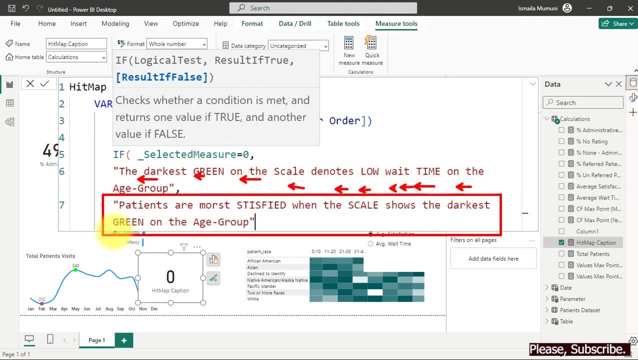 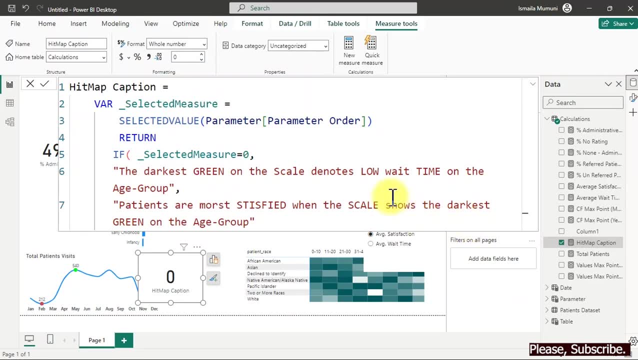 So which is this very one here is going to show it. so when it is actually equal to one, then it will display this very one we have here. so let's just look at it. i'm gonna have to close my if and hit my enter key. then zero will change to the first condition. 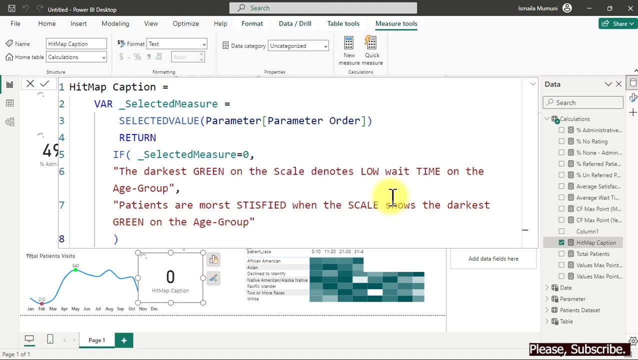 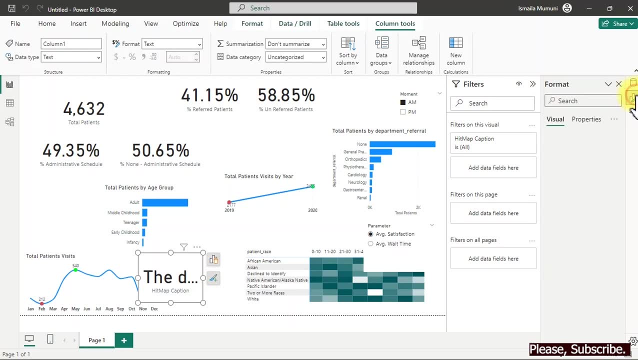 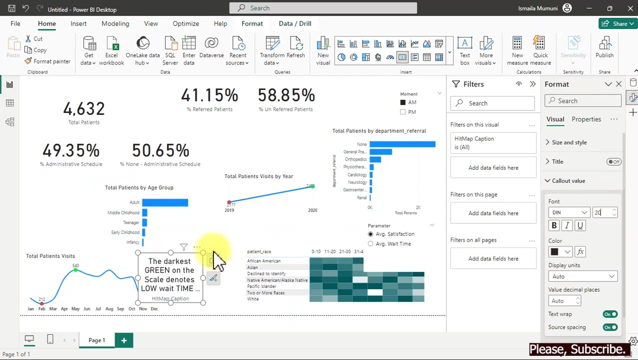 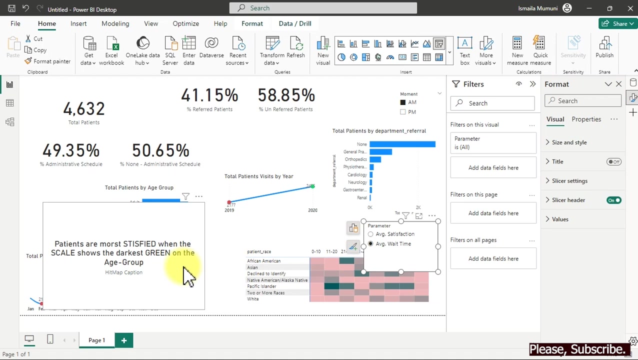 now we have it. let's just look at it. so first of all, i would have to come here and go over to here. let's turn it into 20 so we can maximize it now. so this is what we have. what happens if i use this? it changes exactly. so this is what we want to use on this. 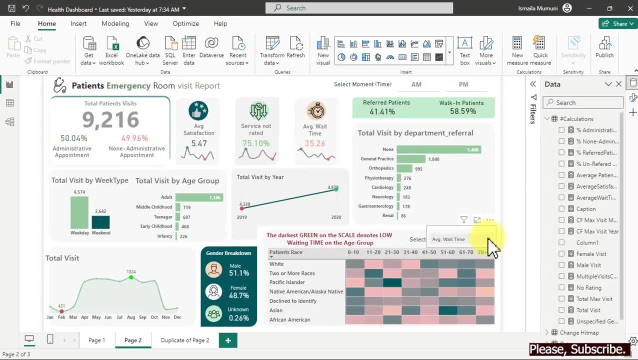 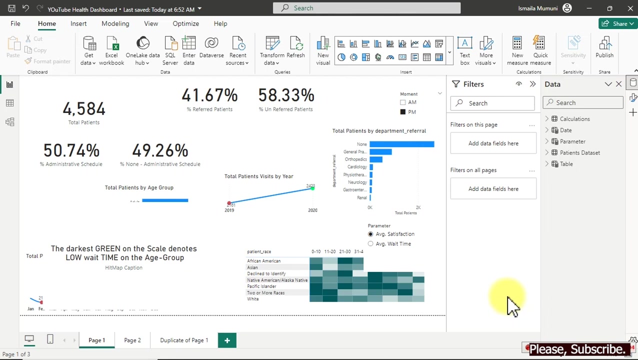 let's look at the final result. here is the final result. just like what you have seen previously, whenever we make any changes, it's actually, you know, change the caption that we have, and it will make the heat map very, very much readable. what about that? all right, the very part you're waiting for is actually here. that is the designing. 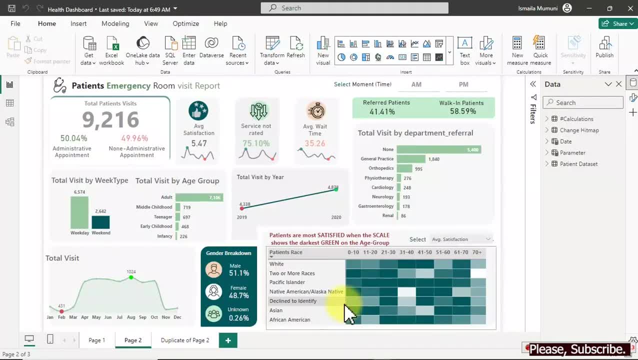 we're going to create something that look exactly like this one right now. you always know. if you had been on my youtube channel before now, you know how i take the view very seriously. so now we have to head up to powerpoint. but before we do that, we have to go back here right first. now we're here. 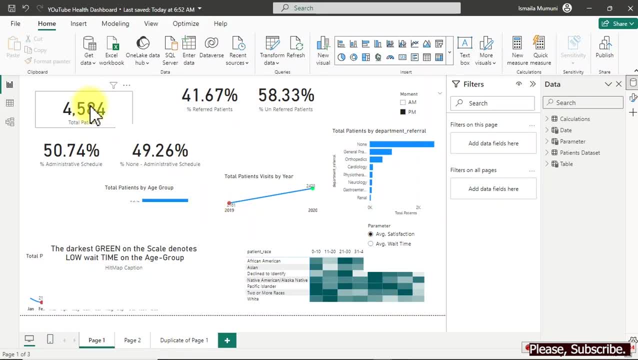 this is not looking fine. so the very first thing i do is to start to some kind of change. what it is that we have right here, so right on this, is our patients. that is the patient total view. so what i'm going to do to it right now. so we have to format it. 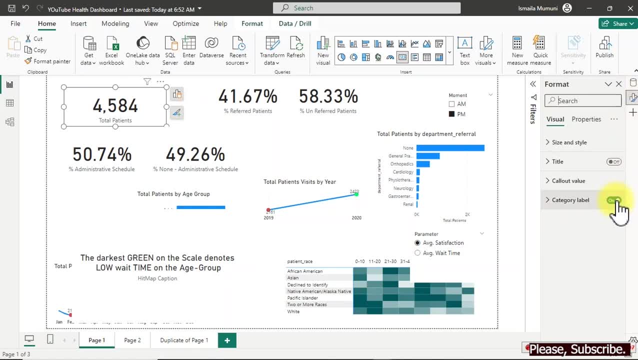 the first format i'm going to give to it is to remove the data or label category here. that gives me this. then click on this particular call out value here. then we're going to leave it at 47, so 47. so i'm going to change this one to a bolder font. 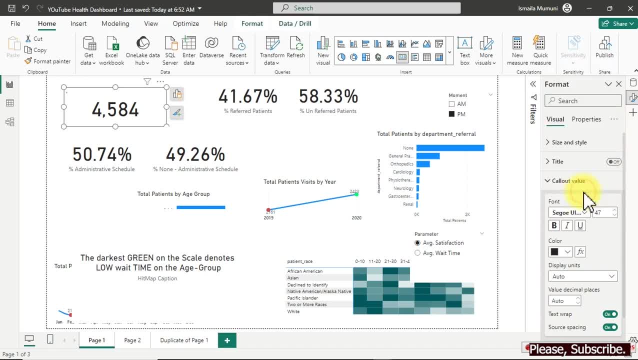 if i scroll down a little bit. so i'm going to have this one here. so this gives me what i want. then, for the color is to deck. i'm going to make it some kind of light, so let's go with this one for now. that's cool, so maybe later, after all, we might decide to change it, so it's all right. 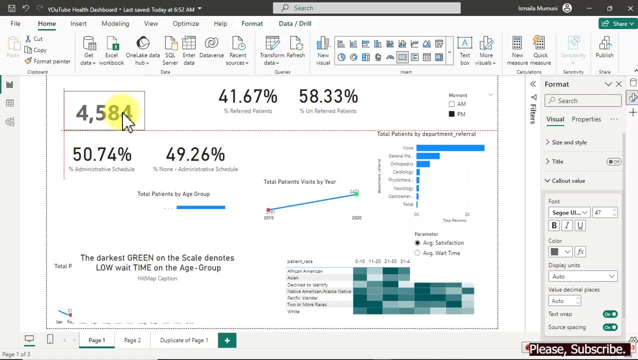 on choice. so i'm going to make it this way. so remember, there's a filter coming from here. if i unfilter it, i have the whole number that that is going to be peculiar the way. okay, now, with this one, let's talk about this, this here. i wouldn't. 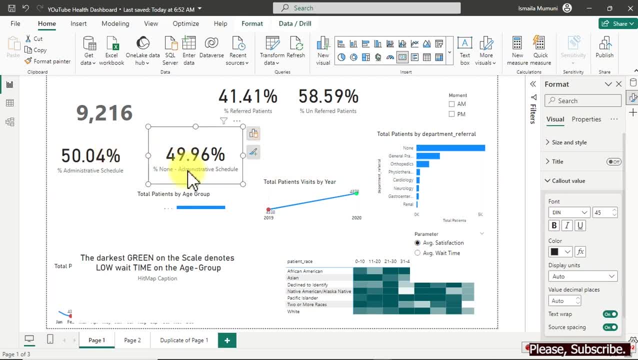 like to show it as well. i don't like to show the detailer bill. i want to get them off. so after getting them off, i'm going to create my own custom detailer bill that will stick the way. i really love it. that is why i do that. so what i'm going to do now is to actually have this one on 20.. 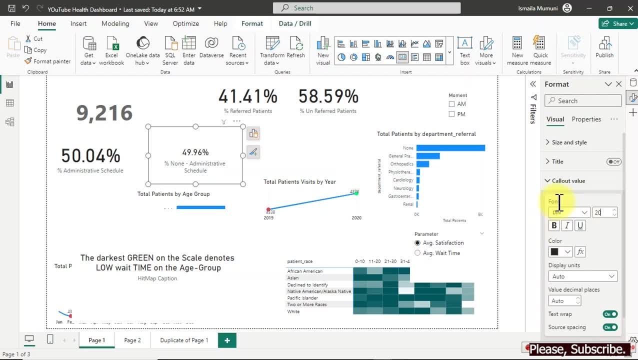 that is beautiful, so i'm going to leave it at this particular font here. then for the color, we'll adjust it later, but for now let's do that. so i'm going to remove the category, so make it smaller. don't worry, we'll find how we can get what is sitting there, so i'm going to push. 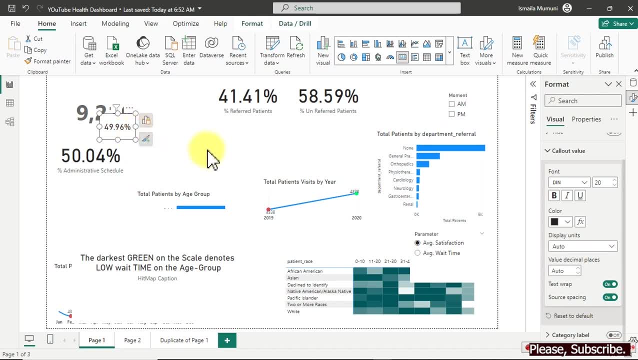 it very close to this one. if you look at it right now, it sends the major one behind. so what we're going to do is to go up and click on this. then we click on this one here. so quickly i'll do the same for this one. nicely done down. the next thing now is to scroll a little bit down and turn off. 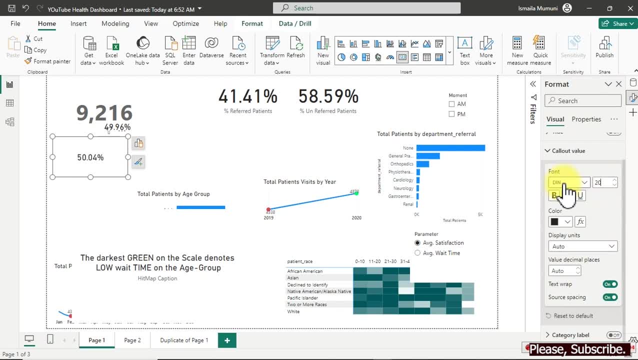 the category and send this to 20.. so we have the same size, so let's make it a bit smaller. so now this one will be somewhere around here, while this one is staying somewhere around here. just make it this way. okay, nicely done. so if you look at it, it's now making a little sense. 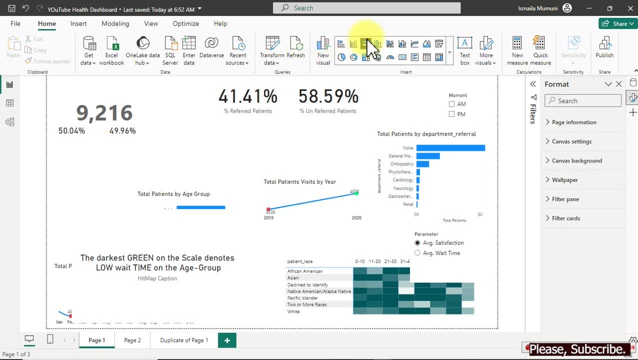 what else could we do to this? so we have to go over to our text box here. inside the text box, we're going to type in something we want to show that defines this and this now for this particular one. i'm going to type in administrative appointment. 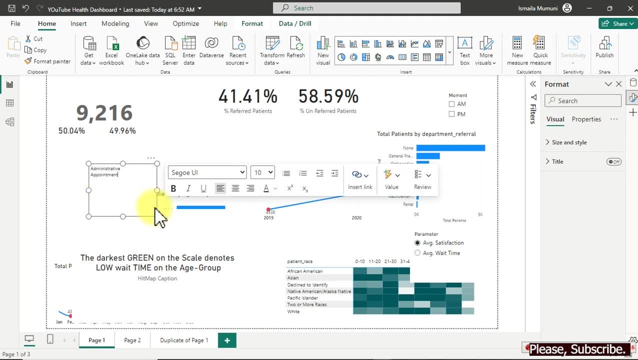 all right, i have this administrative appointment here for you to actually format the content inside this particular box. you need to highlight it. ctrl a will do that for you, so i'm going to push it in the middle. you get that now, beautiful. so now we have this on 14.. then we change this to this: 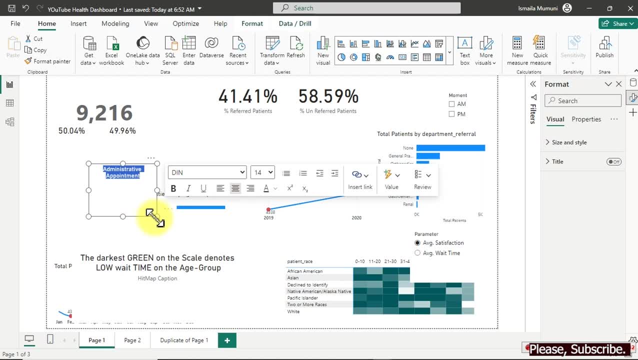 particular kind of font here. so we can now go back to our text box and we can see that we have this font here, so we can go ahead and change the color. we don't want something very dark, let's go with this. so let's see what we have here. so here we go, so you can push this one over. that is broad. 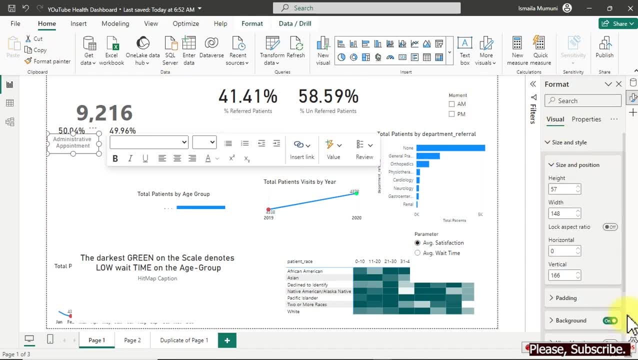 then all i do is to actually go over to size and style here and remove the background i have on it. then it is time for me to copy and paste it and i'm going to drag this one over here. so all i'm just going to include on this one is going to be none. 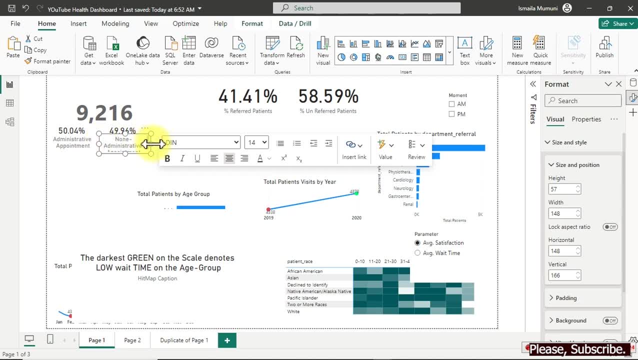 so that is it. so we just stretch this a little bit. so this is what we have. so you look at that beautiful. okay, now we have some three kpis we want to show, and right now you have to be online to be able to actually display that to your satisfaction. 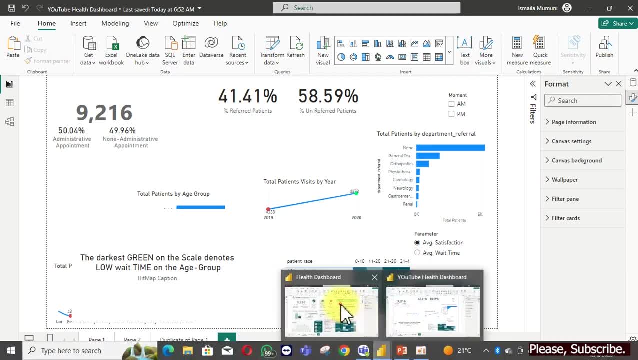 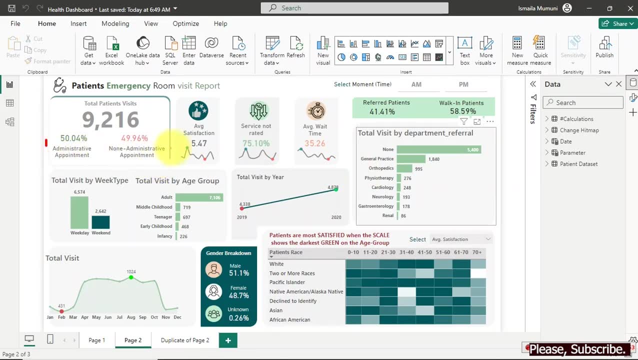 i'm talking about this one right here. so if you look at this, we have this particular part. it's some kind of a custom visual that we need to get. i'm talking about this one here. they are actually custom visuals we need to get from the marketplace and use. so you must have access to power bi. 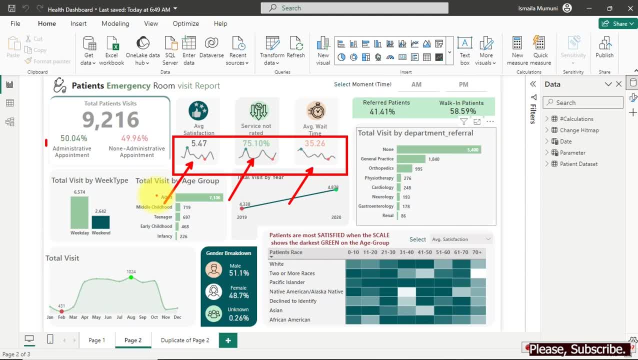 service account before you can log in. if you don't have it, i have a video in this particular youtube channel. they can actually take you to that and see how you can create your own with how you can use it. so you can see how it's. you know, a formal working email. so the very first thing i'm going to do is 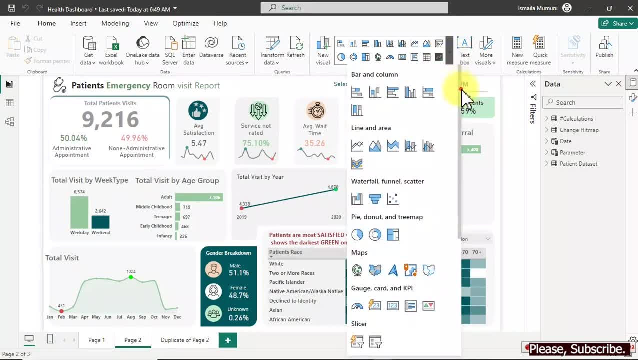 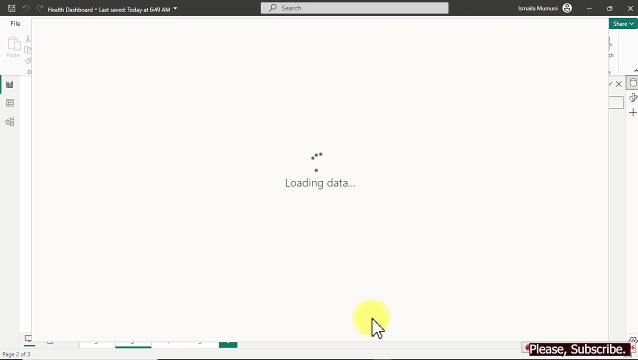 here, for i'm going to go down here. if i scroll a little bit down so you can see, i have this visual called sparkline by okayviz, so i'm going to show you how to get it. so click on this very get more visuals. so once you click on it, wait for it- it's going to open the marketplace for you. 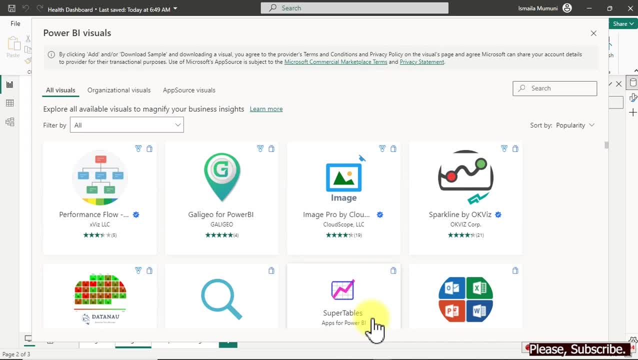 so here we go. the first thing you see is the visual right at the right hand corner. so can you see this? so this is what you're gonna get. so all you have to do is to just click on it. once you click on it, it's very easy, it's gonna. 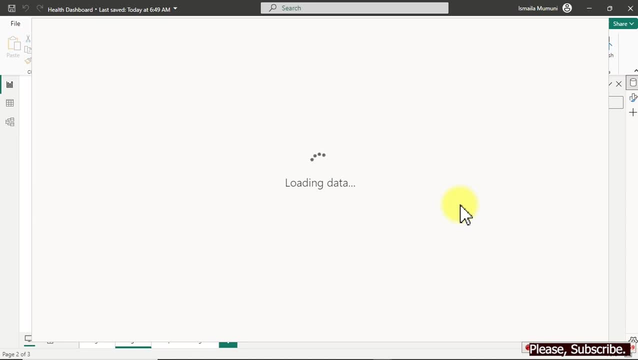 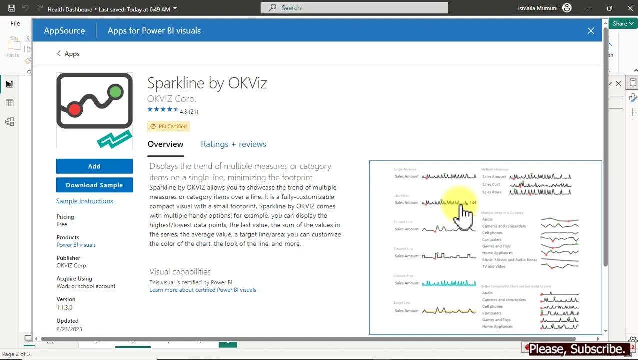 actually move itself to your system by just clicking one single button. all right, do you see that i'm talking about you clicking on add? then it will be added. so if you want to read about it, you can click on the link in the description box and you can see that it's. 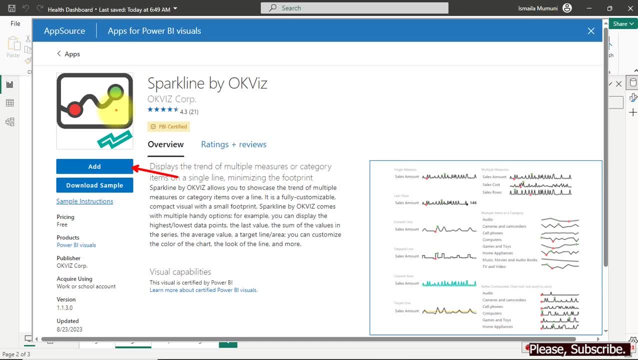 you can just read about what it is right here and see if this is licensed by, you know, microsoft. look at it here. it's 100 free for you. you get it, okay, let's do it. so i'm gonna go back, because already i have it on this visual here. so where we're gonna get it now is on our main visual, on our main. 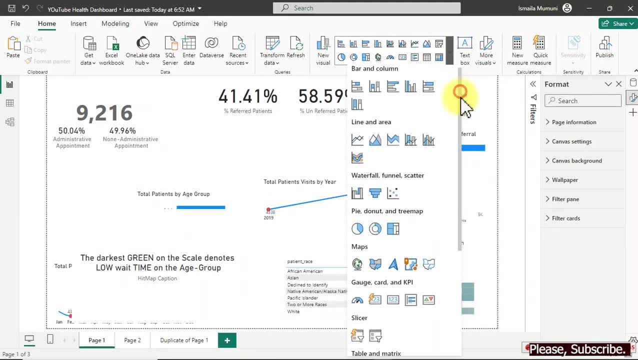 report. this one here does not have it. if you look at it, if i scroll down now, we did not have it here. we need to go get it. so i'm gonna click on the link and then we're gonna get it. so i'm gonna click on. 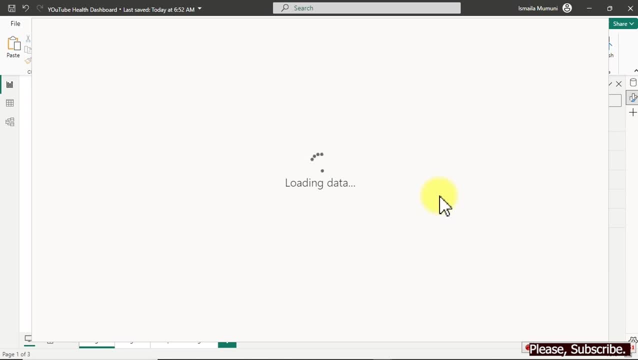 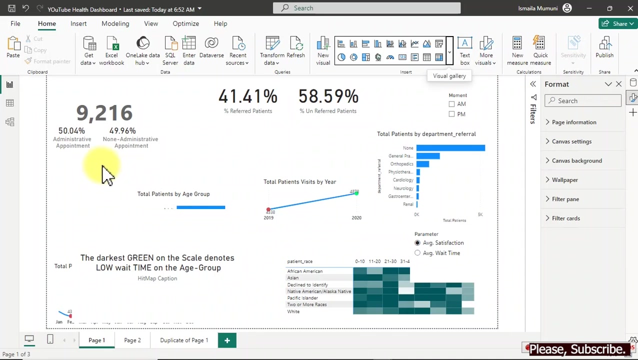 more visual and quickly. the first thing i see i told you is gonna be that very visual. so i click on it. so it's loading, so it has load up, i click on add. that will be added here for me. so now that it's coming up, let's quickly do some formatting before that one comes up. so the formatting i want to do: 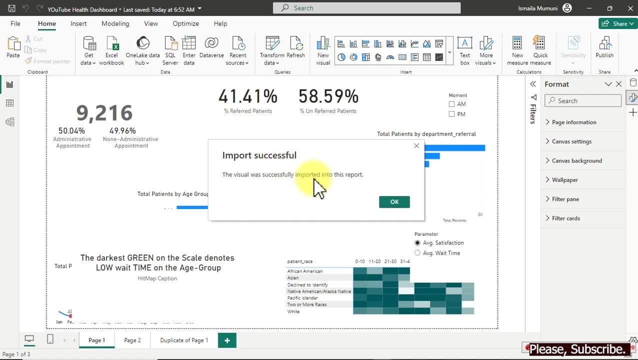 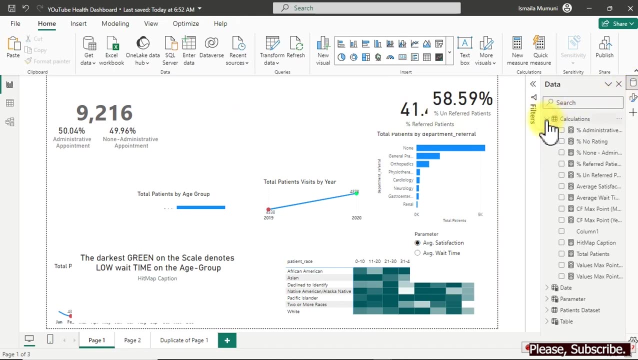 is the formatting for my is here sexually, so i'm going to do formatting for some of the kpis i want to use right here. right, let's come over here, open the calculations and the first thing i want to get is actually average satisfaction, which is this one here. so we have this inside a card, so here we go. 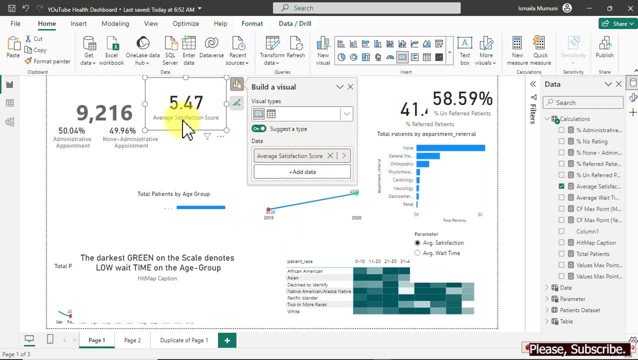 then what do we do to it? we don't want to keep this kind of um, is it title or category label? so i will go over here now. i'll go ahead and find where to turn it off. first of all, the background should be turned off. so we come over here, we go. 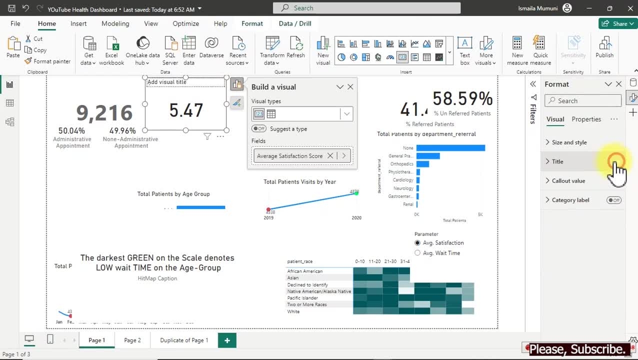 for color. so we turn off this one. then we turn on the title. so once we have the title turned on, we can open it up and what we want to type right in here is going to be a vg, which is a vg here. so, um, it's going to be. 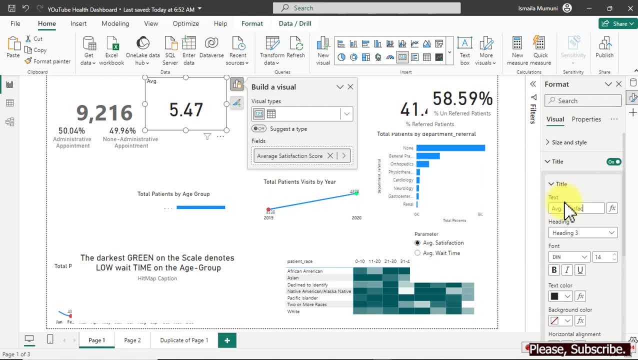 average satisfaction. so here we go. we have this that appears here, so i'm going to push this in the middle right. it's very important, so i will definitely scroll a little bit. i'm going to use this one here for this. i would love to just use something like this color: beautiful. so the next thing. 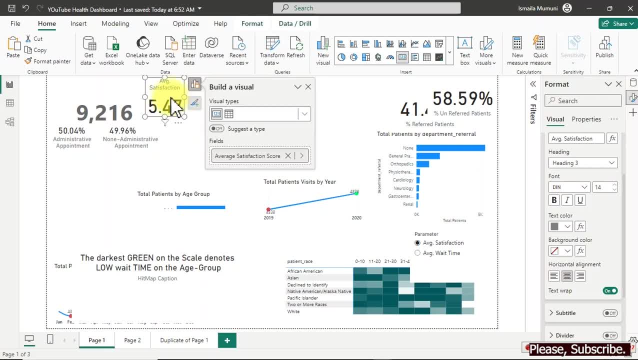 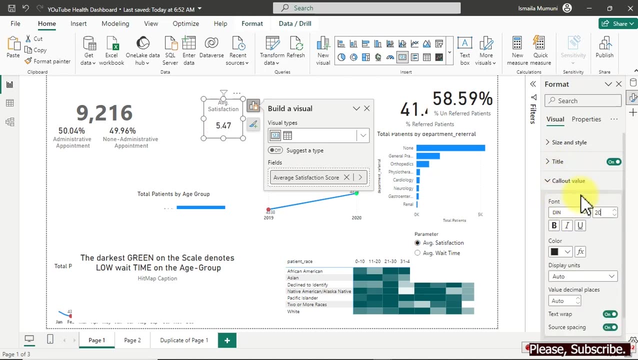 is for me to actually make it until i have something like this. so what about we? looking at how to format this is too bold, so i'm going to actually scroll up a little bit and here we are, call out: we put it on 20.. so you see that then we'll leave it on this one. 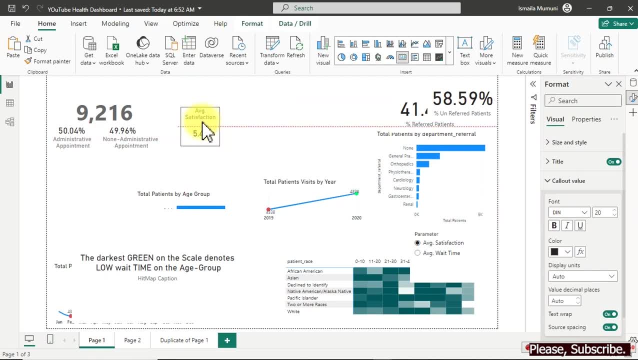 okay, that is it, so we'll leave this right here. all right, i have gotten everything in. so here i have my average satisfaction. i have my service not traded- 75, and here i have the overall average wait time of every single patient that actually visited the emergency room. so this is how you should do a setup. so we are. 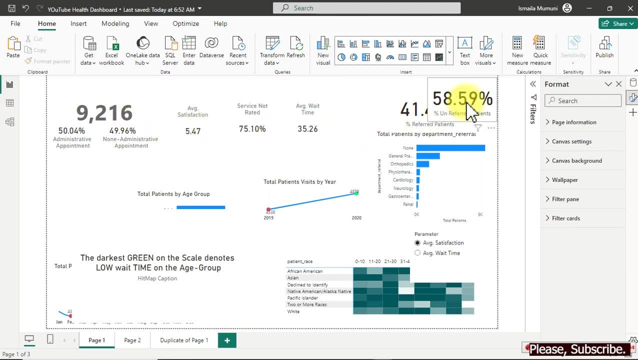 cool with this, let's go into the next one. so over this particular one here. so the very first thing i'm gonna do is to actually bring this and have it somewhere around here for now, for the time being. so we're going to use this, but not actually this one. so we're going to use this, but not actually. 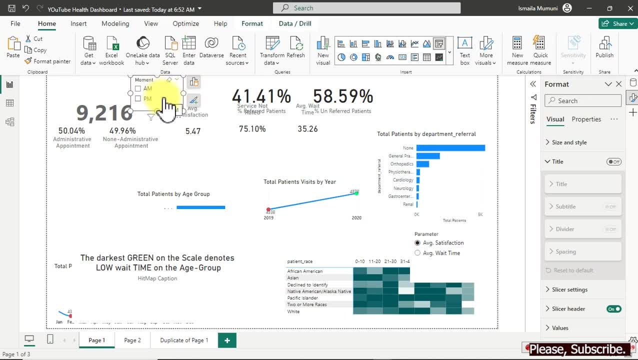 this very kind of you know, slice out. we're going to use the new slides. i'm going to show you how to edit it to look more beautiful. all right, we have this here. the axes are not really cool, so i'm going to go ahead and start changing the axis i want. so first of all, i want to turn off the title. 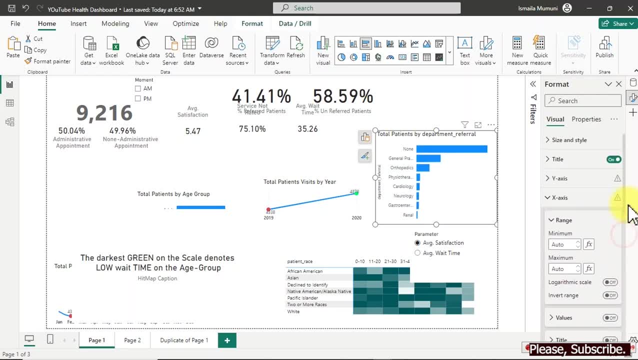 then i'll turn off the value. i don't want that. so once i've done that, that is actually for x. let's do for y, for y, right now. if you look at it, if i try to do this now, this is normal readable. what do i do? let's put this on 50. 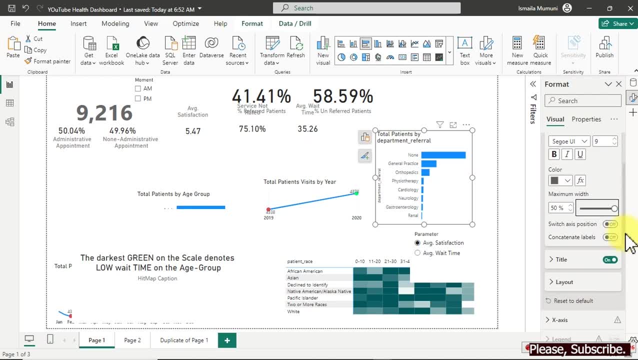 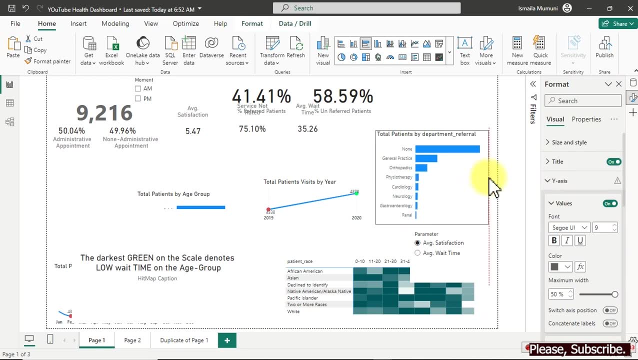 that's, it's cool. okay, now we go a little bit down and turn off the title. it's gone, all right, so this is what it is. i'm gonna just stretch it a little bit like this: i want something like this to be here, so once i have this- uh, for now i'm gonna just 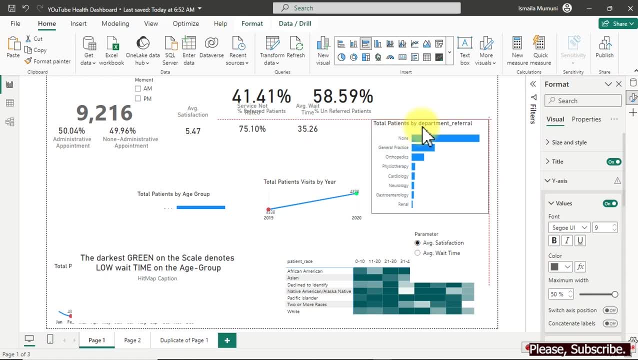 leave it this way: after we brought in our background, we can fix how things should look like, but for now it's okay. so we need to work with this particular one right here. so on this one, we have to actually control how they look and what are the looks? i'm talking about the looks i'm talking about right. 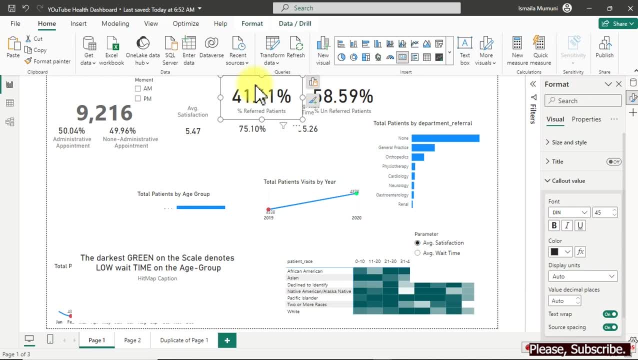 now is actually having it formatted the way it should be. that'll fit into what we want. so i'm gonna come over here, hold your ctrl key to click both of them and over here can actually change again. so i'll put it here with the wheels company and i'll see how it looks like. 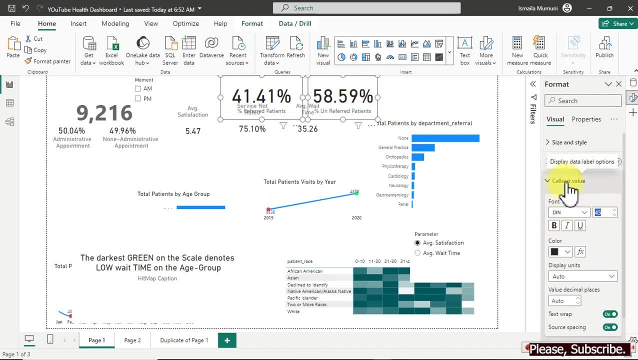 the way it should be. so i'm going to come over here, hold the control key to click both of them and over here you can actually change the game. so i put it in the textbook section on 19 now, making it a bit smaller to fit into where we want to keep it. after that, i just want 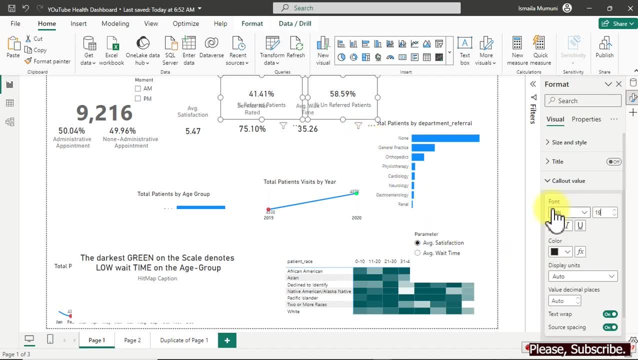 to some kind of um. remove the. you know what it is, so remove this one here. so once you remove it, you might be thinking: how do i remember where i have x, y and z? don't worry, i'm going to show you. so i'll drag this over here now. let it be at this part for the time being. so now for to get. what is this? and? 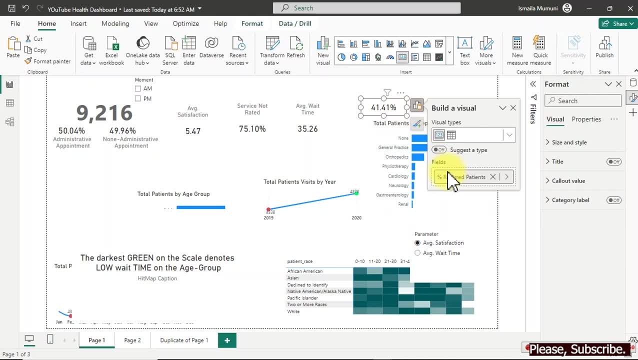 this. so if i click on it right now, you can click over here and this shows you referred patients- beautiful. then if you click over this particular one here, this one shows you unreferred patients. so for that i'm going to just copy this particular previous one we've used, then ctrl c and paste. 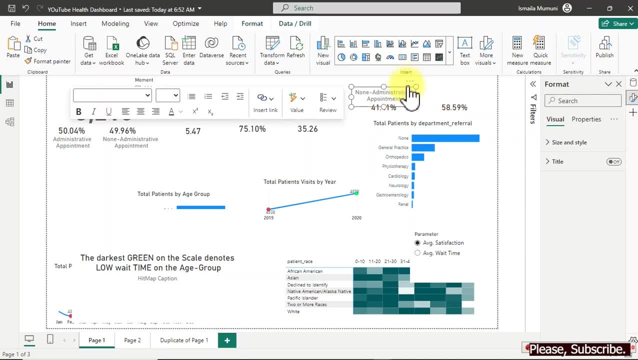 will do that for you. so we keep this one over here and we just change it. so for me to keep the formatting, i'll exclude just few. if you take it out, it will take the formatting you have here already, so you would have to do it all over again. so to avoid that, just select some portion of it and we have one letter. 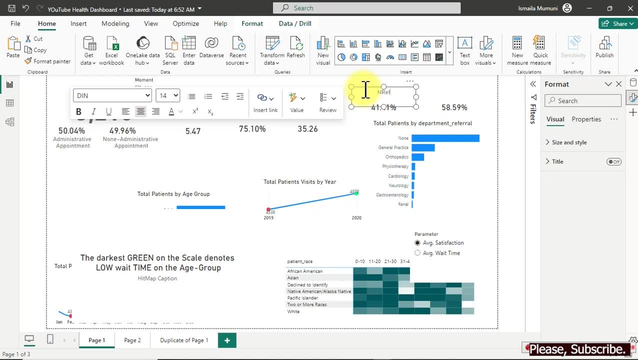 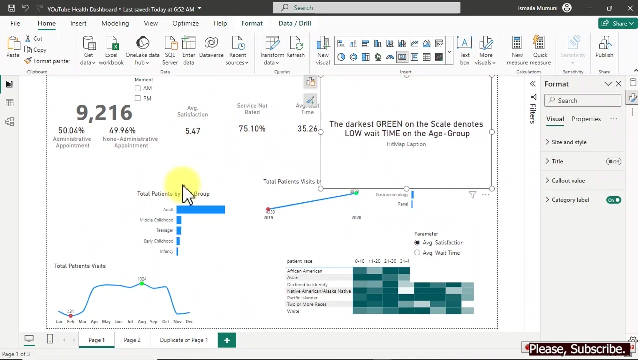 left. so i'm going to just type in here: referred and we keep it right here. all right, we are cool with this right. the next thing now is taking care of this particular part, so i'm gonna move it at the top right here. then i have one more chart to create, which i've never done. 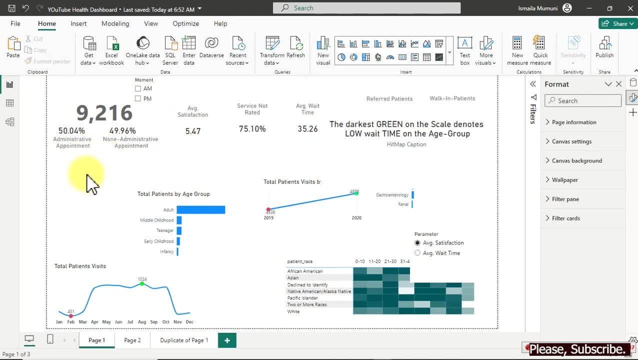 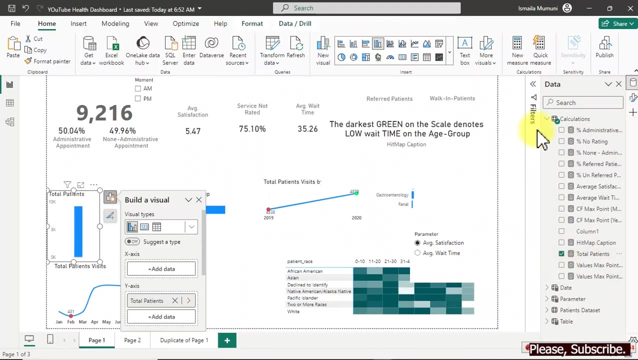 so that is gonna be um, looking at our patient based on type of days, maybe weekday or weekend. so we need to actually add this chart here and i go over here and first of all, i bring in my total patient visit into this chart. then the next thing is for me to go to my date, and i'm looking for that. do i have with type? yes, of. 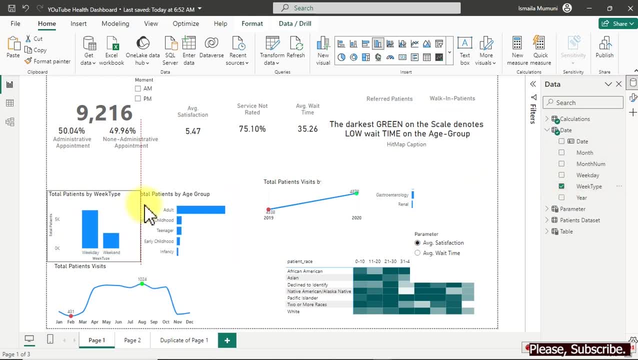 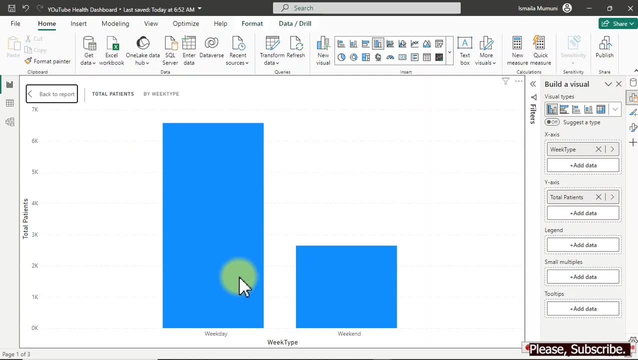 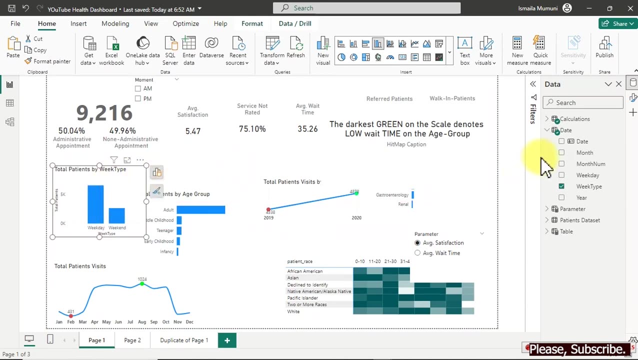 course i have with type. so if you look at what we have here in the week type, so we have more people visiting our hospital for any reason on weekdays than the weekend, beautiful. so now it is time for we to some kind of have this cleaned a little bit. so we just go over here. you know the drill already. 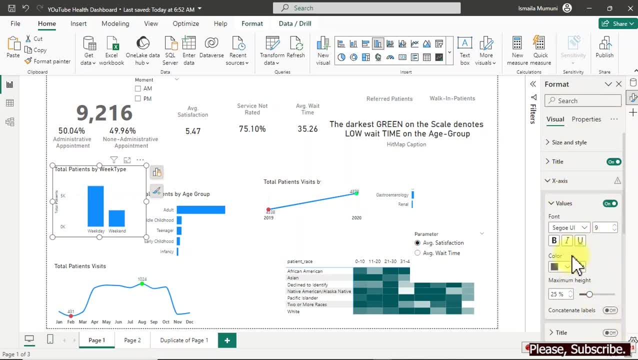 so under the x we turn on the title so we can make it bold to show what it is that we have on it. then i can just go to my y-axis right straight up. then i should, no, not, don't- turn off the value. so my axis here: 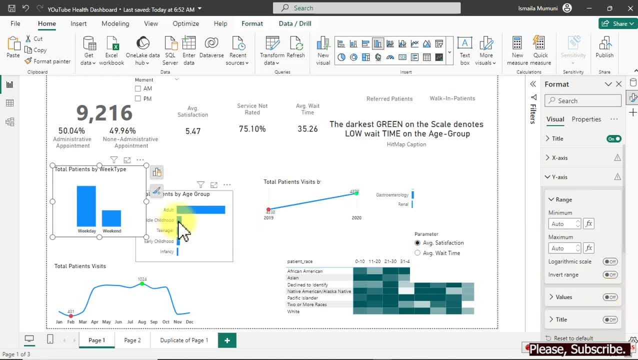 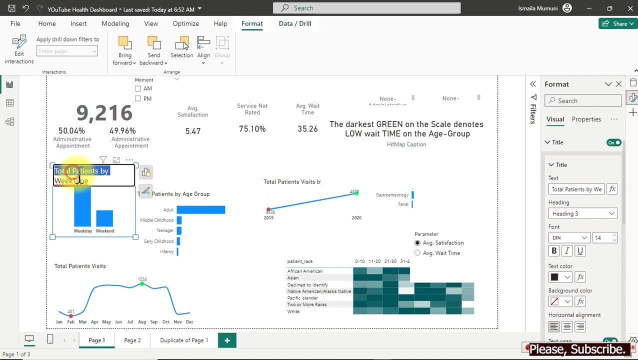 then we turn everything off. we have this very clean. so now to tap patient by weekday? right, we just go ahead and keep this. so if you double click here, it allows you to activate the edit mode. so from here now you can select the part you don't. you don't want to keep. 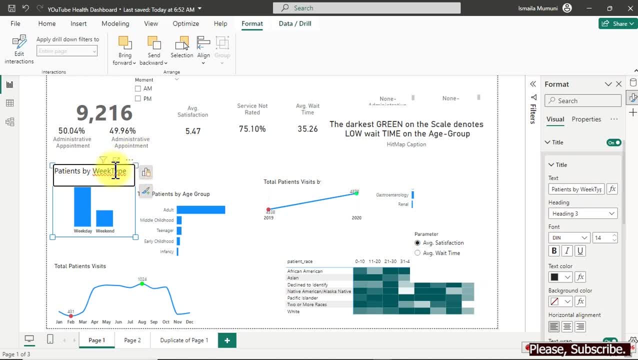 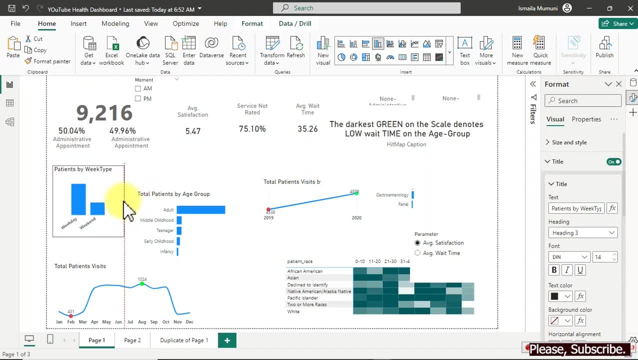 so it's gone. so here we go. i can just go with this week type: i step off. i have something like this, so we can just adjust this a little bit. okay, we go with this. so on this, it's gonna be here and i'll just stretch it a little bit down. 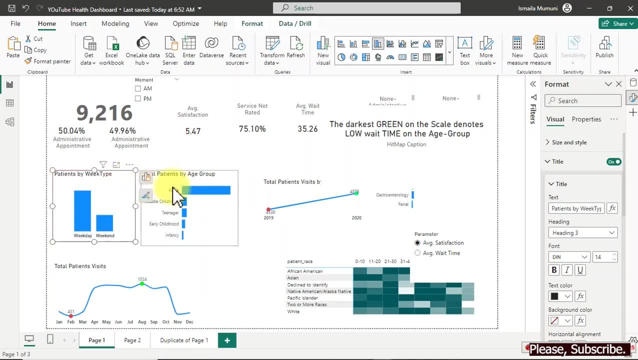 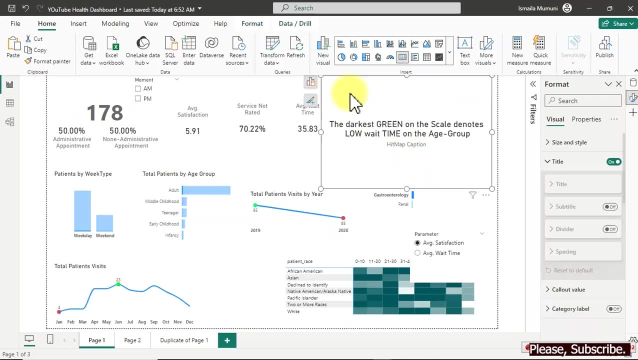 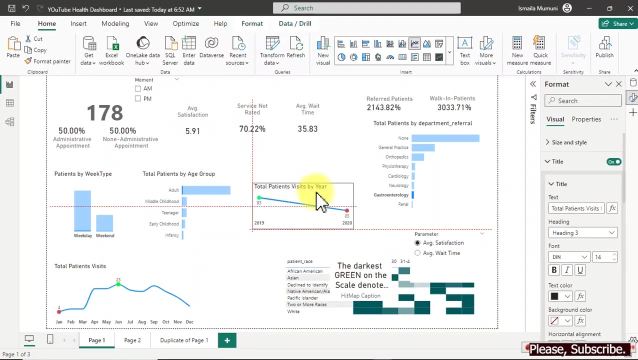 so we just do a rough walk for now. this is what it is, that we have. all right, we have a line chart here. this line chart is gonna be here. let's make this smaller and keep it below here for now. then our line chart looks pretty well. staying here, that is nice. then over here we have this. 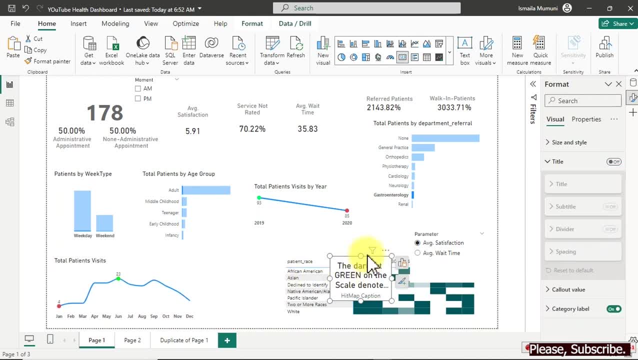 the marked zone thing here, and on the right hand of the axis we have the 작별, and that's for the text added over Gravitas. now this one will just be considered a às'd foundation, so this will be a handle when we go over to actions. 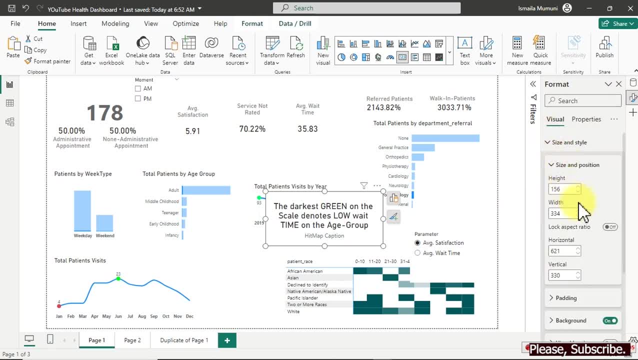 topién than i have the on this one. we just need to make it a bit smaller. that will be readable. so we'll have to format it so we go over to this no background and we turn off the category label. we come over here, we'll put it on twelve. so twelve, you make it bold, so we select all three and we save the four from the vor겠�ering made before us and we select the 아니면. so this option is stereotype. so maybe if you have a body box that allows just some space to print from a child on the table, 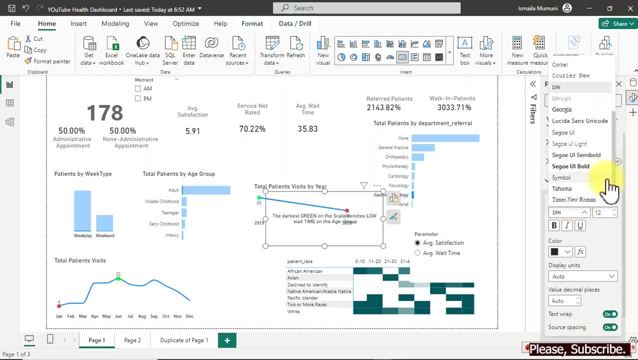 setting up infrastructure, which would be helpful for us. then we can go down to the top right hand side. it bold, so we select a bold font for this, right for the color, don't worry, we fix it later, so i'm gonna keep it right here for the time being. so on this one here i'm gonna have to change this. 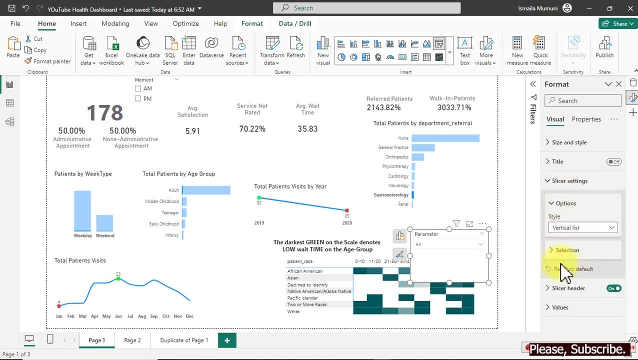 one to what? change it? to a drop down. so here we go. so the drop down wouldn't have header. don't worry, we'll see how we can indicate it. just make it a bit smaller. now we can see what we have in it. so here we can just move this and have it around here. 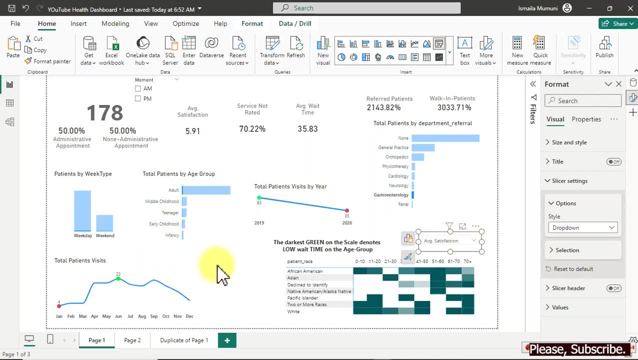 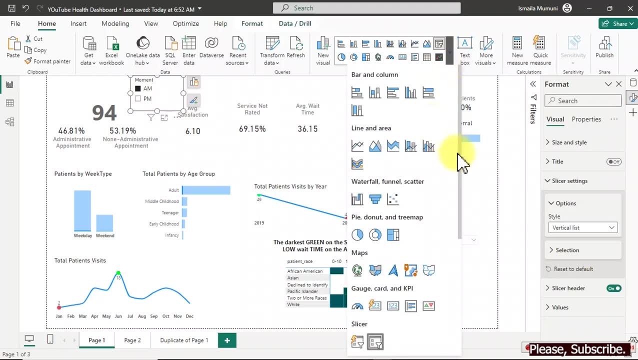 you see that nicely done. okay, now, if you look at it, the settings are almost done, so exclude this one. so, on this one, what i'm going to do right now is to actually go ahead and use the new slicer, which is this one here. so it looks just like this. 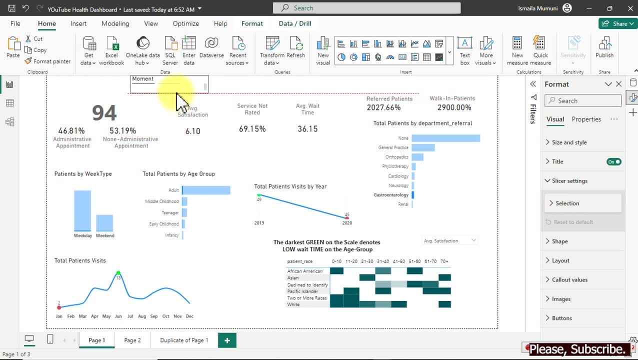 we have to stretch it before we see what we have inside it, so i'm just going to make it a bit smaller now and forget it somewhere around here for the time being, while we actually correct others. all right, so over here we have a card. what this card contains is actually the percentage of 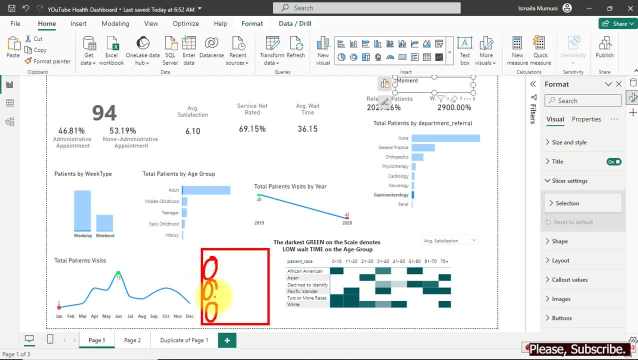 the male, female and the unknown gender that we have right here. we don't know if they are she, female or i don't know, in a sub-country project, some kind of you know, i don't want to go there, so we just want to do something like that. 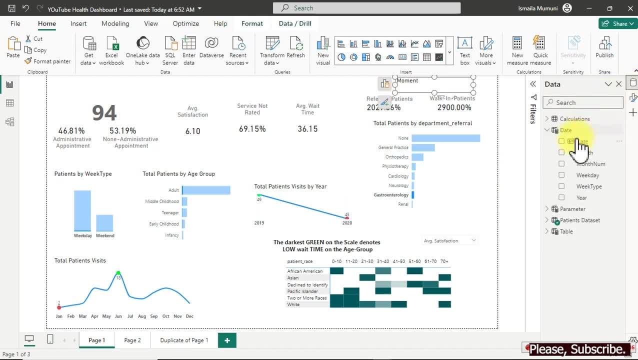 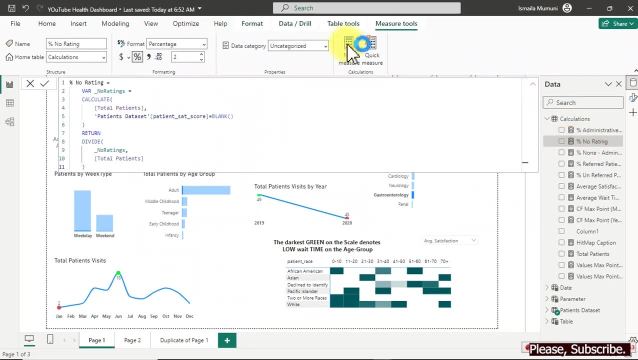 way, though, very simple. we're just going to write a DAX that extract for us the percentage of male and female, and it's something very, very simple. you can pause and write it yourself, you know, test it and see if you can. that is good, so good development. so what do we do? have you done that? all right, i'm. 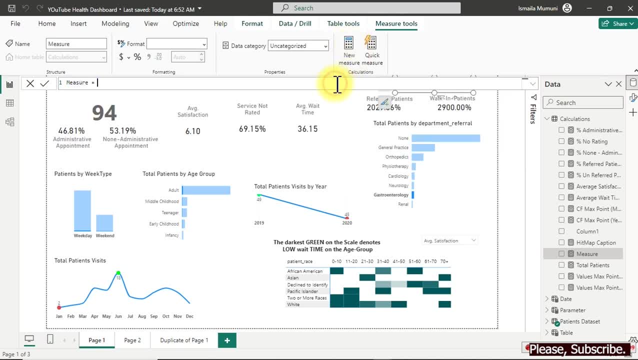 going to insert a new measure. so inside this new measure here i'll call it percentage male visit. so equals here. so what i'm going to do quickly is just for me to say i'm going to divide, so divide here, so inside the division. so what i'm going to do now is i'm dividing. 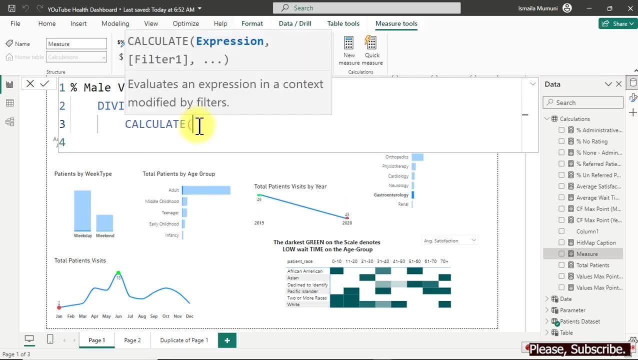 and once i divide i have to use my calculate function to only filter the ones i want. i want for male, so i put my total patients visit here and i try to actually go for gender. here is my gender and i say where the gender is equal to male. 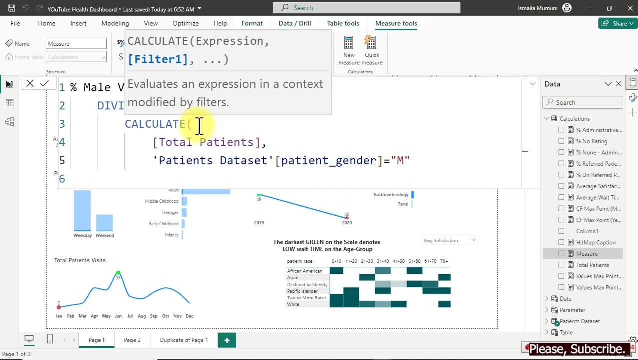 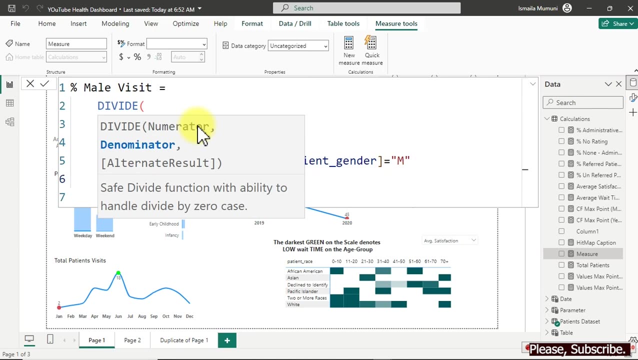 so m for male. so make sure you know this column- that is actually m for male- before you do this, otherwise it wouldn't work if it is male in m a l e. so once i'm done with this, now i can actually go ahead and close this and i'll place my comma for denominator right here. would now be what? 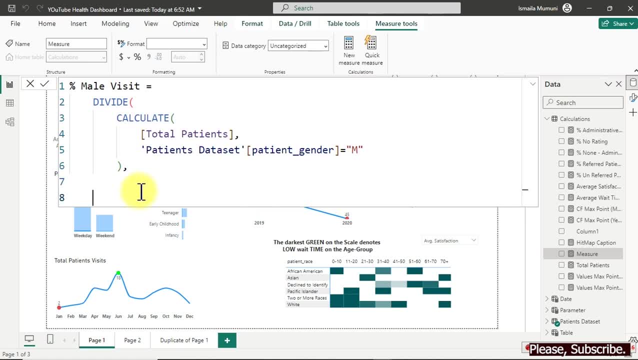 so we'll now be dividing this by the total of our patients. you know value, so which is going to be total here? and i'm going to close this. this gives us the percentage, so you can decide to store it in a variable first and do that. so it's only choice. you can do it and 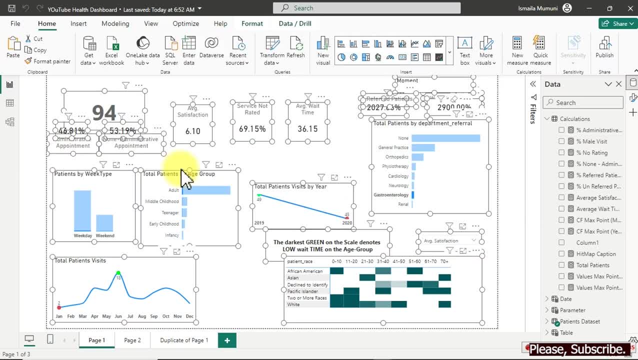 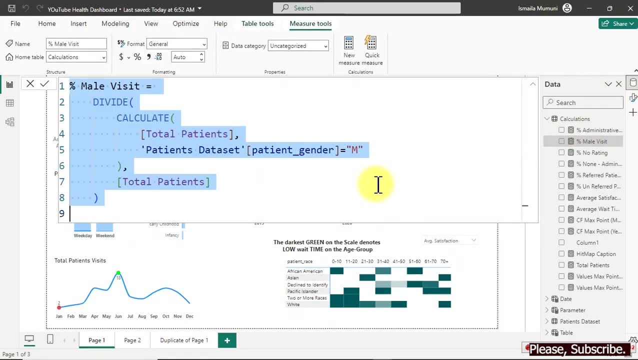 how you like, but right now we've done this all i just. it's all a little bit complicated, but i'll is to do now is to: oh sorry, did i just step off? so now i want to copy this and after copying this, i'm going to change this one into a percentage. so, with this one changed into a percentage, we 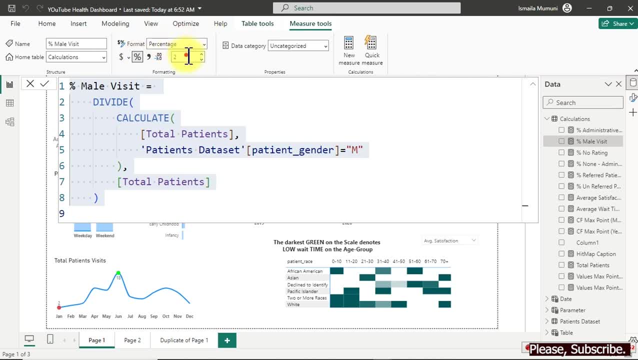 have to decimal places. i'm going to remove one of it. come over here and just do one, and that is cool. then the next thing we have to do right now is to copy- sorry, yeah, we've copied it- is to actually create a new measure and paste the copied one, then change what we have in it. 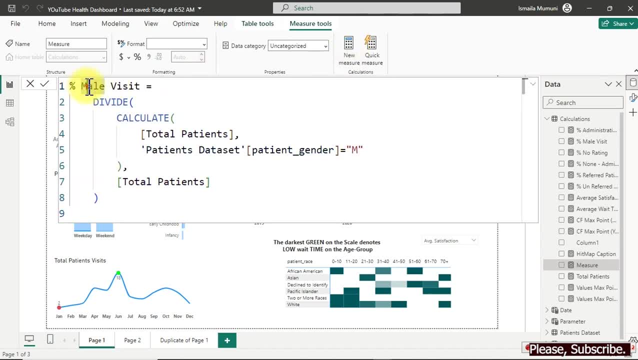 so we have to change this. the first change here is making this one what female, then. the second thing now is to change this one to earth. that is all we have to do. then we convert this one to what? to a percentage as well. okay, before we do the 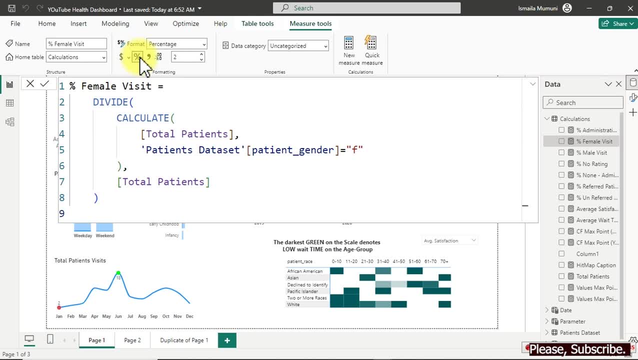 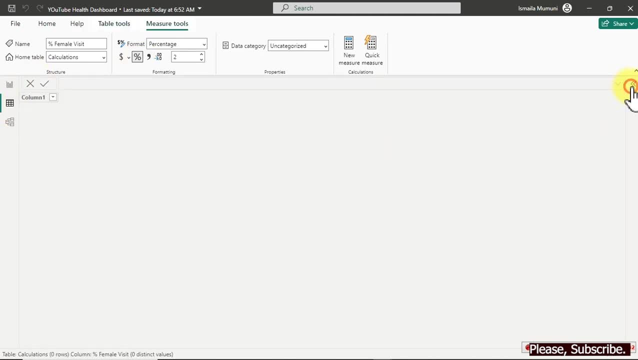 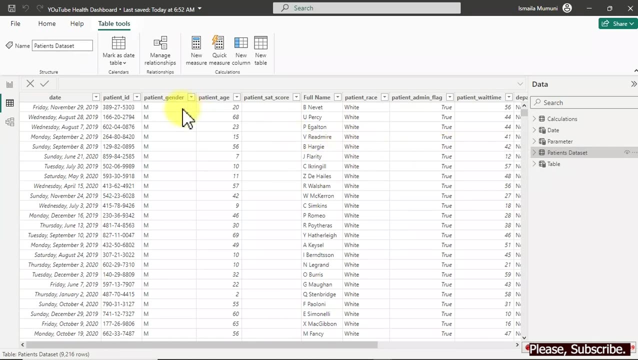 one. i'm going to show you something. i don't know why that is there, but i think the health center will know why they have that there. so if i go to my data, i click over here and i go straight up to the patient's data set. right then i locate agenda. 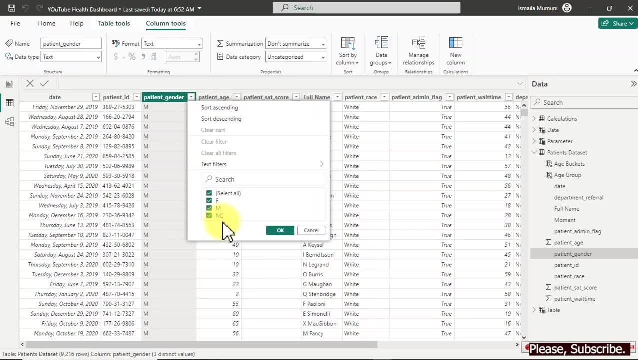 inside agenda we have this nc. i don't know what nc means. maybe nc means something like people practicing. you know what i'm talking about, so i don't want to call it, for you know, for youtube, uh way of doing your own uh rules, and all of that. so we're gonna get strike. so now what i'm gonna do? 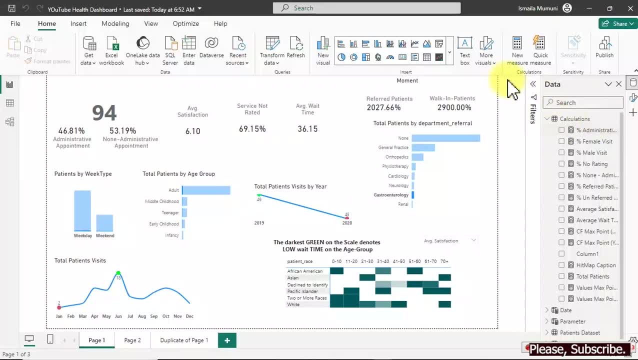 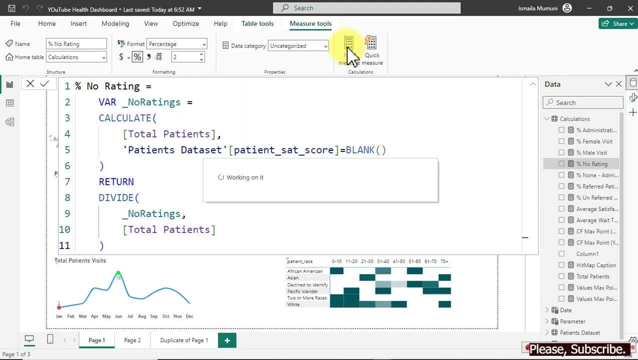 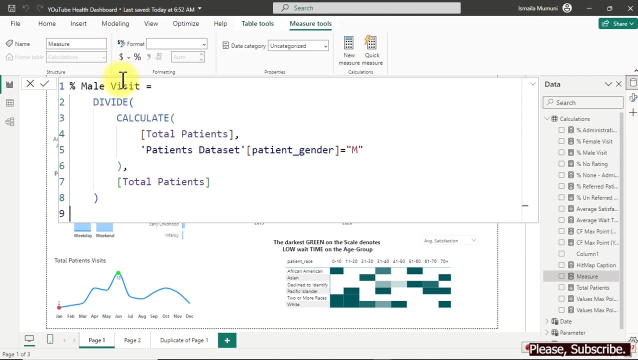 right now is to go over here and i'm gonna do the same thing. so by creating a new measure, so new measure, so with my new measure right now, i will definitely paste this in and i will just highlight here, and i'll put unknown so over here, that particular nc we saw there, we put in there. so we have just done justification. 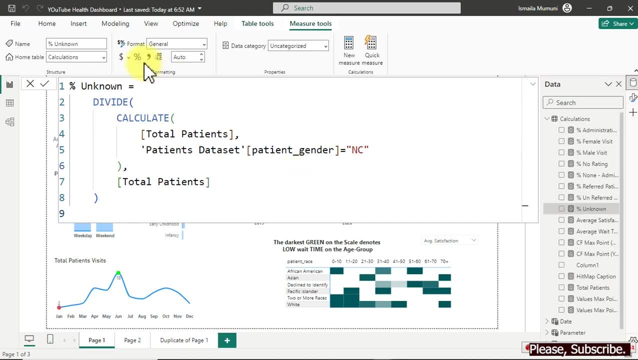 to it. so now we convert this to a percentage, don't forget to use one decimal place instead of two. i think we've not done that on the other one. all right, so female percentage of male or female here, i'm just gonna do this. all right, we have everything we want, so it is time for me to bring them in. 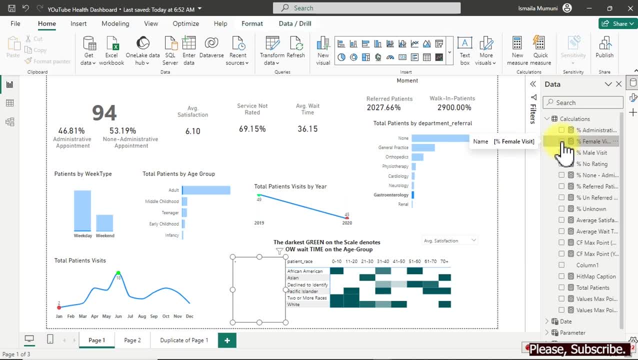 so the first i'm gonna do is to bring in ladies first. okay, here is my female percentage. so i've got my female percentage. the next i'm gonna do is to some kind of find a way to format it and make it look much more beautiful on what we are doing. so what am i gonna do? i'll go over here. 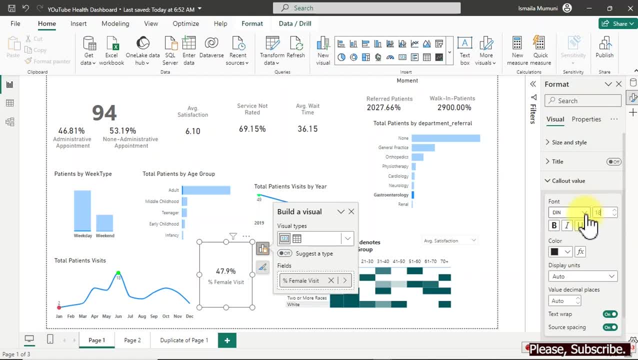 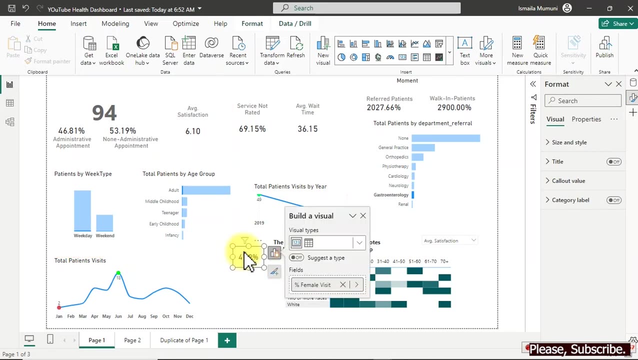 i'll go for 18 beautiful huh, so i don't actually need to keep this. i'll turn it off. so i'll do this and i'll keep it somewhere around here. so all i just need to do now is turn off the background first, so we just copy and paste. 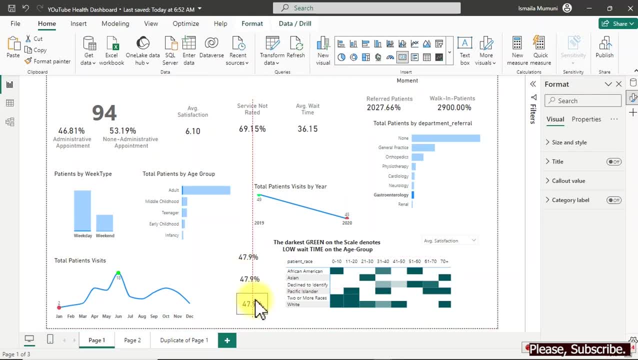 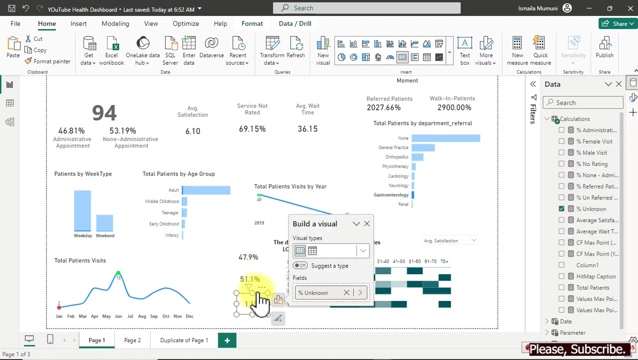 twice. so we have this. on this one, i'm going to change it to mail: mail visit. so on this one, we're going to change it to unknown percentage. oh no, we have to select this first. all right, we have everything we need right now. okay, this is what it is. what else it is time for. 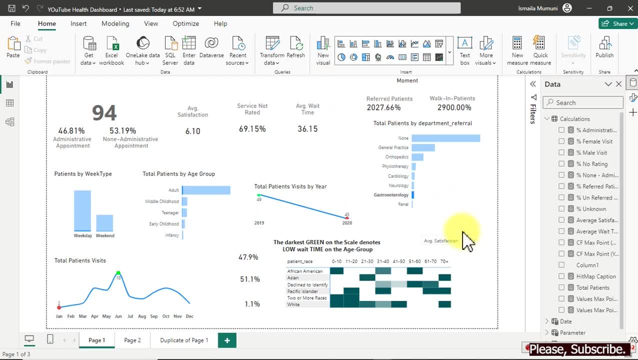 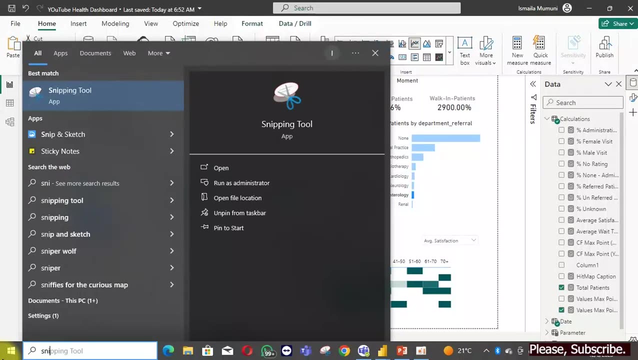 we to start to get things much more interesting, which is getting this right inside our powerpoint. so what do you do? just go to your windows and search for snippet tool. here we have it, so just hit it in the key. now you have this aid here to have this. 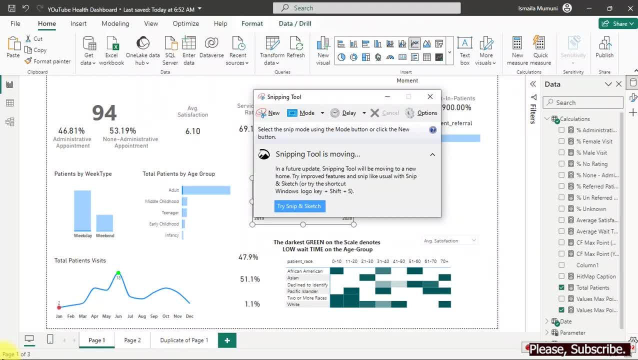 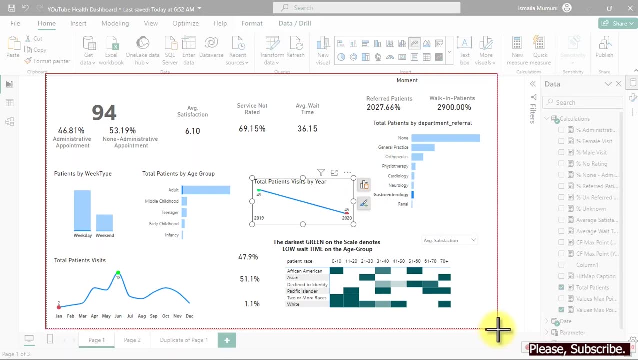 bugün Meeting Brands here to help you capture your screen. so we're not capturing all the whole screen, we're just selecting some portion of the screen and i will do new from new. i'm going to select this particular part right here and i'm just going to cover it up to this end. you can look at where i just selected. 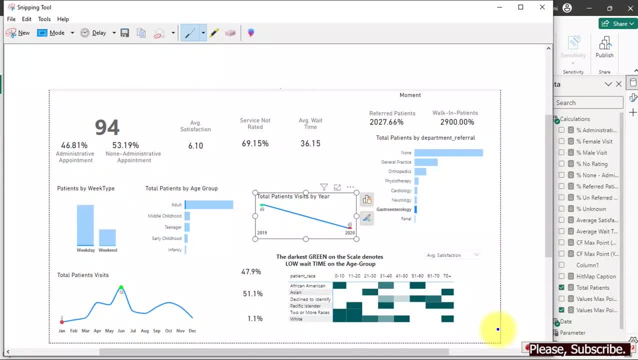 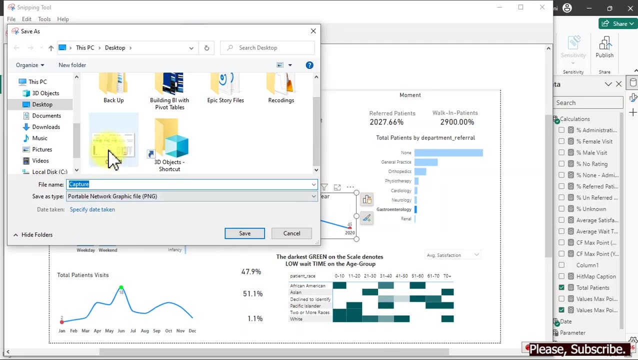 please make sure you do the same thing to have the same thing i have right now. so this is what we have. what do we do next? we have to save this somewhere. and why is there? let's go over to file and say: save us. then we just save it anything we like. so i already have this saved. i'm going. 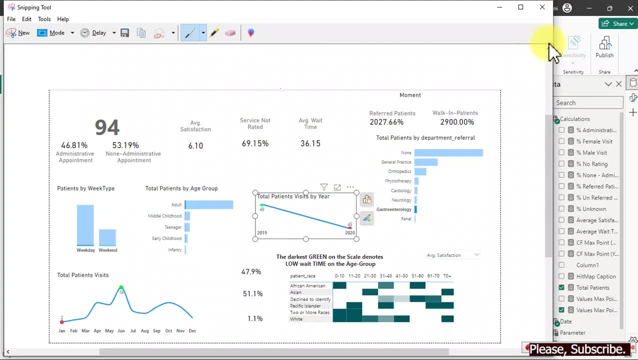 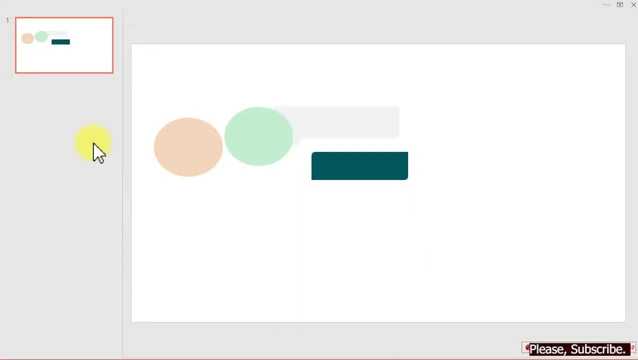 to replace that and pick it from there. so good to go. we head up, straight up to our yeah powerpoint. so i'm going to insert a new slide so you can inside insert new one. then here we go. we'll remove this the very first we're going to do. if i go to the top ribbon, 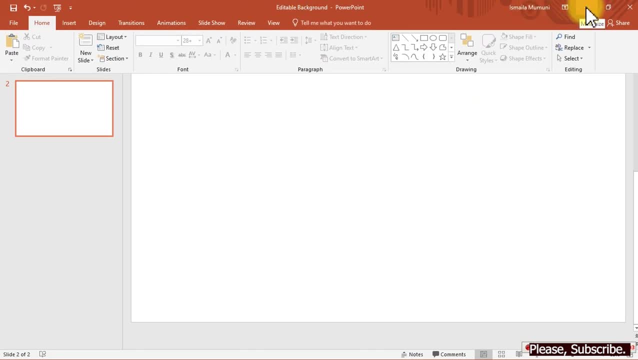 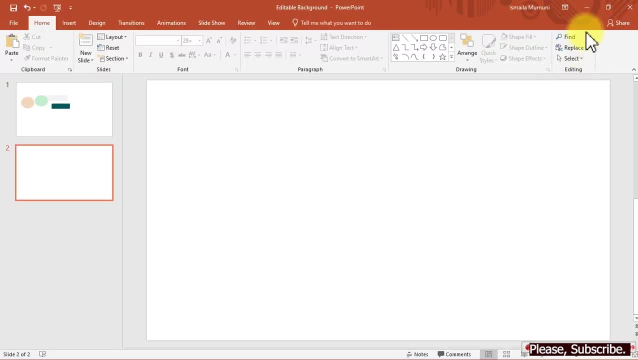 going to be show tab and you have this. that is beautiful. so i always love to keep this auto and that way. anytime i need something, i go to the top ribbon to pick it up. so right now i'm going to click on insert, so while inside the insert i want to go for pictures and from: 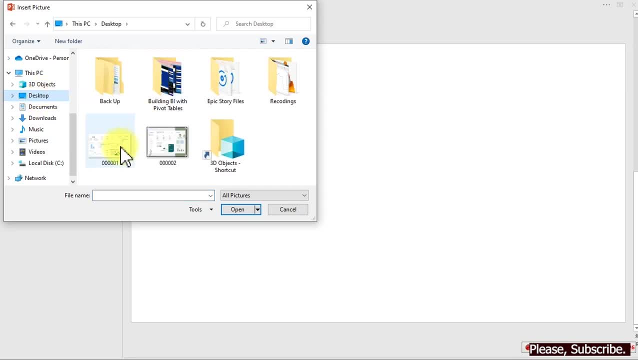 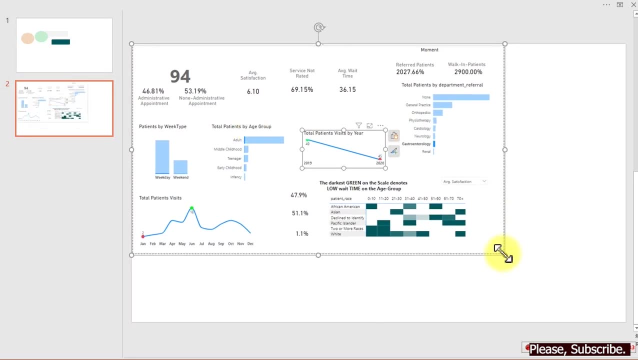 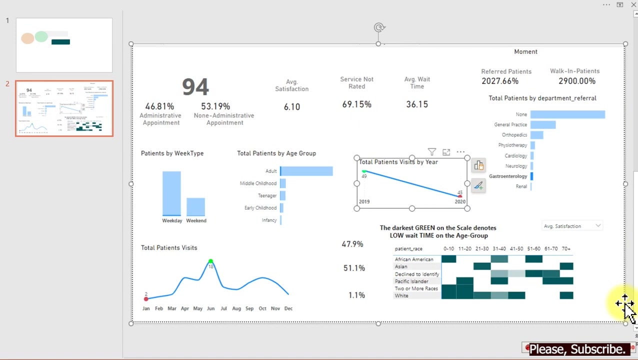 pictures. i'm going to bring in that image or that screenshot, which is this one here. so we have this. fit it into here and just look at what i do. fill it in. so we've just filled the empty convert. it's what we have. so what do we do next? it is time for you to start working with this. the very first. 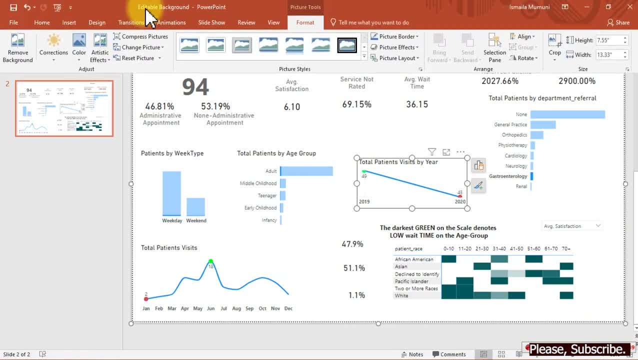 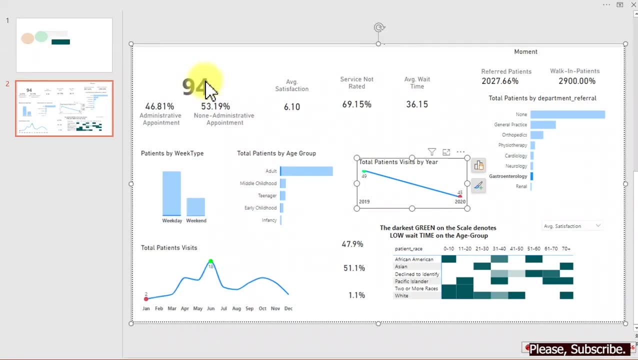 thing i'm going to do is to actually go up again and go to insert. i want to get a shape, and the shape should be the one that has this particular curve. then i'm going to drag it. can you see? so if i do this now, i wouldn't see what is behind it. so what i need to do now is to right click. 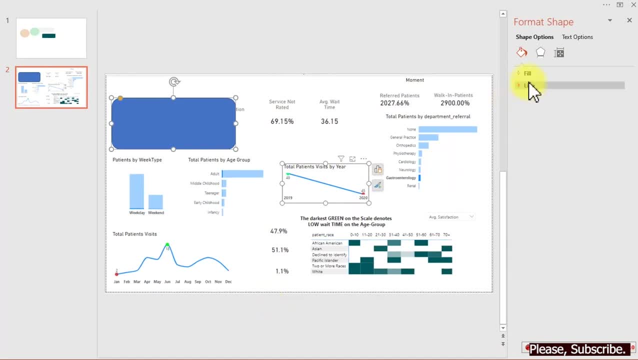 and go to format shape from format shape. i want to do no outline, then i'm going to go to fill. i want to select what. i'm going to select my color, but i wouldn't go with the color for now, i will, just the transparency that gives me what i have behind it. then i can control what they see, okay, so 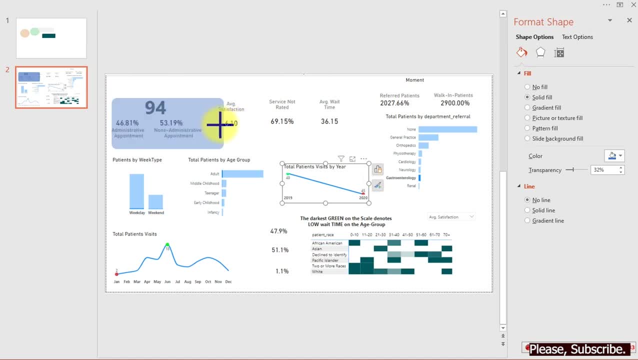 you can just do this and I will do the settings this way. I'll make sure I pave way here. so let's bring this a little bit. so I'll just extend this down something like this: so we're going to work with this. let's bring this down a. 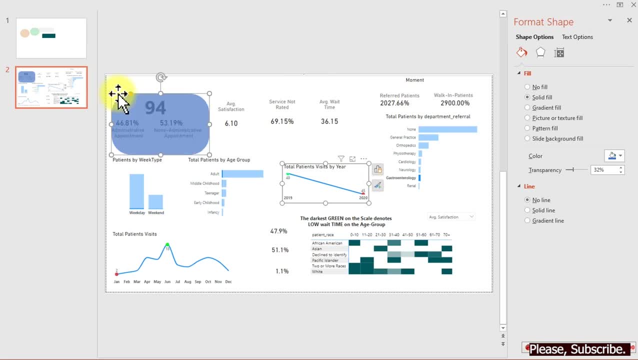 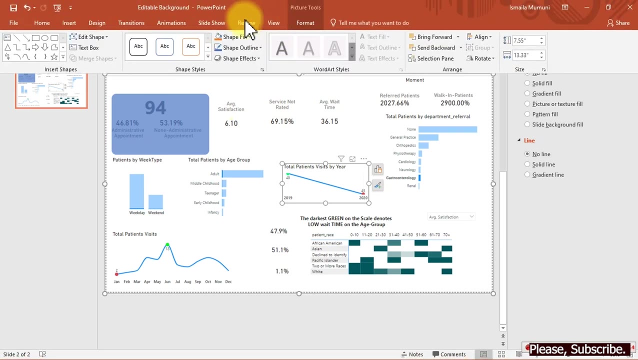 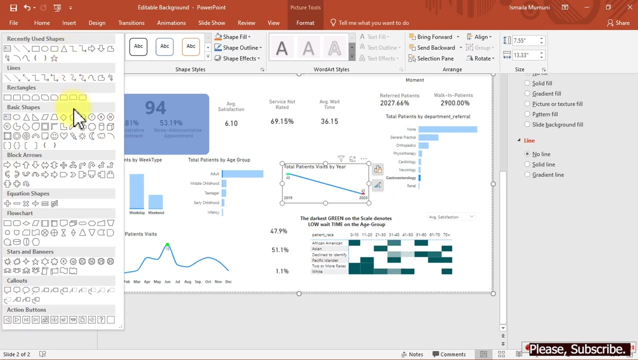 little bit. all right, we have this, so we're done using this particular one here for now. what else we want to cover these three KPIs here? so we go back and now we select. here we're looking for one kind of shape. where could we find it? 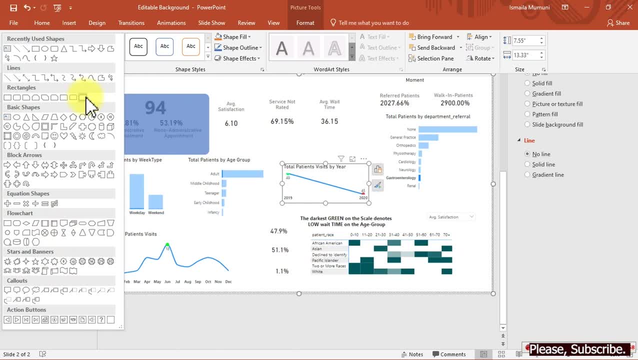 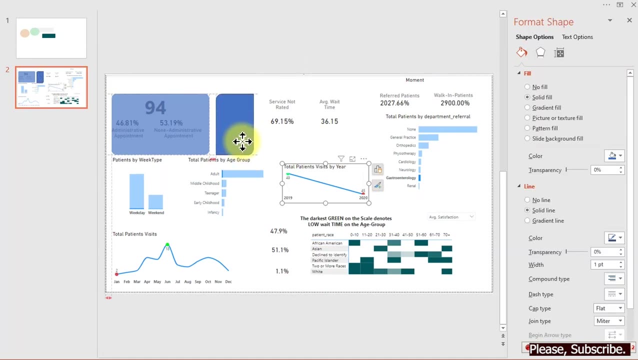 let's look for it. let's look for it. all right, look at this shape under rectangles. if I hover over this one now, it says rectangle, diagonal corners rounded, so I'm gonna click on it. so, right here, this is what I have, something like this, so this is what we. 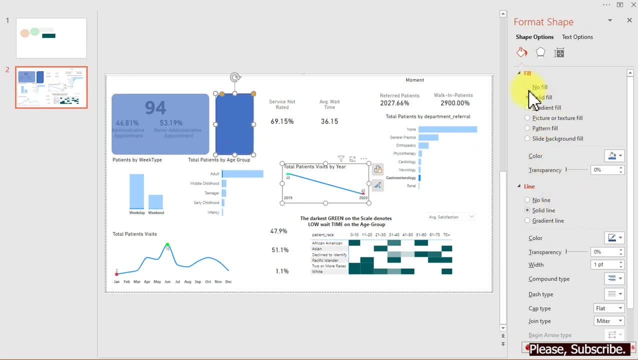 want to use. so remember what I did the other time, so I'm gonna turn off this. so now we just make it transparent so that we can see what is behind it. so we want to get something like this size under rectangles. so we're just putting in this small rectangle tip in here. let's. 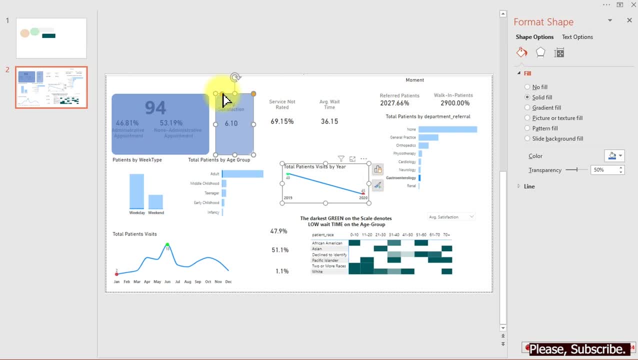 to double it, and it's beautiful. if this corner here is not really cool, you can hold this place to readjust it. so watch one. all right, now I'm gonna go with this. the next thing I do- duplicate of it. I bring this over here. I haven't a. 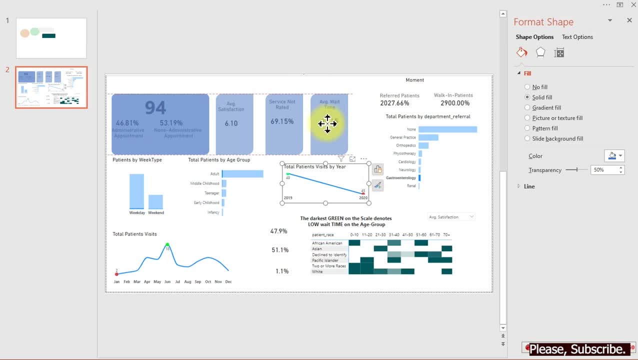 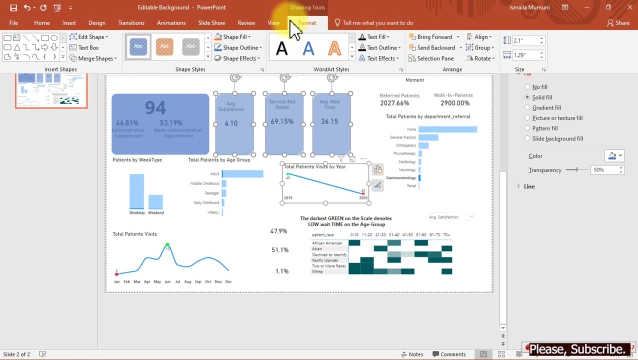 duplicate of it. I bring this over here so it can just make sure I move this. this is the space I want to have it. let's move it a little bit so to have equal spacing. you just go over over to the top. after selecting both of them, you go to align and you distribute horizontally. 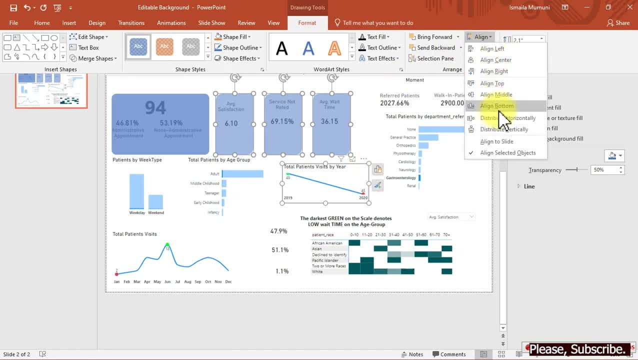 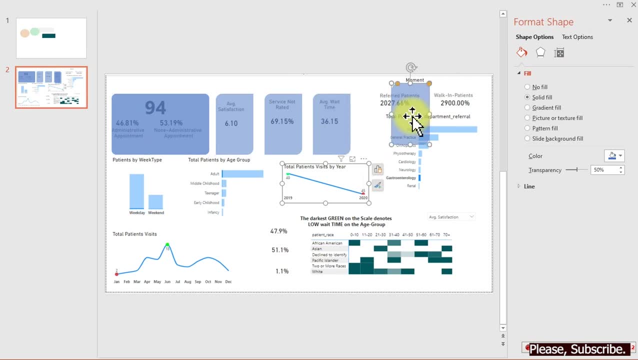 you get it, so you can align this one to the top or to the bottom. here we go. now we have this, so i'm going to get this one and i'll come over here. i'll give it to the top here, so i'll make sure i have it on the same size. so let's do this. i'll stretch this to this end. 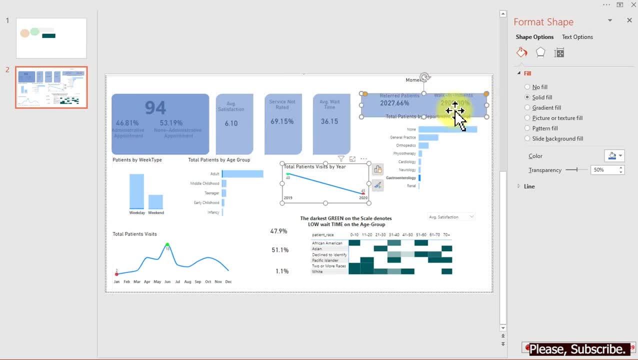 beautiful. now that is done. so this one here. i'll duplicate it and i'll bring it over to this place. so i'm going to create a space between this and my card, so i'll just duplicate it and i'll bring it over to this place, to this, and i will bring this down. 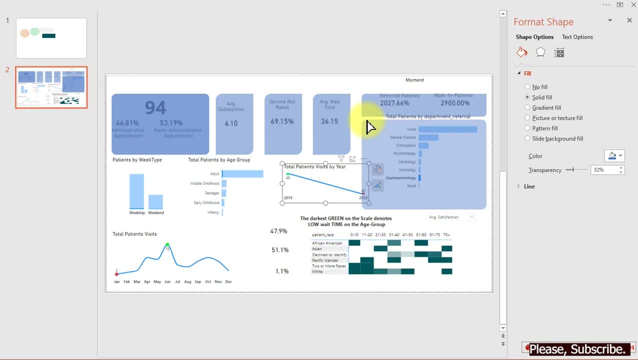 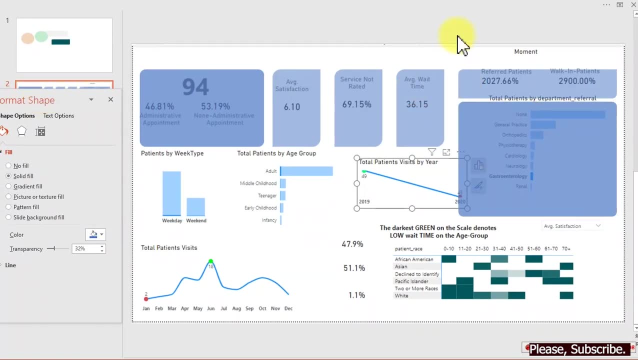 just like this. so the curvedness is too much, so i'm just going to reduce it by holding this. remember, you can move this to give more space, then we can see better what we're doing. so here we go. so once we're done with that, i want to just get the same thing duplicated over here. 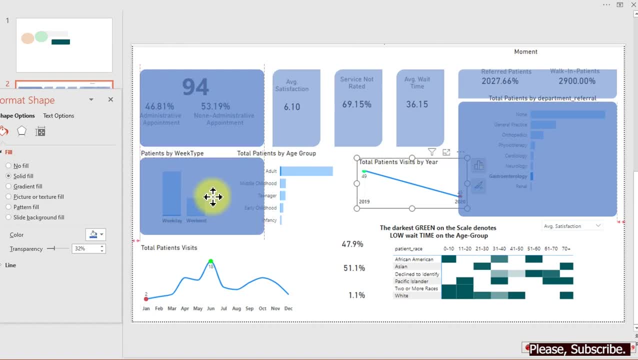 then i bring it up to this part. so, bringing it up to this part, i will maintain this and i will just adjust it to this level. so here we go. the same duplicate will come over here to create this for me, so you can use your arrow up and down, left and right, to adjust things the way it should be. 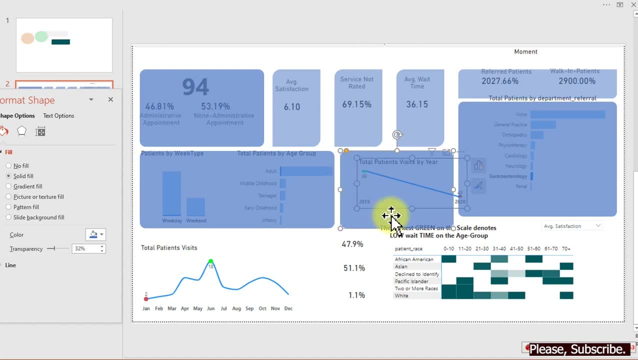 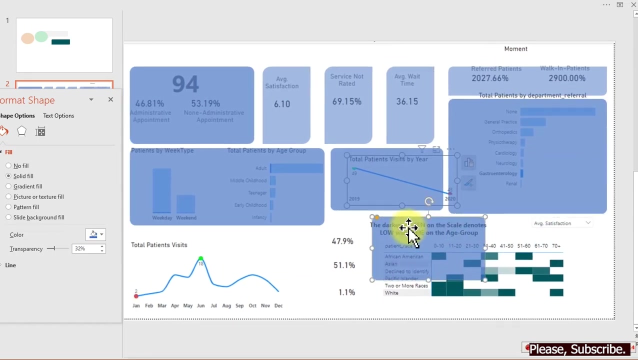 and now i have a good thing right here. so once we have this, i would love to just take this up a little bit like this here. i want something as small as this. so you can now see, i have this piece here. the next i'm gonna do is to just do this copy, and this copy would come over here. 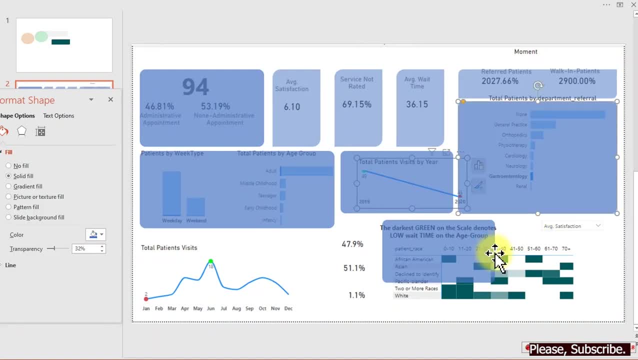 whereby i'm gonna move this one to. i resize it on this, then click on this one. you'll go this way and always keep a white space. if i talk about white space, what is white space? the white space is actually the space between here here, here here, and the space between here and majorly. 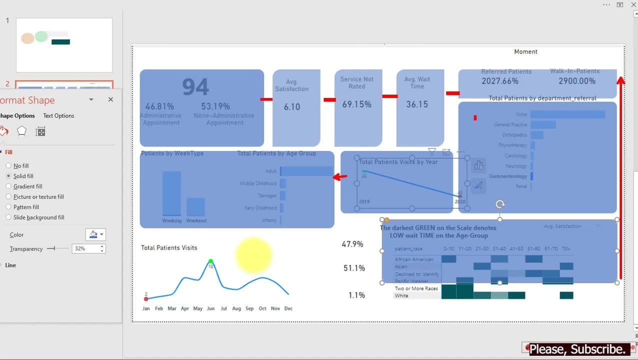 the space that you leave before the edge, and the one at the top right here is absolutely important. with the one that you're gonna have to put at the bottom, it's gonna make your work to look very much. you know, cool, right, you need those spaces. okay, now we have this, i'm gonna actually extend this down. 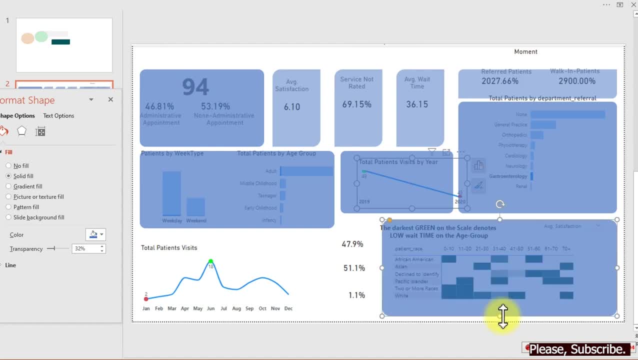 so i talk about spacing, so i'm gonna give a space like this. you get that. so the rounded corner will be reduced just this way. so once i've done that- now i will do under copy again- i'll bring it over here. then what i'm going to do is to just 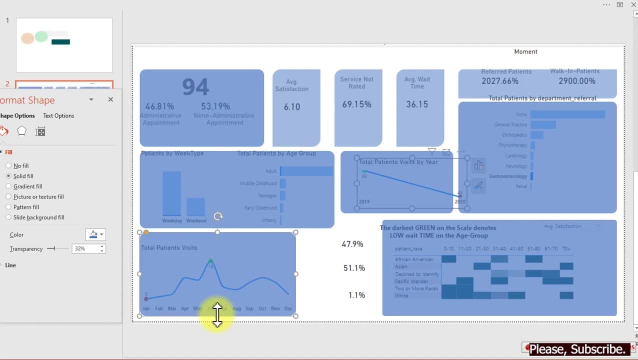 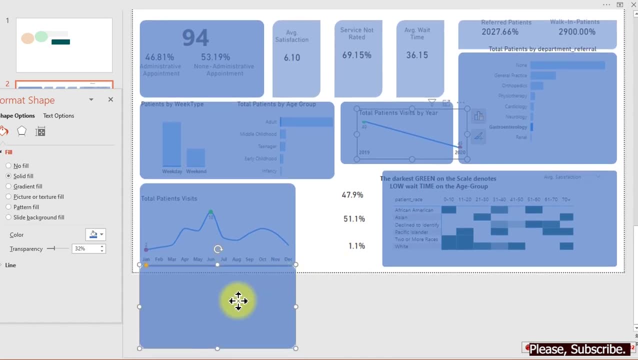 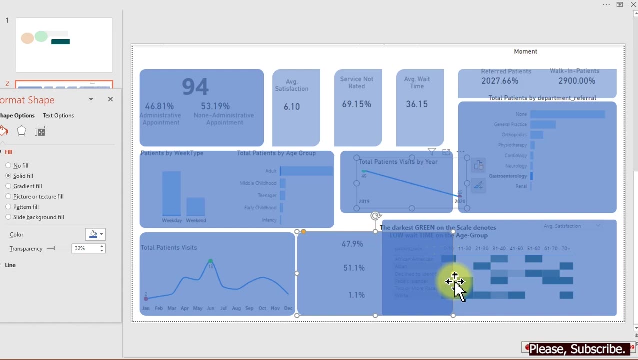 resize it and i have it this way nicely done. so i have this piece in between here, so what am i going to do to it? so it is time for me to just do this, and we go over to here to fill the space right. so we just do this. 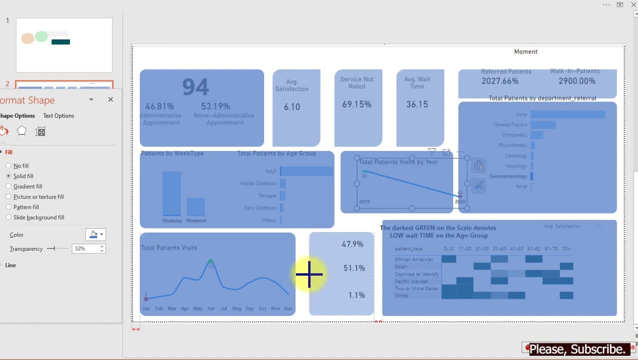 okay, so we have this piece filled. i wouldn't love to use too much of it. i'm cool with this. now i want to extend this a little bit closer to this one. then, while i move this closer, just do what suit you. i think this is cool, but if you look at it right now, something is a bit wrong here. 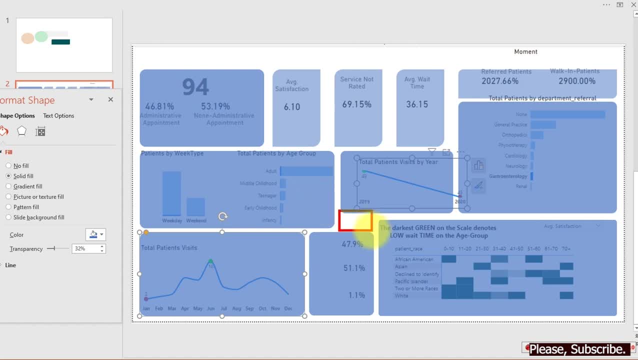 and that is this particular space we have over here. so how do we manage it? so we need to manage this particular space we have. so what do i do? don't worry, we're gonna manage this now. I mean right now. so I would just copy this and I will make it a bit. 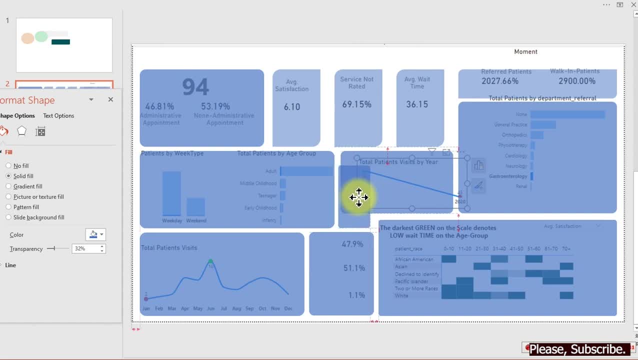 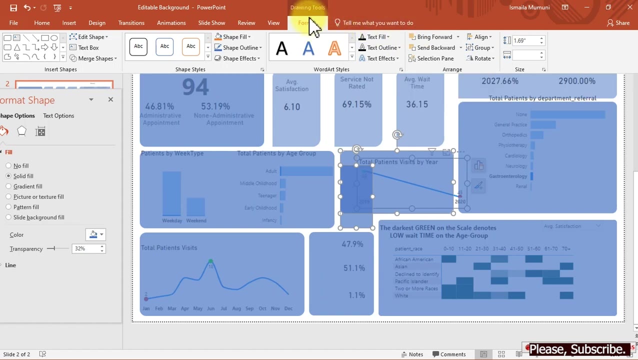 smaller. I'll fill it up to this level like this. it's cool. what I'll do is to select both of them at the same time. go to the top layer over here and over here you click on format. once you're in format, click on merge shape and here you have Union. so you click on the Union. you. 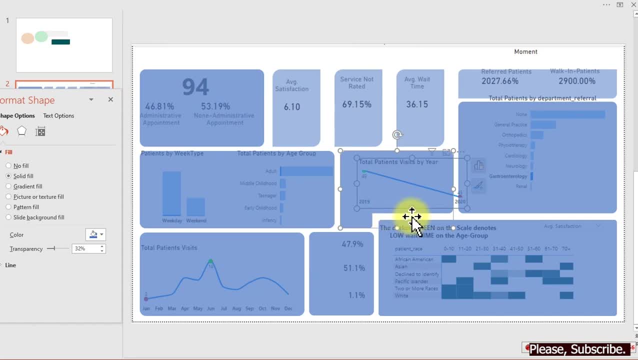 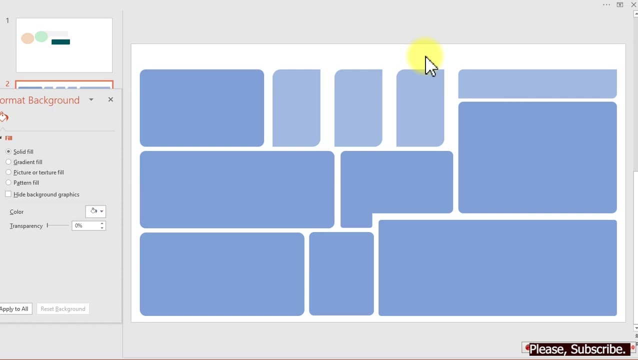 have this. can you see what it is that we have right now? beautiful? okay, we are done with all the cards we want to have right here. it is time for remove the one behind it and just delete it. this what that does is giving us a guide, so we 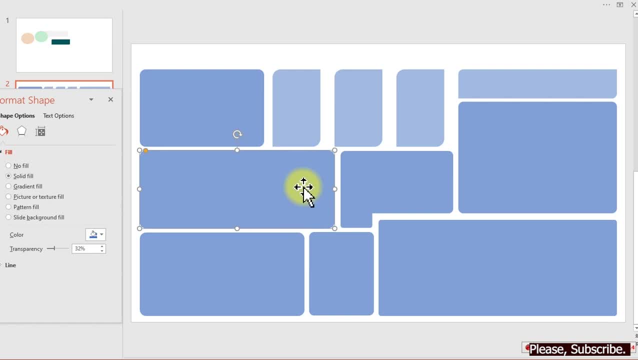 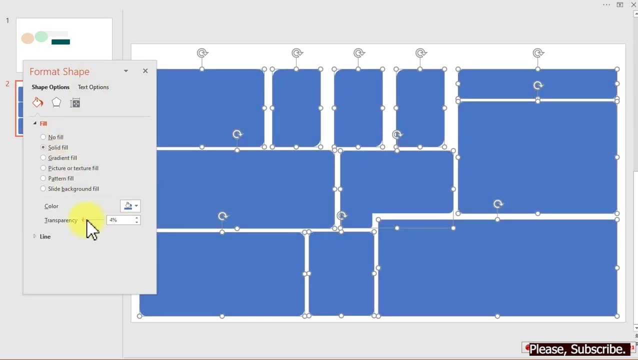 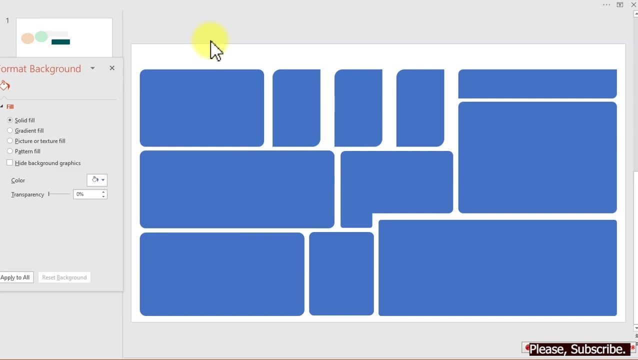 enjoy that guide gave us, so it's gone so pretty nice. the next I'm gonna do now is to glue control a and come over here, go to my color. so here you can see I put them all back to 100%. okay, it is time for we to start changing the colors. 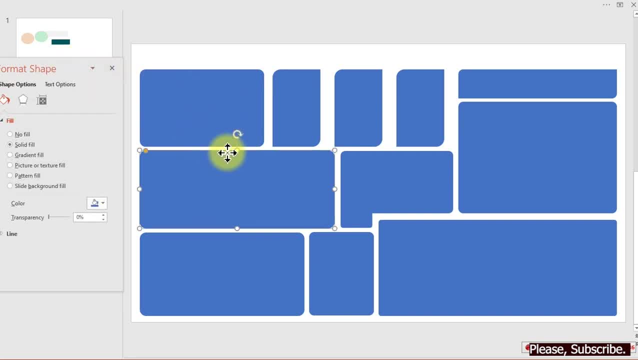 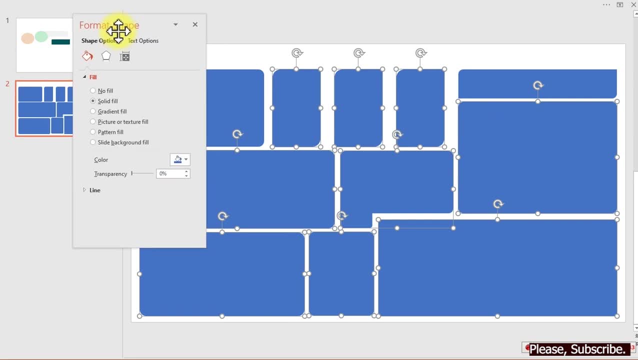 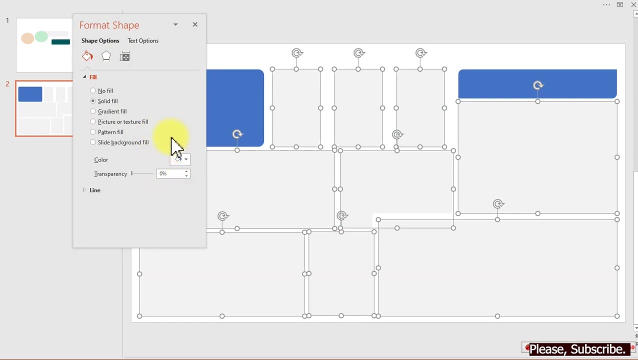 according to what we want to use. so I'm gonna click on this. okay, let me highlight everything. exclude this one and this one here. for the remaining one, I'll change it to this color, something like this. so I would like to give a warm, some kind of transparency to 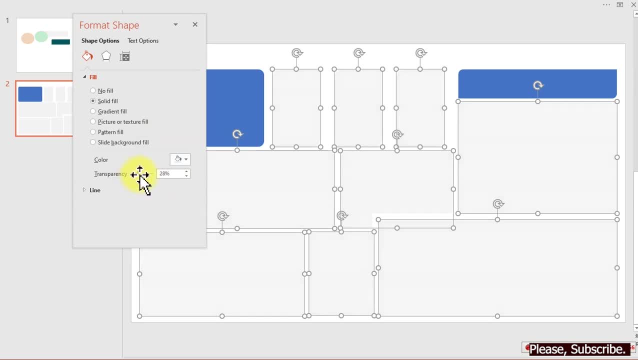 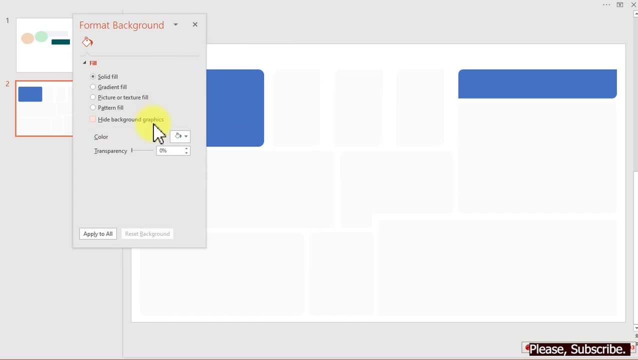 it because I don't like it to be as dark as this, so I'm just gonna reduce it a little bit. it will look lighter, just like this. so if I step off now, hmm, we have something like this- it might not look much beautiful. what do we do to? 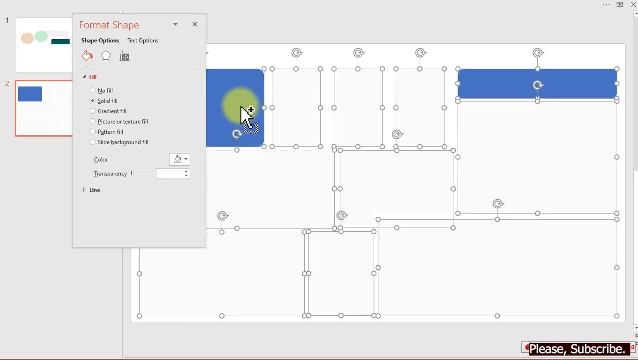 them so we can do control a again and select them, and the next thing is for me to remove some part of it, like this one and this one from it. so once I have done that, what else do I need? they can go over to here and go to. 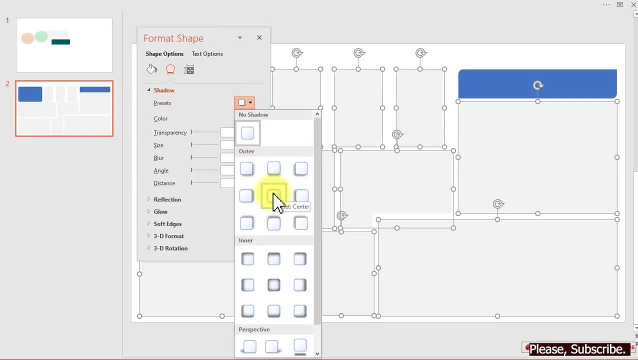 shadow and I'll apply this particular one. that is offset center. so all I'm going to do is to reduce its so much that you will know that we have something like that here. so I'm gonna put it on 93. okay, let's go 96.. So now it appears very well this way. I like to call it swing. 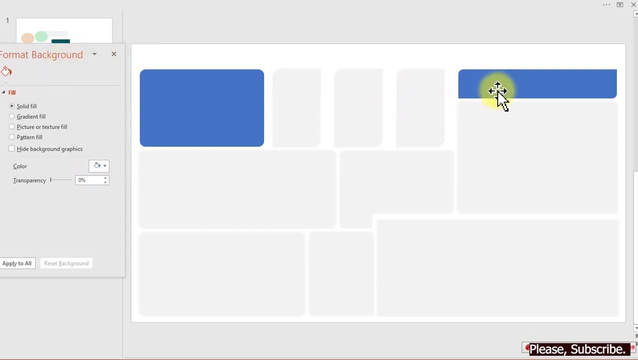 it. okay. once we are done, it is time for we to actually make use our colors. right then, the first color I'm gonna use is to click on it and here we go, we have this color, so I'm just gonna copy and I'll take it down to here, then paste it down. 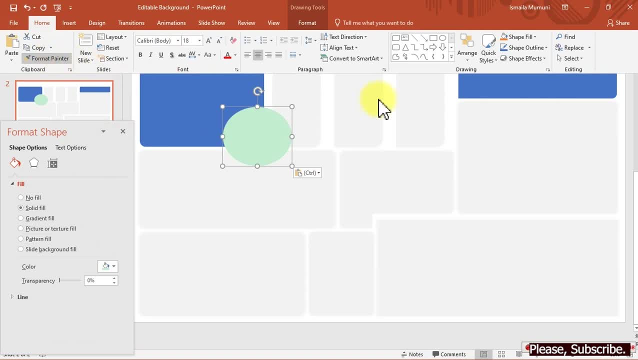 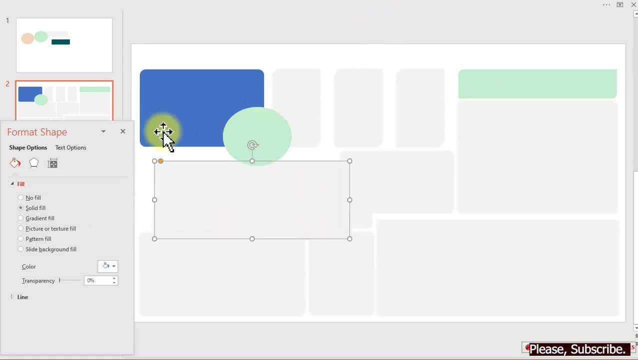 here. so I'll just use it for my printer to get a copy of it and I'll have it on this one. so the second one again is actually going. I'm gonna delete this one for now, going back over here, and I'll copy this one: ctrl C. I'll come here, I'll. 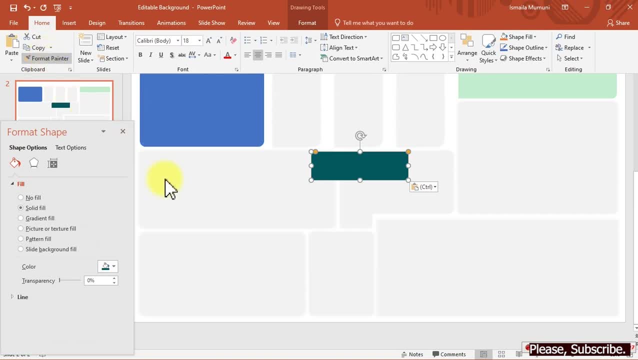 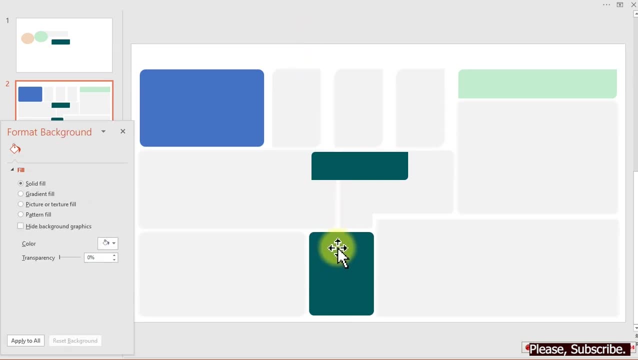 paste it and I'll go to the top, I'll grab this, then over here, I'll give it to this one. can you see that? so unfortunately, this is not the card I want to be here. I'm gonna have it deleted. so I want this same card to come. 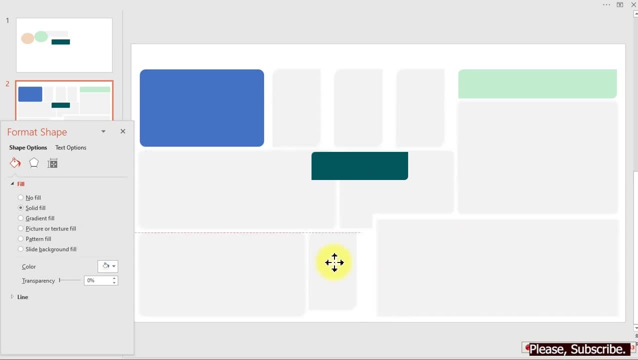 down there. so I'm gonna delete this one. so I'm gonna delete this one, so I'm gonna bring it all the way here. so stretch it until I have it sitting right for me. so you have a guy that is some kind of dotted red red line. that will be. 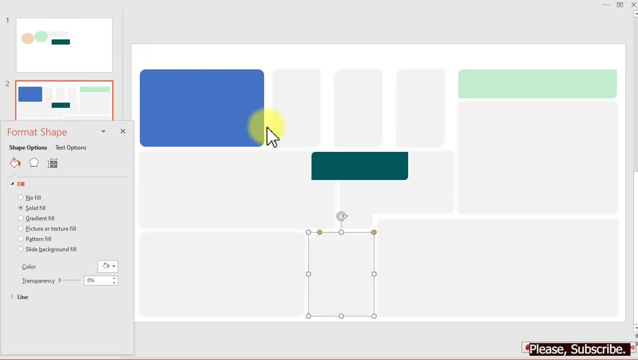 vertical and horizontal. that gives you a guy to stare you that. okay, what you're doing is a good match. you can release. so I'll go over here again. now this is what I want to have. can you look at that? so we don't want to keep this one again, so we can now delete. so on this one, I'm 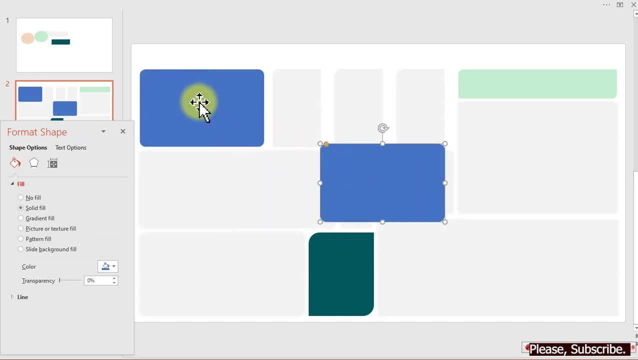 gonna have to duplicate it into two. I'll move this one over here. then, for this particular one here, we want to use the same color, like this same color we used here, which is this one. then, for this particular one here, I'm going to convert this one to white. then this one will be placed above this one. 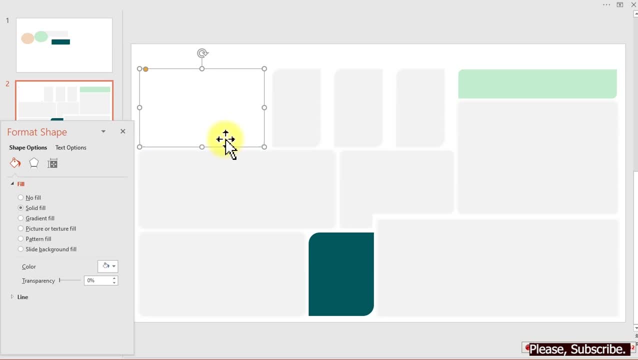 like this, then we're going to actually make sure we show part of it like this, and over here I would just adjust it so we'll have something like this card we have here. do you get it now? so on this particular part, we have a transparency previously, before now, but transparency is gone. 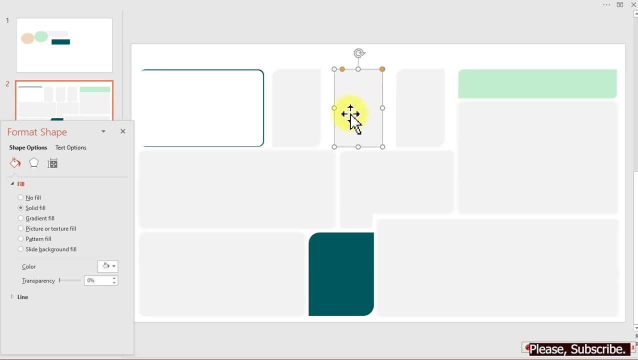 so we can leave it this way. I want to make this one a bit darker than the other. what do you do? you can come over here and select this one. so now, reduce the transparency to do the darkness a little bit, and we keep the same thing to. 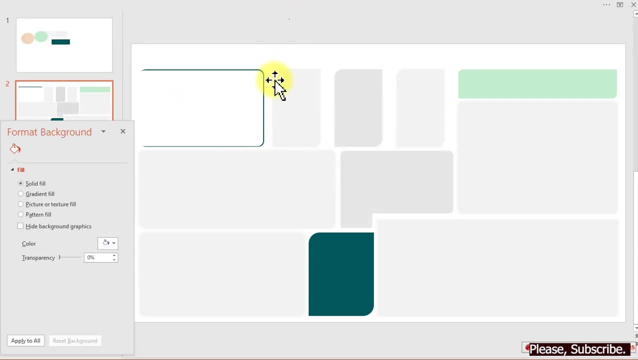 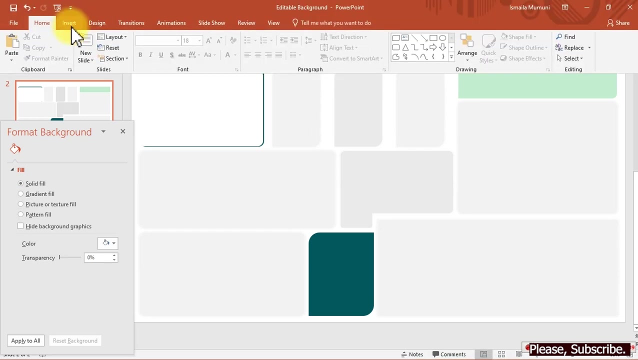 this one here. we just make them stand out a little bit. you get it down. okay, now we are almost done. the next thing we're going to do right now is to go all the way back here and go to insert, and from insert we click on these same 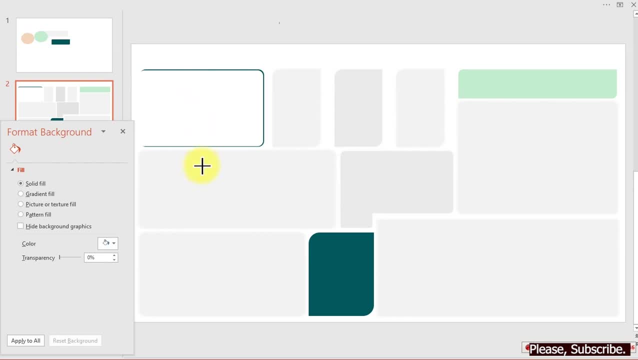 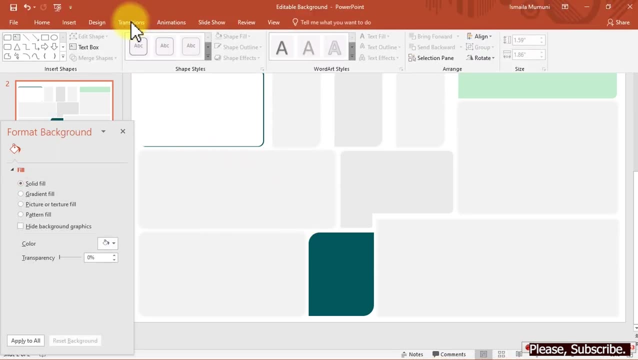 shapes. now click on circle. if I drag my circle like this, I will lose the perfect circle I need to draw. so what I'm gonna do right now is to go back and click on the circle. before you drag your circle, just click on your shift key or hold. 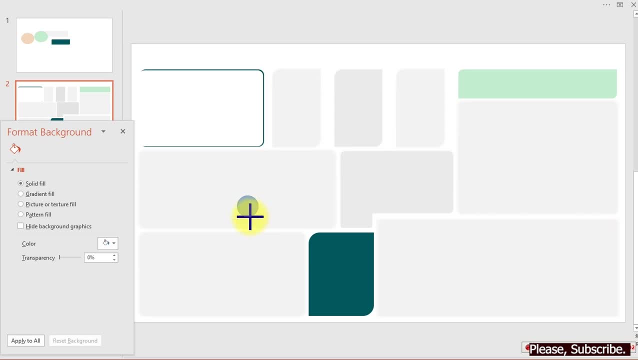 your shift key down. now you have a perfect circle so you can reduce it to whatever size you want. so I'll bring my circle right here. so it's too much, I'm gonna hold my shift to reduce it. now I'm gonna be working with this one here. bring it down a little bit so I'll have it duplicated. 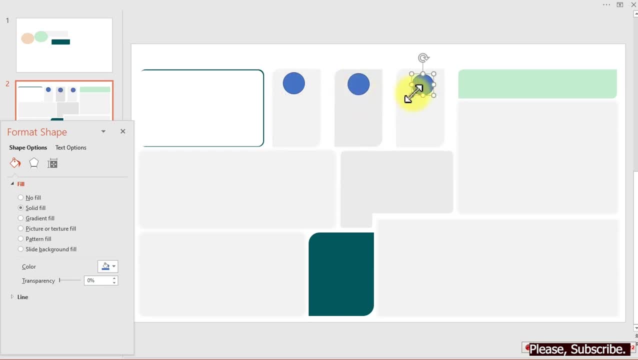 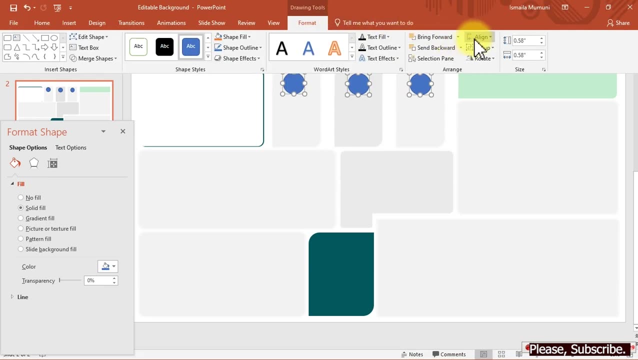 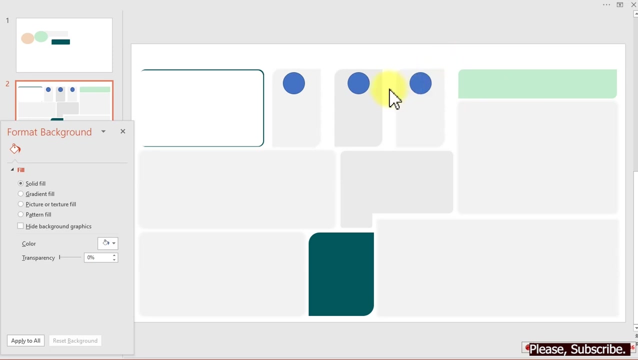 move it here, duplicate it and move it over here. so now, select all of them, go up and go to align, and you align them to the top. here you go. so after this, now we need to change the color. I'm gonna come over here and copy this again, then go. 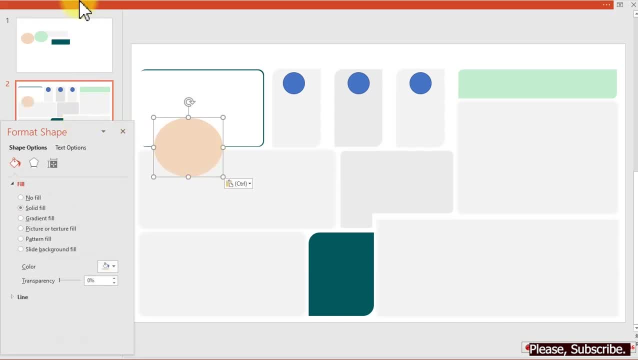 over here, paste it down, and all I need to do is to get this and I'll give it to this one. let's say: over here, then I can get it out. we don't need to see you again, sorry, so if I click on this and now we just need this same color and the 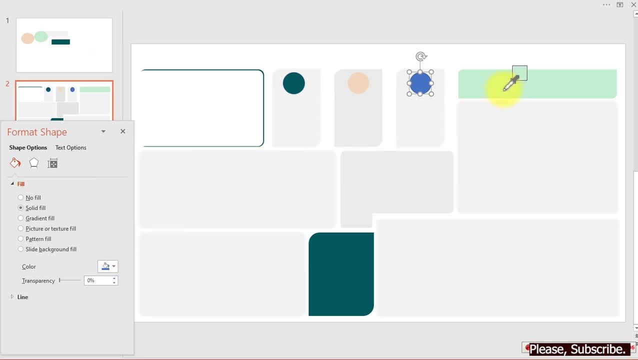 next one again if I click on this. we need to use this very color, so we have some outline on them, so make sure you hold them all and go to line and have the line removed. so this has gone off with my control Z, so I'm gonna. 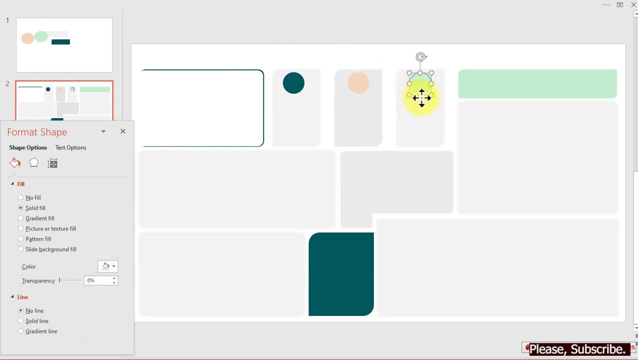 go ahead and remove it again. now we have this. what do I have here? how many times do I have a double? okay, remove this one and we just gonna go ahead and do this. okay, this is what we have. the same thing I've done right here. right now, I'm gonna get. 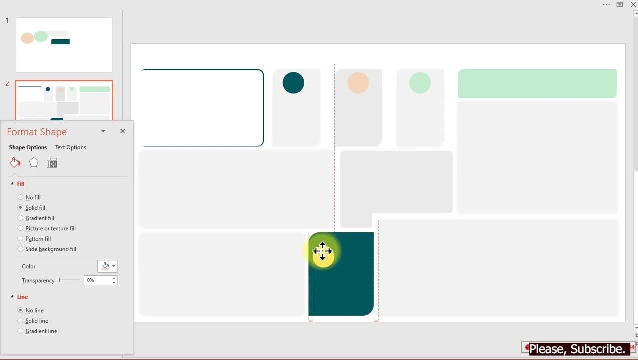 a copy of this one and bring it all the way down here for my gender. so place it right here. so over here we have this, and if I contradict to duplicate it, I have this one beneath here. I bring it over here and doing that one again. so this is. 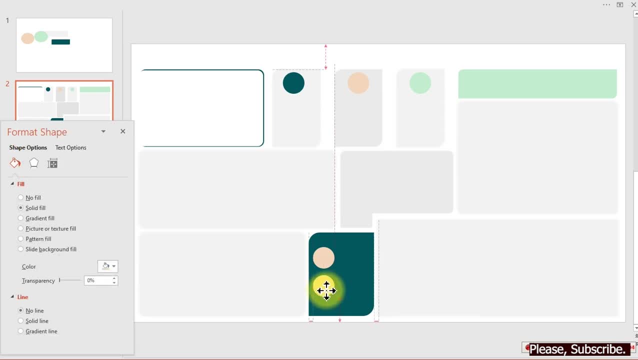 pretty big, for me huge. so I'm gonna have to remove everything now and I'll reduce this a little bit before I duplicate it. something like this would be fine. so we can do this and we can do this. so, once we are done, hold your control to select all of them and let's go to the top go. 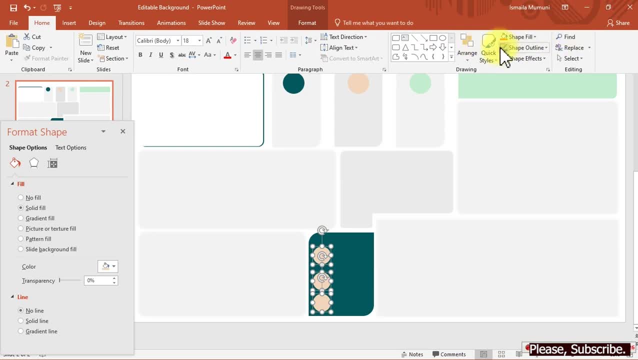 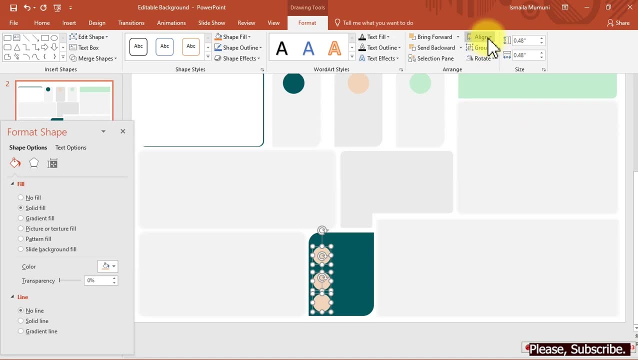 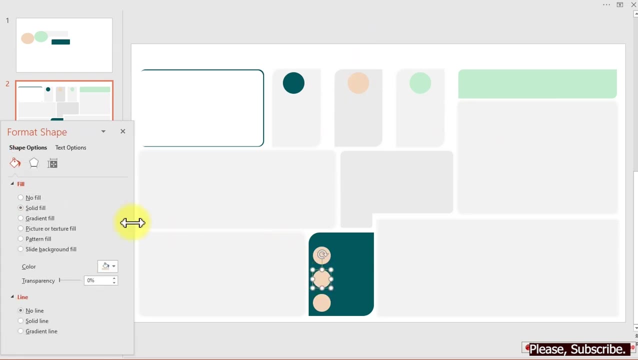 to format and from format. we use this particular. where the heck is it? click on format, we use a line and we distribute horizontally. we now come back again vertically, so it gives us this. so on this one here I'm gonna use your white color. so on the top one here I'm. 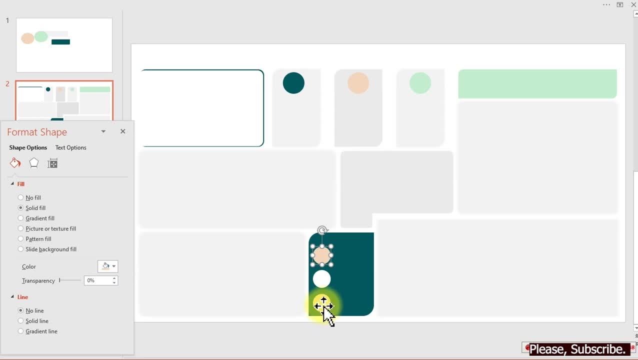 gonna use that color, then over here I'm gonna use the green, light green color. so what about this? okay, if you enjoy this, please leave a thumbs up for me and share like. if you have not subscribed, you just have to do that. so we have this. we are good to go. it is time for it to visit our power bi. but one more thing to go: we need some. 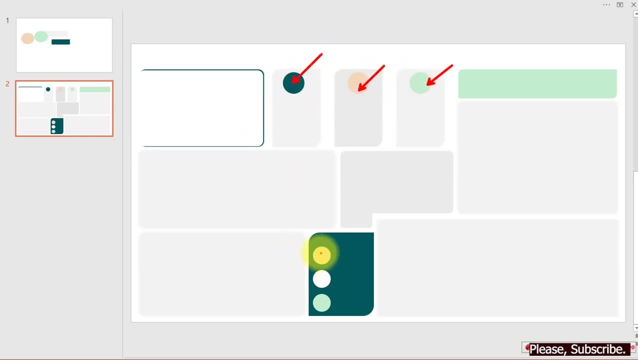 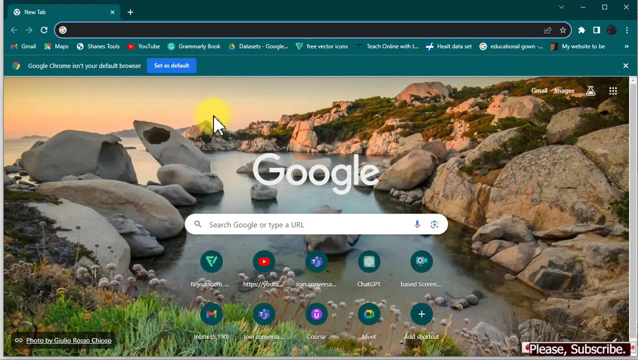 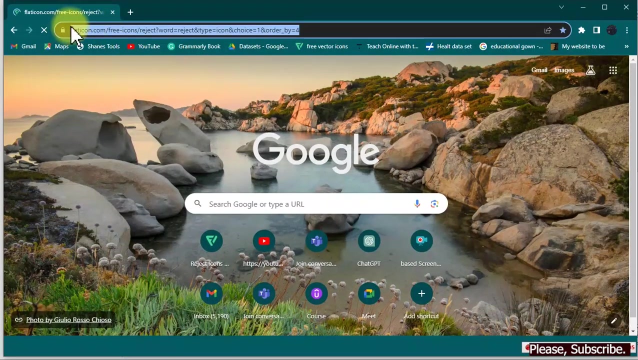 couple of images over here, here, here, so here, here and here. so let me show you the site where you can get your images for free. so let's go to our browser, all right. over here you can actually search for flat icon com. so here is the URL: flat icon comm. so flat icon comm is actually a free 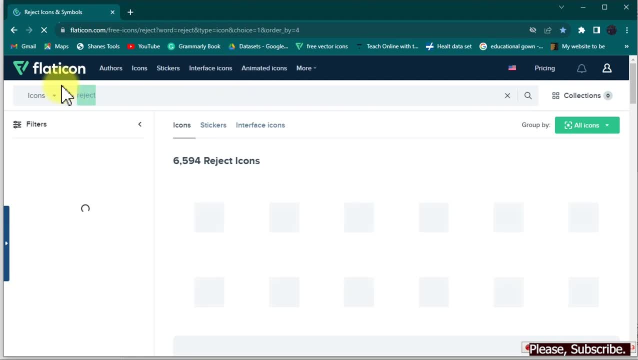 you know, website, you can actually create your icons without any background. so you can create off norma I turns, or you can create an animated icon. so here we go. I'm gonna research for a man, so here we go go, we just click and enter, so it's working on it. so we have lots of image that you can actually. 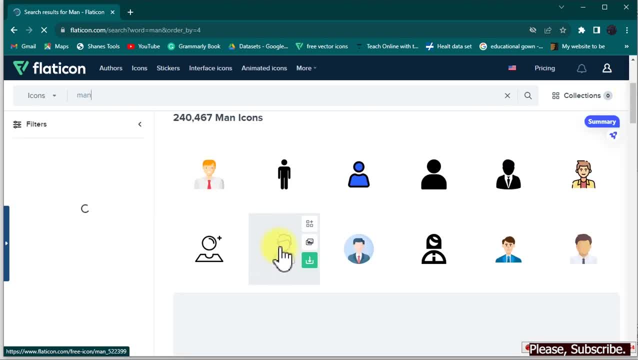 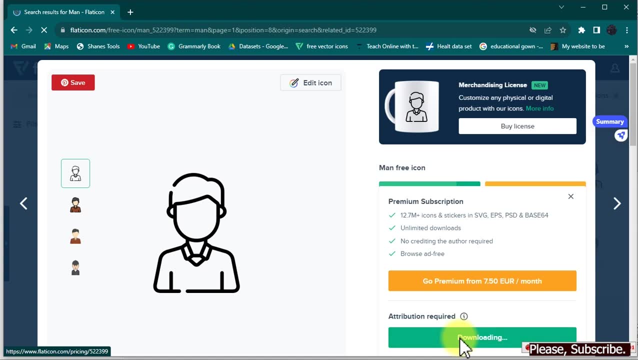 choose from right now. can you see this now so you can choose this one once you click on it? you click on png, so you click on download, all for free. do you even need to sign up? i guess no. it's 100 free, so you can decide to take the colorful one or this kind of one. this one fits into what i want to do. 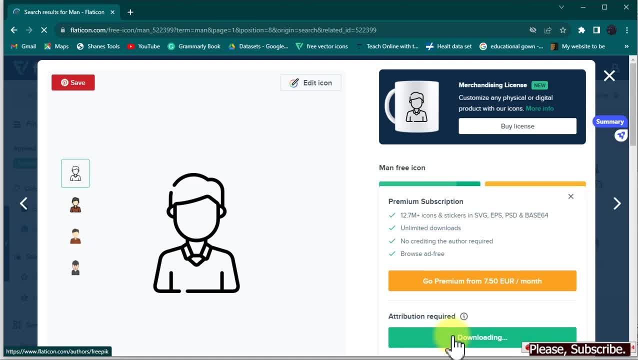 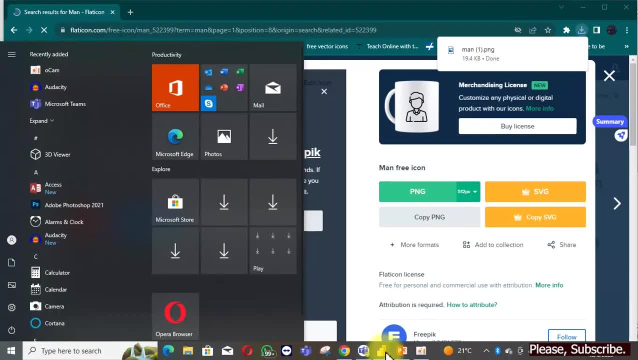 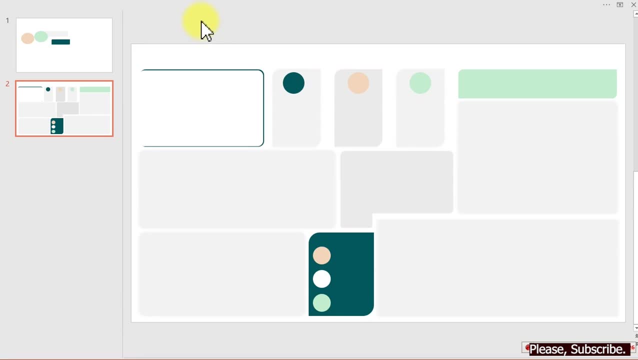 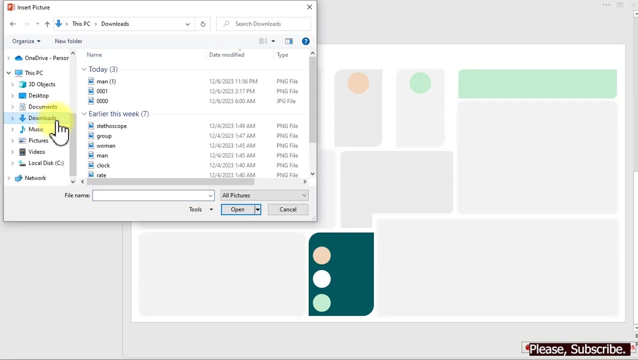 i'm going to go with this. already i have all my icons downloaded and we just need to go ahead and use it. so all i'll do: once you have gotten your icons downloaded, come over here and go to insert and from insert, click on pictures to pick them up. so download. so i have this icon, this, this. 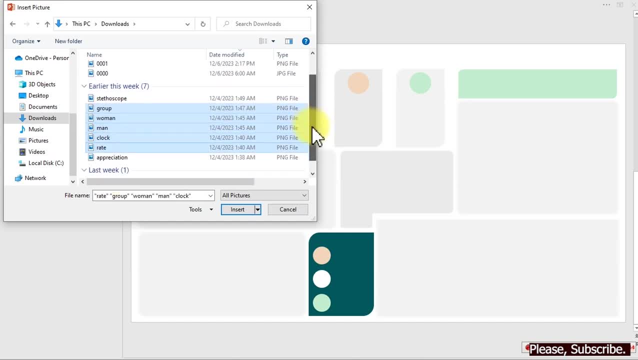 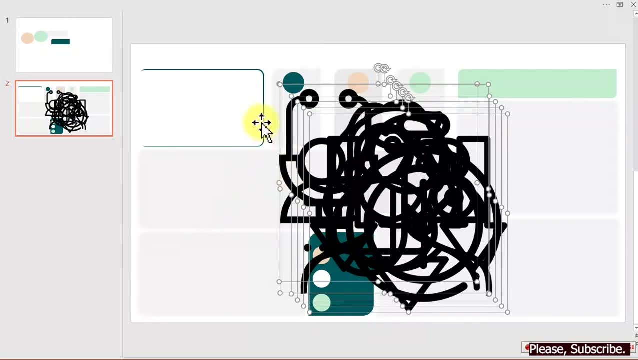 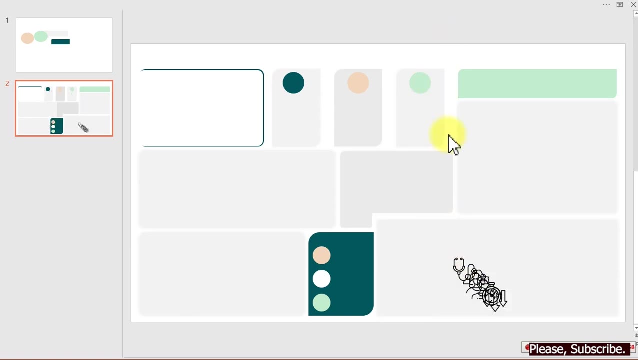 this. this one, i think the eyes are. i'll just import it in so you can just do this adjustment like this. okay, so individually i can start moving them, separating them, separating them, separating them. this icon is going to be my logo, so you can just transfer them with any how you like that can fit into this particular space. you have right here. so 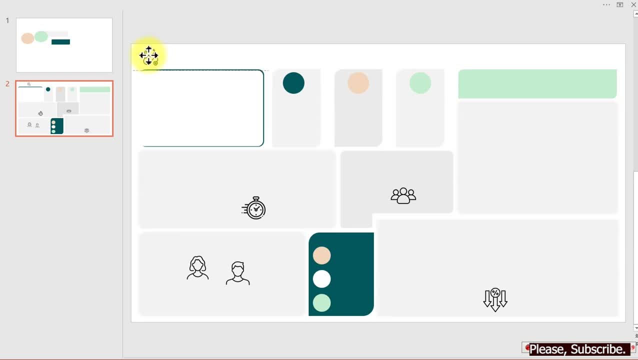 i'm going to have this one somewhere around here then that is it. so make it a bit smaller and fit it into here. so after that, now we come over here. so you always make sure you make it fit into what you want. so i'm going to move it and have it over here then for this one, here for my. 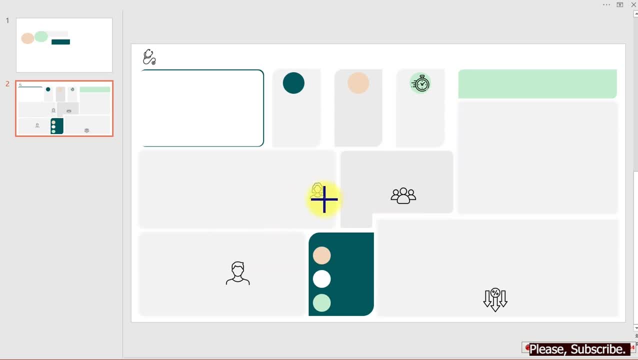 male gen for my gender. i would love to actually have this for the female gender over here. that fits in a lot for the male gender. i will do this. i'll bring this over here. then for the unknown gender, i'll just get this icon, make it smaller and push it in over here. 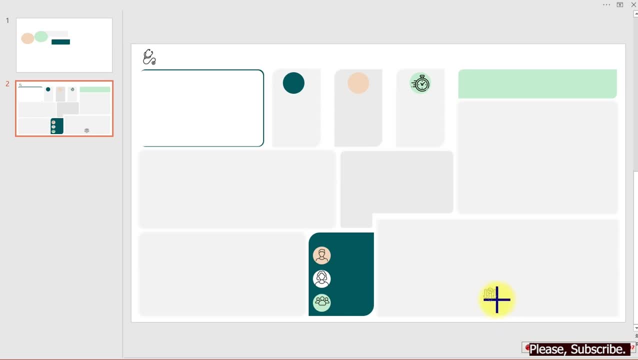 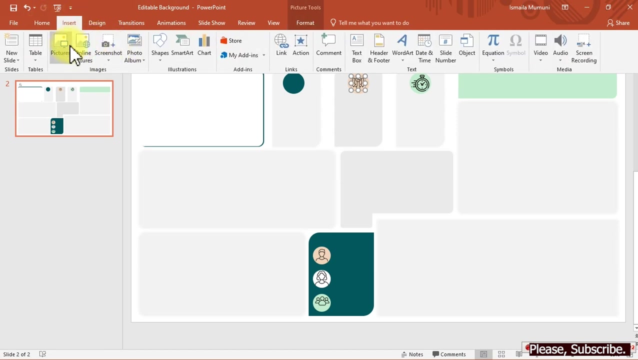 now this one is actually service, not rated. that is why i have this arrow down, so i'm gonna move it right to this particular spot here. so i have a thumbs up. i didn't have it right here. i think that is that one that says appreciation, right? so we go over to insert. i'll go to picture. 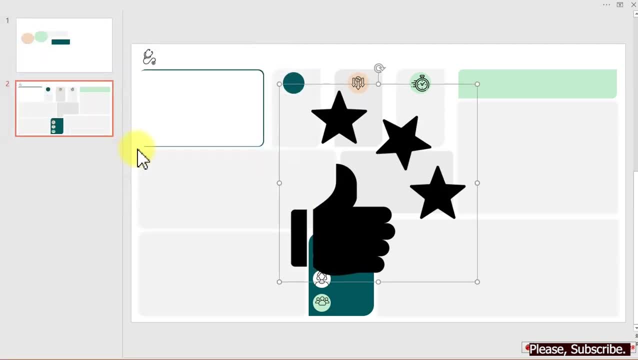 so we scroll down here, we have this appreciation here, so we just make it a bit smaller. so if you look at this now, if i put it over here, where i want to put it right now, it won't be visible, just like this. so what do we do? we have to change it a little bit. so what do we do? we have to change. 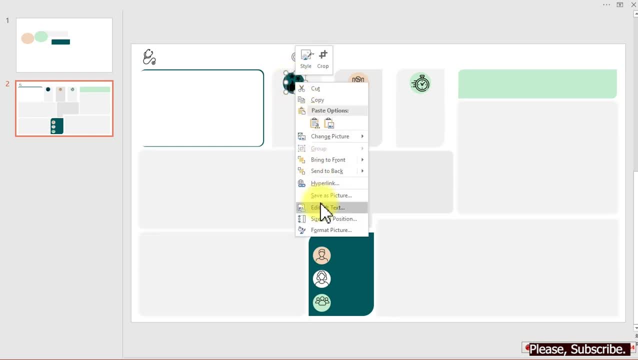 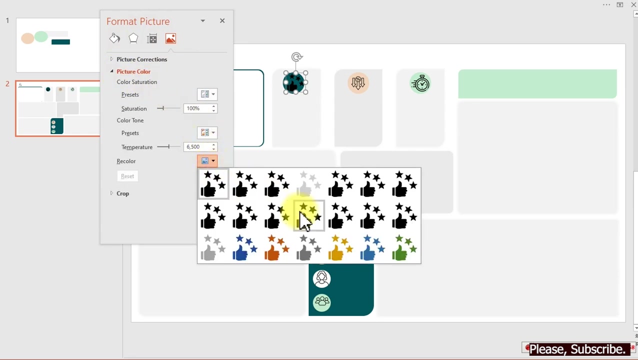 its color. so all i have to do is just to right click and go to picture, and we are here. the next thing we do now is to click on this particular picture here, then click on picture color and i will click on this part- and now we choose a bright color. something like this looks better: 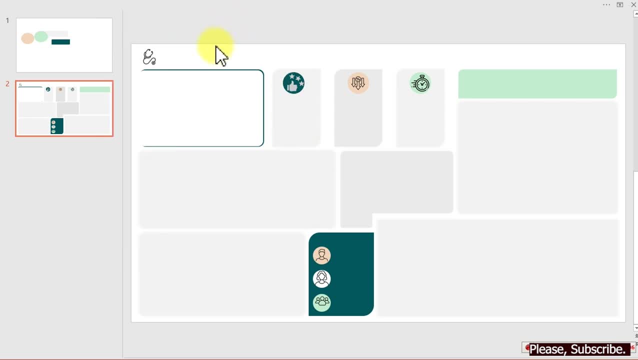 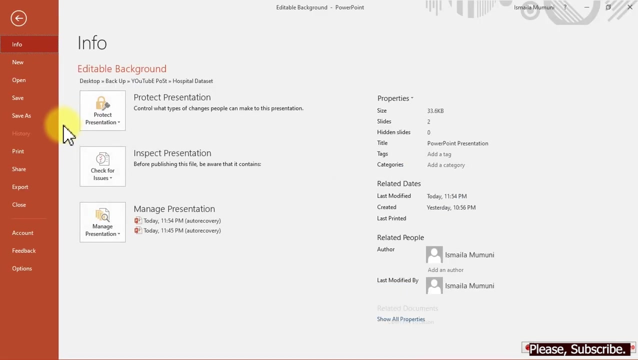 right, this is all we have to do to create our template or our background. we have just done the justification. the next thing now is to actually export this out to whatever file size we want to use, or format rather. so I'll click over here, then go to file from file. now we have to go to export from export, we go to change file type. 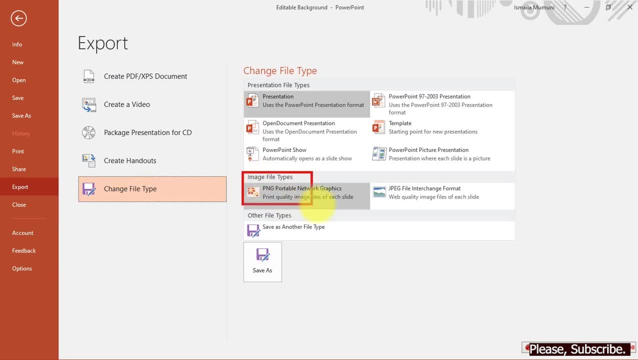 and you have two options over here. you have the png, we have the jpeg right here and we have the gif. if you click on what? if you click on this particular part where it says save as another file type so you can use the gif file format to save, it is your, is all your choice, so I'm 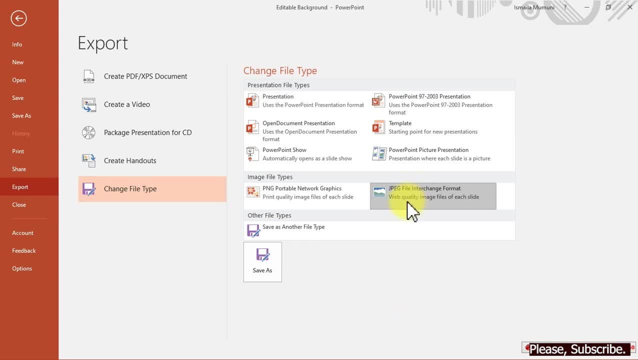 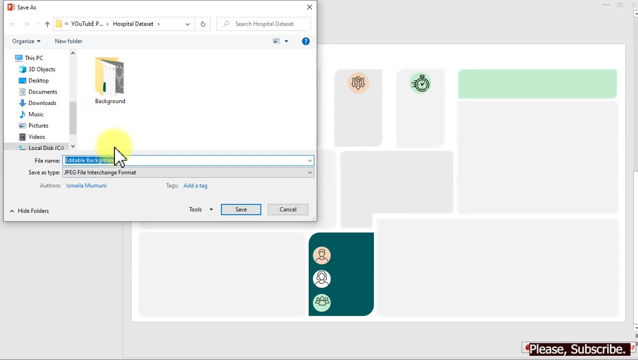 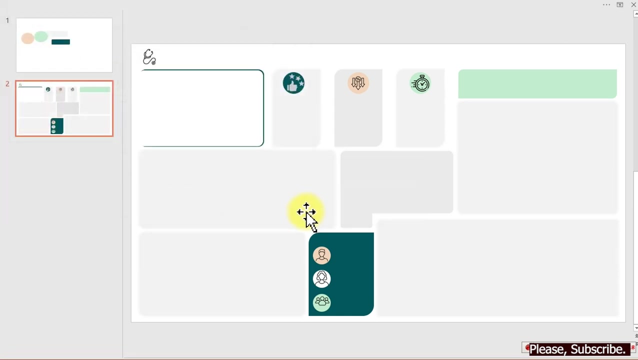 going to go with this particular, this one here, so I'll double click it. so now that we are here, what I'm going to do is just to say, um, bg or background, okay, let's go with bg 01. so now I'll save it in here. so just say just this one. then, once you're done, the next. 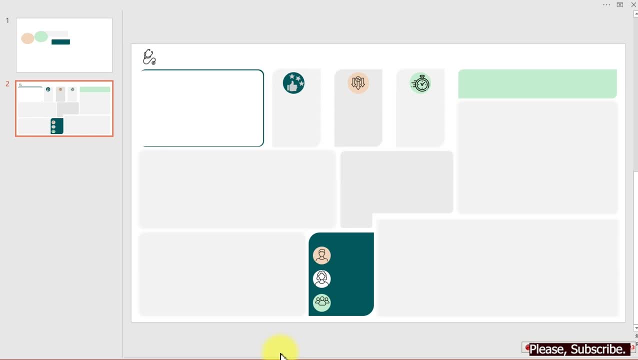 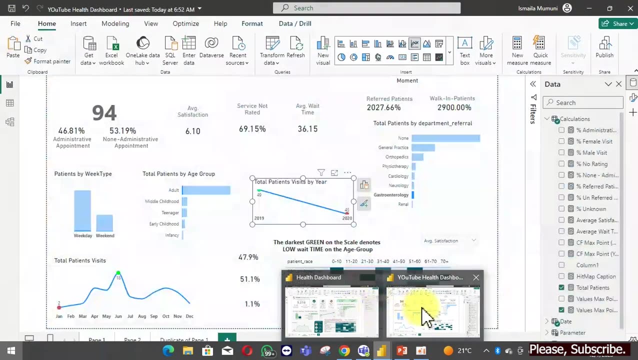 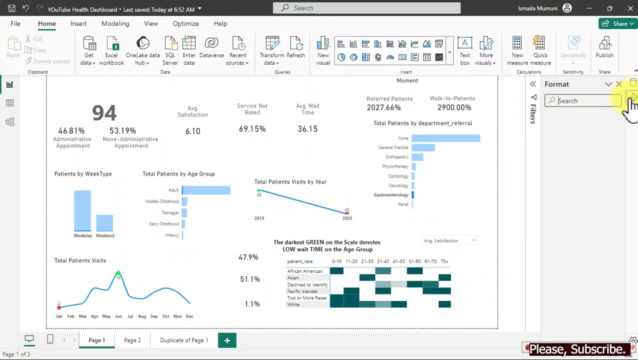 thing is for we to go and visit our Power BI desktop. all right, we are right here on our Power BI desktop. click on your format. once you've clicked that, make sure you don't have anything selected like charts. don't select any chart right here. just leave it the way it is. if you select chat, what you see here will be different. so if you 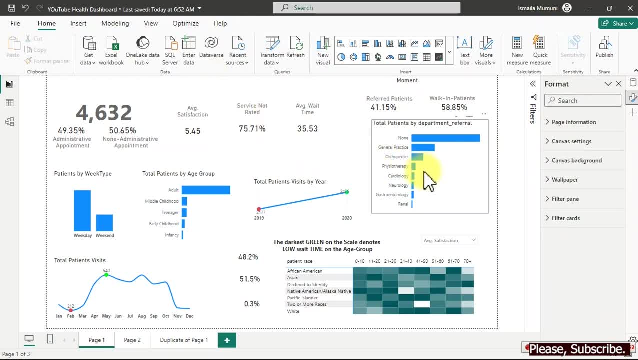 select nothing. just click on the empty Converse, then you're gonna see this option right here where you can actually, you know, Converse settings, background, your wallpaper. don't use this. what you're going to be using is the background right here, so click on it and go over here. then after. 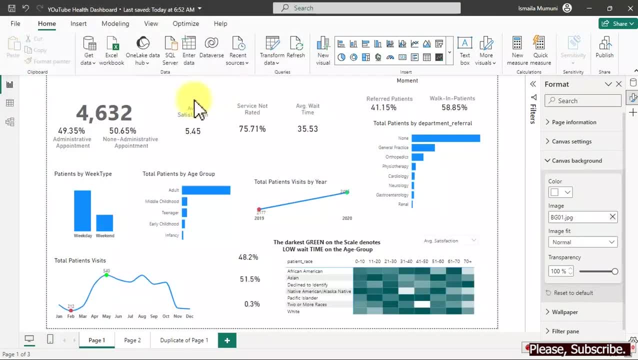 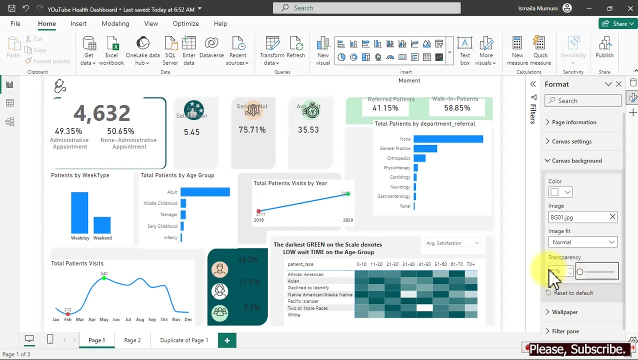 that now you can click on this. oh, what the heck, where is it? oh, don't worry, let me panic, I'm gonna show you now. make sure you turn this one to zero percent, and that will definitely give you this beautiful right. so now it's not looking cool. anyway, it's not looking very, very cool. what do we do? how do we adjust things? let's. 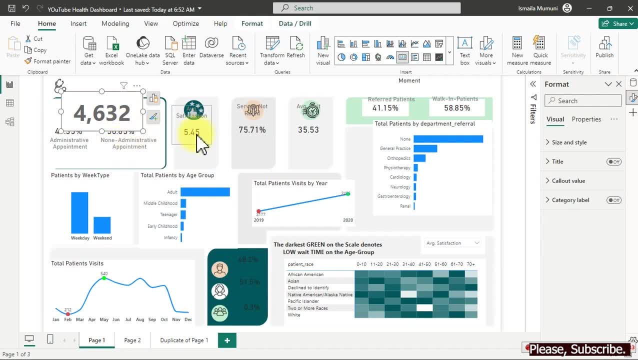 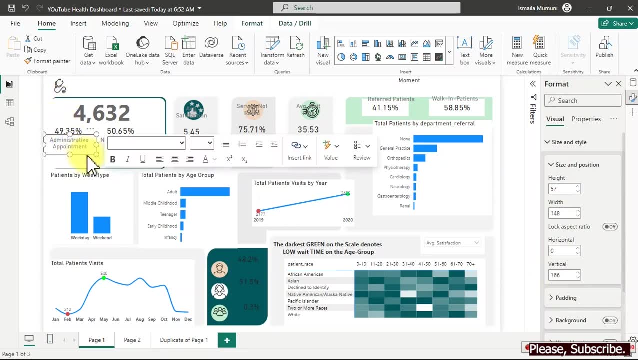 start our creation from here. now I'm going to click on this and remove its background by coming over here. I have the background click done. I've removed it. click on this and just move it down this way, right, so once we have moved it down so we can click on. 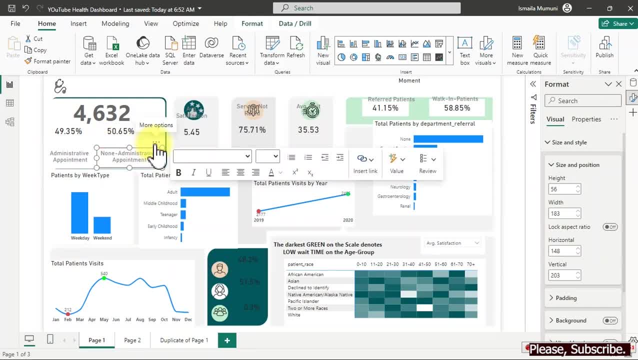 the same thing here and move this down. okay, then we can just move this to this level and we move this to this level here. then we can now move this down like this. all right, so if I click on this one, I would have to go out and create a duplicate of it, so it's duplicate will do something for me. 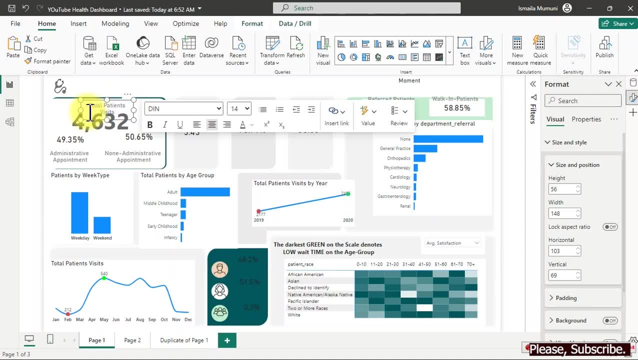 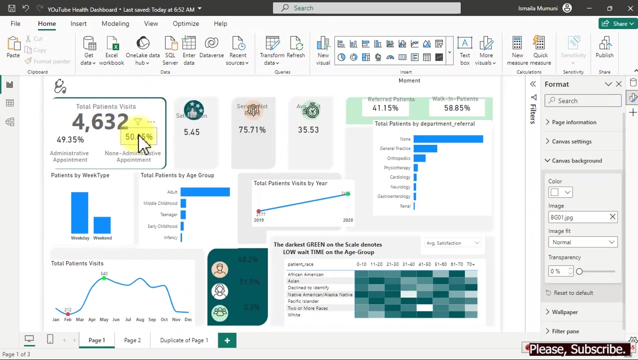 that is gonna be so. to type patients visit. so we stretch it, so we can control it. to make it a bit bolder, I'm gonna use 16.. so we settle it down right here. so target the middle. this is what we have. so right now I'm gonna have to move this. 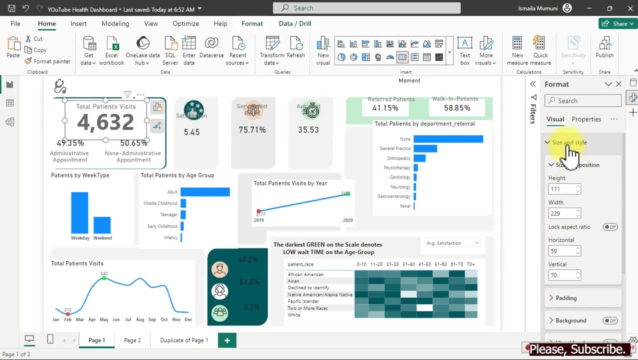 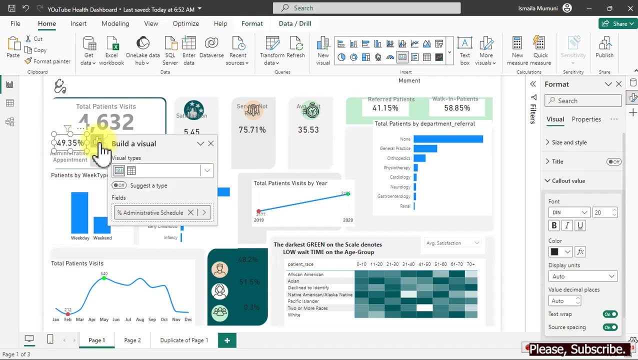 then we come over here to change the color. it's time to work with our colors, right? so come over here, we do this. let's go with this. okay, something like this would be cool. I love it. okay, now let's look at this here, this one, click on it and make sure you know this is. 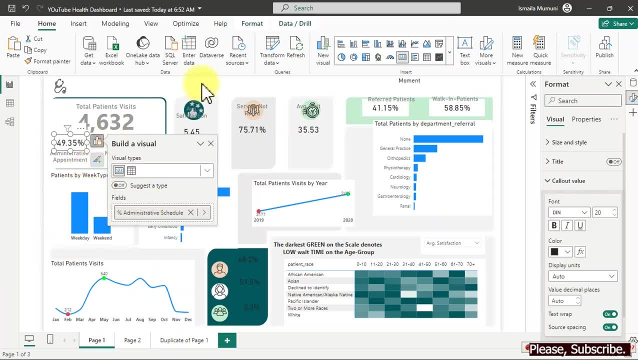 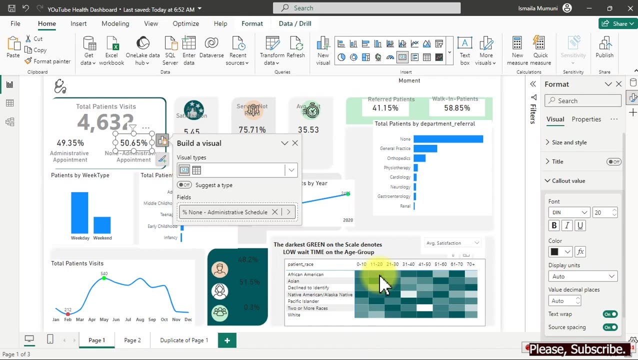 administrative schedule right, we get it right. then if I click on this, we have to verify: this is none and it's correct for the none. I would love to use a different color and that would make me to start going back to our. if you remember the color code, you don't need to do that, so you have. 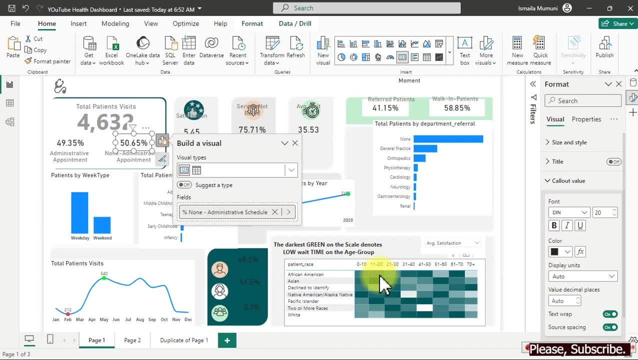 to go back to your PowerPoint to pick the color code. but right here we know the color code, or we know the kind of color we're looking for, so just click over here. I will select something like this that corresponds to this, but something lighter that shows up very. 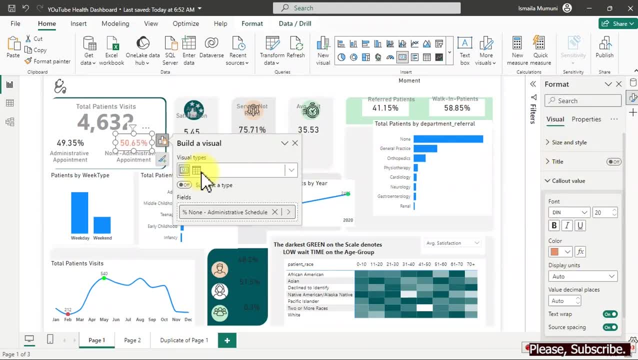 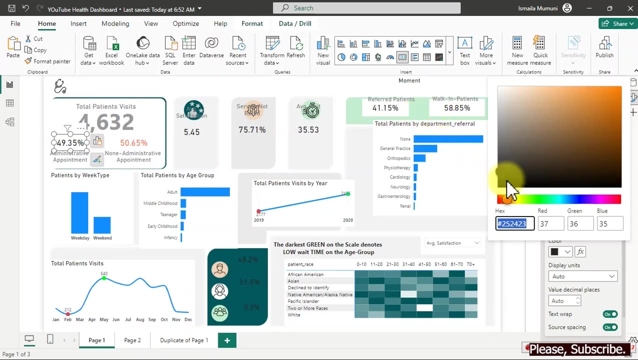 well, so we do this brightly, right then, I am cool with that. so I select this now. I want to use a color that looks like this one, this particular background right here. unfortunately we don't have a color picker, but I can just try to guess. it's right, right, if I do this now. 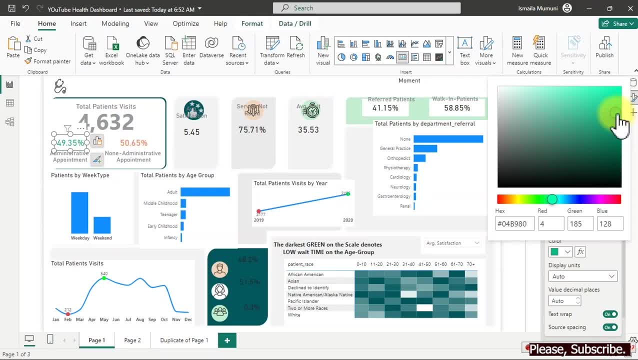 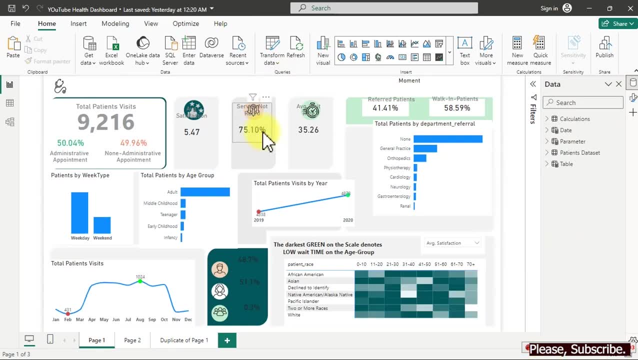 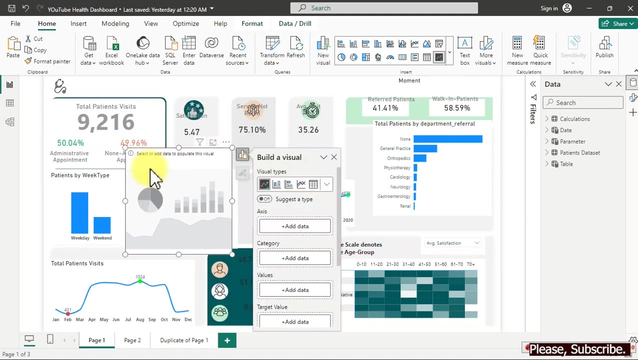 I can just say, okay, this is the color here, I'm going to use this color, right, so we'll release it all, right? if you remember, we actually brought in this particular sparkline in the class prefer now, so we have the sparkline here. for the sparkline to work we need you know two things that. 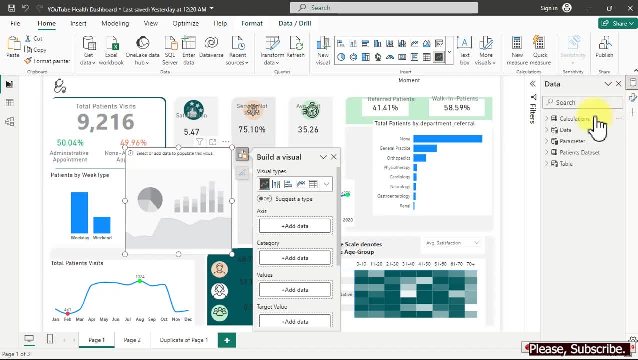 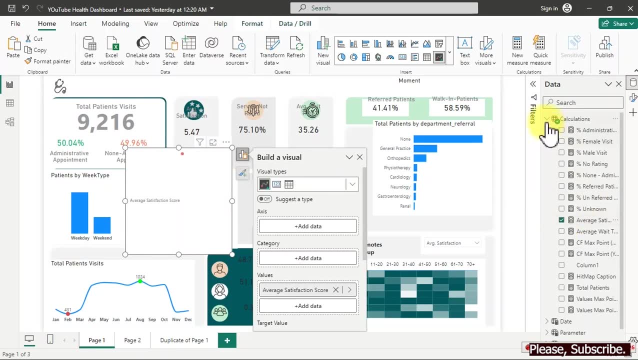 is the average satisfaction and the month. so what I'll do is to come here now and I will see my average satisfaction right here. so once I have it I will go to the date from the date I'm going to pick the month here. that gives me this. so now I have to some kind of adjust it. it's not. 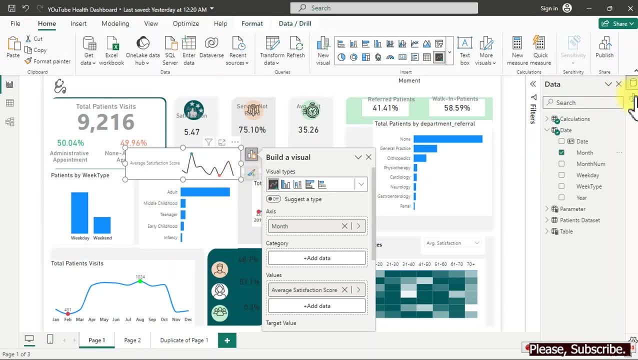 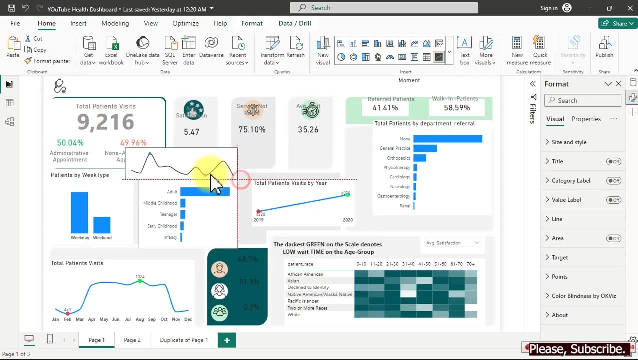 looking very beautiful. what can I do? I'm going to go to the format. from the format, I need to turn off the category label. then I have something like this, so I'll make it a bit smaller. so drag it to this- the three dots here- and make sure it sits right at where you want it to be, just adjust it. 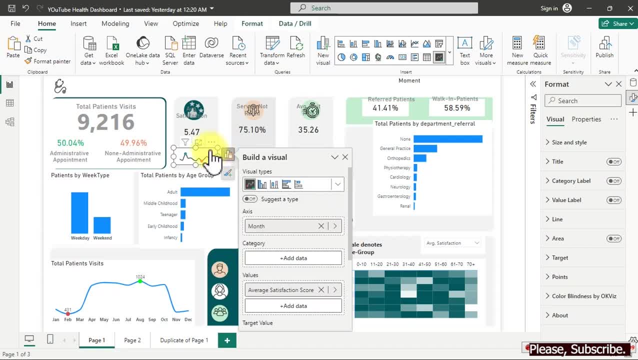 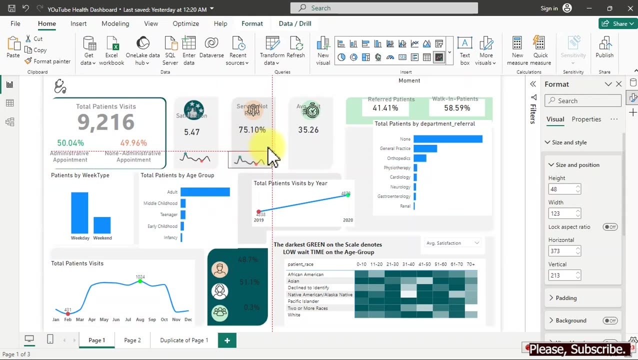 Move, Resize. all right, we have this. if you look at it now, we have background distorting it. all we have to do is to go to size and style and we turn off the background quickly. we can do copy and paste. so when paste, we bring this over here. right, and the only thing we're going to change now is the satisfaction. 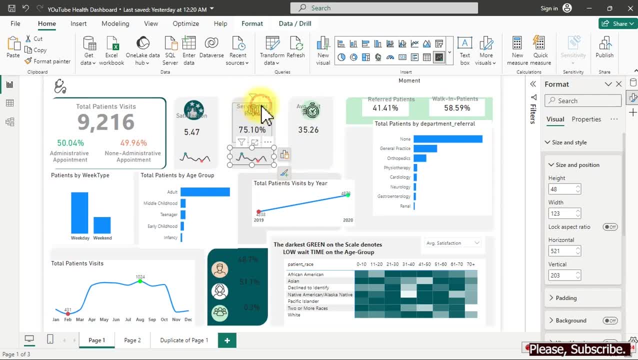 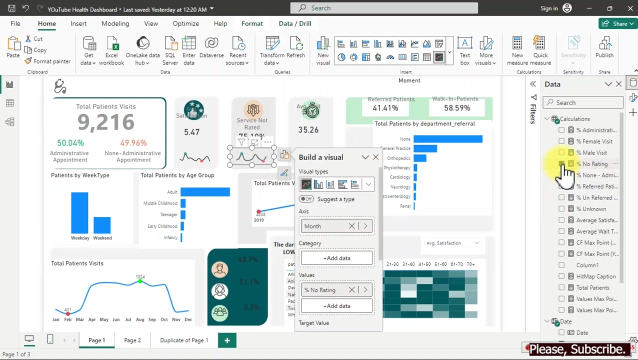 um, not satisfied, not sorry. that is going to be this one here. i think it's going to be service not rated, right, so we just change the merger alone. so we change to service not rated. that is going to be under this one here. so, not rated, the percentage of not rated. so quickly we actually get. 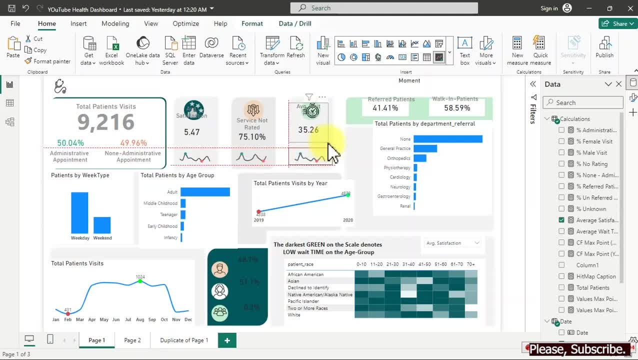 another duplicate of it and we bring it down to this particular part. so what we're trying to achieve here is looking at a trend on a monthly basis, how it goes so quickly over. here. we are changing this one to be our average uh waiting time. so here we go. 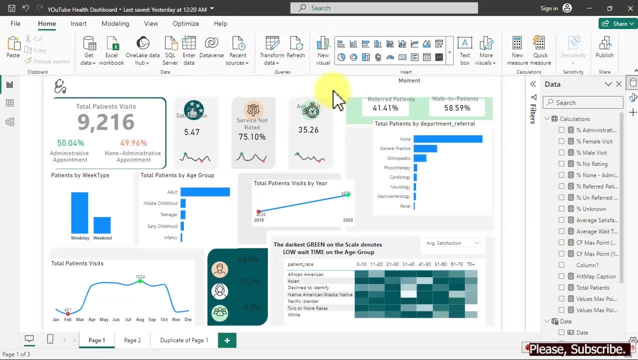 so you can see trend of average waiting time. so once we have done this, the next thing now is to make sure this one sits right to show the yes, i'm gonna bring this one down, then this one as well. we bring it down to this level. okay, here we go. so we have something like this: 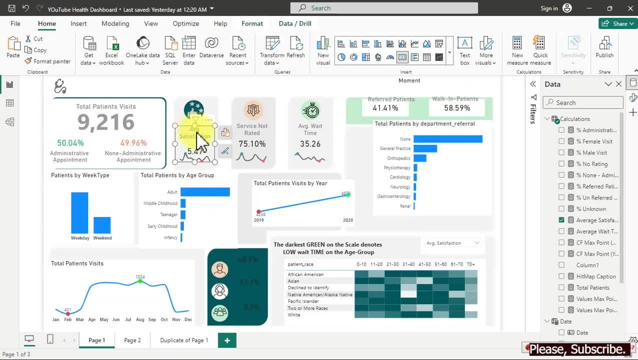 so let's go ahead and adjust the format a bit for you to see how it works. so let's go ahead and adjust the format a bit. so spend some time adjusting the formatting to suit what you really want to have. so you get. that is it? here we go. 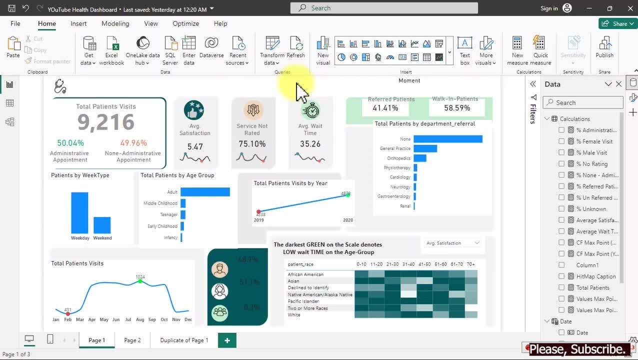 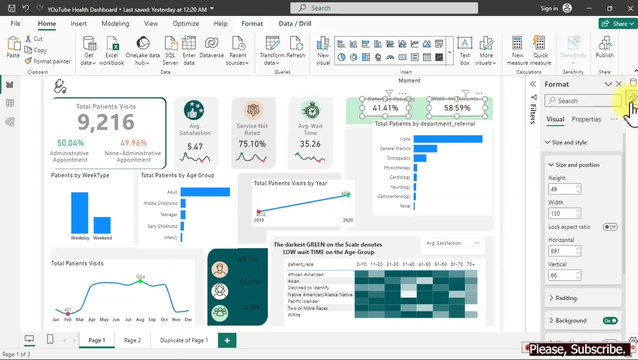 spend some quality time adjusting all of this very important. so, as you can see, now it's taking shape, but not really fine the way we wanted. okay, the next thing now is for me to click on this, hold your control key to select this as well and go ahead to the format. from the format, you can see where the 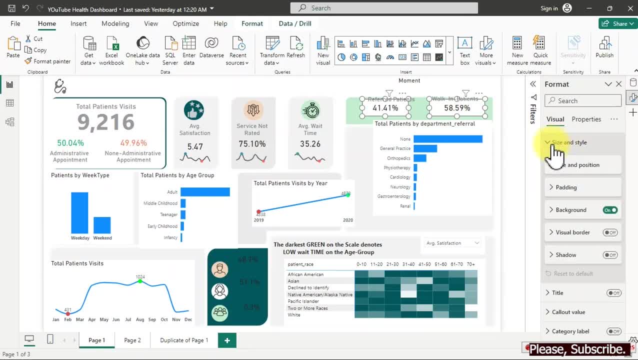 you can see where it says style, size and style. we turn off the background. good, so we can move it down a little bit to this level here. so manually we can change what we want. let me bring this down so we have this one controlled first. okay, for the label at the top, we need to actually move it down and fit it into. 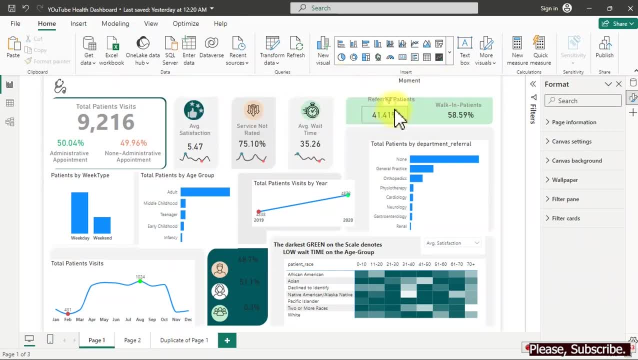 here, so we come over here. we bring this all the way to this level, alright. so the dark color here is cool, but not that cool for me. I will need to work on it, click over here and select something like this: let's see beautiful, so let us. 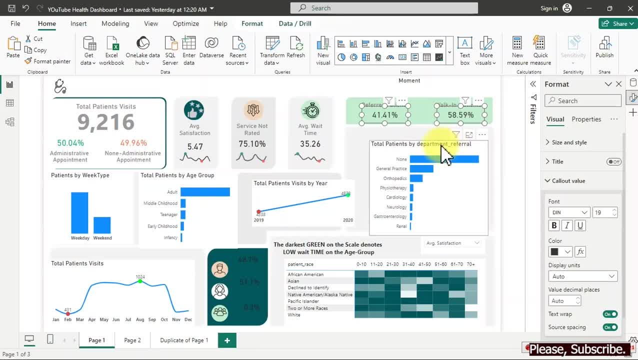 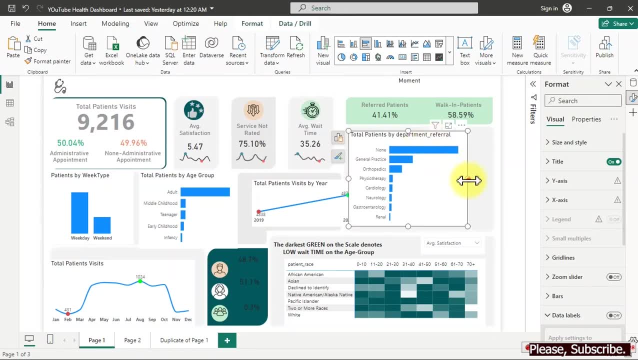 make it a bit darker. we go for this one better. okay, it is time to work with this. if I just go ahead now and align it, I'll bring this over, stretch it over here. I will go for my size and style. I'm gonna have to turn it off. all right, the next thing we're gonna do right now is: 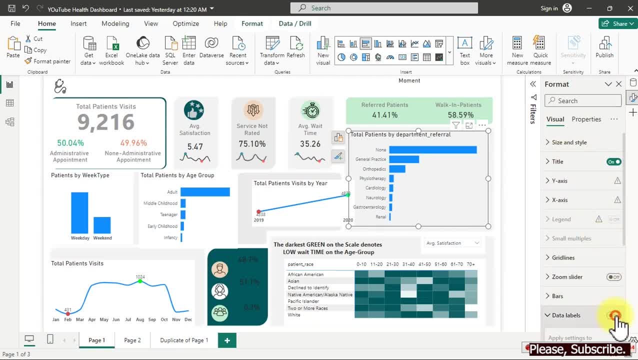 going for detail a bill and turn it on. we have something like this, so I would love to show it fully then. what I need to do now is to make sure I have it opened and I go for where I can actually select the option I want. so go to values and if you scroll down, 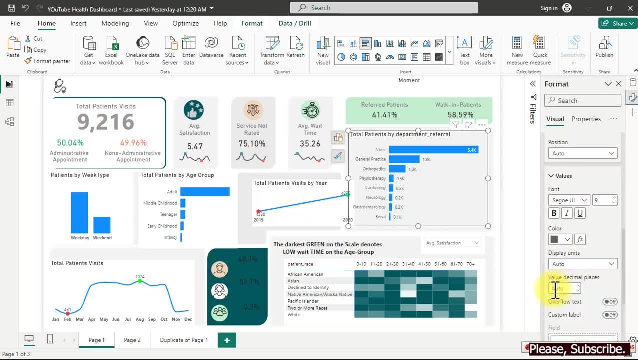 under values, you see this option, so display none. then you have this all right. I would love to show the green color which we have over here. it's not really easy for me to pick it up right now. what you can do is to come over here. we have it right here. we can take it and make sure we adjust it to fit what we. 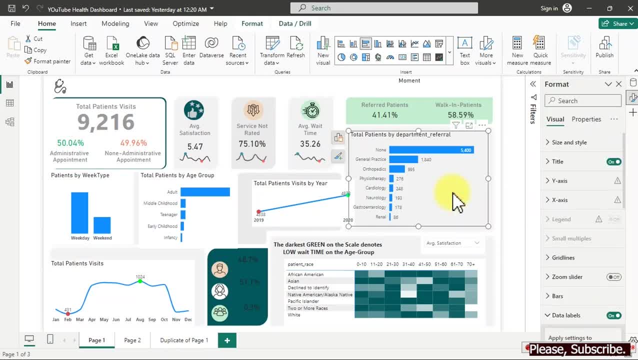 want so quickly, click on this particular chart. so once you click on this chart you go to the bars, so you scroll down a little bit. so here we go, so we can pick the color here. so it's a bit different from what we have at the top here. we want to get this exactly what. 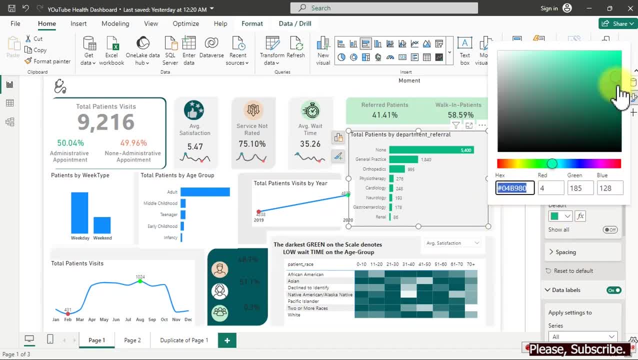 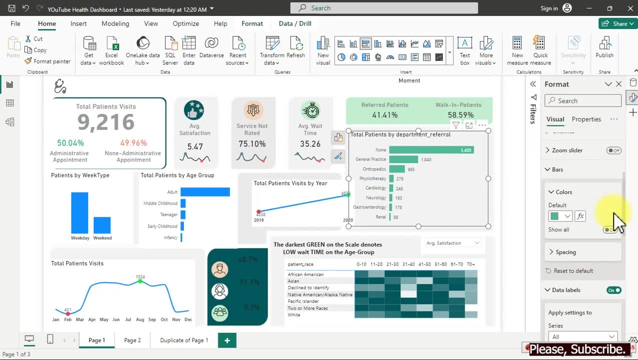 can we do? can we find a way to get that done? so once we click here now, we can start adjusting things up to this level. let's try this and see. okay, it's still a bit. I'll just go remove things over here now, very close to it. this is exactly what we want. okay, we have this particular chart. 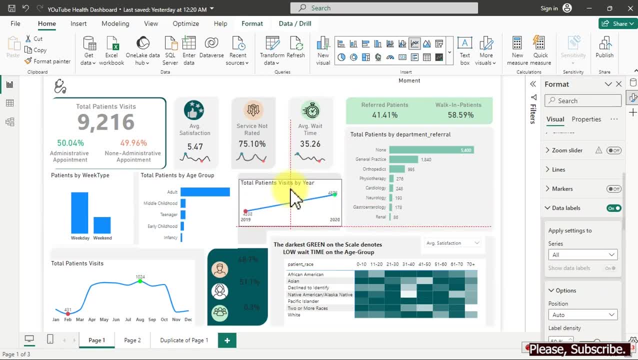 here we have a line chart that we have to some kind of take control of, so all I'm going to do right now is to come over here and turn off the background. for it, no background. then next thing again is for me to go for the label- sorry, the color, so you need to. 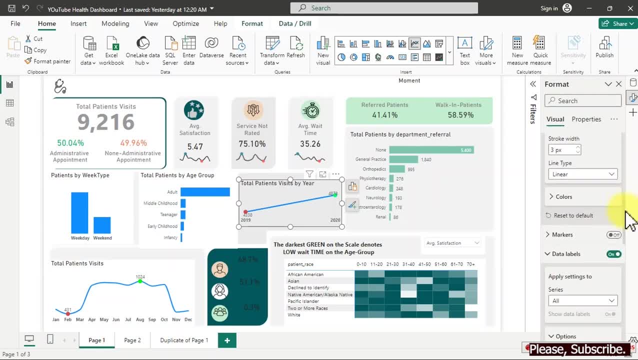 go to the line from the line we look for where we can find the color and change the color we want to use for it. all right, we have the color here, click on the colors. so I'm going to change the color to this. yes, there is one here. 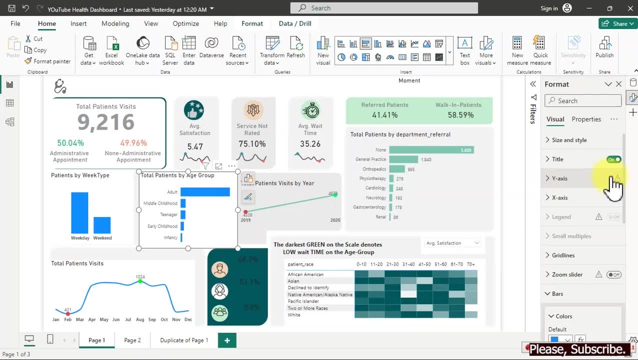 we have something like this: quickly, we click on this one and the very first thing we're going to do is to actually change the bars right here. so when you click on the bars, it opens up this one for you. so we select this very color. so we do the same thing to this particular one. we select the. 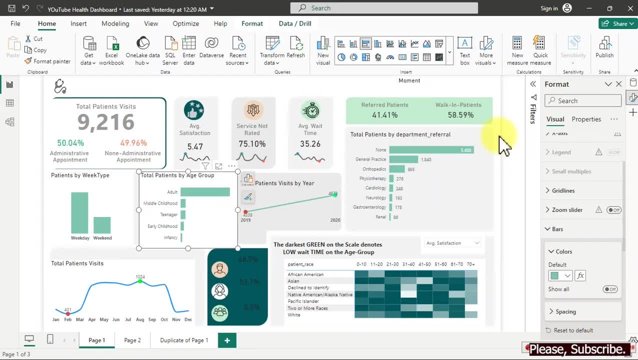 same color for it. so now let's do format this properly. so I'm going to turn off the background, including this very one here. I have it turned off, so if I click back on this one now, i want to make sure i align it, and the title should be aligned properly. 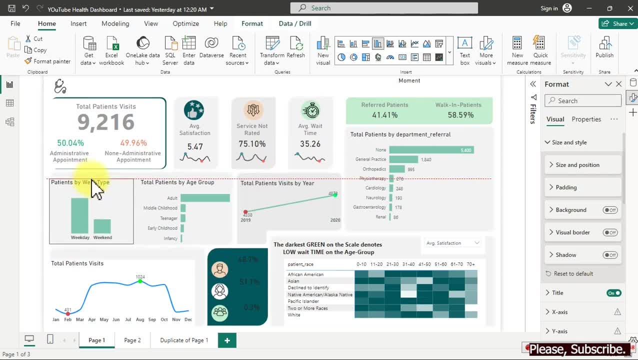 with this one here, so i'm going to do the same thing to this particular one, beautiful. so now, if i click back on this one, all i need to do now is going down straight up to where i can actually turn on the detail label for it, which is this one here. then you know the drill we're going to use. 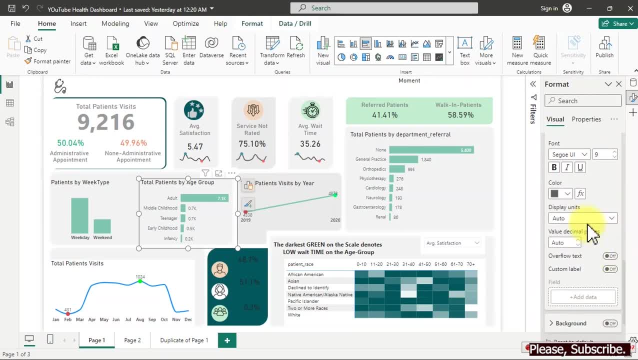 none on the value. you scroll down a little bit, you display the unit and you choose not for it. beautiful, huh. so if you think it doesn't pop out, well, you can do bold. then let's do bold for this one as well, you can do bold. that pops it out. right, then we do the same thing for this one. 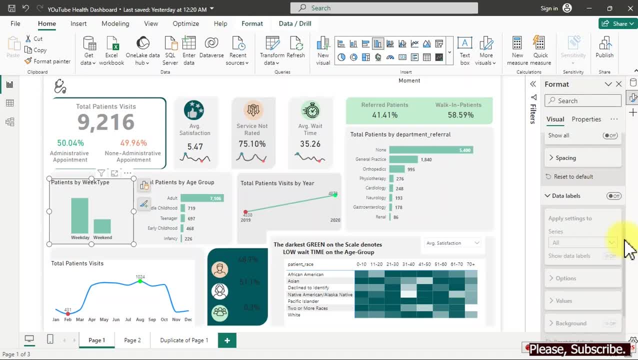 on phone for this one. we are going to go ahead and turn this on, then we scroll down a little bit and we play this one on bold. all right, if you look at this, now i want to do something. i want to use this color here for one of it, so, like for the weekend, i want to change the color to be a bit. 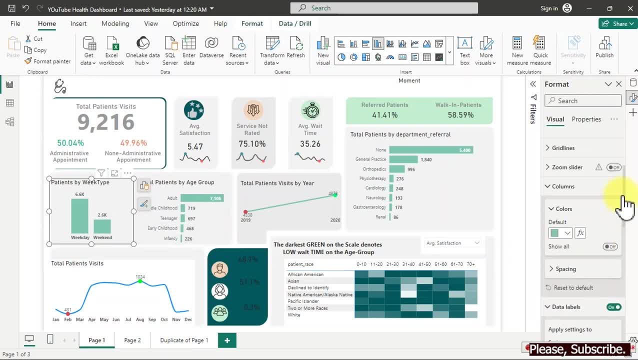 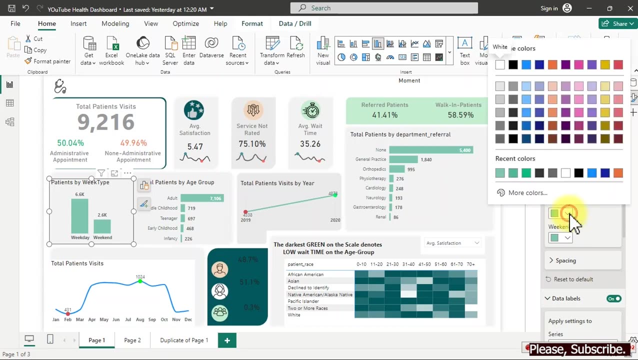 different. then i go straight up to where we have the colors. then all i just need to do is to turn on this here and i have this. so once i have this now, i can individually change the color i want for my week day. i'll leave it at this. 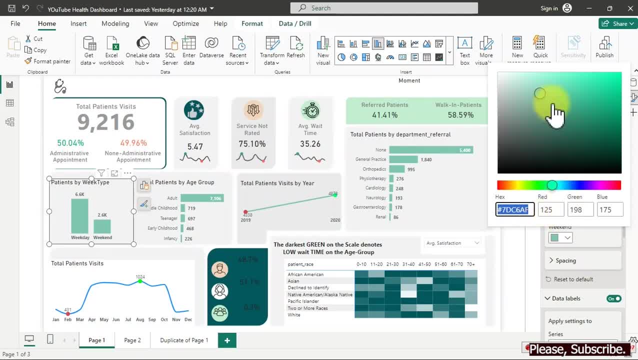 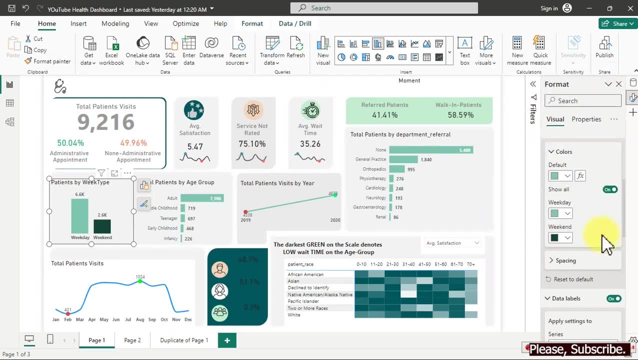 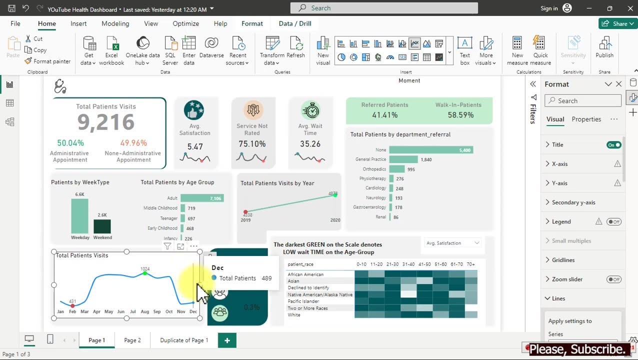 for my weekend. i would like to go a bit different. let's choose a darker form of it. beautiful huh, all right, this is what we have right now, and we are beginning to get it right. so, clicking on this one now i have to properly align it right here and make sure it sits right. and the next thing: 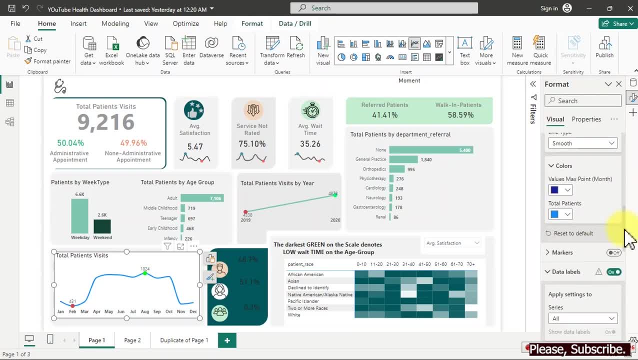 i do is to go to my line and if i scroll down on the line i have these two here. i'm going to change it to this one here and click and click on this. so now we have the color the way it should be. i want to change the chart i'm using to this. 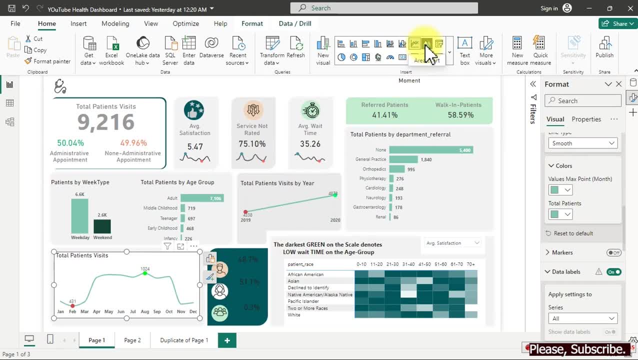 particular area chat right here, and that gives me something different. so this is what we have for area chat. we can control what we see on the area chat, specifically this particular one. i want to reduce the transparency. what do i do? shade area. then here we have it, on nine percent zero. 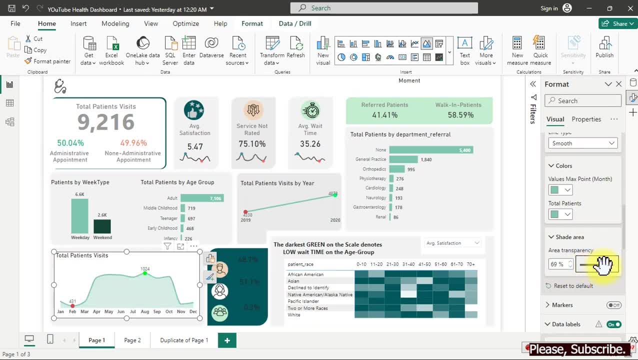 percent looks darker. i'm gonna reduce it to this level and i have something like this: this is beautiful. okay, if we are done with this, the next thing we are going to do right now is to scroll a bit up, click on size and style and turn off the background. that makes it look okay for me. good. 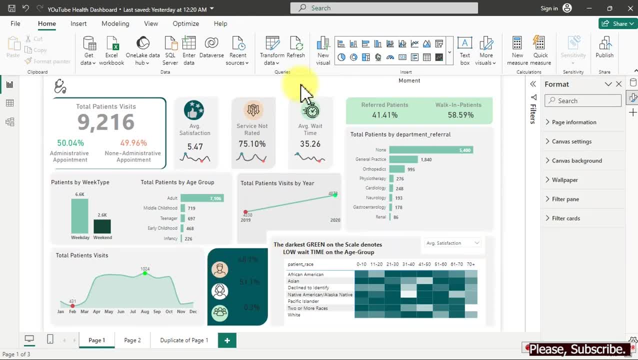 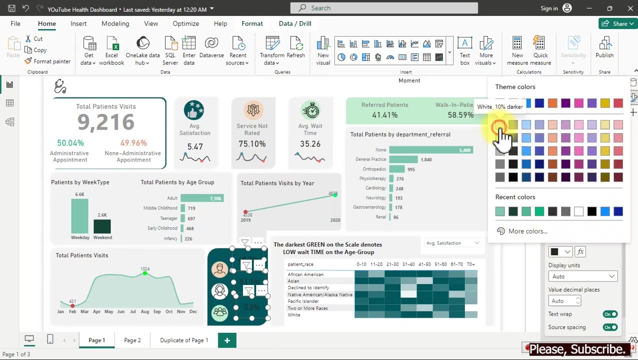 so now it's taking shape. we're getting there now. look at this particular place here. just hold your ctrl key and select all of them. quickly go to where you can actually have the color changed. so i'll come here and i'll select this so nicely done. so after getting that, we have to properly. 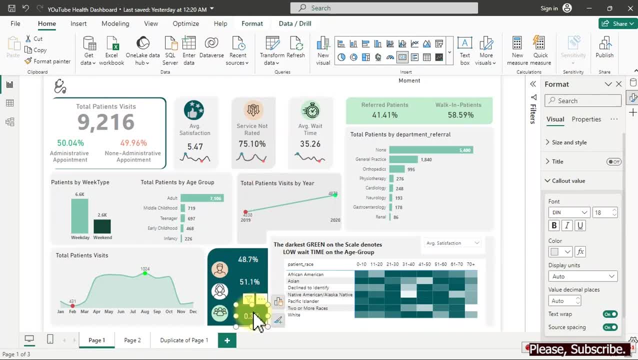 align them. i'm going to bring this one a bit down here so you can use the up and down arrow to fix this the way it should be. i'll bring this one down as well, then i'll convert here. i will bring this one down all right now. the first thing i'm going to do is to actually get this. 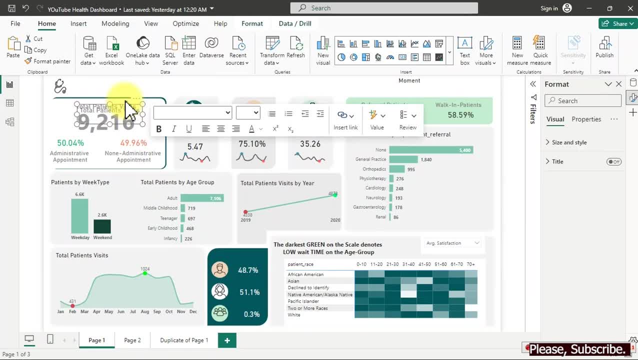 duplicated. so in ctrl c and ctrl v, that paste the one you have copied for you. you come right here and you drop it in. so what i'm going to do right now is to type in gender breakdown. so, gender breakdown, i'm going to control a. so from 16, let's have it on 14.. 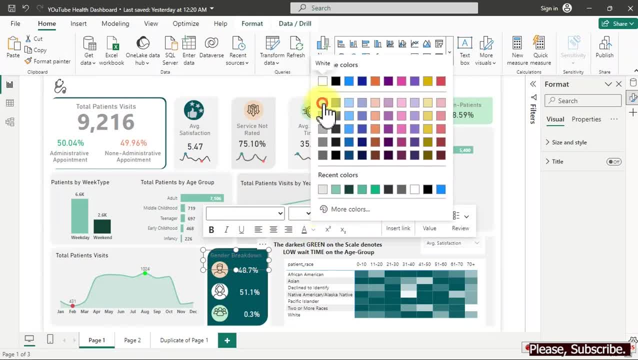 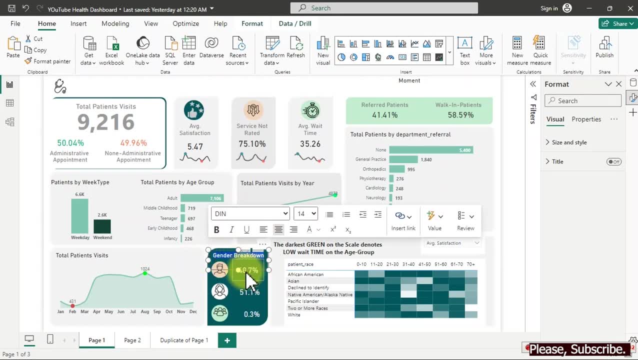 beautiful, huh. so we change the color. let's make the color a bit brighter. that is so for agenda breakdown. you can just make it this way. then, once we are subtitled with what we have, we can actually paste on that one and drag it up from there. so over here we are going to do uh mail. so for mail. we don't want. 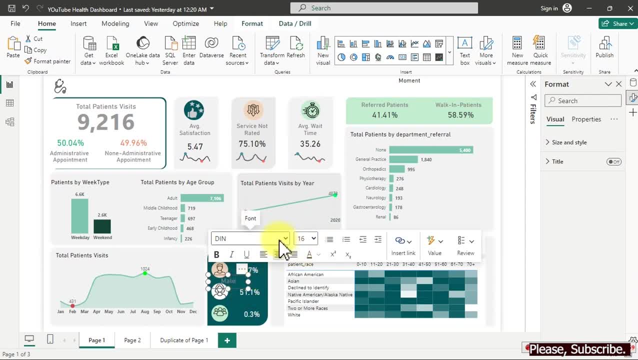 to have something as bold as this, so i'm going to go for 12.. so before we do that, ctrl a to highlight it, go for 12.. so we have 12 here. so we change the color to white, this one, so we can make it a bit smaller. so bring it over to this place. 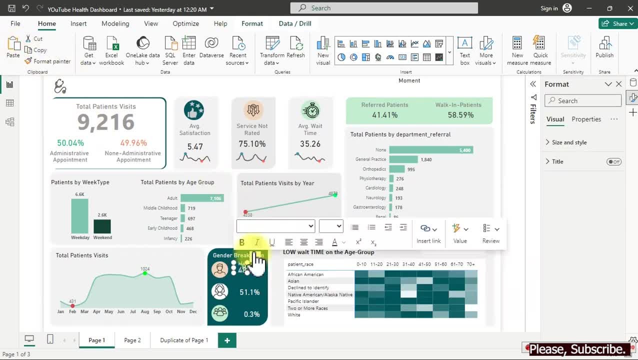 so all i'm going to do right now is just to make a copy of it and move it down. so we want to make sure that we are actually at the right gender. so for this one we turn it to male to female rather, so female, we stretch it. 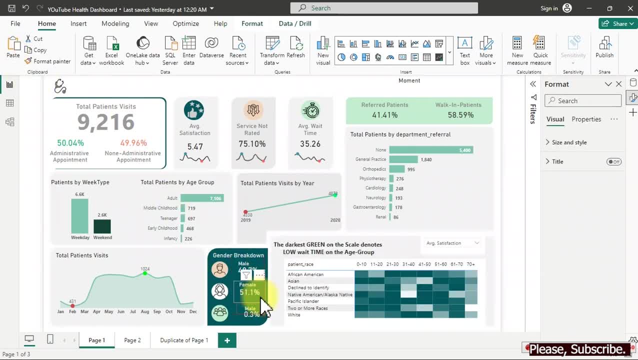 then we paste a new one, and this one is going to be unknown. so the gender of this one is not known. maybe he, she, male, or whatever, i don't know. so on this one it's going to be unknown. so i've told you. spend some time. 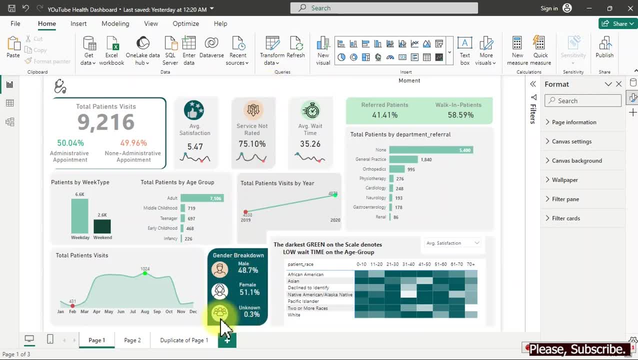 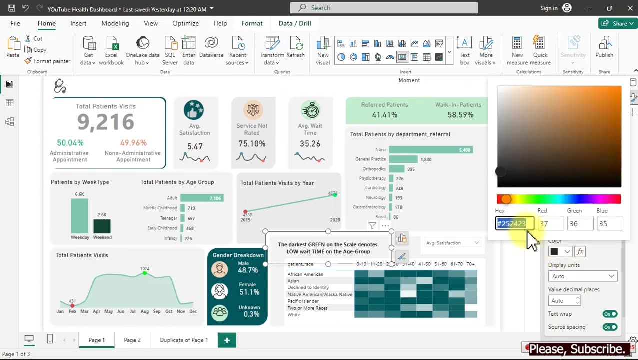 formatting this. i think i've just done something good here, better, all right, we are right here. you click on this. let's reduce it to like 11.. i'm gonna make sure i change the color. let's use a different color. i'm gonna click over here. what if we use something? 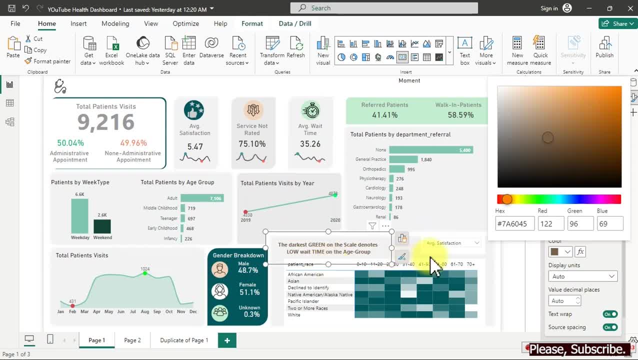 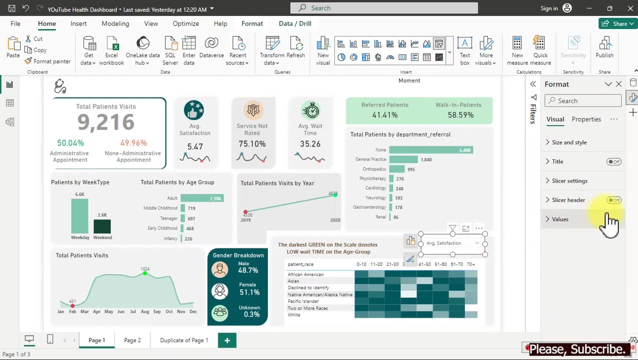 like this, something like this would be cool. right here we go. so for this one, we have here, uh, a slider drop down, so i'm gonna click on the value area, rather go on the size and style and turn off the background once i'm done. here we go. we have this. so if i open it up right now, 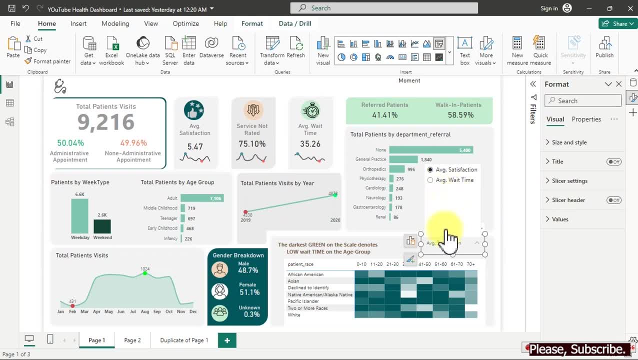 this is what we have inside, so if you don't want to have this color, what you can do is to change the color from white to any color you want. that would fill to your dashboard right now. this is what i want to have on it. okay, now, how do you make people understand what exactly is here? 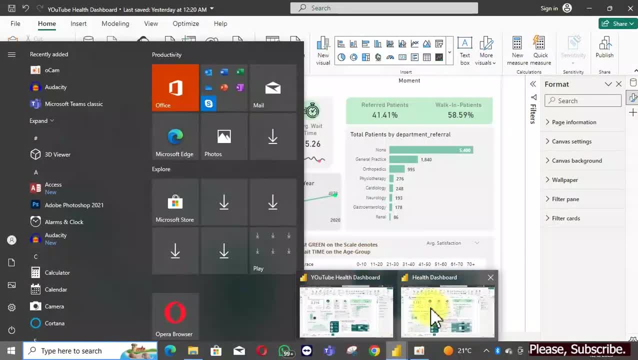 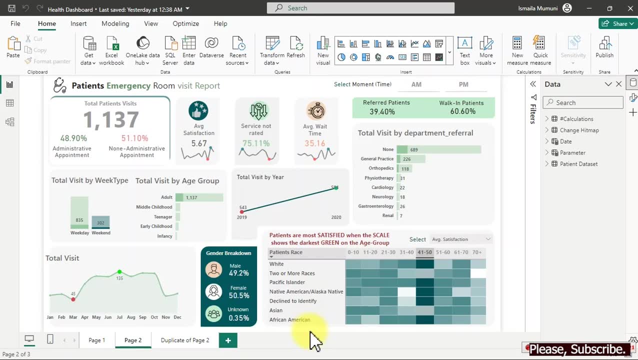 let's go to the previous dashboard we've built before this one, which is this particular one right here. if you look at it right now, this is what we have: very clean mm. just like what we have just left that we both created together, right. so now i'm gonna have to some kind of say: okay, 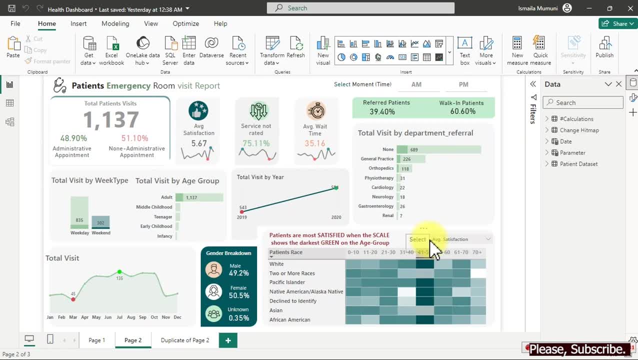 select. when i say select, that actually prompt whoever is using it that way. Let's start by typing with the battle right now to select something from here and make a switch. that is exactly what we are going to do, so let's quickly go back here and we're gonna paste a new one. we've copied. 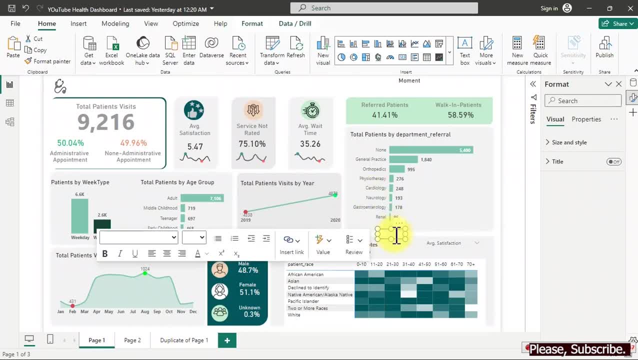 from here before and under this one here, I'm going to type in here: select what is, select a control a. I can highlight it under a and I just have to make it on 16 and for the color. let's do something like this here, so we might decide to. 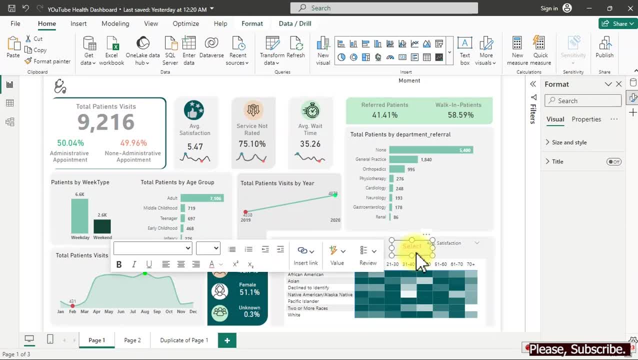 bring it down a little bit. so if we do that, what we're going to do right now is to click on this one and make sure we bring it down a bit as well. okay, here we go. we have this, we have this here. the next we're gonna do right now is, if you 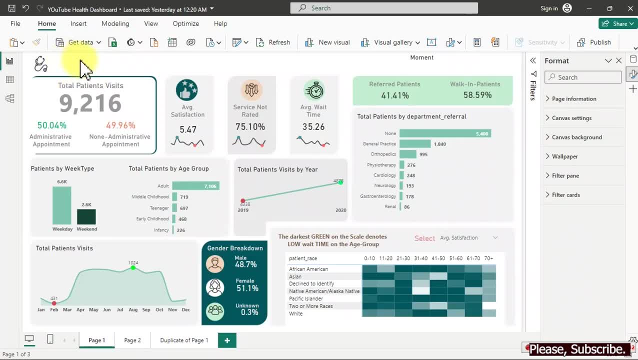 look at this particular part here. we do not have the title for it. we have to put a title, and to put in the title is very, very simple. I'm just going to get this one copied. so ctrl c and ctrl v to paste it. then we bring it up here straight up. I'm gonna have to stretch it. 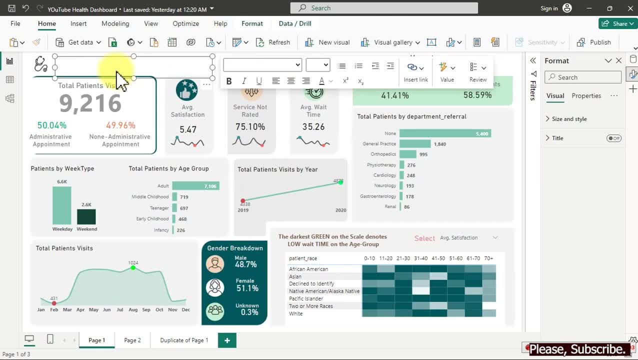 so ctrl a I'm gonna do here. so I want something on 18 and I want the phone to be on this, so I'm gonna stretch it this way. so I am going to move it close to this icon I have here. so on this particular one, I'm going to select it and, if I can make it bold, beautiful. so I'm. 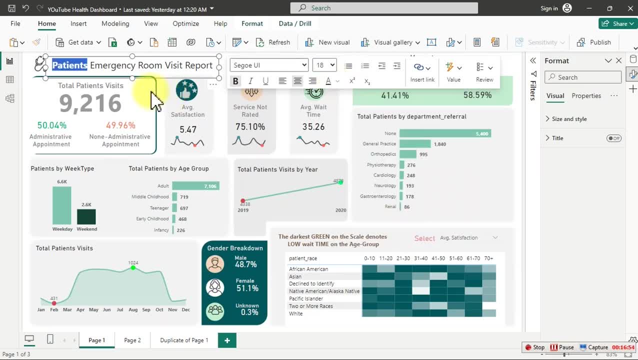 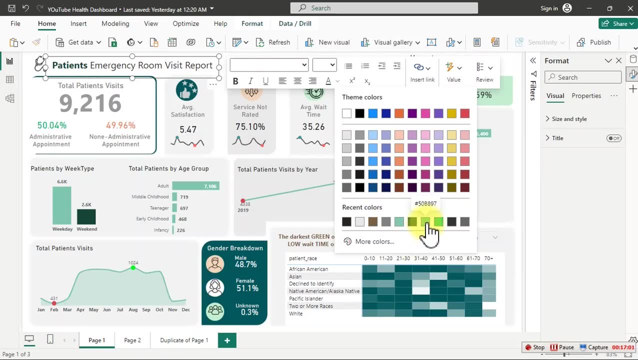 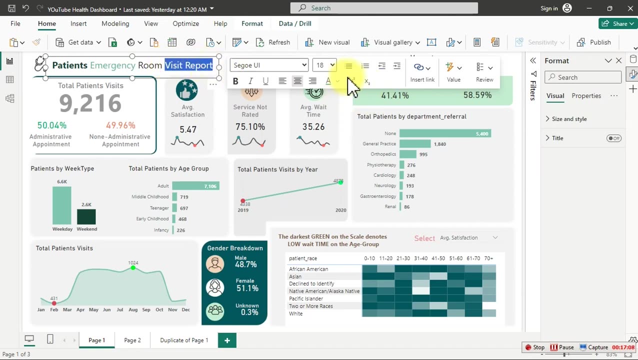 gonna use this very color for it. so for this particular one here, I'm gonna select it. then I use a different color, like this: let's go with this color, so let's find out how it looks nice. we have one more. that is our slicer here. you know, we can't forget, is so this slicer is actually, uh, the. 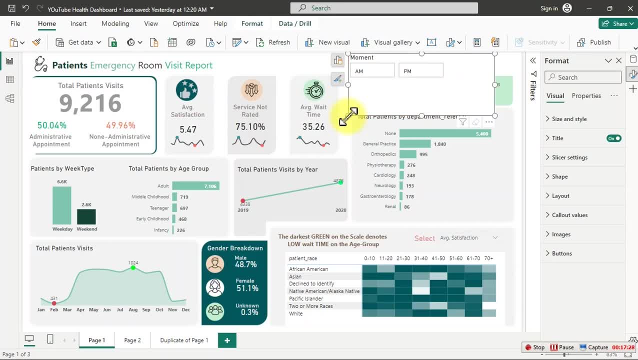 new slicer. that's probably I just roll out of recent, so we just have to make sure we touch it. But before we touch that slicer, if you look at this now it's not looking pretty fine, because what Here? No, no, no. 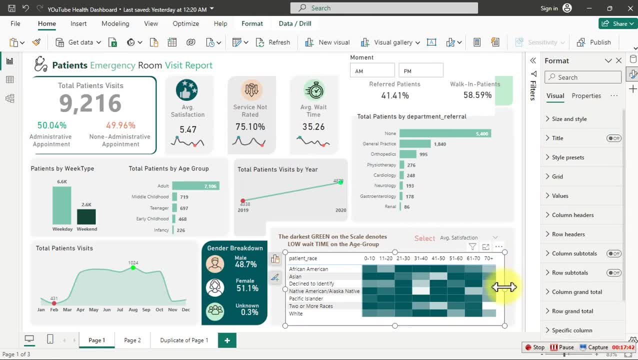 We have white background that overlay the, you know, the background we have, the real background we have. So what are we going to do to it? So let me just stretch this here. So once I've stretched it, I'm going to stretch this a little bit up here. 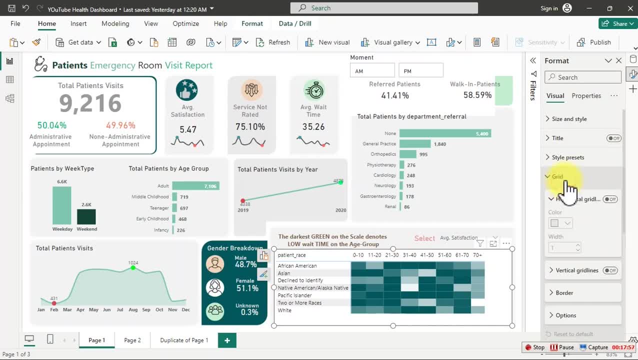 Then we have to touch this part. So quickly, I'm going to touch my grid lines, I will turn it on, Then I'm going to put it on to, for example. that opens this off for me, right? So here I have something like this: 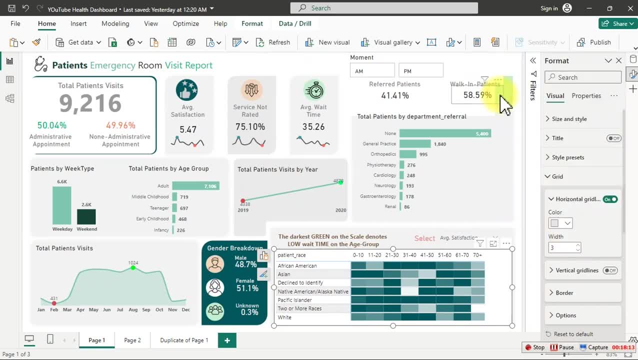 I'm going to come over here now and let's do this. Okay, we select that For the value. here, if you look at the value part, we have background for value and it's on white. Let's choose this color. So we select the alternate background, which is this one is on white. 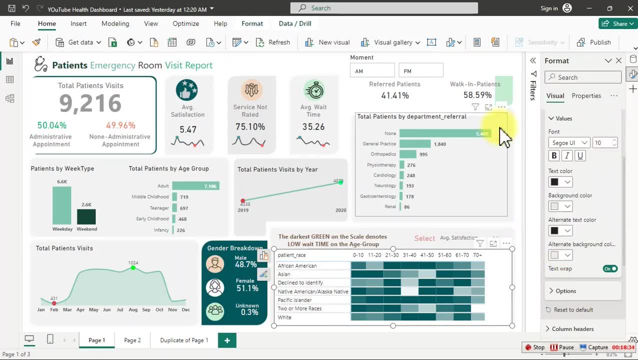 Let's choose the same color. That gives me something not really quite what I want. So what I'm looking forward to having is actually something that looks like the main background, because I want to actually bring the background up. So what can we do? 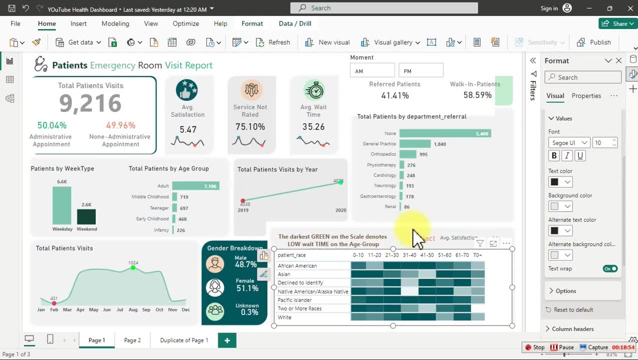 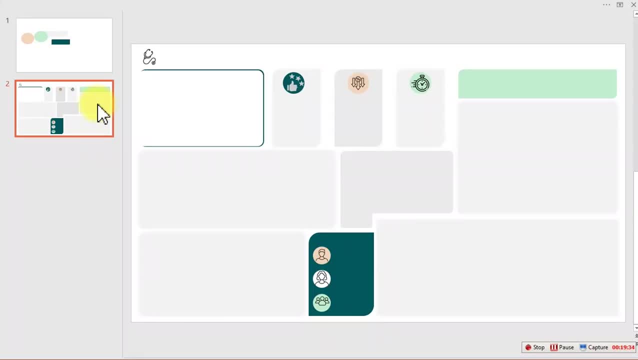 We have to go ahead and copy the same background. we have here the same color. if we can't really understand what color is it. All right, as you can see, here is the color. All I just have to do is to go ahead and bring the color code over. 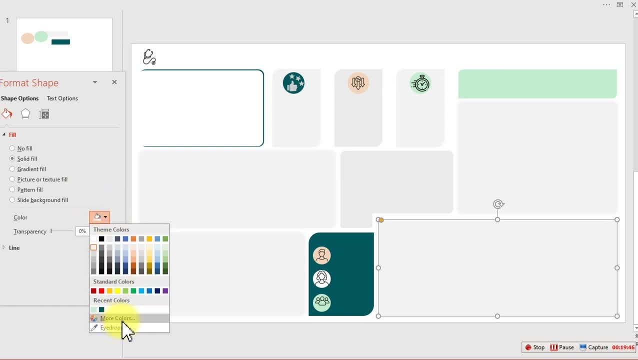 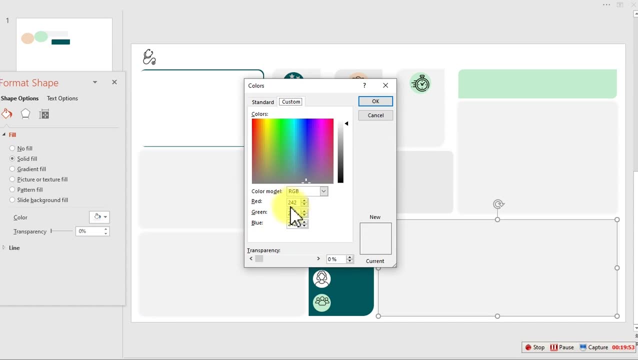 Here we go. We choose the color code, so we can go ahead. So if you don't have the hex code on your own, all you have to do is to understand what the color code is. Red is 4-2 or 2-4-2-4 and all of it is 2-4-2-4.. 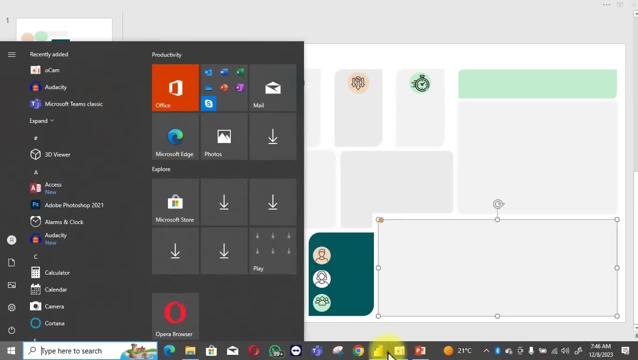 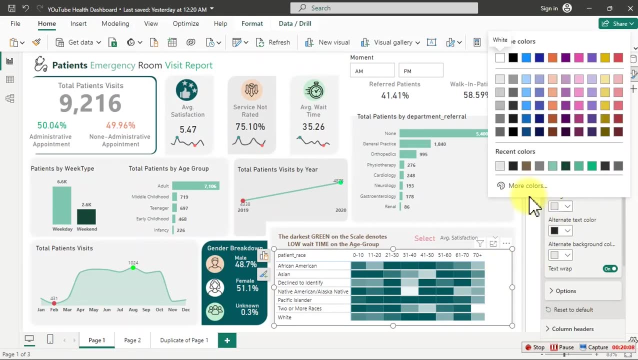 So we're going to use that. Let's quickly go back to our Power BI desktop. So, on our Power BI desktop, when I click on this over here, I'm going to click over here. So I'm going to do 2-4-2 and 2-4-2 again. 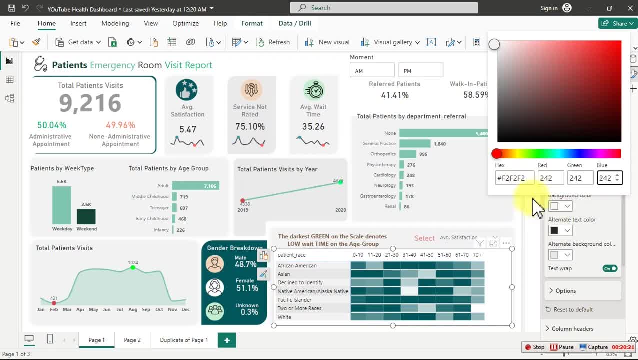 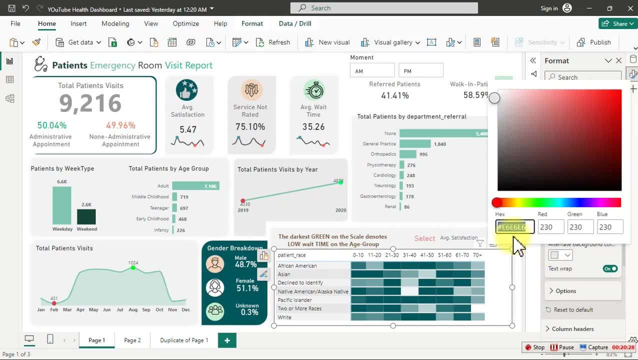 We do 2-4-2.. This is it. So now, this is the hex code for 2-4-2.. And if I copy it and I come over here, I paste it down in here. That has changed this for me. 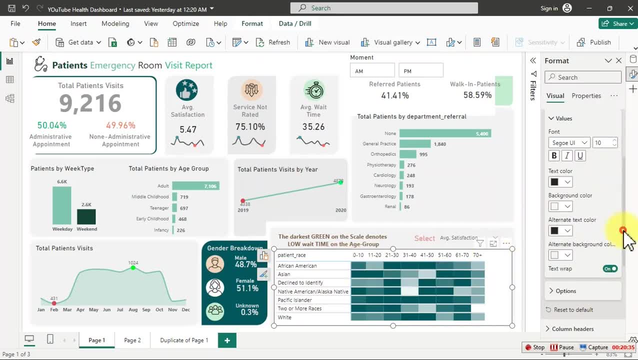 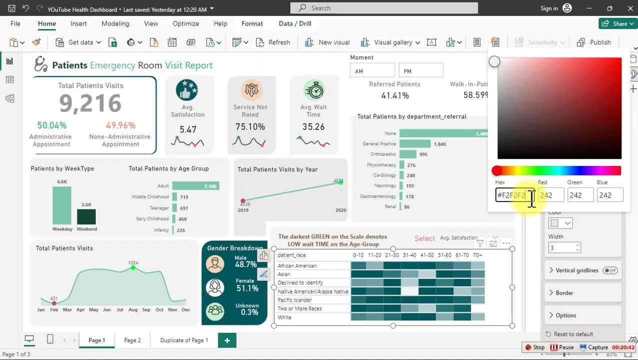 So what I'm going to do Quickly now is go over to my grid. So we come over here. We're going to use the same 2-4-2 over here. That is beautiful, huh. So now here we go. 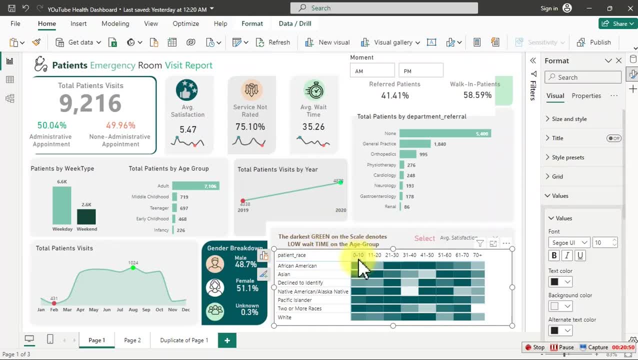 We have something like this Now quickly for the header: it's not standing out at all. We want to change it, So what we're going to do right now is column header here. So for column header, we can bit free, increase it like this: 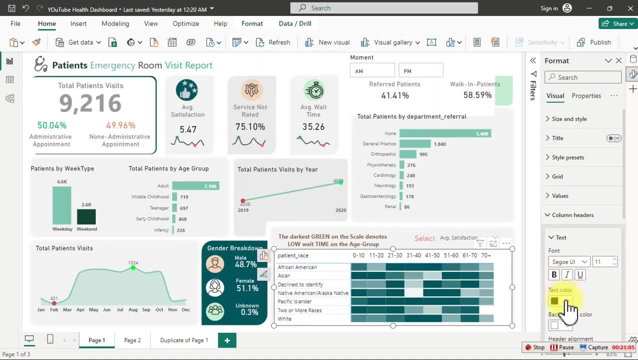 Then we go ahead And change the backgrounds to look more like this one That's separated from the background for the main background we have. You get it Okay Now if I change it from here to different one, like this one right now. 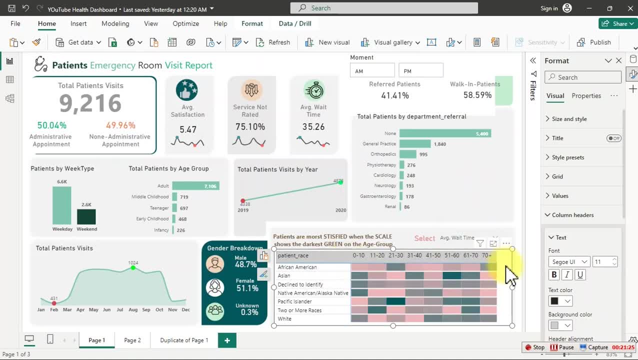 This is what we have, So, right away, I'm going to have to fill this particular gap here, So all I need to do is just to stretch this particular part. That is beautiful. So, So we have something like this: Do you get it now? 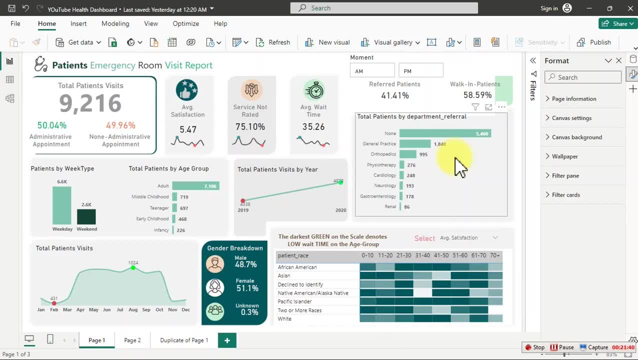 So it's looking more, much more okay, So nicely done. If you are very much satiated with what we have done here, let's go ahead and start formatting this one. On the format of this one, what we're going to do now is we have clicked on it. 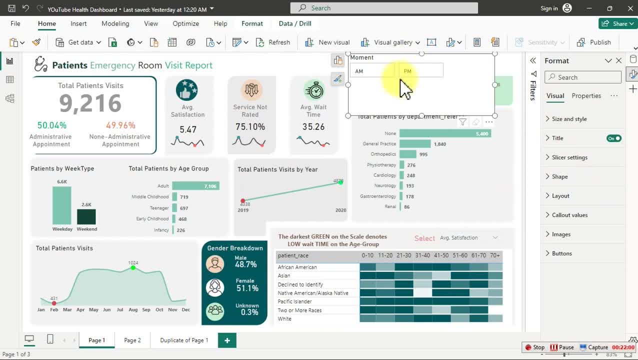 The very first thing we're going to do is to actually turn off the detailer bill. And you look at it, If I start to do this now, It decides some kind of you know- getting distorted. So first of all, I'm going to turn off the title. 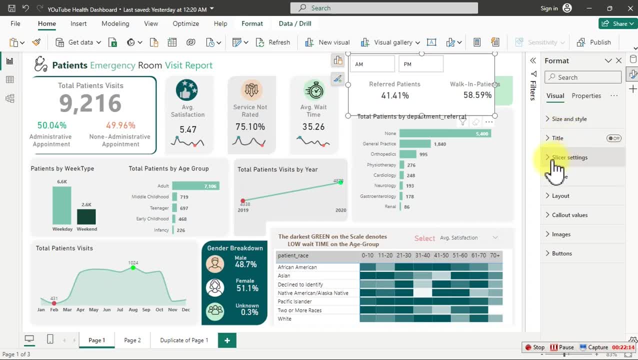 We don't need it, Right? So let's go to the slicer settings here And what you have now is actually select a single selection. I'm going to turn off the single selection so we can select multiple. That is good. So we have the shape. on the shape, we click here. 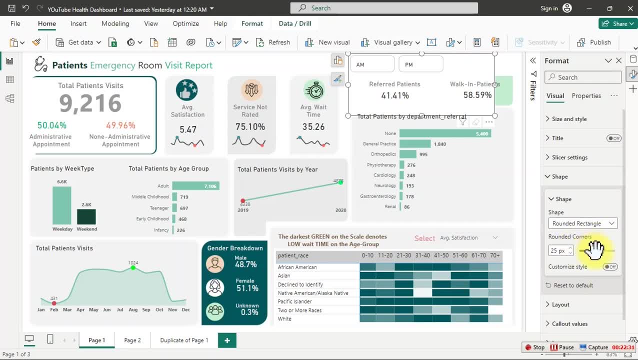 You can select this particular kind of shape, so you have the ability to actually change it to what you want. If I click over here now, you can actually- you know- mess around with what we have here, But here we go. Can you see it now? 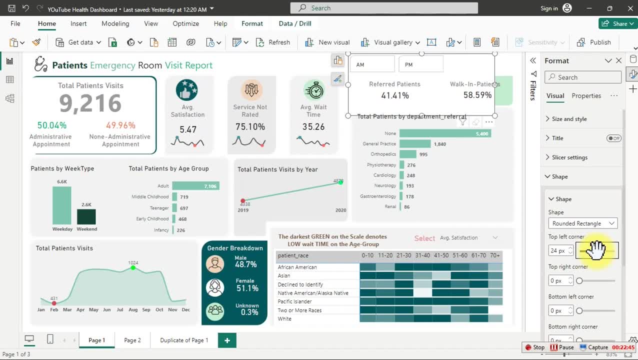 Can you see it? I'll let it. only one top left is actually the one that is. you know this way, Like I love it, So let me leave it. that way I can close it and go to the layout here. 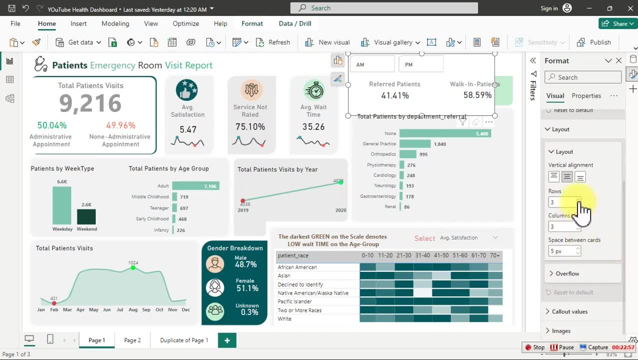 On that layout. you want to see how many rows you want to have, So let's have more than that. So I'm going to have just two columns for two columns. I feel this right. So you have this particular part to play with, to know what exactly it is. 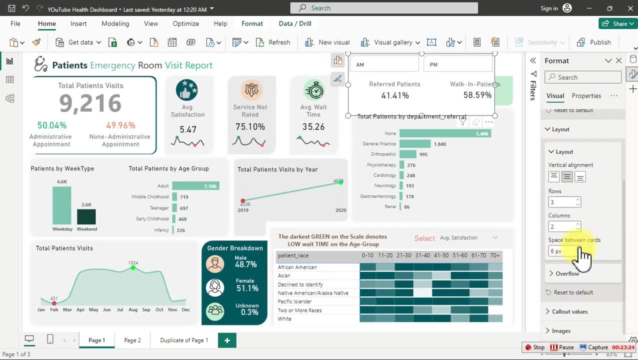 So if you don't play with this, you wouldn't know what it is or what it does. Mostly she just scared of like I don't know how to use it. So coming here now when we do this, it's still getting distorted. 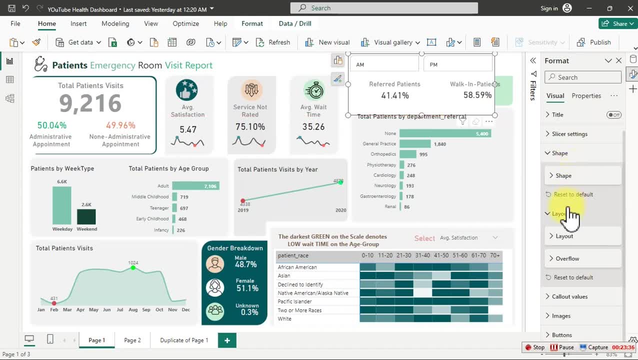 What do we do? Let's close the layout here. So here we go for shape, crazy shape overflow. here You can see. Go right Here and test it out and see what it does is a new stuff You just have to explore. 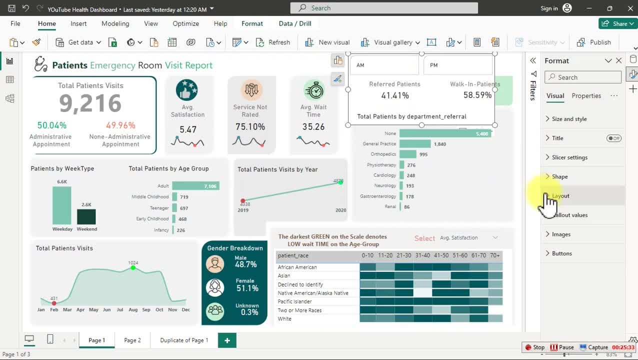 All right, In order to fill this particular place up, let's go back to layout. on the layout, We turn this one to one. that field is up for us, right? So we can now come here and make it this way, Right? 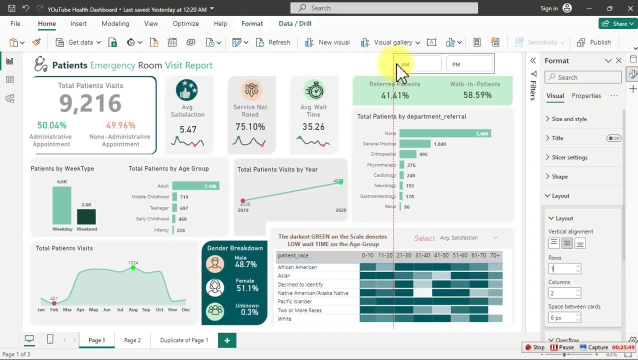 But don't allow the text to disappear. Then we can do stuff like this. Now we have achieved this, but we don't actually want to leave a button like this. We want to make it a fill of the website. All right, Right here. 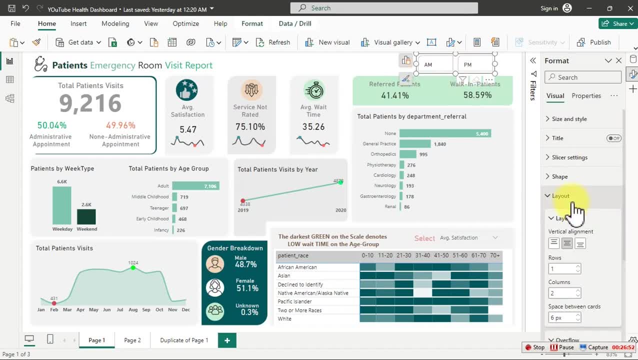 So let's do something: Click on it, close it And while we get to the button here, we can play around with the button. Now, if you want border, we can have border. We turn off the border. It looks plain as this: 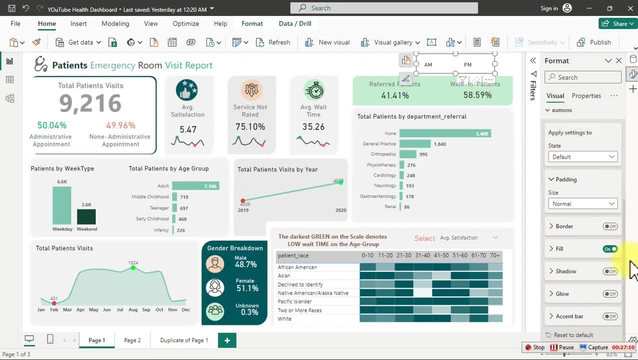 All right, so if I scroll a little bit down here, now we have okay, so here we have it. Extent bar. I'll turn it on, so we can not choose the position. we want that to be. open it up and let's choose the position. 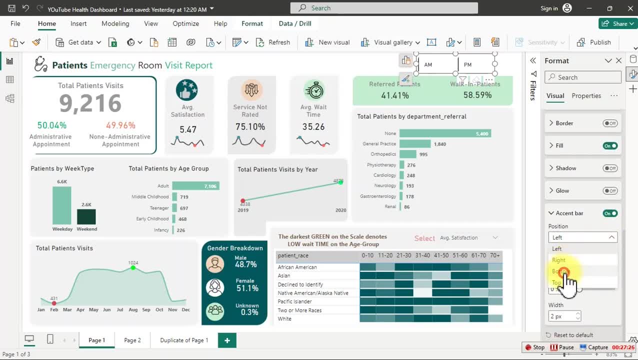 Now we have it at the left hand corner. We can decide to have it at the bottom. This is what we want, right? So I'm going to make it some kind of not to appear this way, Right? So What I'm going to do next now is go to the state here. 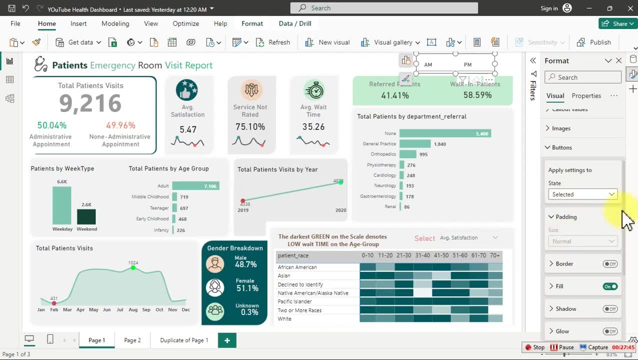 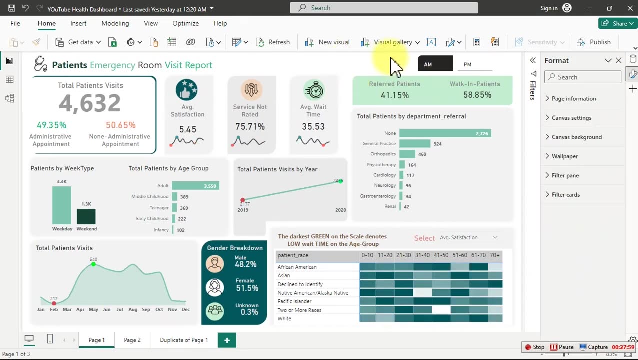 I'm going to choose selected. for the selected one, I want to go ahead and release the transparency, put it on full. So now, if I hover over it, nothing happens By the time I select. now we have the state to be like this: 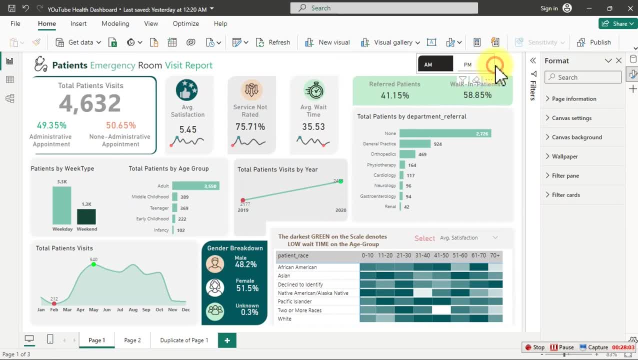 When we have a selection, we don't want to have a field color, We want to remove the field color. So we put it on Selected and we change the field color to blank. So when we change the field color to blank, what happens to the text we have in it? 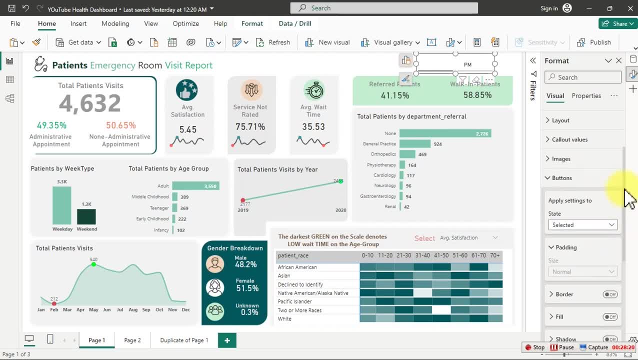 That means we have to touch the text we have on it. So we locate where we have the call out value right in. So the call out value here. So we go where the heck is that? So let's choose the selected As well on the call out value. 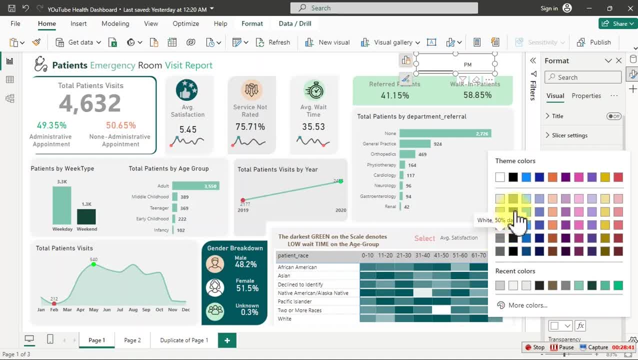 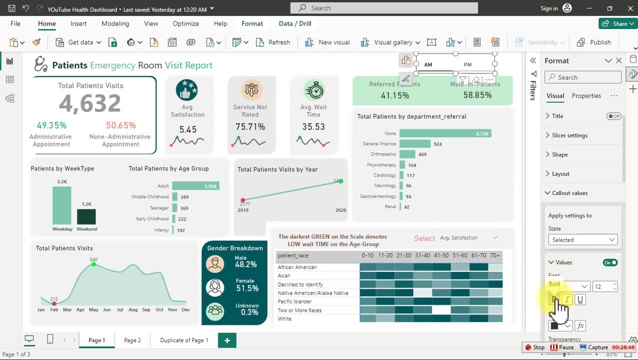 Now, we can now choose a dark color. Can you see it? now We have a dark color, so we can even make it bold because we have selected it Right. Or you can unbold it and come over here. Select under font. that will look bolder when we are under selection. 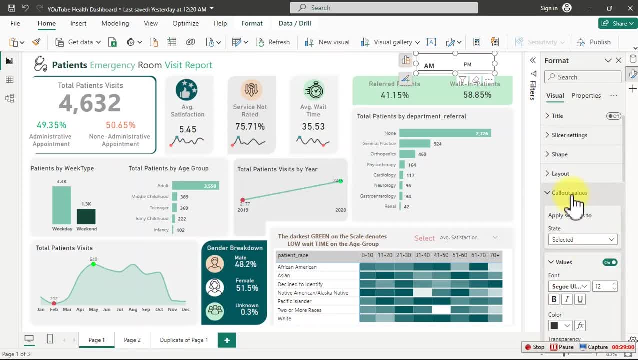 We have something like this: You get it now. So if this is what you want, let us reduce this like this: Okay, So Let's say we are cool with this. When we hover over it, nothing happens, But when we are under selection, what we have selected is has more bold on the line.